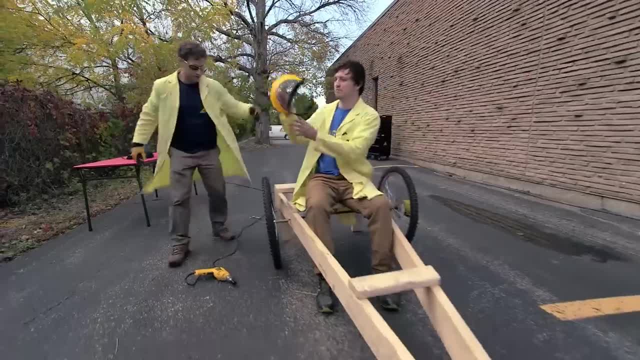 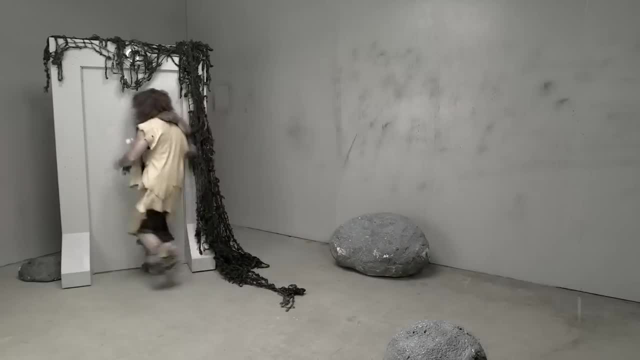 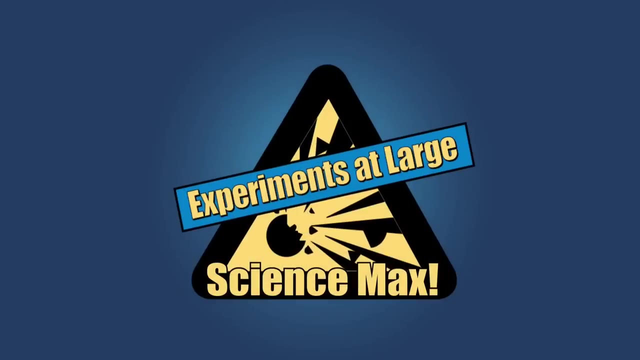 Science Max: Put on your helmets. for this episode of Science Max, We try to build a human-sized cart powered by inertia Plus Newton's laws, from a caveman to crockery. Inertia on Science Max, Experiments At Large, Greetings, race fans and Science Maximites. 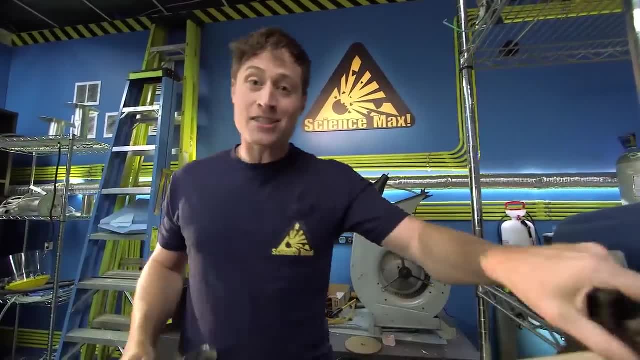 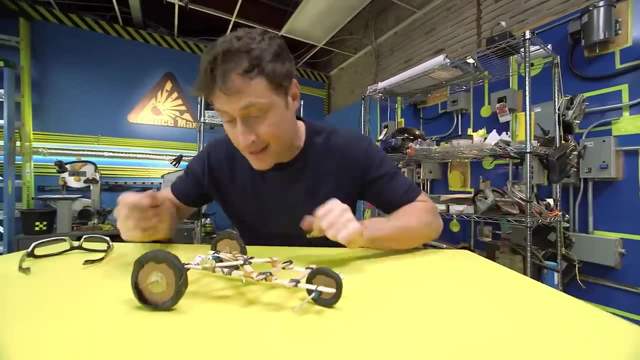 I am Phil McCordick and this is Science Max Experiments At Large. Today we're going to be experimenting with the drag racer. Pretty cool, It works like this: You pull the string and get the wheels going really fast, And then you let it go and it just drives away on its own. 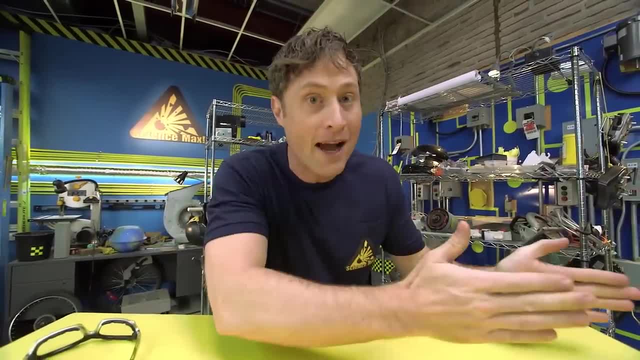 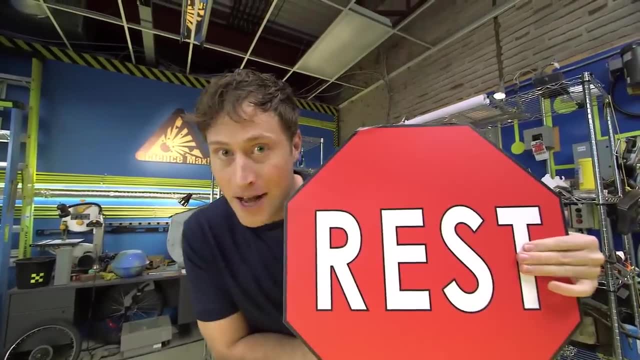 The interesting thing is I don't have to push it, It goes by itself. It all has to do with Newton's first law of motion, which is: an object at rest tends to stay at rest and an object in motion tends to stay in motion. 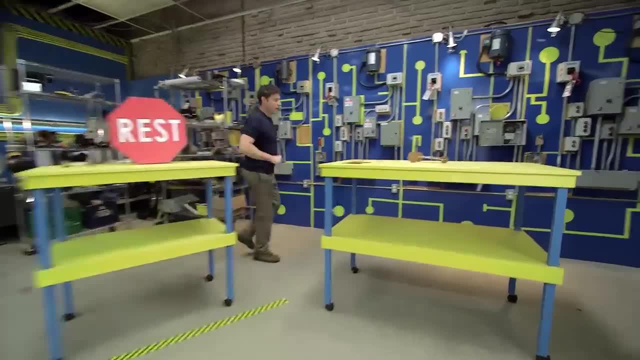 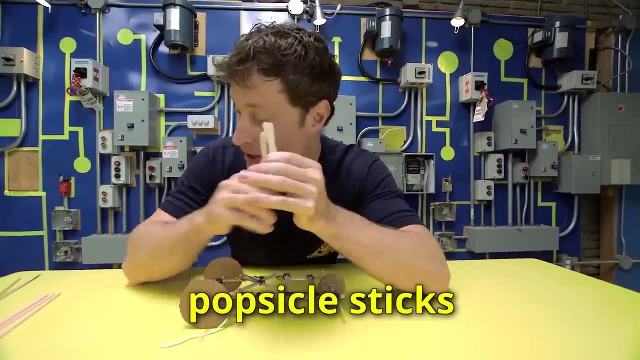 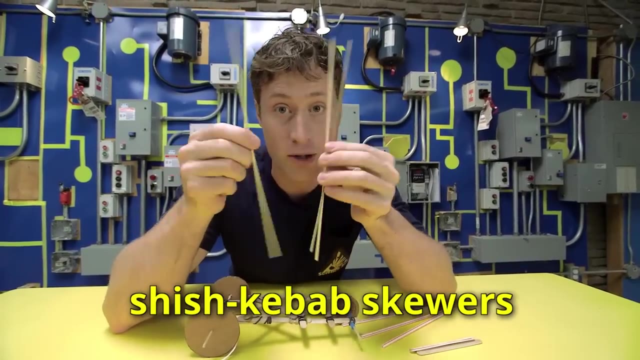 Yeah, Let's get building. Here is everything you need to build your very own dragster. You need some popsicle sticks, some straws and some shish kebab skewers. I love these. You can get these at the grocery store. 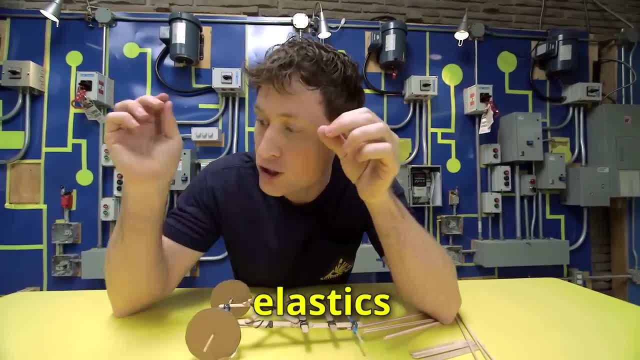 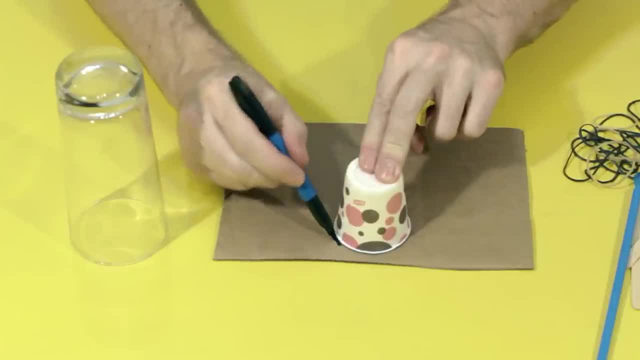 Let's see Some elastics. And of course you want wheels, And I just cut my wheels out of cardboard. So here's a quick explanation of how to build your dragster. First, use anything round to trace three circles out on your piece of cardboard. 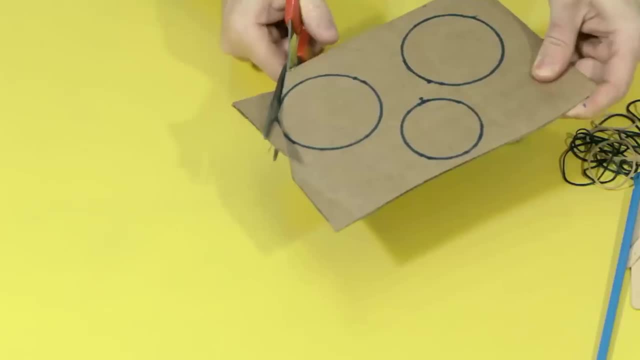 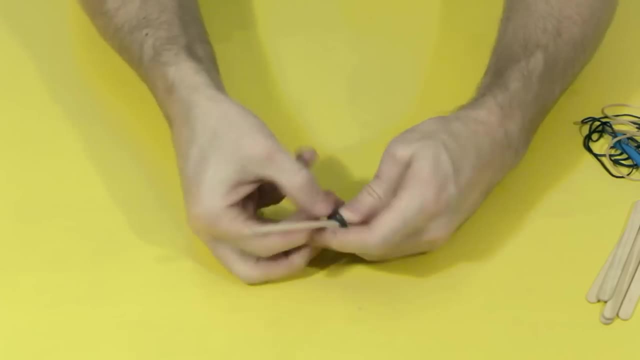 Remember, you want two big and one small circle. Then cut out your wheels. Then it's time to make the frame of the dragster using popsicle sticks and elastics. Just put two popsicle sticks together, then wrap the elastic band around them to keep them together. 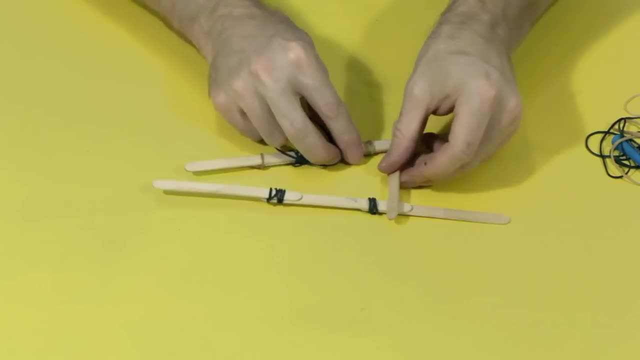 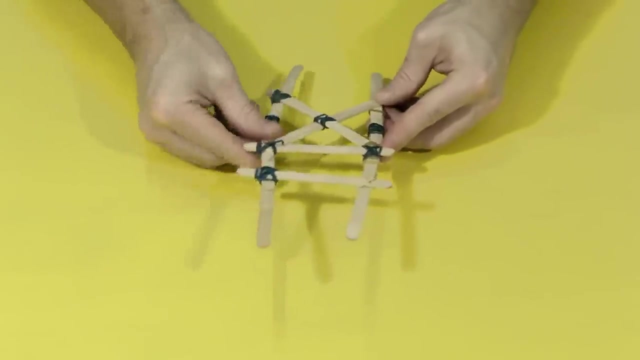 First you build one side, then the other side, Then add some pieces across the middle to give it support. Remember not to put any popsicle sticks too near the ends, because they'll get in the way of your wheels. Next, cut the straws into small pieces. 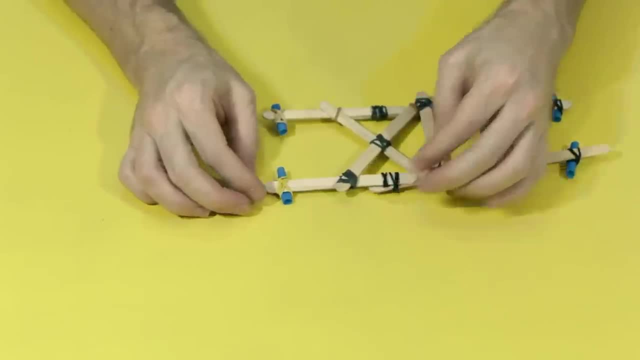 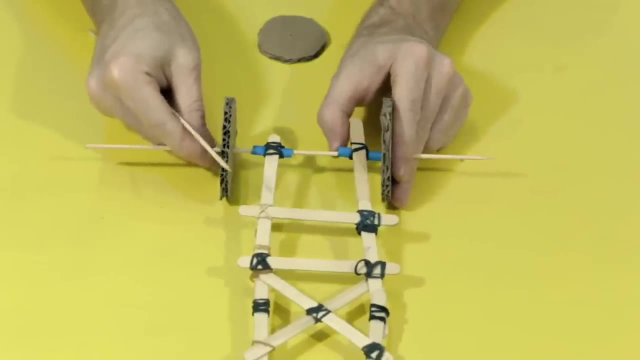 and use an elastic band to tie them together. Tie them to the ends of the popsicle sticks. Then it's just a matter of sticking the shish kebab skewer in a wheel, passing it through the straws and sticking on the other wheel. 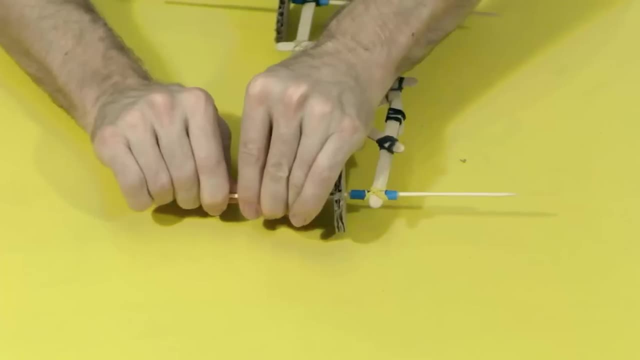 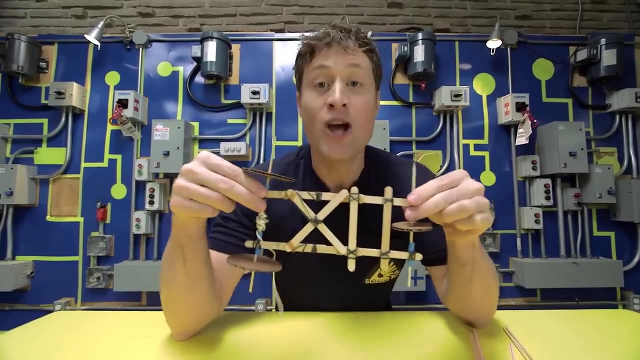 Don't forget that the small wheel goes in the middle at the front. You can trim the skewers afterward by just breaking it off short. If you want step-by-step directions on exactly how to do this, you can go to our website. It's all right there. 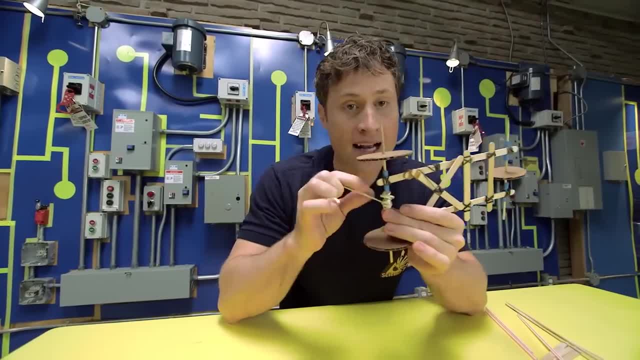 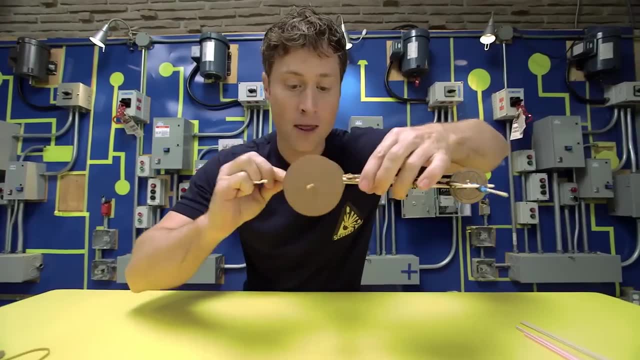 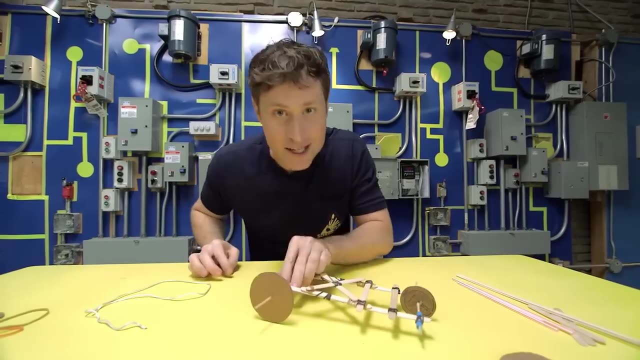 Now the last part is wrap some string around the back axle so you can pull and the wheels will spin. Let's check it out and see how it works. Didn't work that well, did it? That's because we haven't added the secret ingredient. 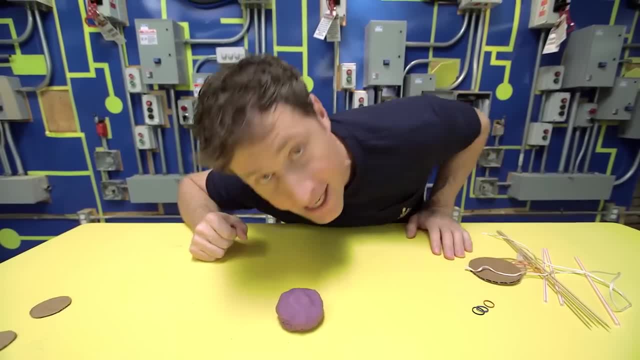 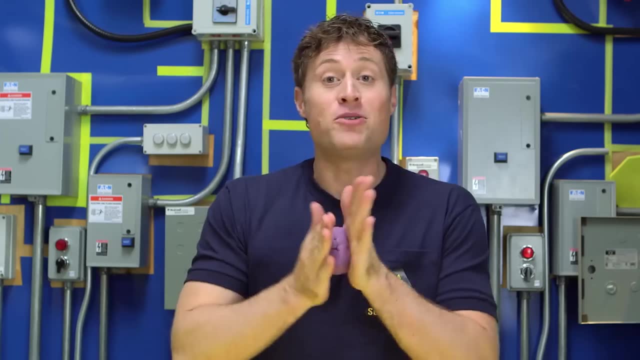 Plasticine, The perfect secret ingredient for all of your dragster needs, And also sculpting, because that's what it's for. Remember how I said: an object at rest tends to stay at rest and an object in motion tends to stay in motion. 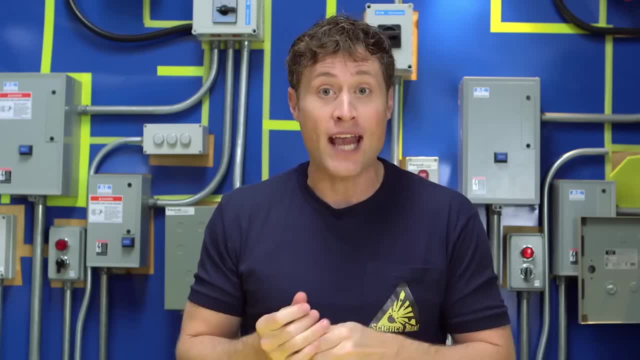 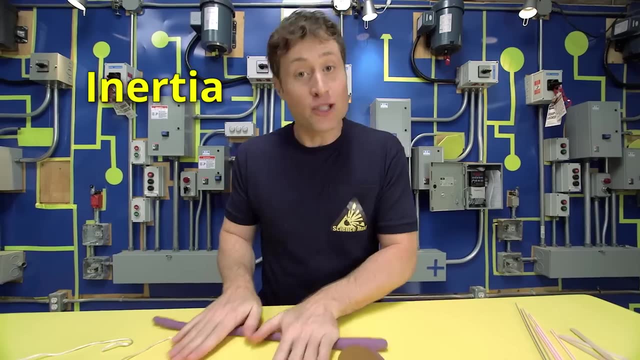 Well, the heavier something is, the more force you need to change its direction: either get it moving or make it stop. That is called inertia. It's the tendency for an object to resist a change in motion: either getting it going or making it stop. 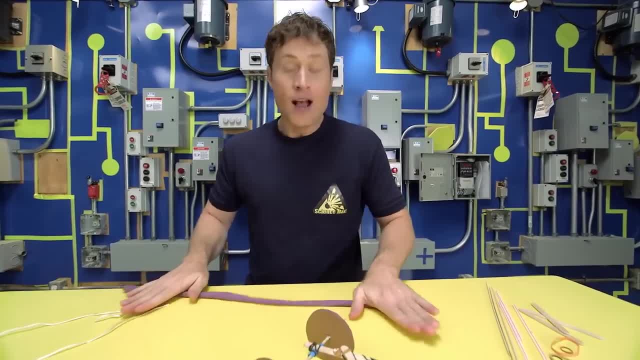 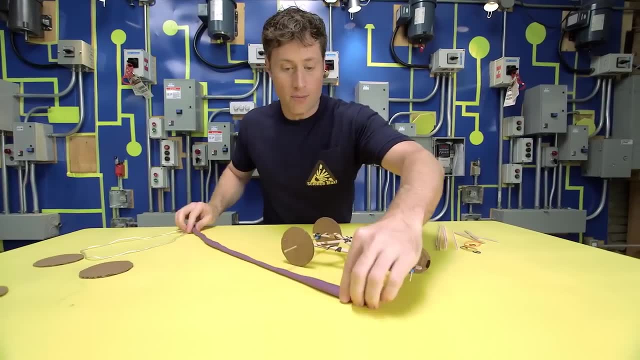 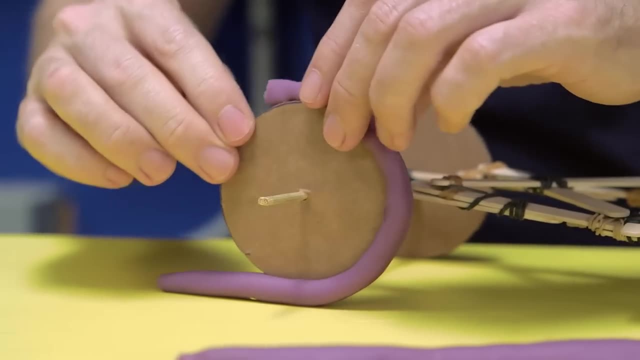 So the heavier we make the wheels of our dragster, the more they will resist a change in motion. So what I've done is I've stretched out my plasticine and then you roll the wheels of the dragster around in the plasticine. 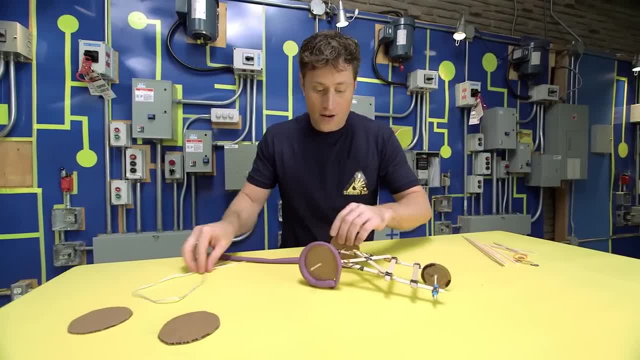 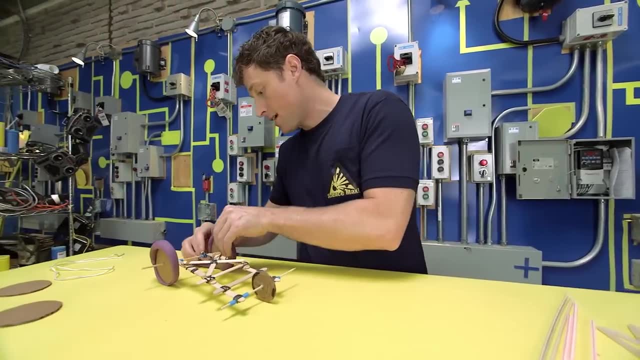 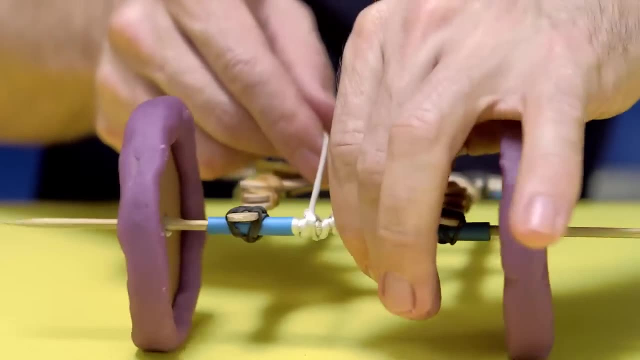 and this will make each wheel way heavier than just the cardboard by itself, And it will make it much better in terms of keeping the dragster going, because if the wheel has more weight, it will have more inertia. Now I have to wrap the string around the back axle. 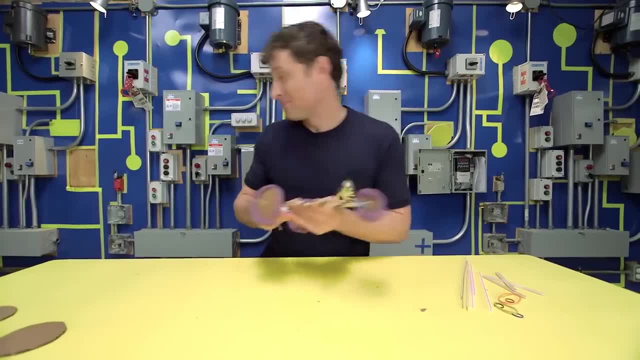 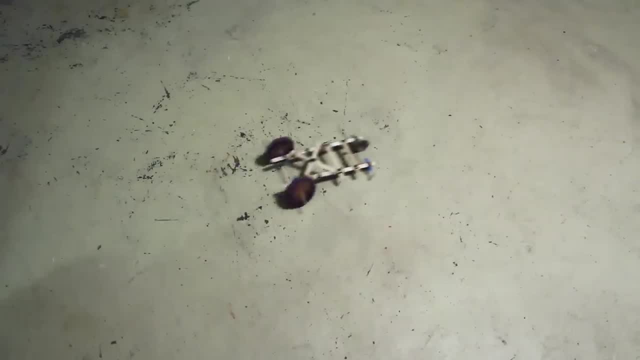 just like that. and there we go. All right, let's try it out. All right, let's give it a shot and see how it works. Pull on the string, get the wheels going real fast, and there it goes. Now, of course, this is Science, Max Experiments At Large. 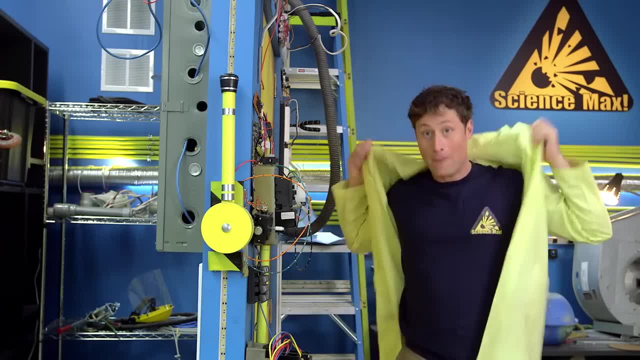 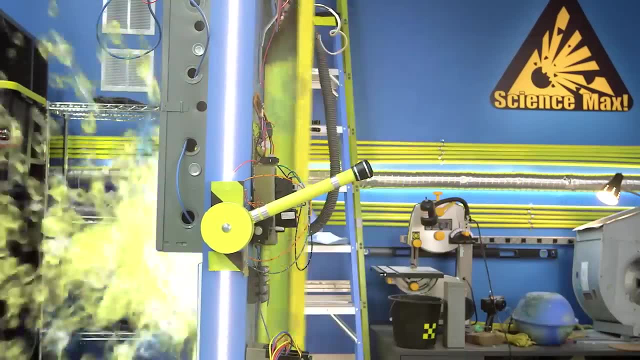 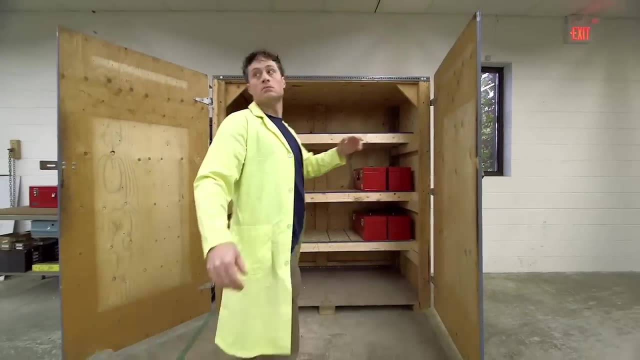 and we are going to do it again, and we're going to do it much, much bigger. That's why I'm going to the Center for Skills Development and Training. I thought it was bigger. All right, here we go, Oh. 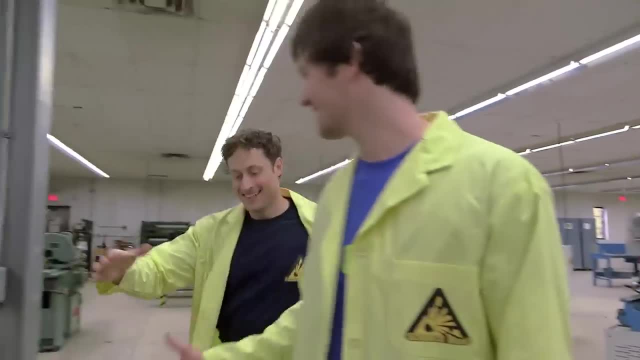 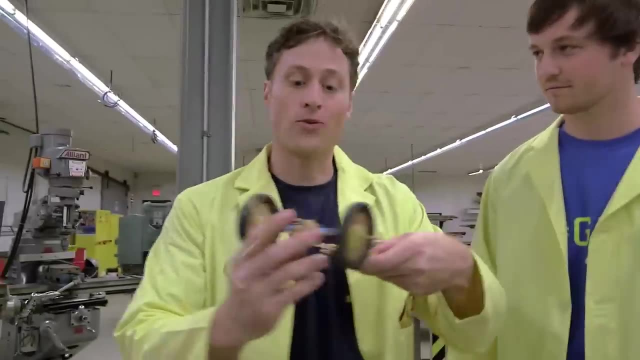 Right, Hey Chris, Hey Phil, How you doing? Chris is from Logix Academy, Logix Academy, And he is going to help me max out our dragster. Now. you guys at Logix Academy go into schools and build all kinds of cool stuff with the students, right? 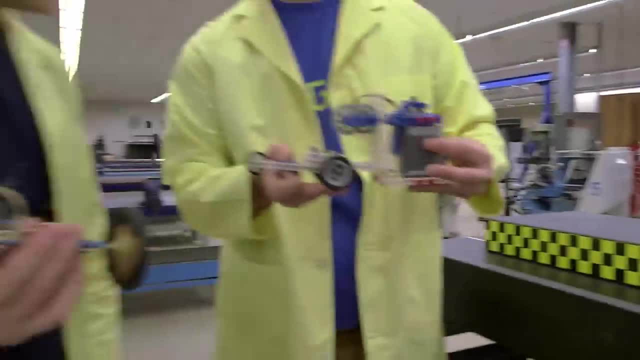 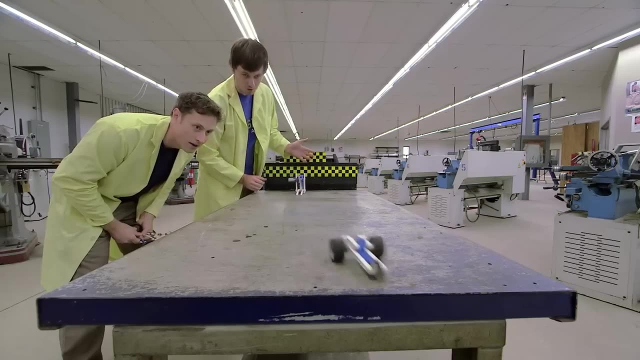 That's absolutely right. This is our dragster over here, actually, and this one has an electric motor, which is kind of fun, And these gears touch. Ooh, I like that, And Oh, all right, See, our dragster works on good old human power. 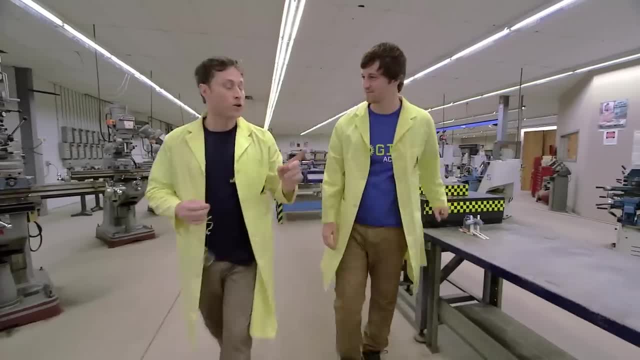 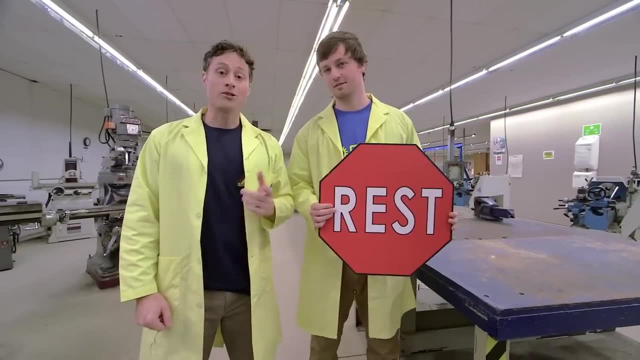 You pull the string, and There it goes. Now you have a physics degree, right, I do, Which means you know Newton's first law of motion. Of course, An object at rest tends to stay at rest, And an object in motion tends to stay in motion. 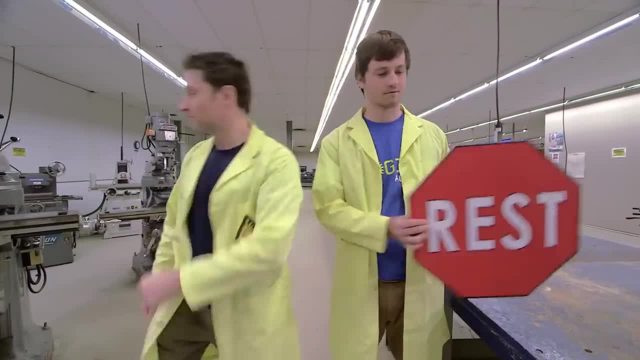 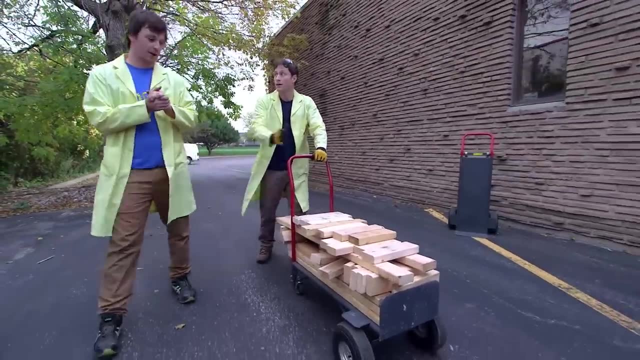 I thought it was going to come from over there. All right, Chris, I want to make a dragster big enough that we can ride Whoa. Okay, Well, it's going to have to be pretty big. Yeah, I think we have enough wood, though, right. 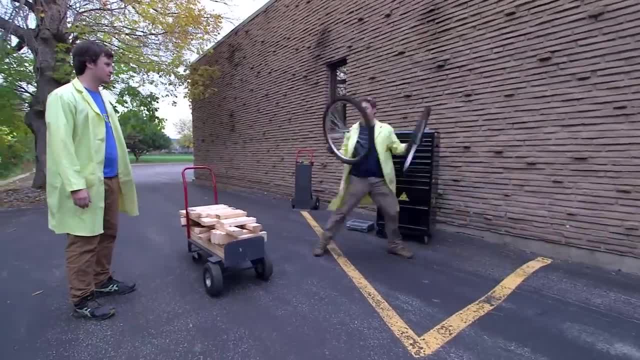 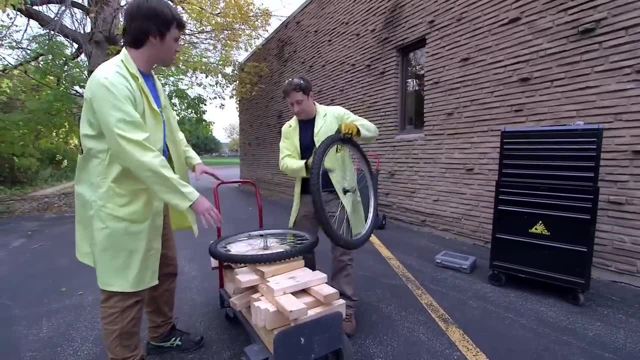 Yeah, Looks like it. Oh look, I've got some wheels. Perfect, These are bike tires And I filled them full of air, so they're bouncy. Check it out. Excellent, Whoa, Okay. So yeah, we build our frame out of wood. 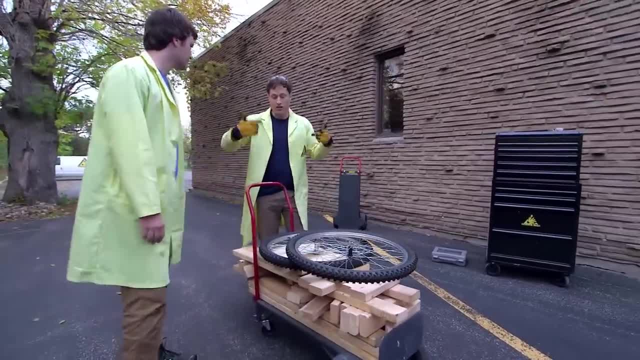 Yeah, attach the tires on and then find a way to get them spinning. And if the tires are spinning, Yeah, we don't actually have to push the cart because it'll just go on its own. That's the idea. 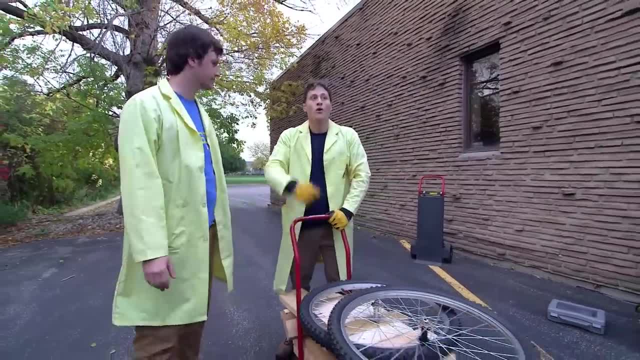 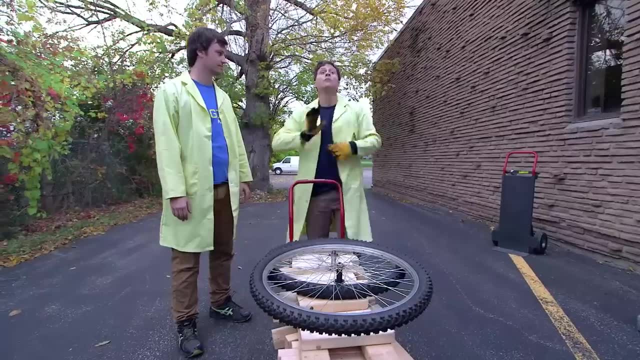 The inertia should carry And the wheels should carry us down the track. So in this case, the object in motion is the wheels, That's right, And it wants to stay in motion, which means that when it hits the ground it'll push the cart. 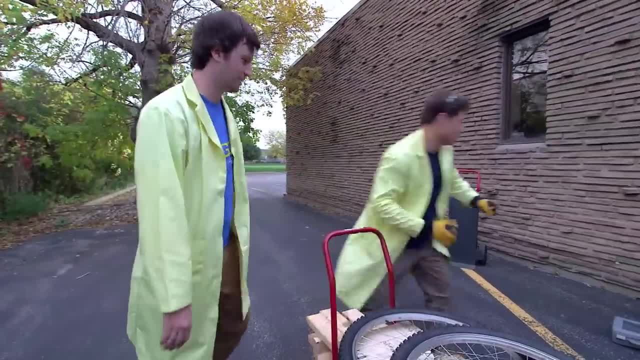 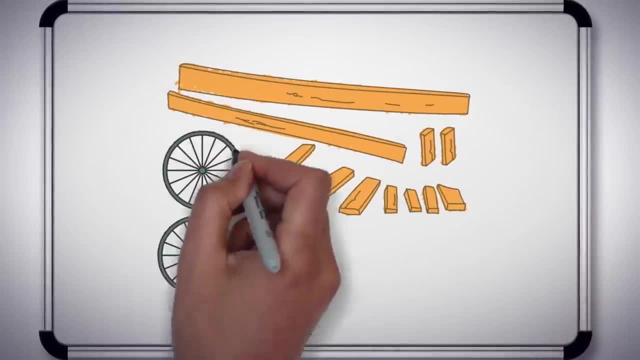 And hopefully us too, And hopefully us too. All right, Let's get building, Let's do it. So Chris and I get to work building the dragster. Our maxed-out version is going to look just like the popsicle stick version. 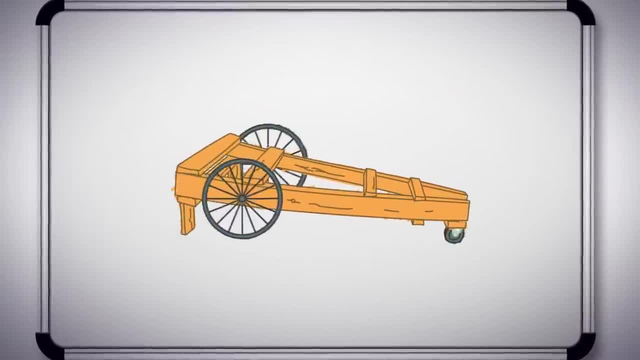 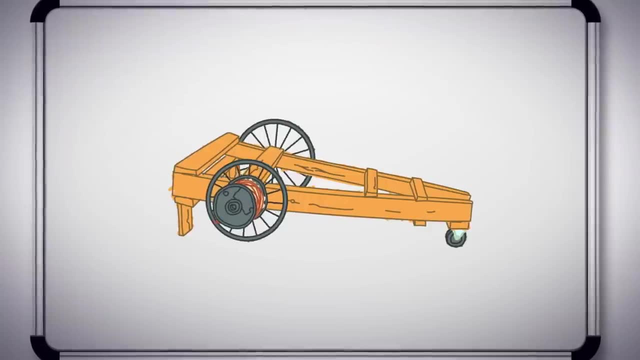 A triangular frame with two large wheels at the back and a small one at the front. What's more, we're going to do the same thing. to get the wheels spinning, We're going to attach a rope and give it a pull When we drag it. 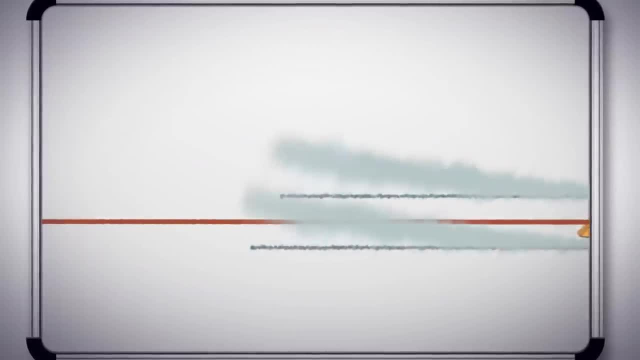 and drop it down. the inertia of the wheels should make the dragster take off. All right, Here we have our dragster. This is nice, Chris. Yeah, it looks good. So the only thing I don't understand is: what are these for? 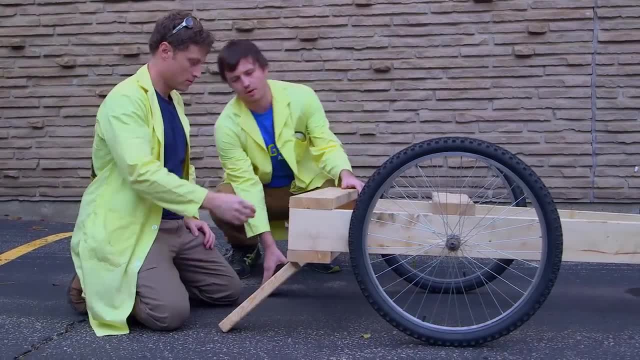 Right. So these are going to help us lift the wheels off the ground like this: Oh okay, Pull it back, And what's going to happen is We're going to run real fast with that string and we're going to give it a little kick. 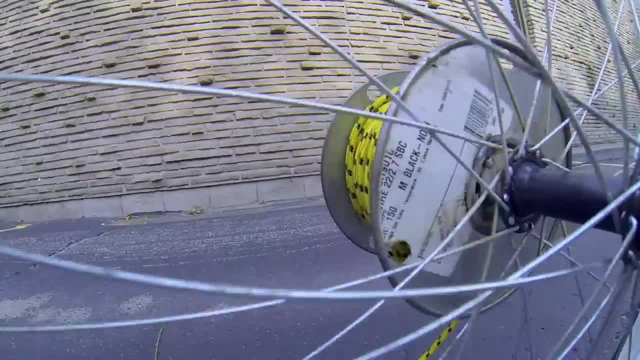 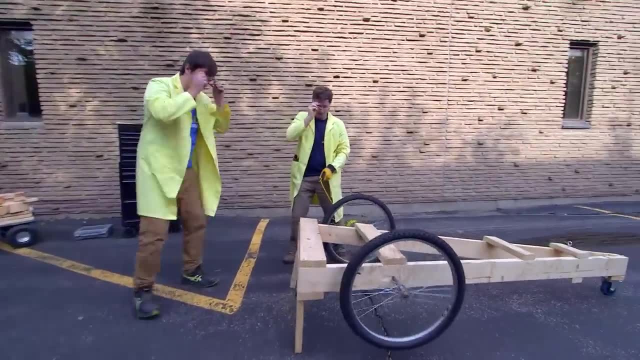 and hopefully it'll take off. Yeah, All right, I like it. So I just run backwards as fast as I can, As fast as you can. All right, Here we go Ready, All right, Okay, Safety glasses on. 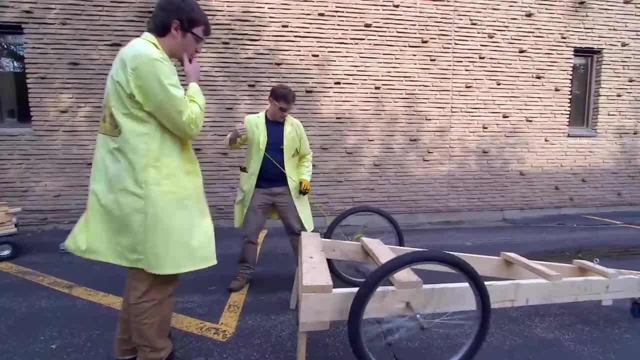 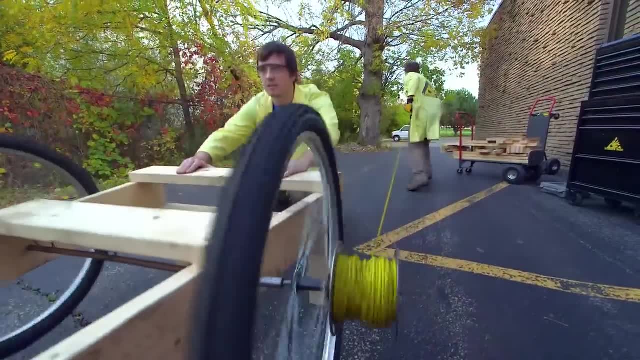 And Oh wait, Did you want to sit on it? or? Oh right, Let's wait until we see it working and then we can. Okay, Dry run. Okay, Dry run. Ready Go Run Phil. 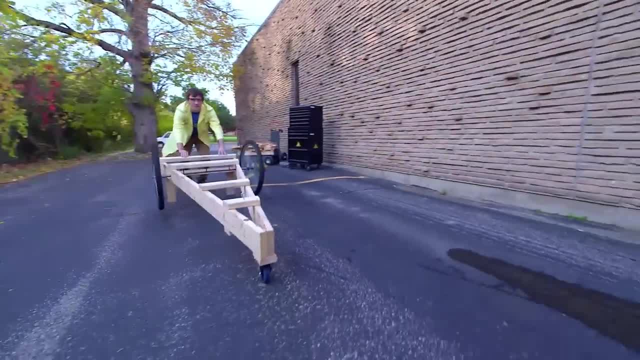 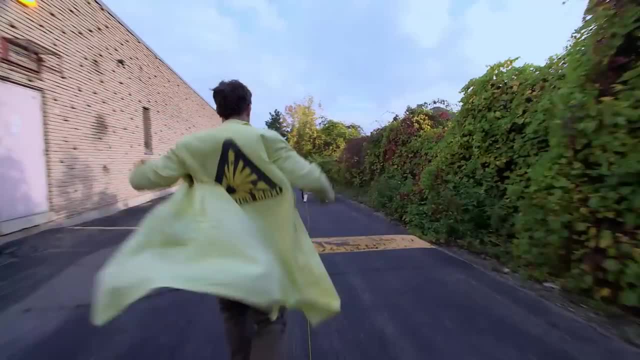 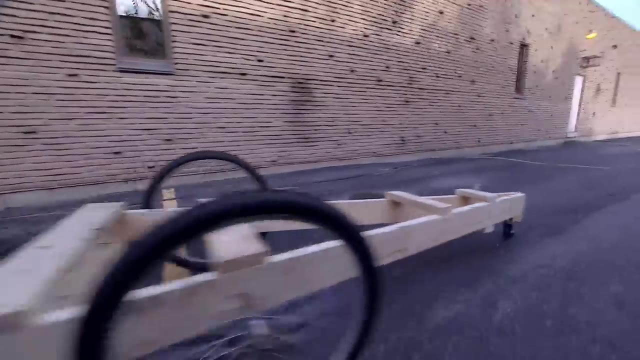 And go Yeah. So here's what happened. Remember the cart has no power when it's on its own. It was able to drive away from a stop using the inertia it got from its spinning wheels and a little bit from Chris' kick. 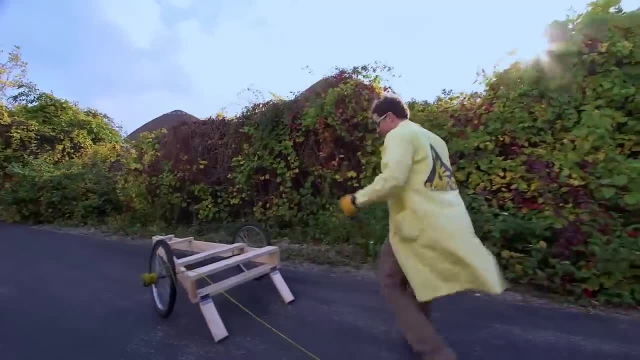 That worked pretty well. That was awesome. Yeah, I think we can make it go even better. You think so. I just think we need a bit more speed. Yeah, All right. Well, let's pull it back to the start. 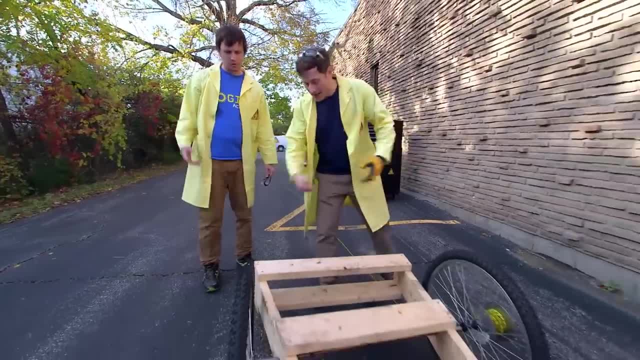 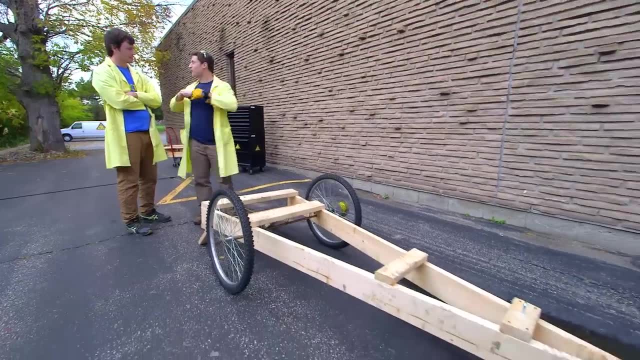 Okay, So what? We just The wheels weren't going fast enough. Yeah, I think so. I think that you running, I mean, was great, but maybe if we use something motorized, Well, I think using a motor feels like cheating. 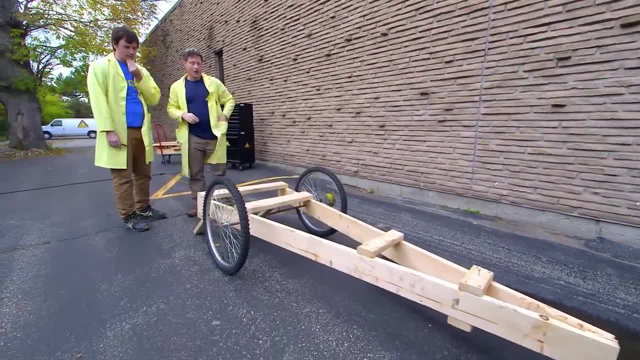 No, no, no, Not on the wheels Maybe. Oh, just to get the wheels spinning fast. Yes, that's right, But what do we? I don't know how that would work. Well, I was thinking a power drill. 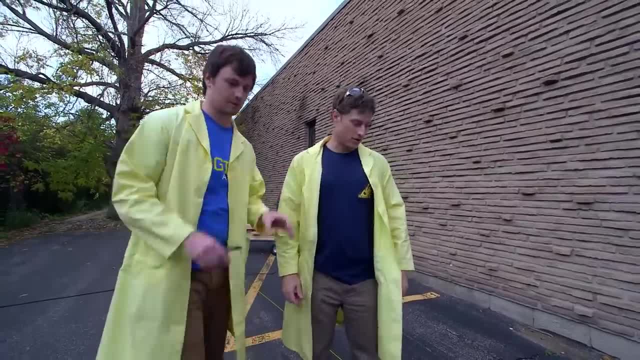 A power drill? Yeah, I don't get it. Okay, How do we use a drill? Let me explain. So we'll take a drill Right and we'll attach it right under this axle here, and that'll get the wheel spinning a lot faster. 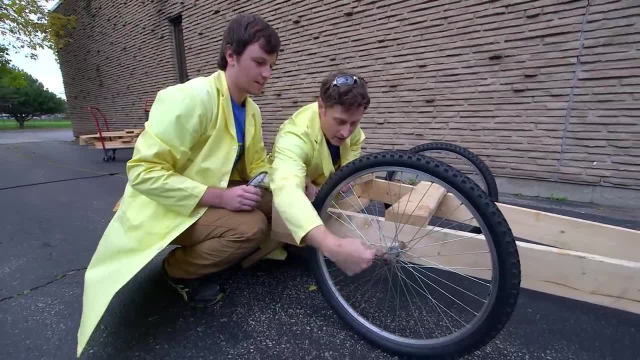 than we had it before. Oh, I see. So you put the drill right here at the end, That's right, and it'll spin the wheel, That's right. Oh, That's the idea anyway. And once we get it up to speed, 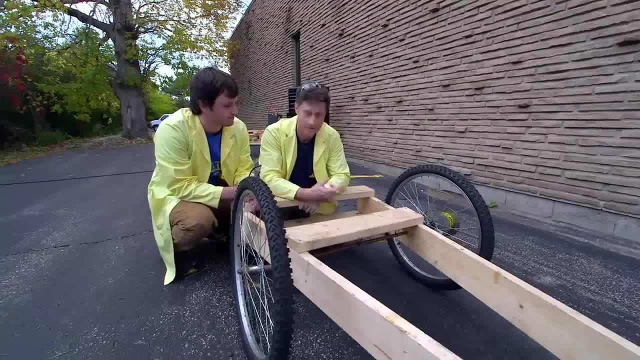 hopefully a lot faster than before. give it a kick, it should go a lot farther. Okay, great, So that's way better than me running all the way back with the rope. I think so. All right, Now here's the real question. 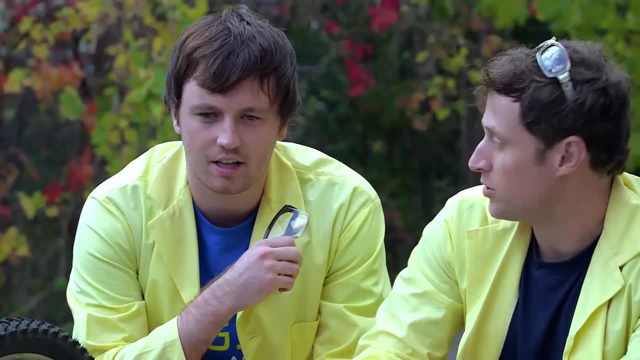 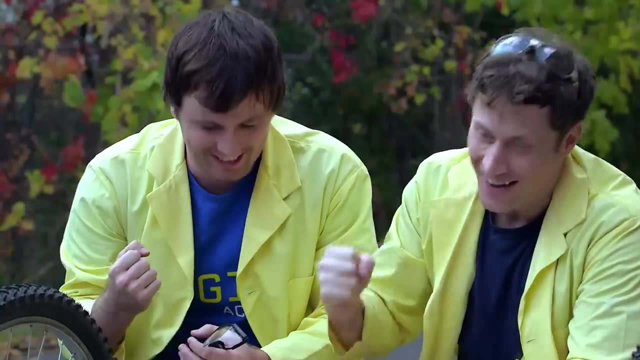 Should we just go for it and have someone ride it when we do it with the drill? Well, who gets to ride it? Oh, rock paper scissors. Okay, Let's go One, two, three, Oh Yes. 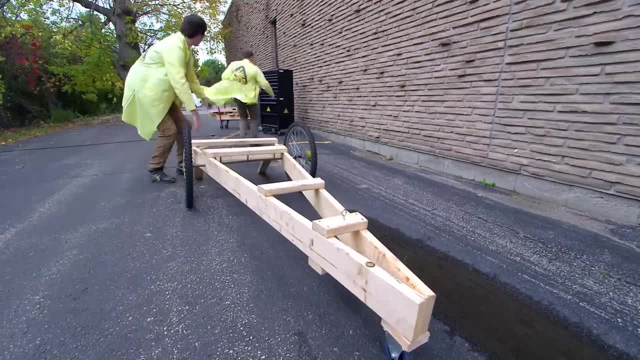 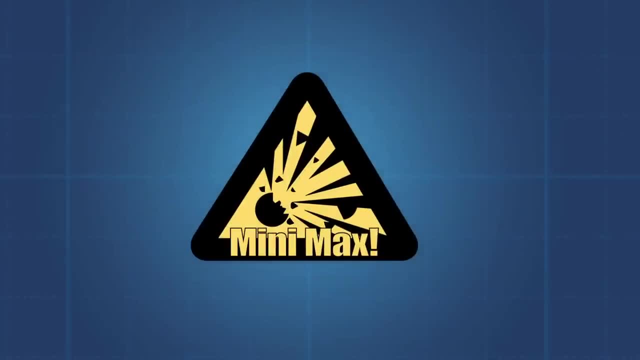 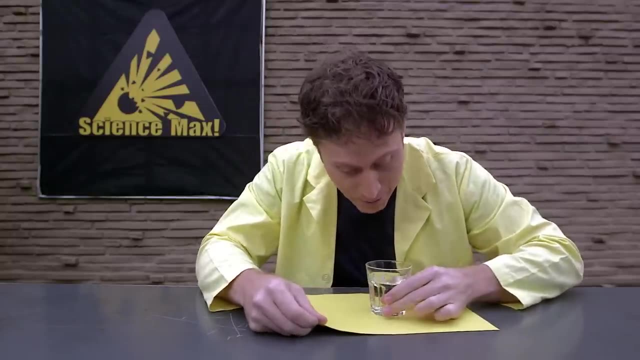 All right, I will get a drill. Okay, What kind of bit do we need? A hex bit. Here's a fun experiment you can try If you have something heavy, like this glass of water and you put it on a piece of paper. 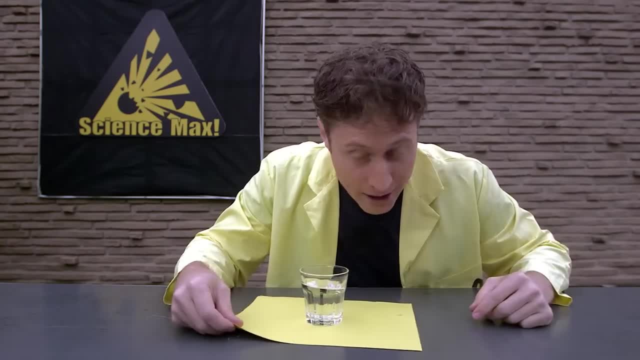 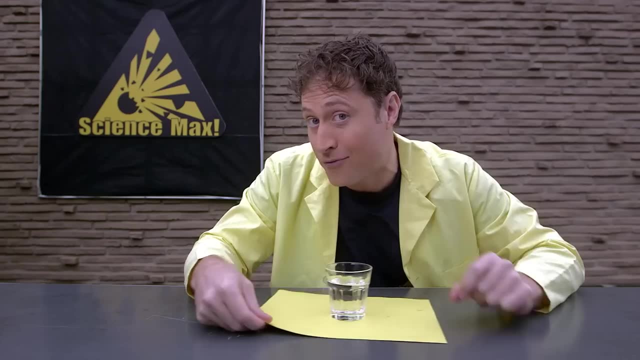 you can experiment with inertia. If you move the paper slowly, the glass moves with the paper because the friction between the paper and the glass is enough to overcome the inertia of the glass. But if you move the paper quickly, the friction is not enough to overcome the inertia. 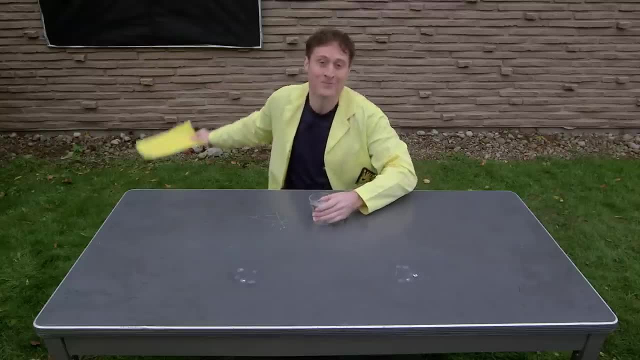 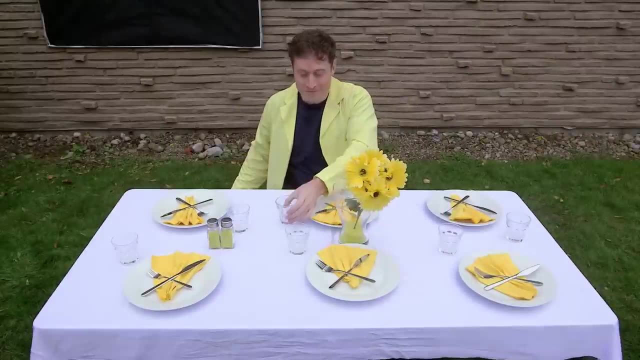 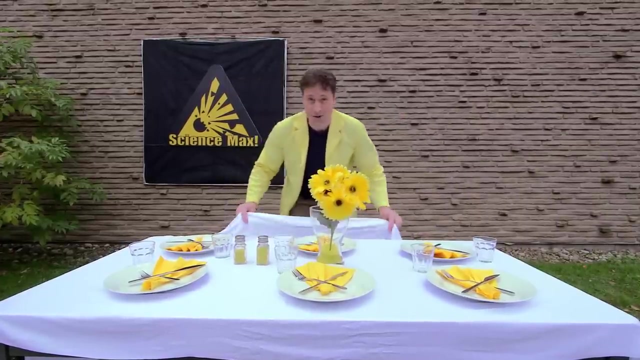 and the glass stays put. And now let's max it out. Okay, Let's do it All right. Now you might be tempted to try this at home, and you can, but please for me, promise that you'll let an adult know. 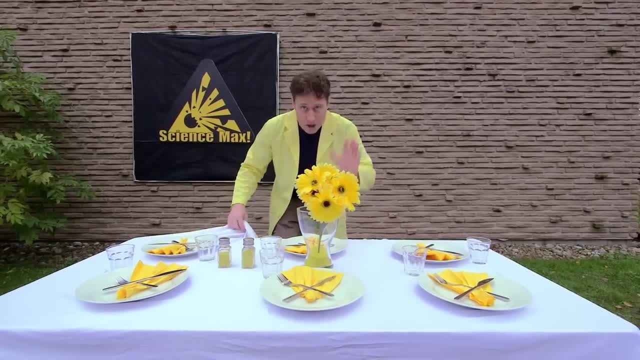 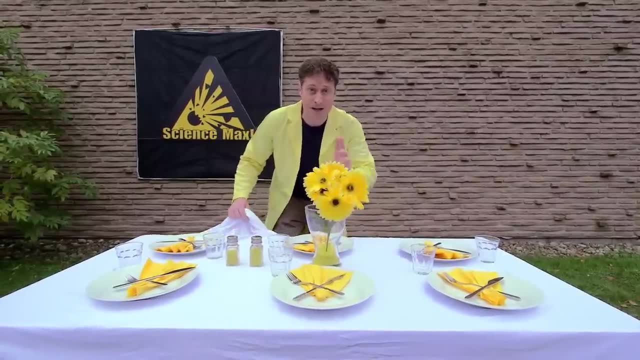 you're about to do this, And don't use breakable plates. Use plastic plates, because this will take a couple times of practicing before you get it right. Put something on the plastic plates, because the heavier they are, the better it will work. 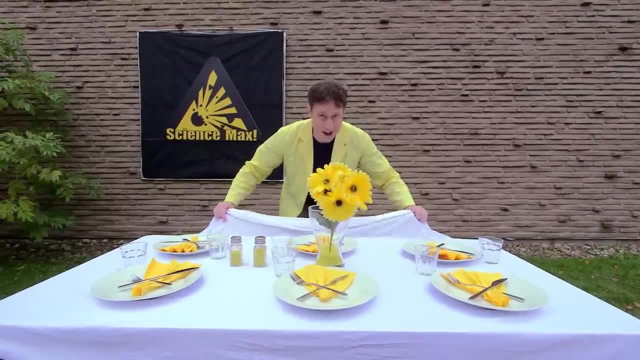 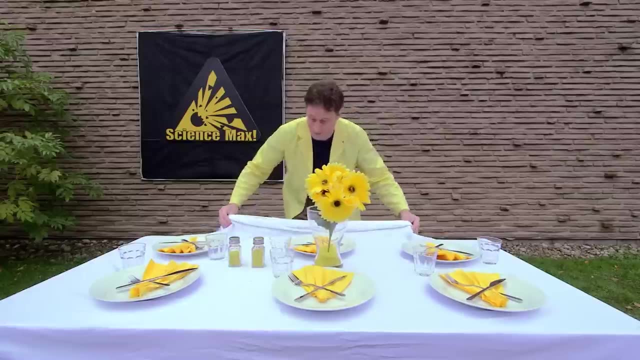 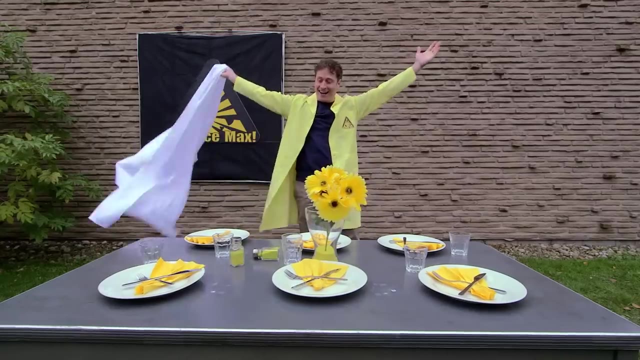 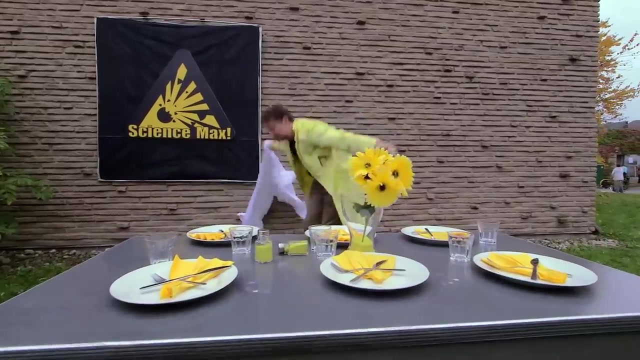 All right, Did I mention not to do this at home unless an adult knows you're doing it? I cannot stress that enough. Okay deal, All right, deal, Here we go, And there you go, Newton's first law, Thank you. 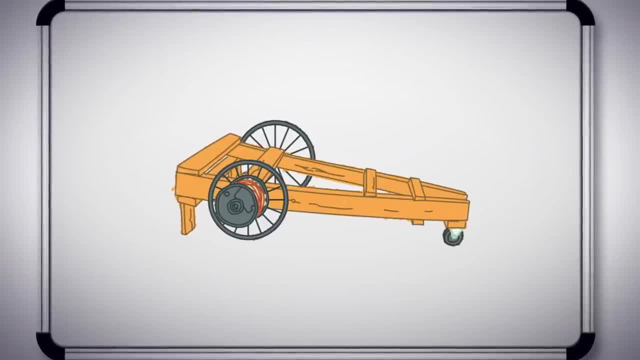 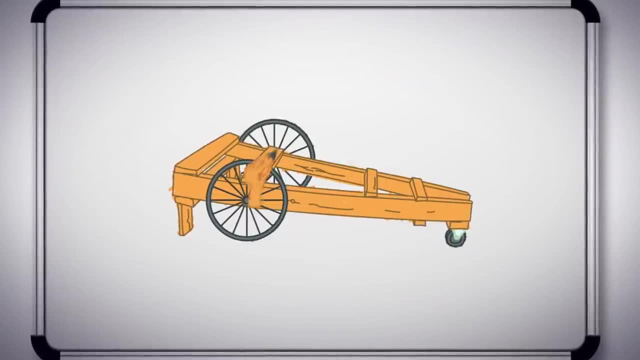 Our dragster worked pretty well, but now we're going to try sitting on it and seeing if the inertia of the wheels is enough to accelerate the dragster and the human rider, Because we're going to need a lot more inertia. we're going to make the wheels spin even faster. 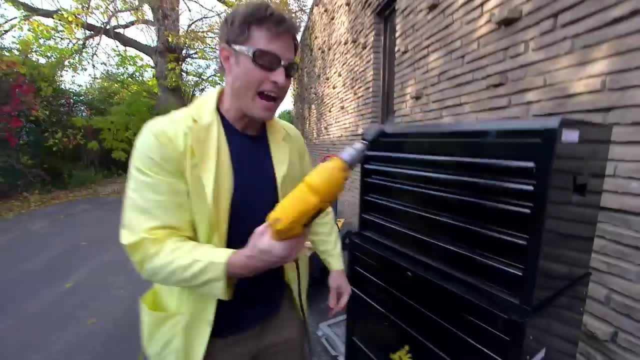 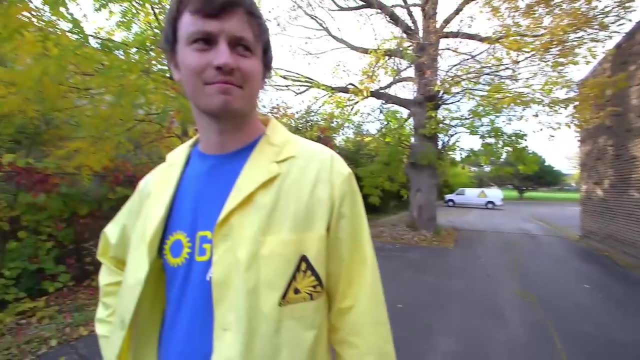 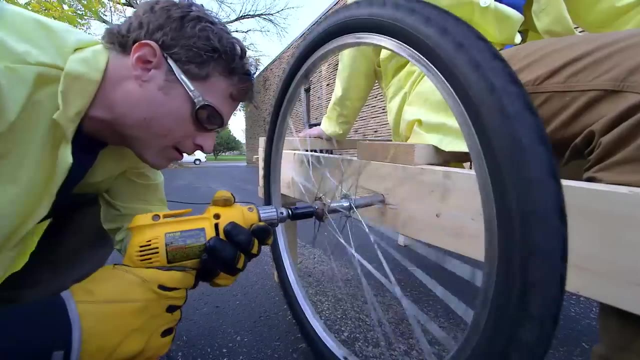 using a drill. All right, Power tools, Yeah, Power tools, Whoo-hoo-hoo-hoo-hoo, Yeah, Ha-ha-ha, Ha-ha-ha. Sorry, When I attach the drill to the wheel. 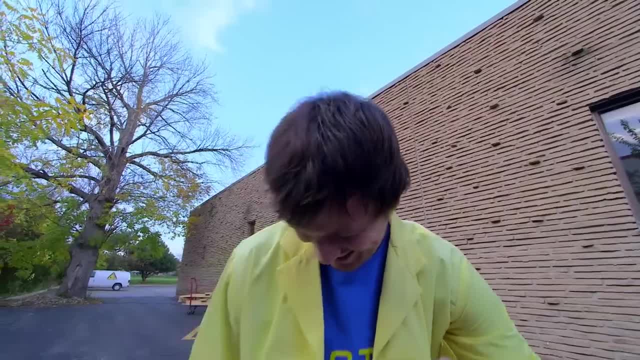 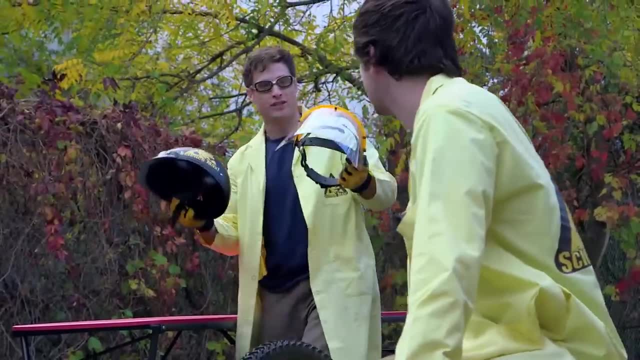 it works really well. Yep, That is really going to work. All right, Let's do it for real. So, uh, what do you want? Helmet or blast shield? Blast shield, Blast shield. All right, there you go. 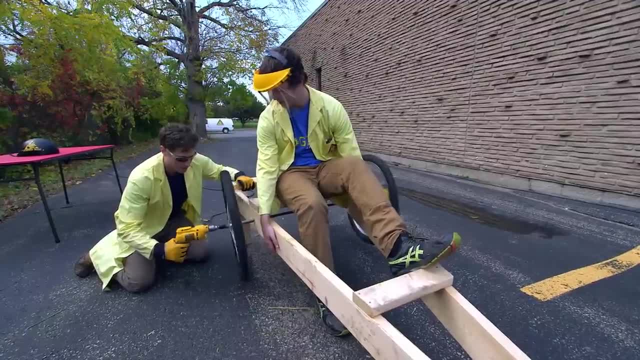 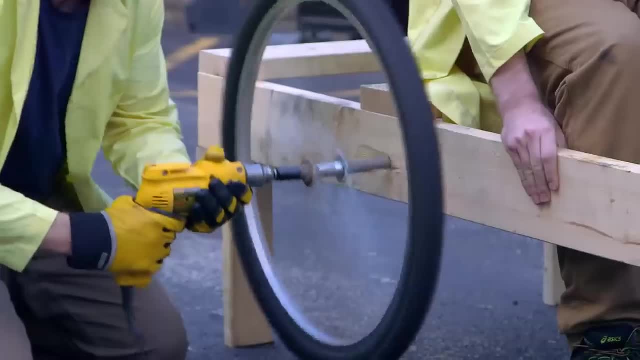 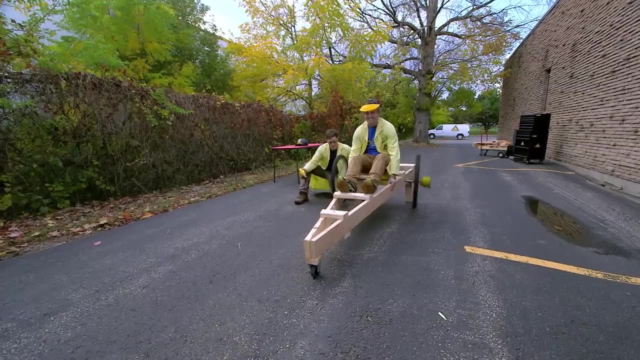 You ready? Go There, you go, Okay, Okay, Okay. Remember: the faster the wheels are spinning, the more inertia they will have. Ready, Ready And Ugh, Ha-ha-ha-ha-ha-ha-ha. 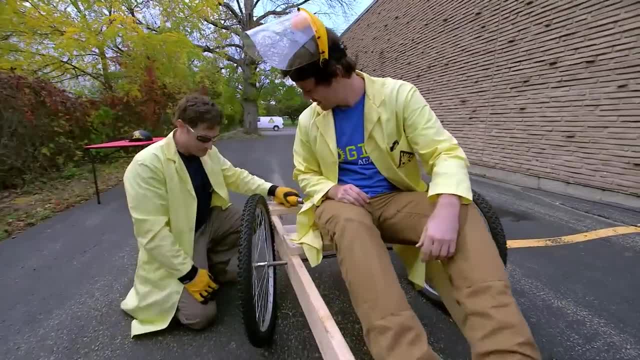 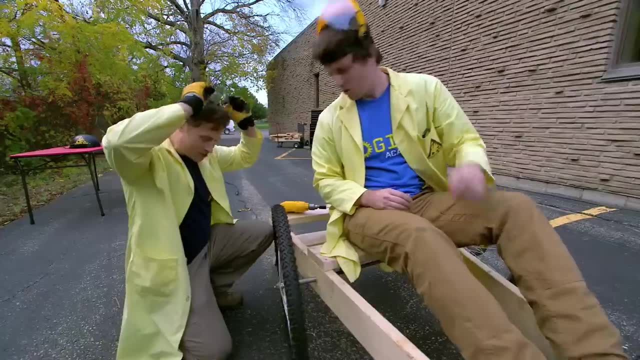 Well, What happened? Uh, So you went. you went a foot, One foot. So why didn't that work? uh, nearly as well as the last time we did it. Well, I think my extra weight caused a bit of a problem. 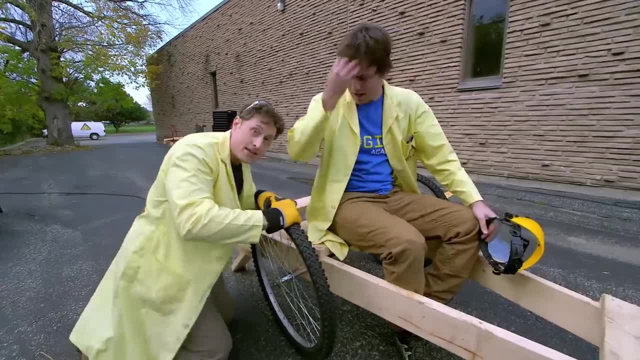 Yeah, So the inertia wasn't able to carry us forward, But the whole, the whole point of this is so that someone can ride the dragster, because why build it if we can't ride it? That's exactly right, I think, if we're going to have someone ride it. 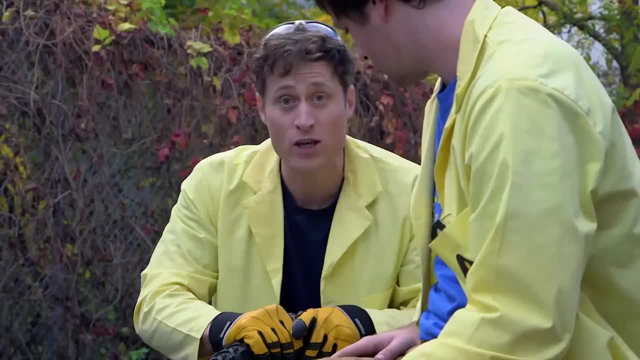 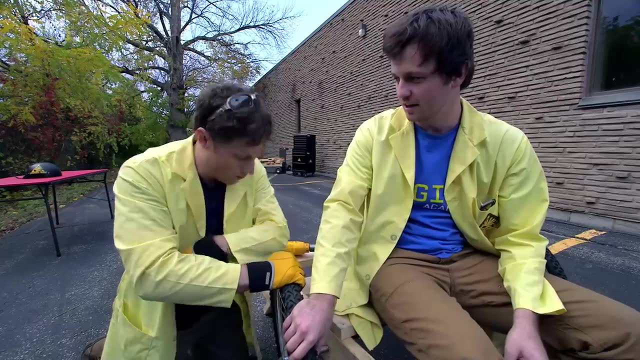 we need heavier wheels. Well, on the small one, we used plasticine. Yeah, I don't know if that's what we should use. What if we used Car tires? Car tires- What on this? No, I think we're going to have to build something bigger. 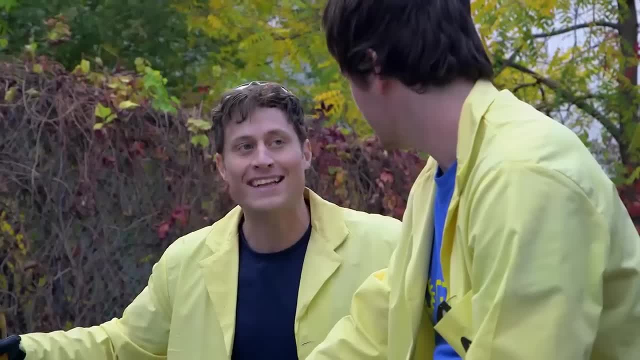 So we, Okay, so we build a whole new frame. Yep, What if we got like the axle of, like the back axle of a car or something That's a great idea, The back axle of a car. and then what we use, the drill. 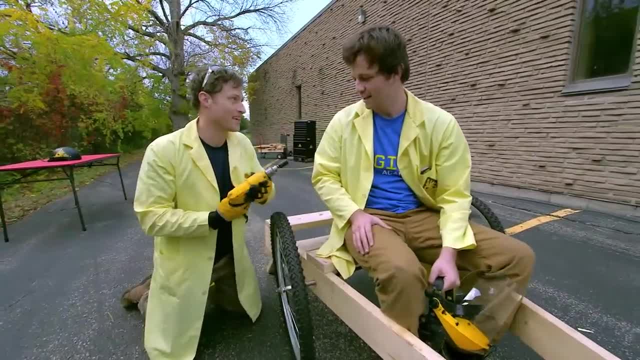 I don't think the drill's going to be enough To move the Why? You don't think it's going to be enough to move the back axle of a car. Yeah, it's too, yeah, too big. So what do we do? 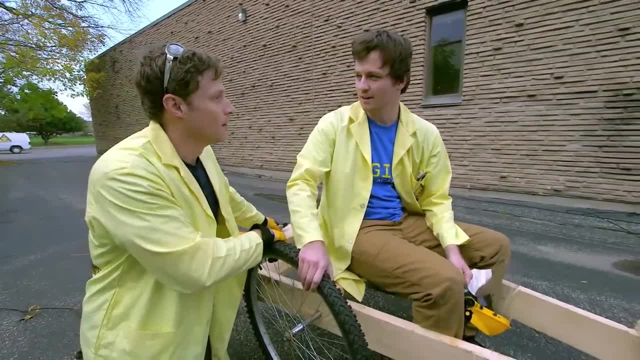 Well, what's good at moving the back axle of a car? Well, I mean a car, but we would have to take it off the car, so We could use another car. We could use another, We could use, we could use another car. 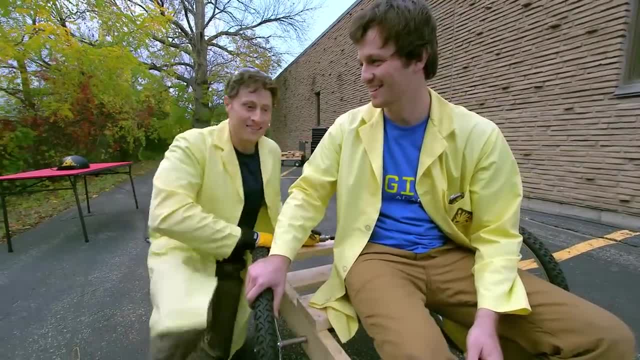 We could use another car. Um, you'll have to explain how that works. Okay, Let's go. let's go get the stuff and you can tell me how we're going to use. So how do we use another car to make the first car go? 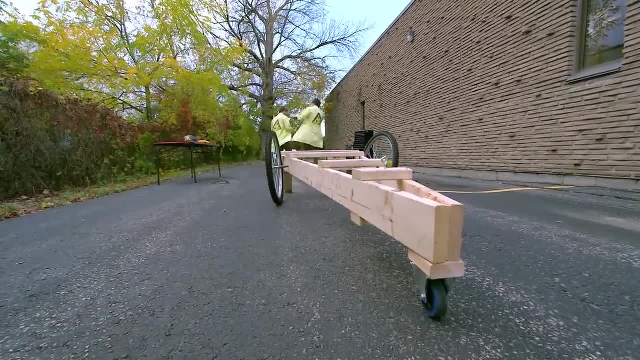 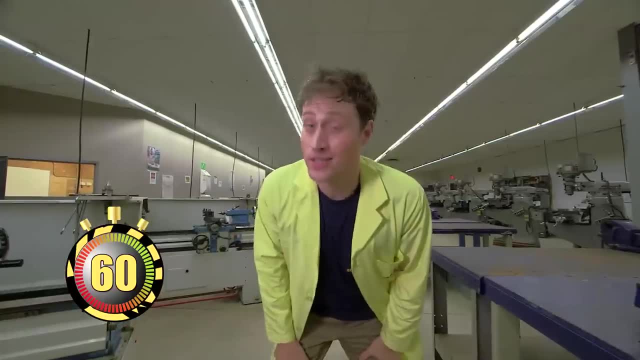 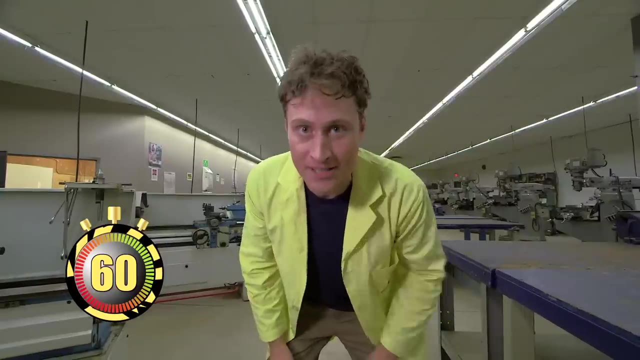 Okay, I'm thinking we jack one car up. Yeah, Back our big dragster Newton's Laws in 60 Seconds. Isaac Newton was a super genius, and among the many things he did was come up with three laws of motion that describe how everything moves or doesn't move. 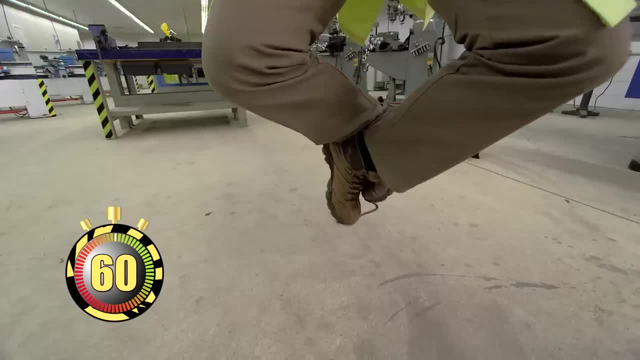 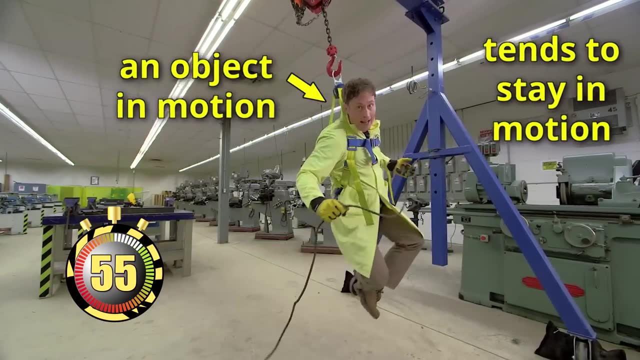 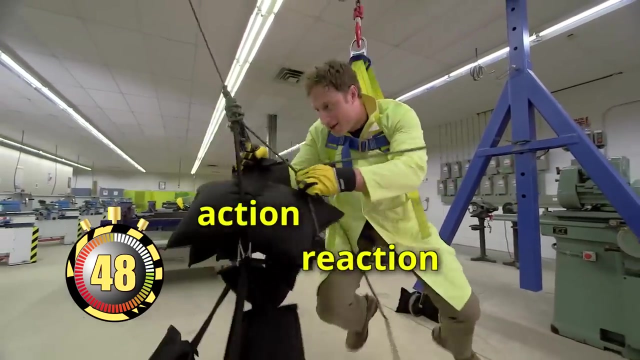 I will demonstrate using myself Newton's first law: an object at rest tends to stay at rest. An object in motion tends to stay in motion. Newton's third law is: for every action there is an equal and opposite reaction. These sandbags weigh as much as I do. 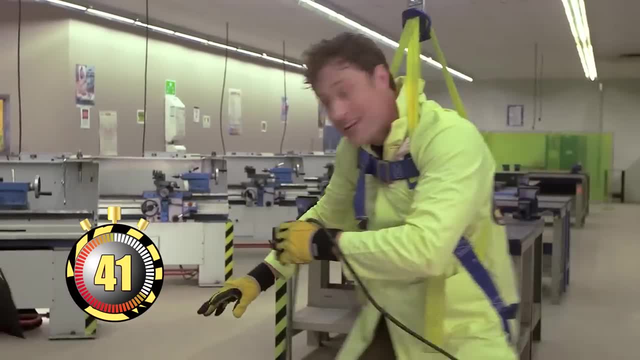 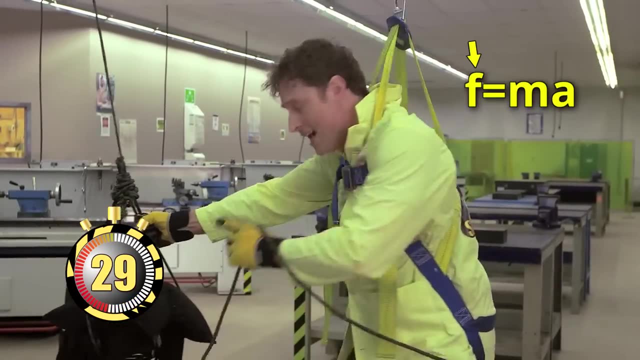 so when I push them forward, I go backward the same distance. Now Newton's second law is: F equals m. a Force equals mass times. acceleration: How hard you push something is equal to its mass or its weight times its acceleration, or how much you change its speed. 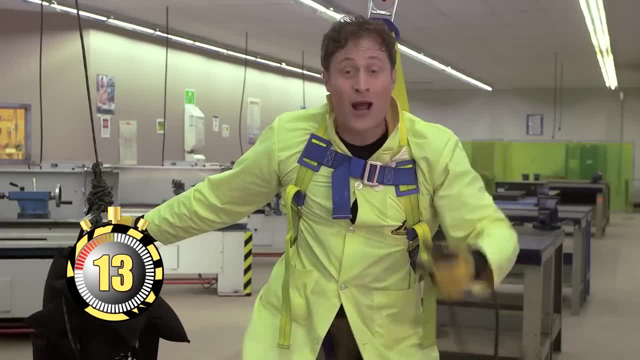 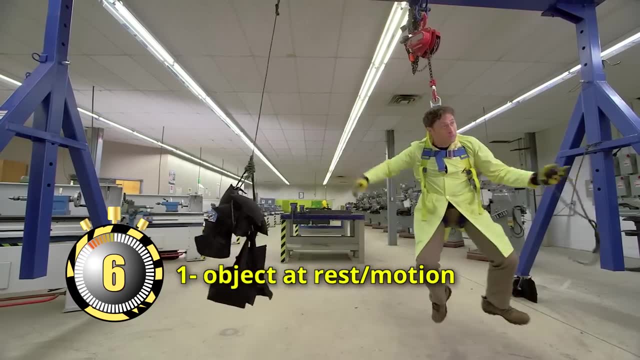 I know It's a little bit more complicated, so we're going to have a whole other segment describing that one coming up Meantime. let's recap Newton's first law: object at rest tends to stay at rest. Object in motion tends to stay in motion. 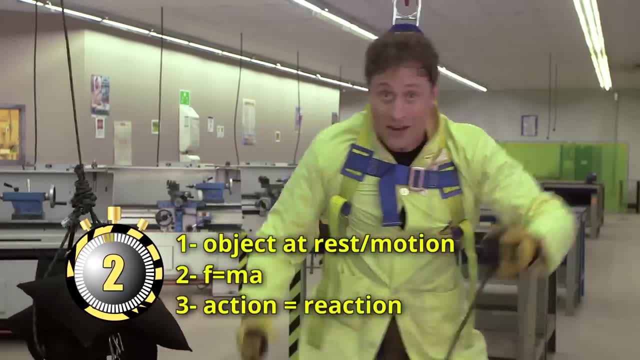 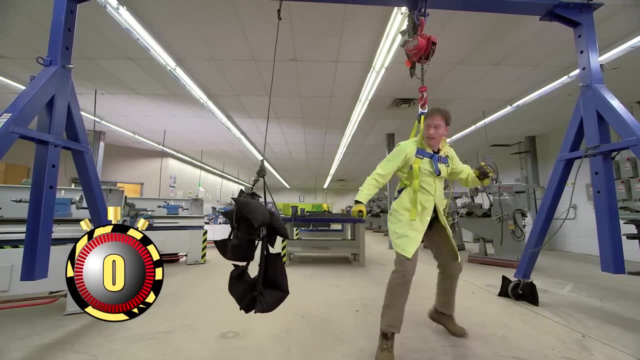 Newton's third law: for every action there is an equal and opposite reaction. Newton's second: F, m, a. Newton's three laws of motion. Now, how do I, how do I get down? How do I, how do I get? 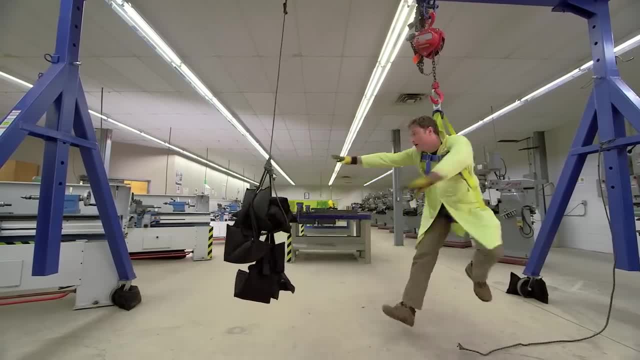 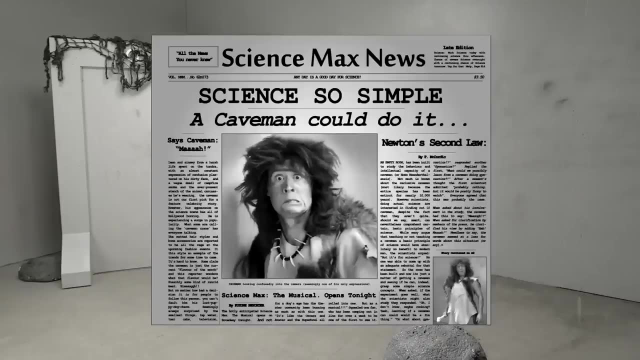 oh wait, I know, I know. Oh no, that wasn't. that was not a good idea. That was. Now it's time for science. so simple a caveman could do it. This is a caveman. This is a door. 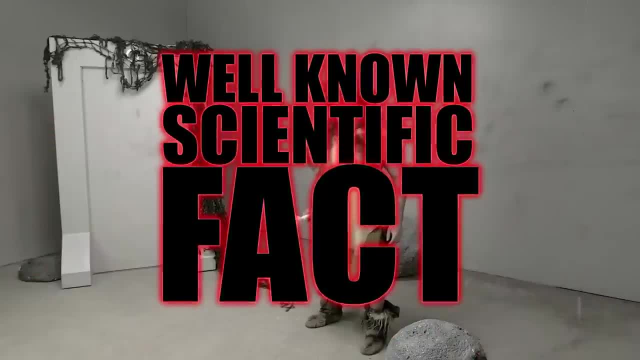 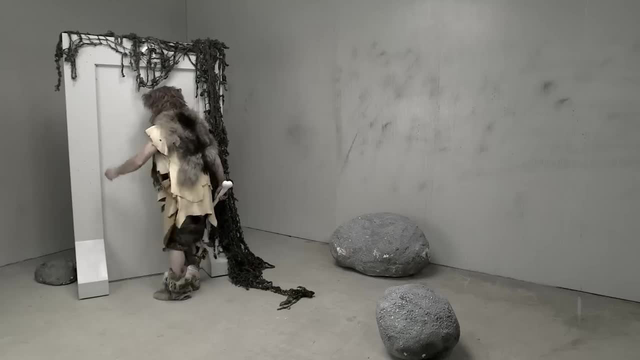 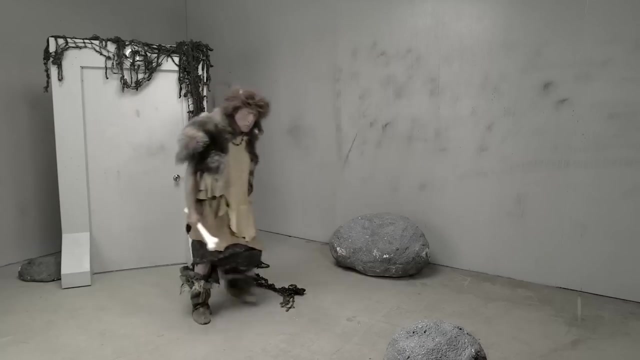 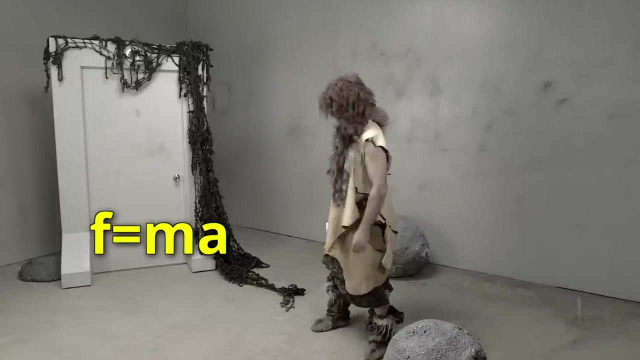 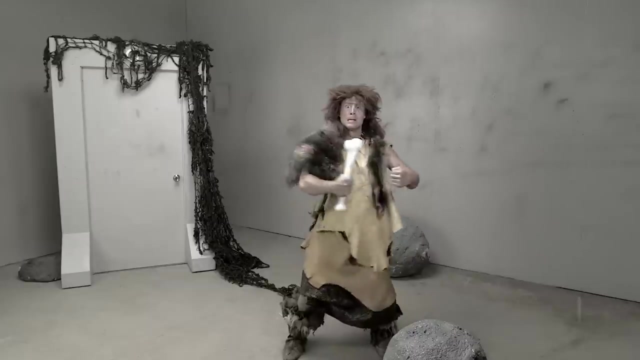 It is a well-known scientific fact that cavemen do not know how to open doors. This is Newton's second law: Force equals mass Equals mass times acceleration. Our caveman thinks he can open the door if he uses force. Well, what if he was to walk briskly into the door? 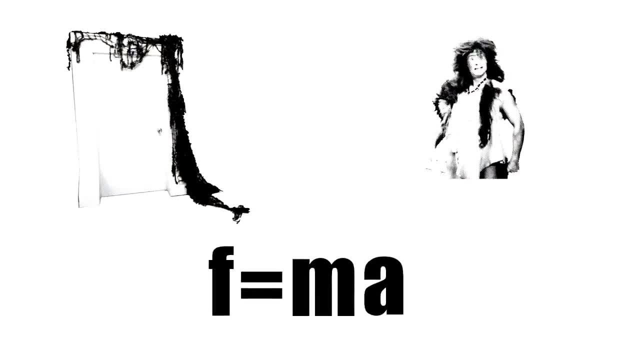 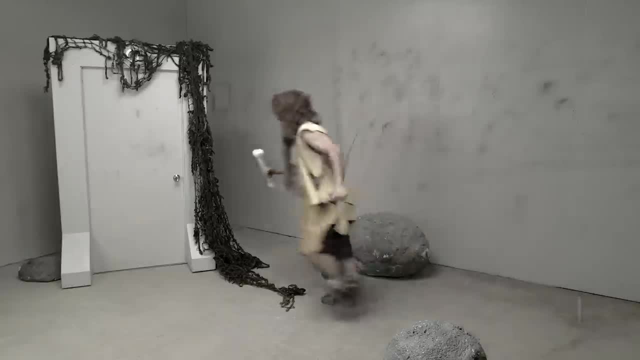 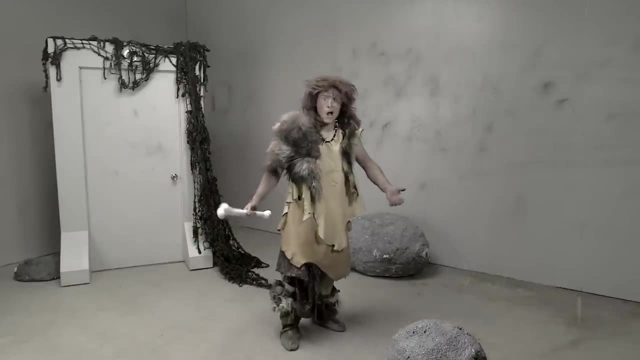 Then the force that he will hit the door with will be equal to his mass, or how much he weighs, times his acceleration, which will be walking speed to zero. It didn't work, did it? Looks like we need more force. 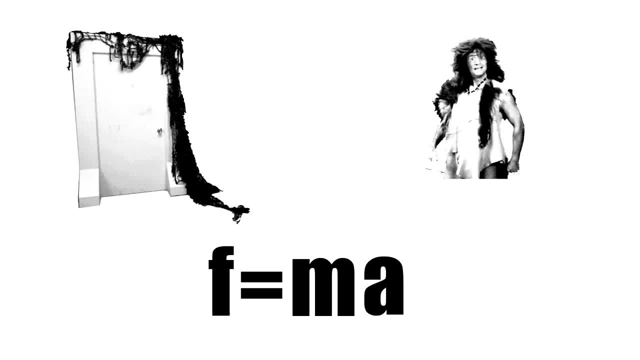 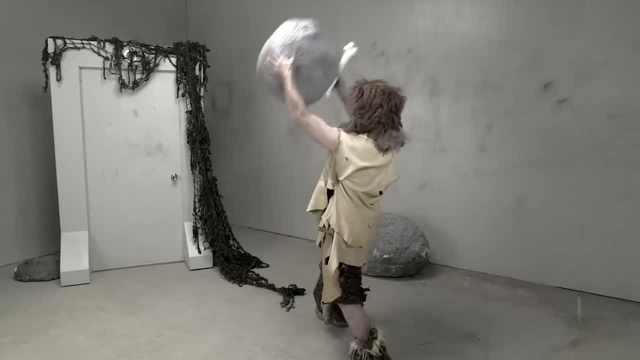 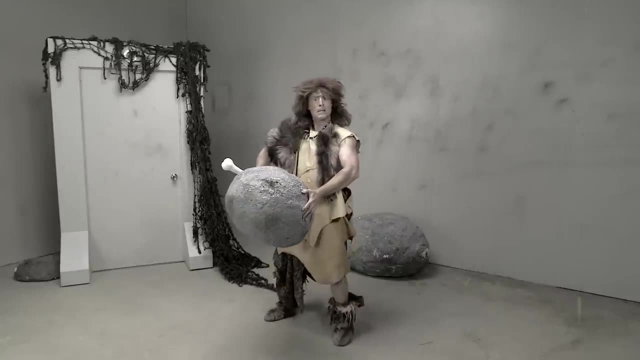 If we want to increase the force, we need to increase the mass, increase the acceleration, or both. A rock, That's perfect. If the caveman holds the rock, he has a greater mass. Now we just need to increase the acceleration. 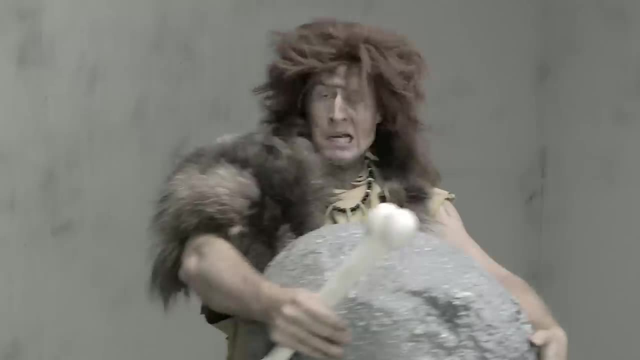 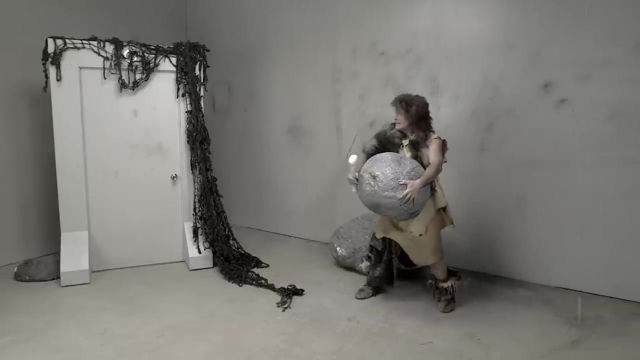 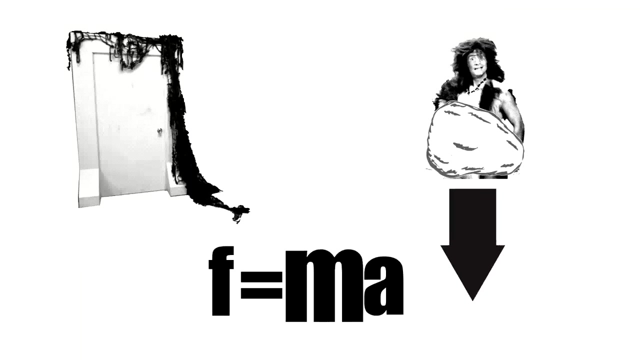 which means going faster. Let's try running. Go on A little further. That's good. Now the caveman is going to run at the door To get more force. we've increased the mass to a caveman plus a rock. 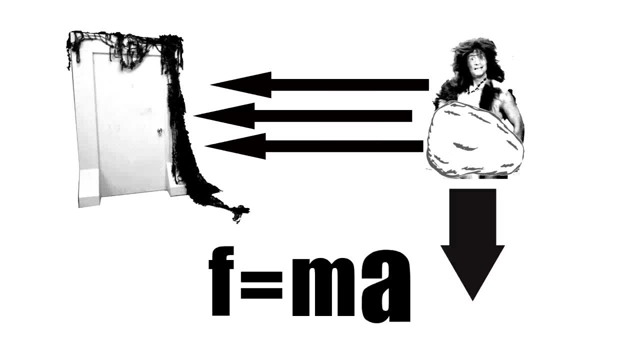 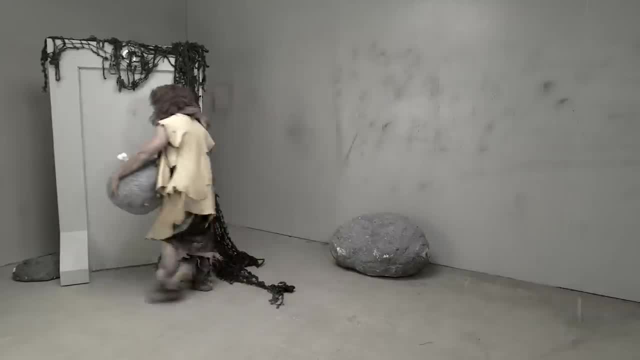 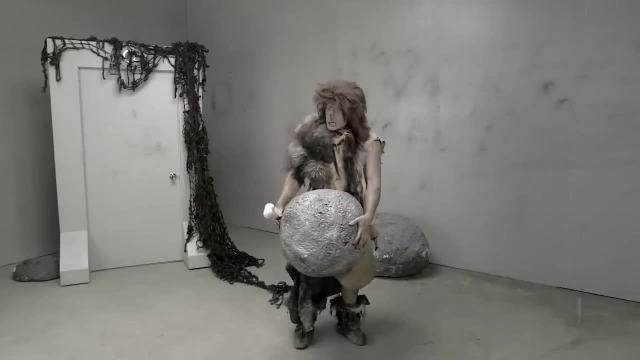 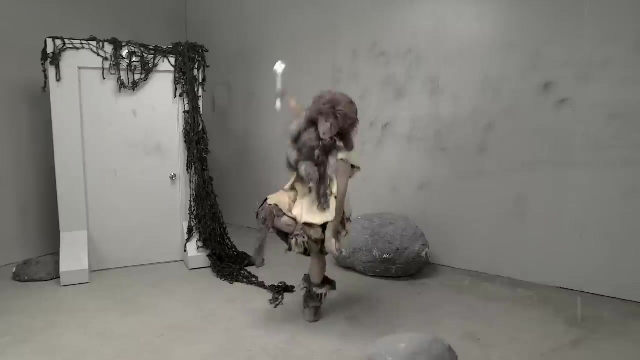 And we've increased the acceleration to go from running speed to zero. And there you have it. That's how Newton's second law works. Join us next time for how doorknobs work. What Our inertia-powered dragster just wasn't maxed out enough. 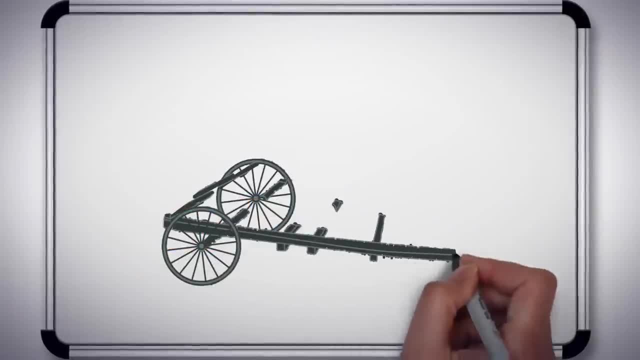 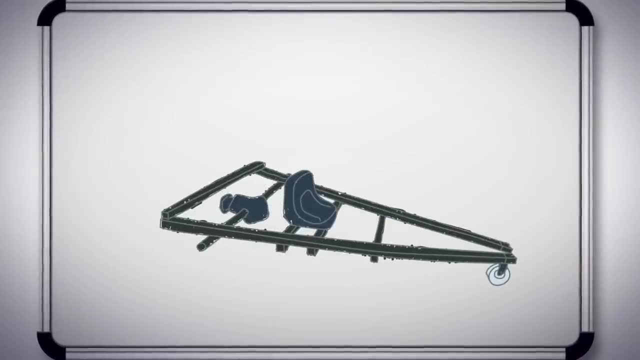 So Chris and I built a second dragster, the Dragster Mark II. This one is a welded metal frame and instead of bike tires we're using car tires, because they're much heavier than bike tires And to get the tires spinning fast enough. 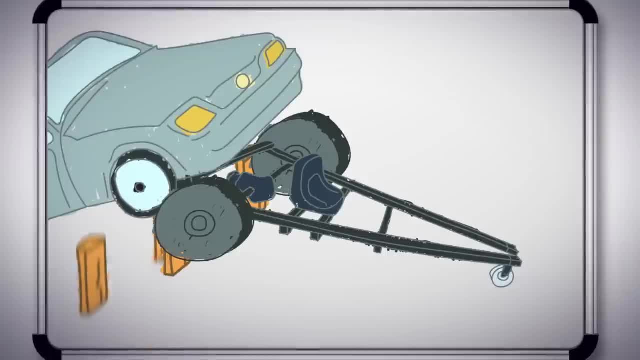 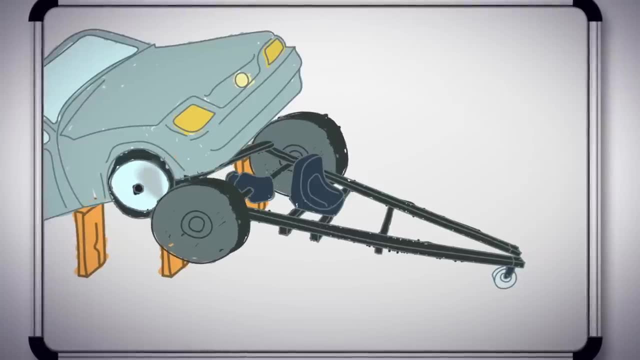 we're going to use a car, That's right. We jack up an actual car and have the tires touch each other. Then we can get those heavy tires spinning fast enough to get enough inertia to get me going from nothing. The Science Max build team. 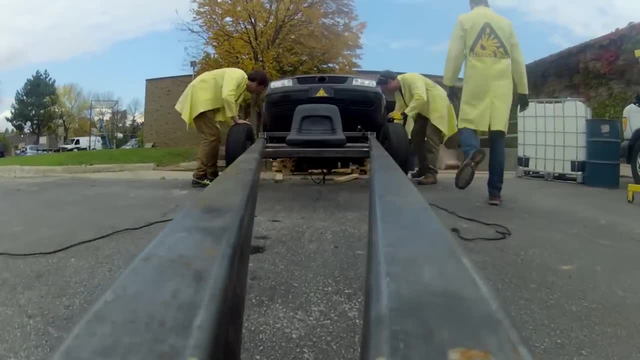 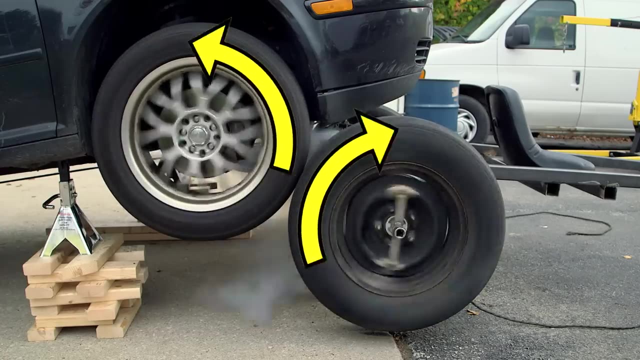 pulled out all the stops on this one. Just like the smaller version, the dragster has to be up on jacks so the wheels don't touch the ground as they get spun up. The wheels of the dragster touch the wheels of this working car. 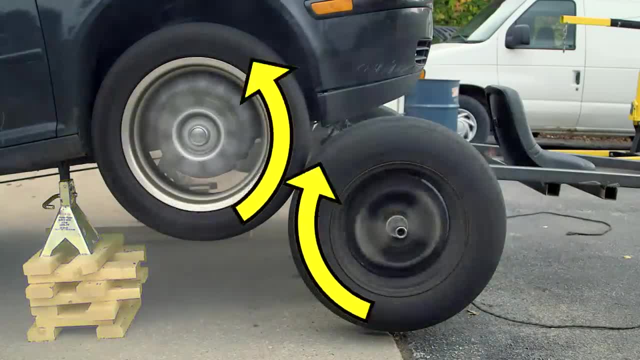 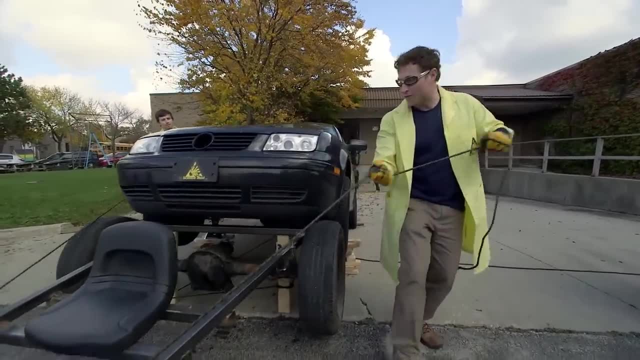 which is also jacked up. That's how we're going to get them spinning fast enough. Chris is over there. He's got a rope, just like I'm going to have a rope, And when we're ready, we're going to run forward. 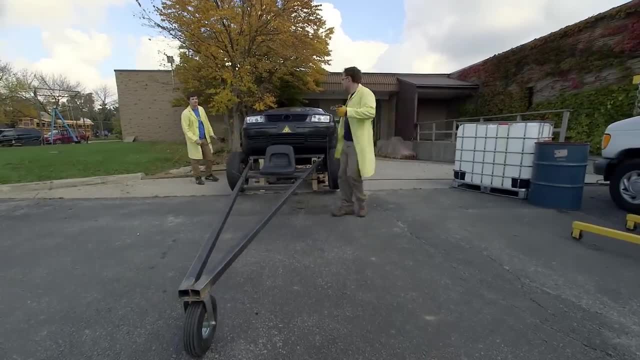 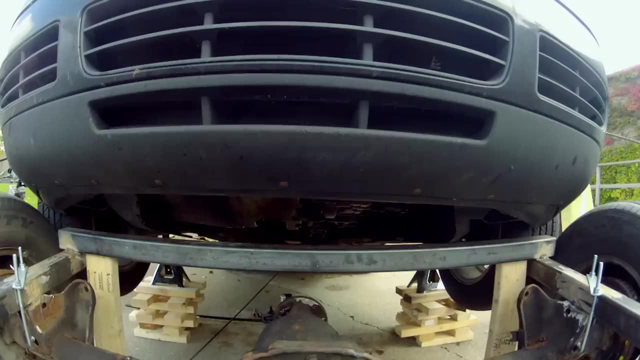 and pull it off, the jacks and our dragster will go. We hope right, That's the plan, right. I think it's going to work. I think we should do it. Ready, You ready, Paul Ready. 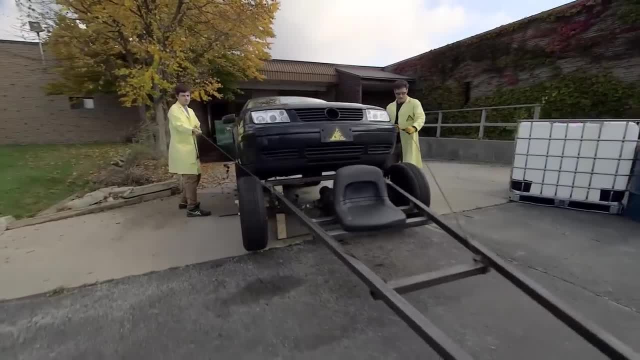 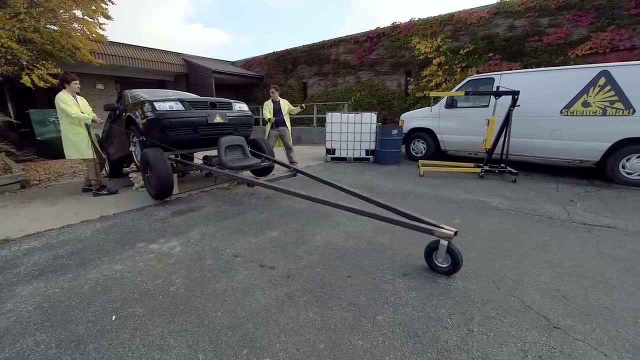 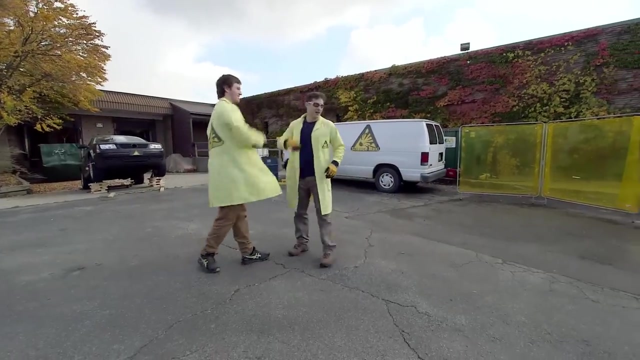 Fire it up, Go, go, go, Faster, faster, faster, Faster, faster. Keep going After three right: One, two, three go. Nice, Pretty good. Yeah, that worked All right, I think. 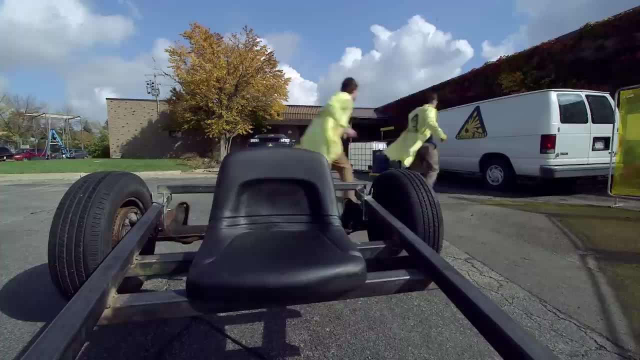 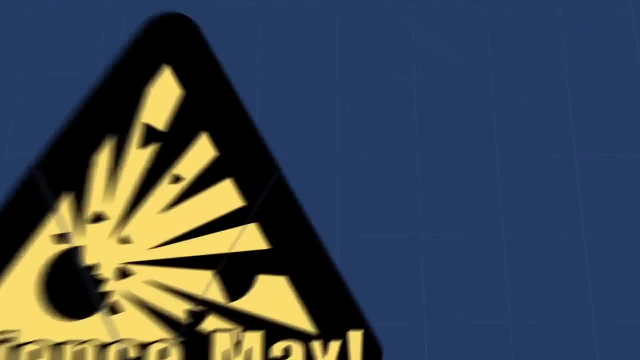 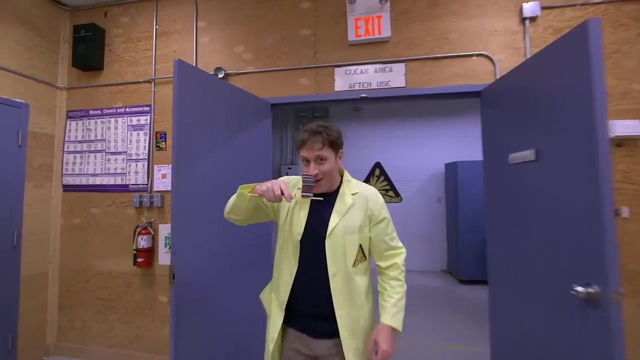 are we ready for me to be in it? I think so. All right, We're going to do it. The helmet's in the Max van. Do you have the keys for the Max van? Uh, keys for the Max van. Here's another small experiment. 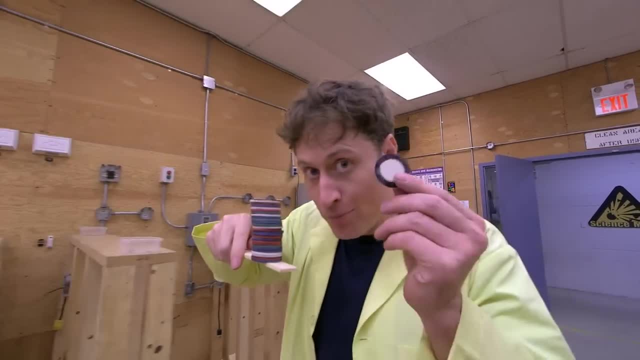 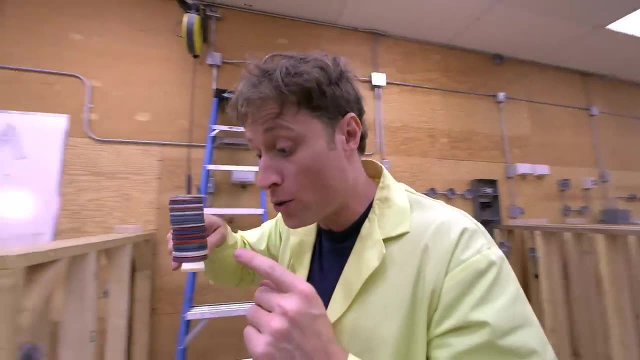 you can do with inertia. Take a stack of checkers or game pieces like I have here, Oh, or coins- Coins work really well- And a ruler or something else that's flat. This is the kind of stick they give you at the hardware store. 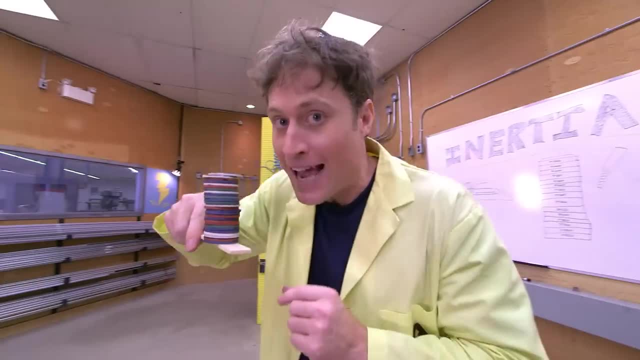 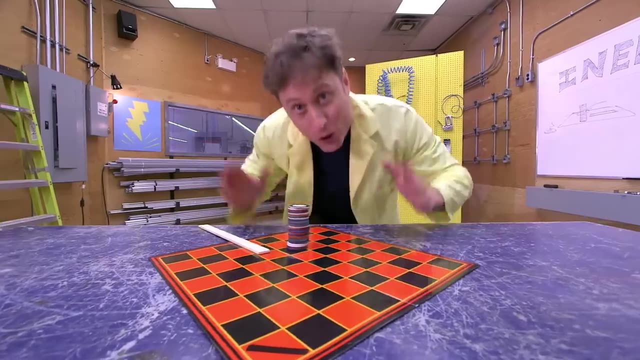 to stir your paint with. Now you can knock checkers out of the middle of the stack without the stack falling over. if you're very careful, You see, the friction of the checkers leaving the middle of the stack won't be enough to overcome the inertia. 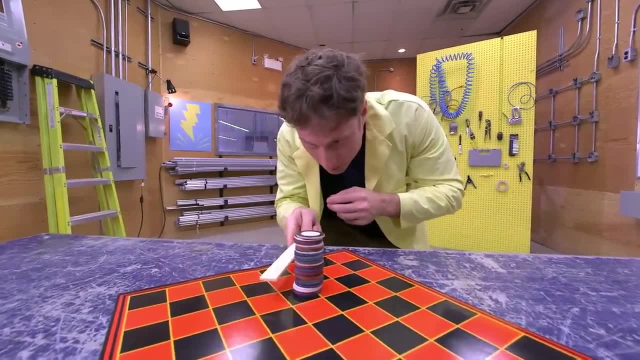 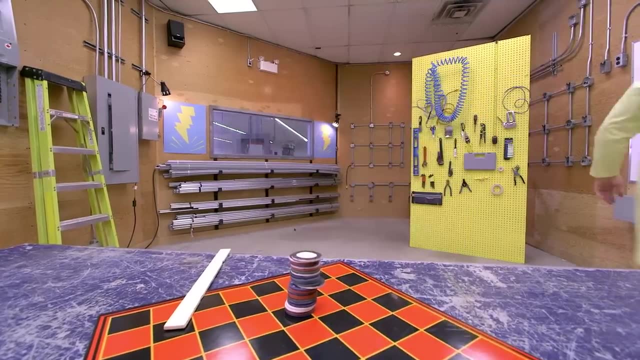 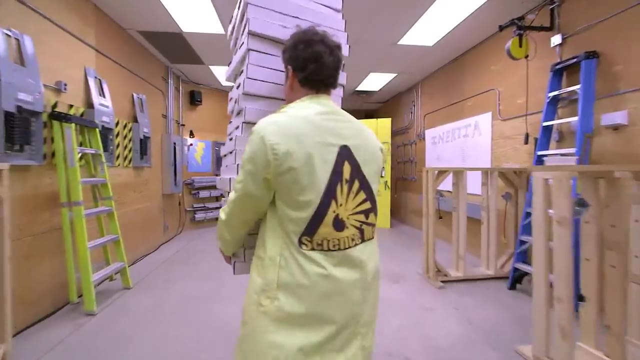 of the rest of the checkers Ready. Now let's max it out. Oh, I have these pizza boxes and they should work the same way. You see, you get a stack and don't worry, I've already eaten all the pizza. 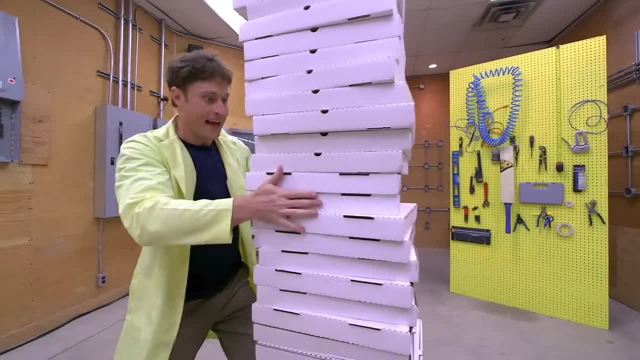 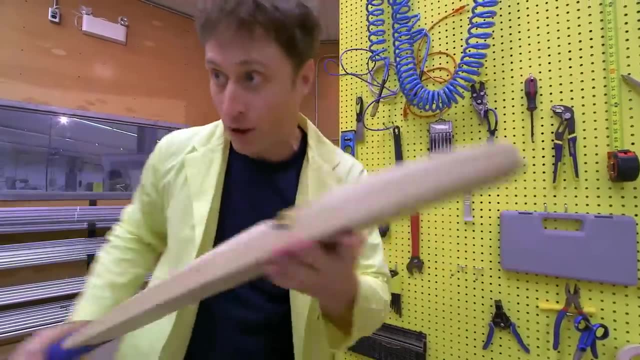 And I put them on there like that. And now I need a ruler, And what I've got is this cricket bat. You see, it's got a nice flat edge, just like the ruler. Now, if this works right, I can hit it hard enough. 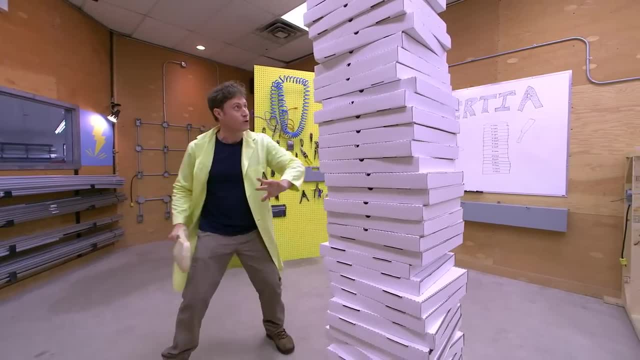 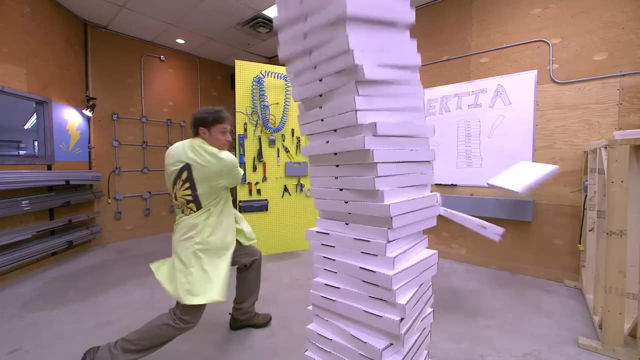 to knock out just one or two pizza boxes, and the rest of the stack should stay Here. we go Ready. Ha ha, ha, ha ha. Science Awesome, Ha ha. And there you have it, Newton's first law. 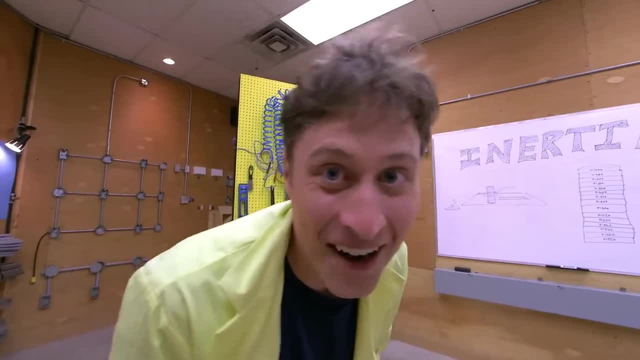 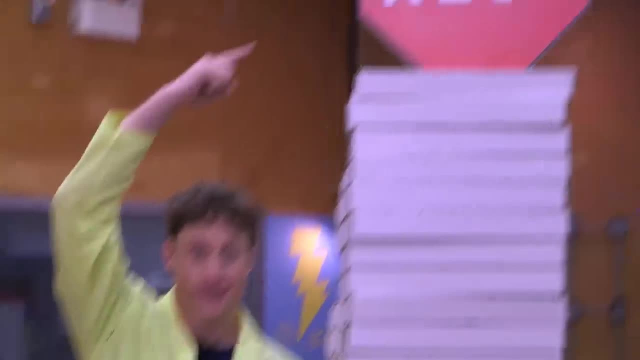 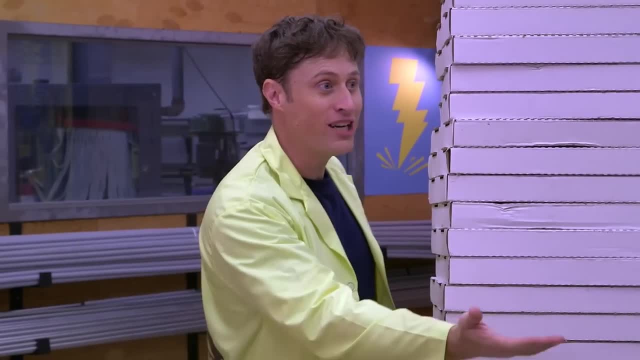 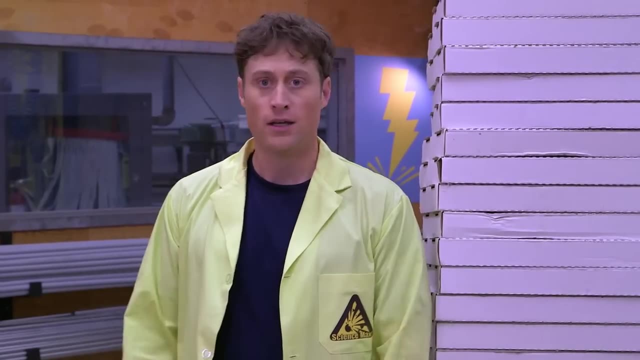 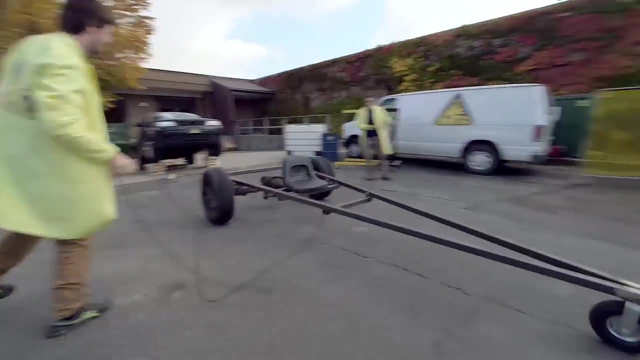 and an object in motion tends to stay in motion. An object in motion tends to stay in motion. Usually there's a sign that kind of: Well, our inertia-powered dragster worked really well, And now it's time for the final step. 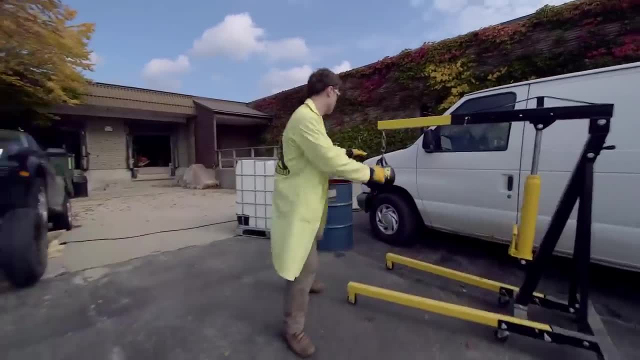 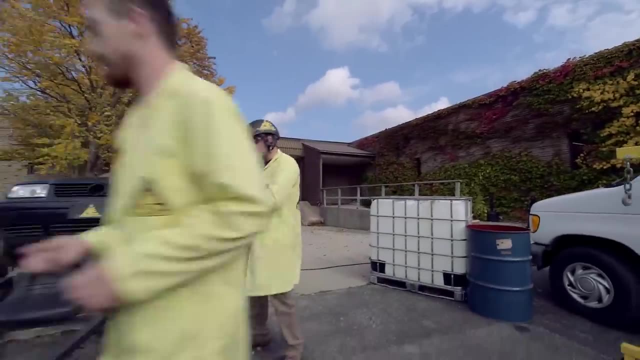 me riding it to glory Now. I know that probably doesn't need saying: but don't try this at home. Not that I think you really can try this at home, because this is kind of involved, but I figured I should probably tell you guys. 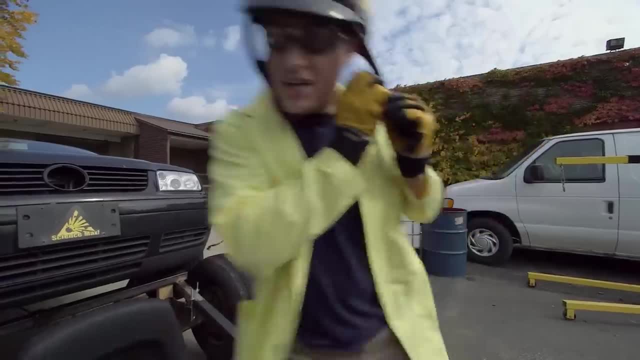 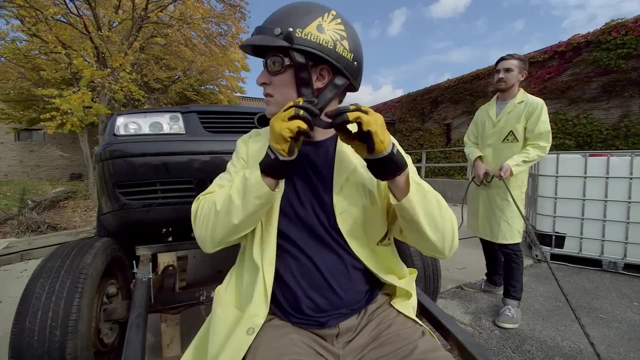 just in case you were tempted to try it at home. We know what we're doing. We know what we're doing, right, Chris? Yes, Yes, Yes, we know what we're doing. All right, Fire it up, Keep it going. 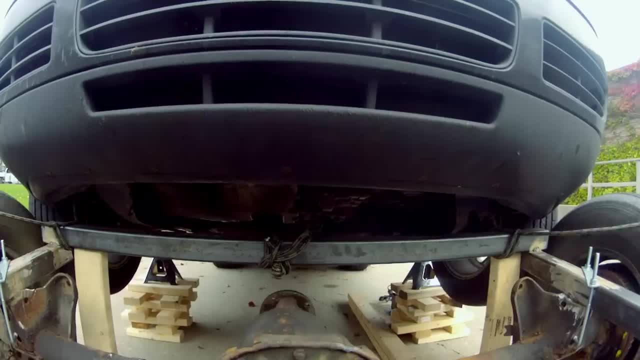 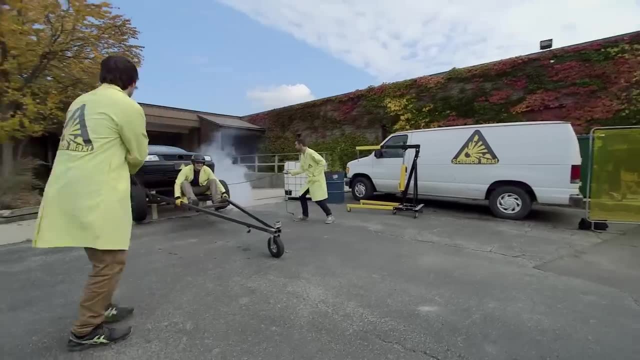 Keep it going All the way, Whoa, All the way. Three, two, one go Run, Run, Run, Run, Run, Run, Run. Yeah, Whoo-hoo-hoo-hoo, Yeah Yeah. 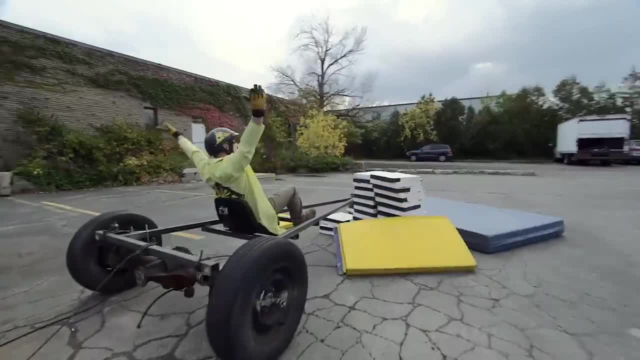 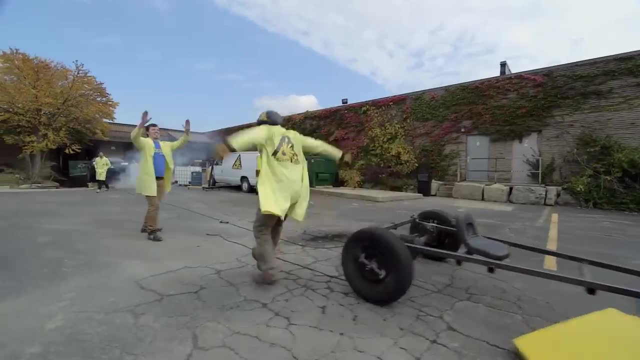 Whoo, How's that for inertia? Wow, look at that, That's amazing Cool High-fives. Yeah, Let's recap The weight of the tires as well as how fast they were going, provided enough inertia to accelerate me. 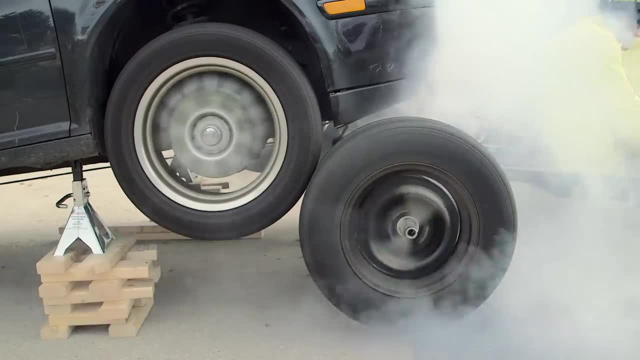 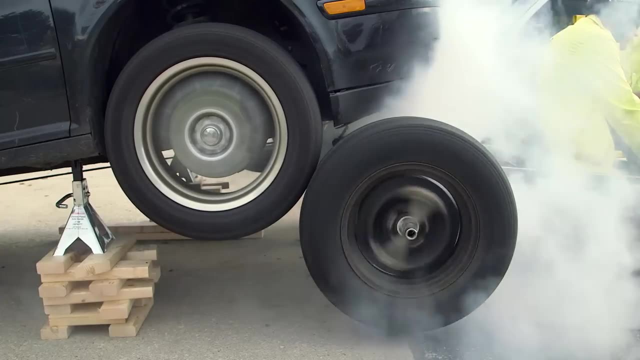 and the weight of the dragster, The objects in motion. the wheels wanted to stay in motion and the wheels wanted to stay in motion, and the wheels wanted to stay in motion, and the wheels wanted to stay in motion, so much they moved the dragster. 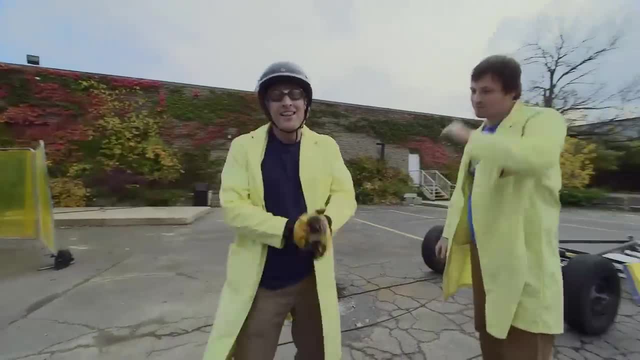 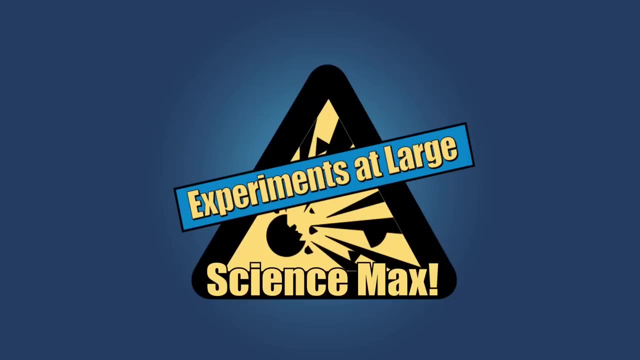 all by themselves: Inertia and Newton's first law of motion. Thank you for joining us on Science, Max, Let's go again. Your turn, Yeah, my turn, Okay. Whoo. Science Max. Newton's third law is the science. 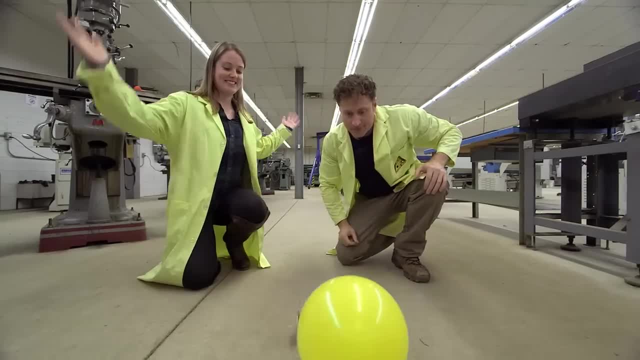 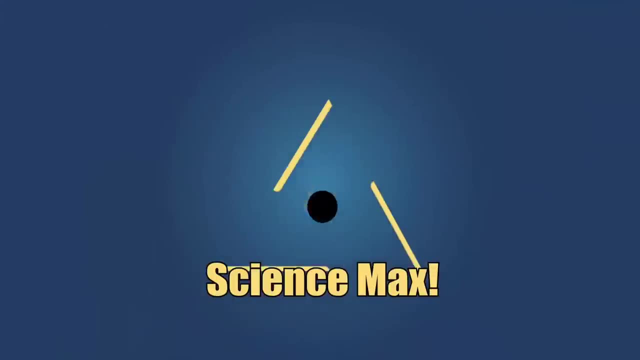 behind balloon-powered rocket cars. It's also the science behind a maxed-out rocket car that I can ride, plus bowling balls and an interrupting sign Today on Science Max experiments at large. Greetings, Science Maximites. I am Phil McCordick. 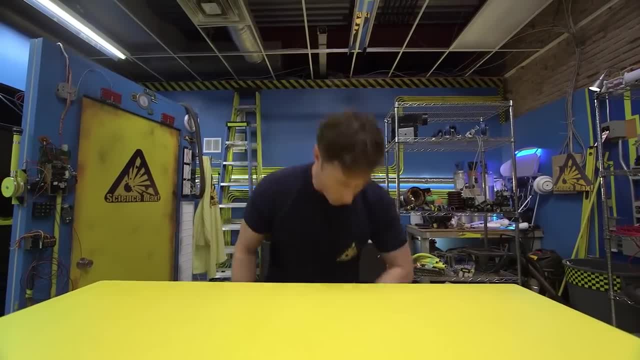 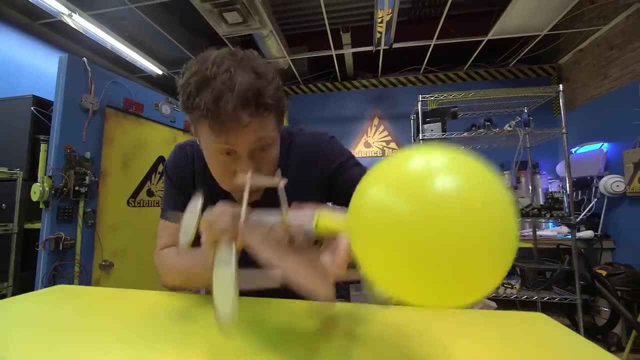 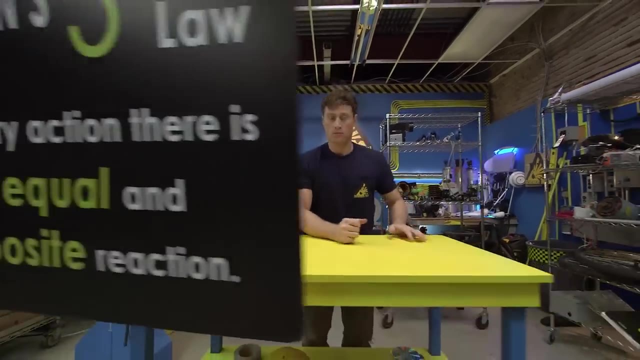 and this is Science Max experiments at large. Today, we're going to be experimenting with the balloon-powered car. Here's how it works. Whoo-hoo. It all has to do with Newton's third law. Newton's third law For every action. 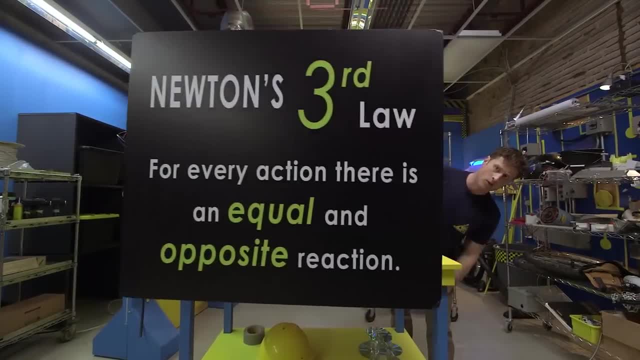 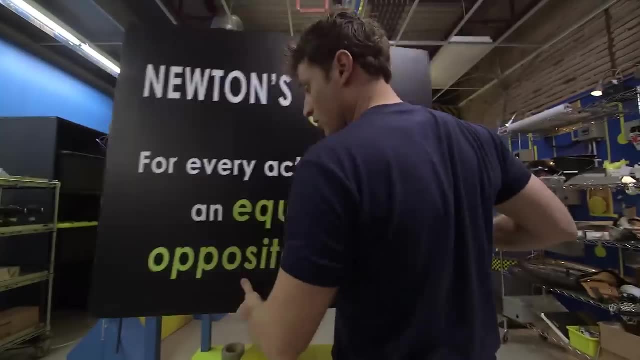 there is an equal and opposite reaction. Uh, we don't have to do this, now We can. This is all for later. We can build the cars first and then we can. Uh, Let's go over here. So how do you build? 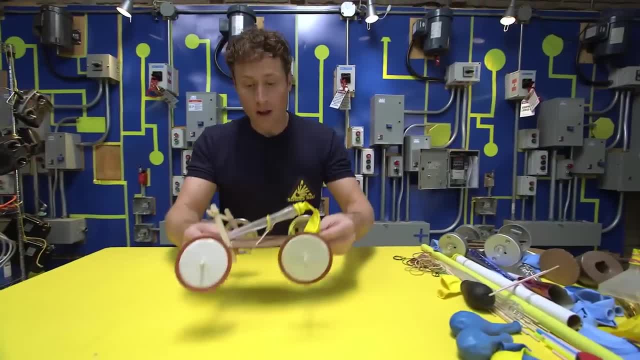 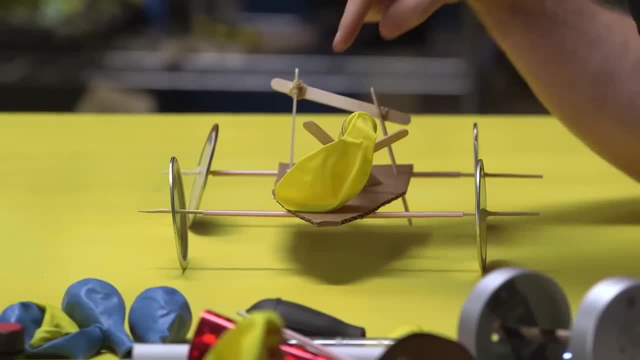 a balloon-powered car. Well, I suggest you be Science Maximites, because there is any number of ways you can build a balloon-powered car. You do not have to follow my design. You should come up with one of your own. It may even be better. 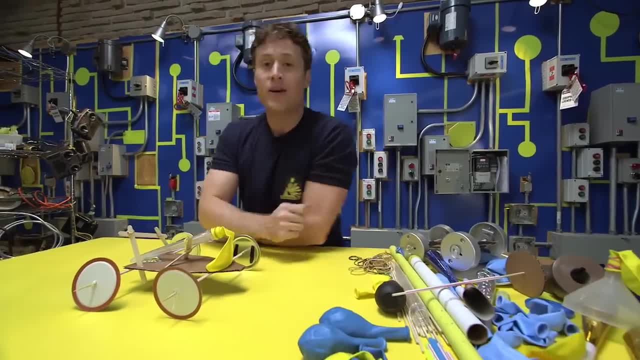 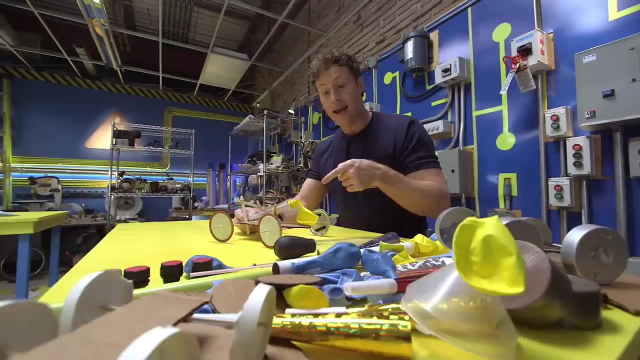 than the one I built, But I will give you some tips, though, that make it a lot easier. First of all, you need something to stick your balloon on that has an opening on it. I used a turkey baster for this car. 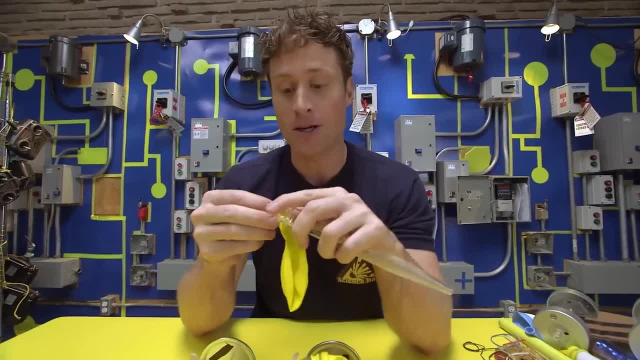 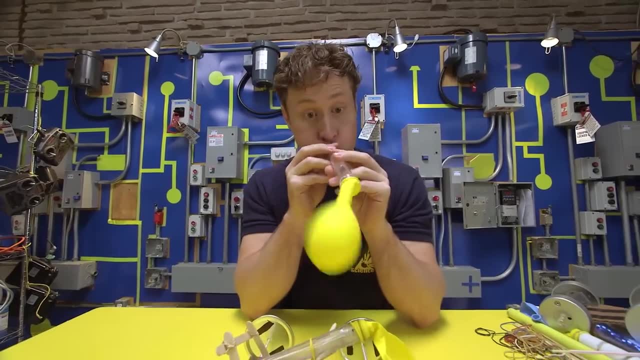 I just pop the top off and remember to tell an adult that you're using the turkey baster, And then you stick the balloon on there and it allows you to attach something to the car and it also makes it easier to blow up the balloon. 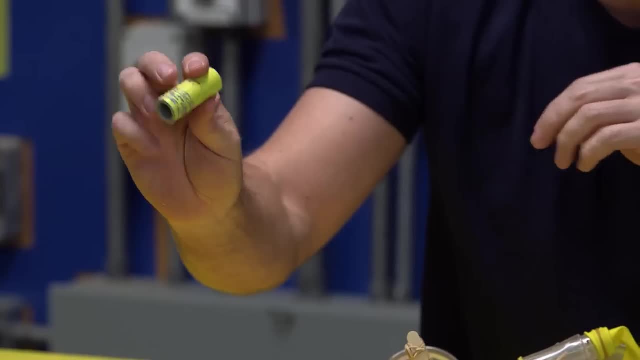 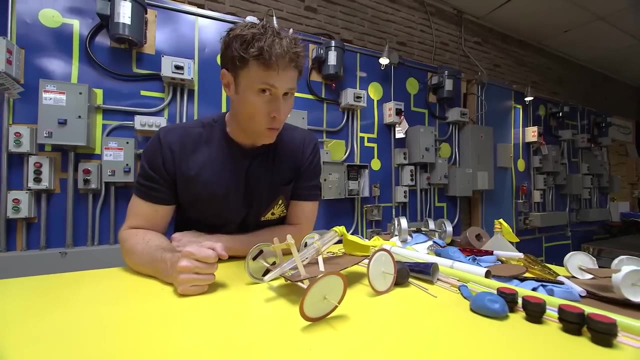 You can use any number of things, even just any kind of tube that you find lying around. It helps you attach the balloon to the car and it helps you blow up the balloon way easier- The other thing you can do when you make your balloon-powered car. 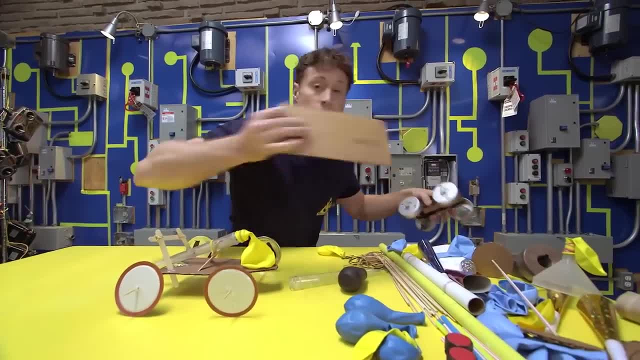 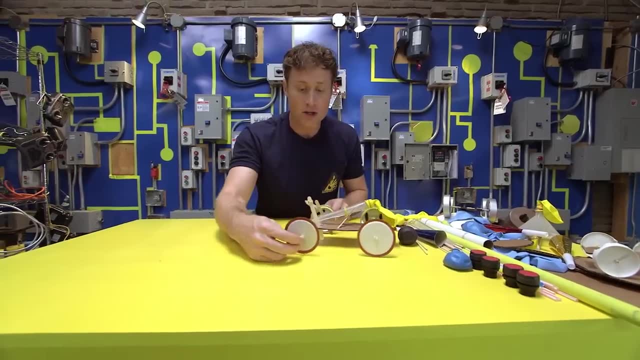 is how you're going to make the wheels roll. Once you've decided on the base of the car, you could use anything, even just a piece of cardboard like this. you can do your wheels in two ways. The first way is to attach. 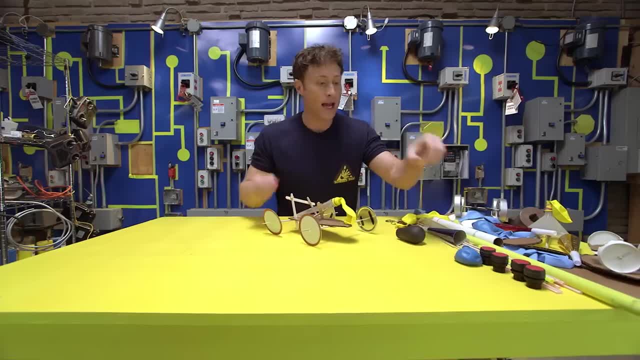 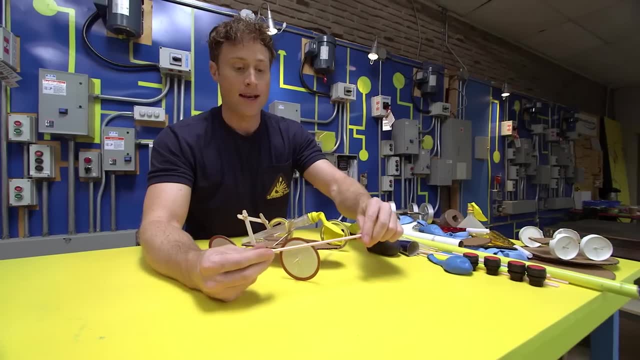 the wheels to the axle. This is how I made the axle of this car. I used a shish kebab skewer and I stuck it inside a straw, just like that, And then I attached the lids to the shish kebab skewer. 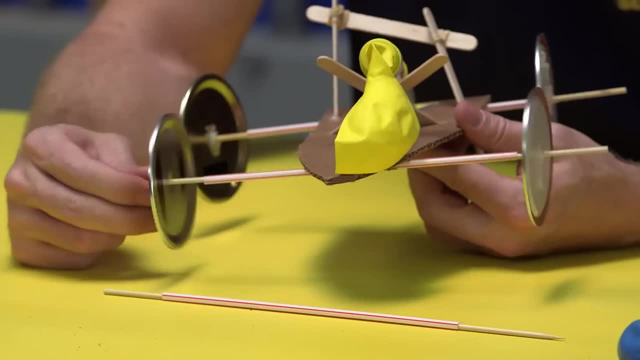 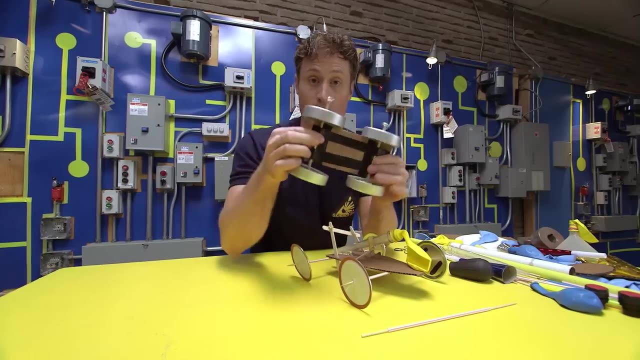 So the lids of the shish kebab skewer are attached and they rotate in the straw. That's one way to make the wheels turn. The other way is to tape down the axle, or whatever you're going to use, and have the wheels spin around. 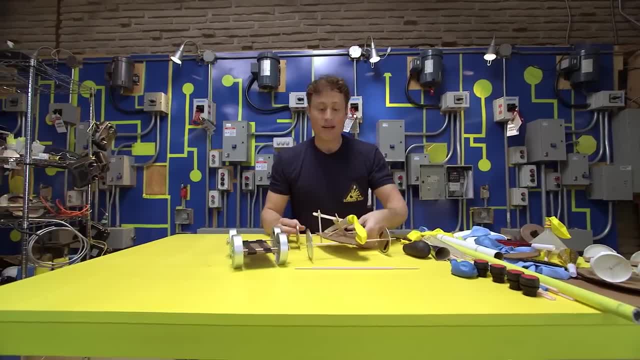 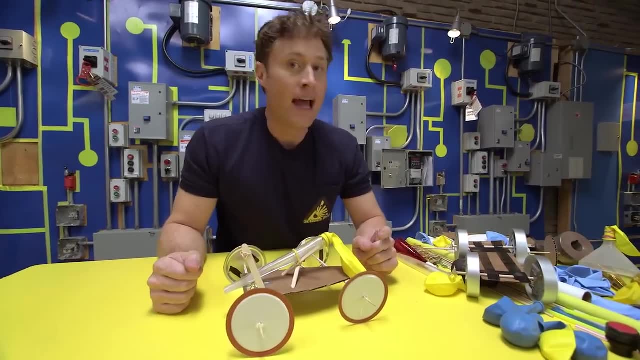 on the axle- Two great ways to make your wheels turn, and it really kind of depends on the wheels you're using. You can make your own design and keep refining it and making it better and faster, or do what I like to do and make a whole. 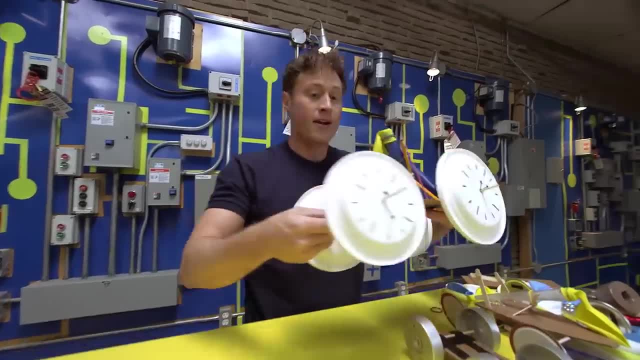 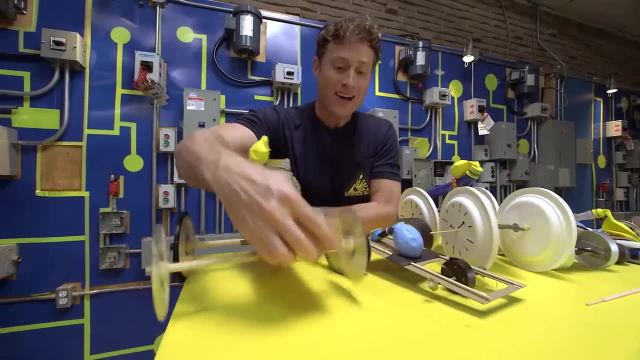 bunch of different cars. So we've got this one I made out of paper plates and this is a snorkel- Awesome. This one is the rock car, because there's a rock on it. I've got a dragster model. It's a long. 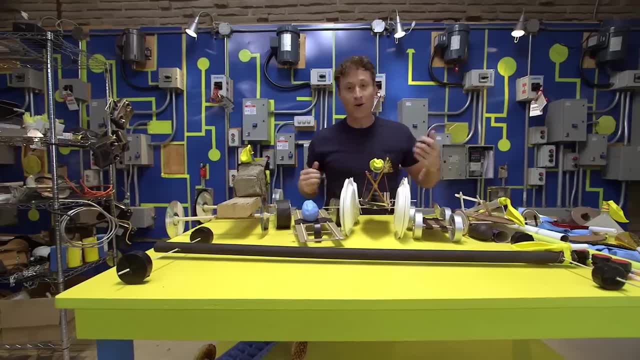 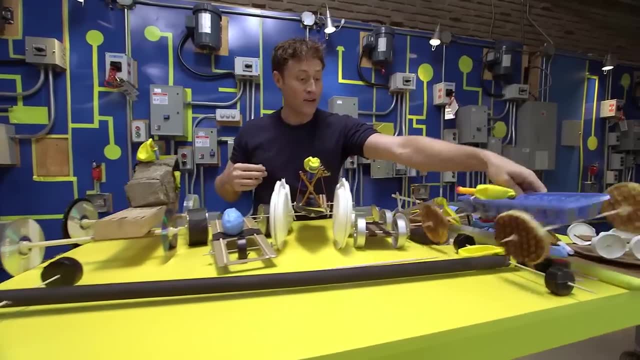 broom handle and it might not work that well. but who knows? And this is my favourite design: It's made out of waffles and an ice cube tray. This is why I make a whole bunch of different cars, because I can race them. 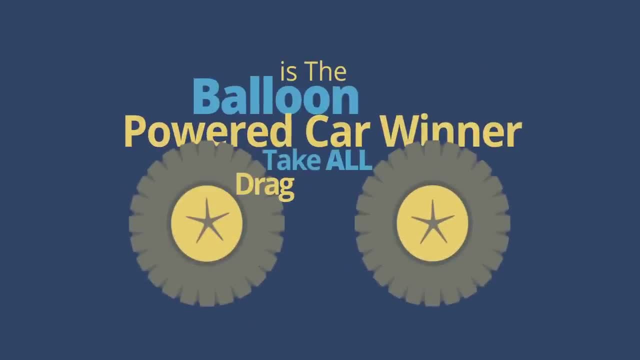 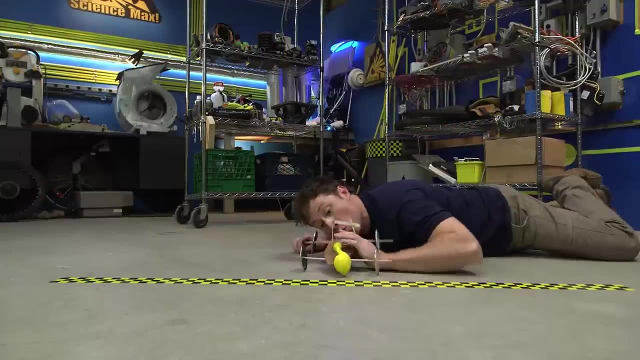 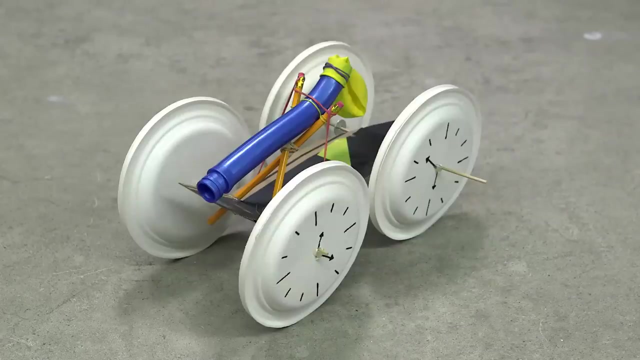 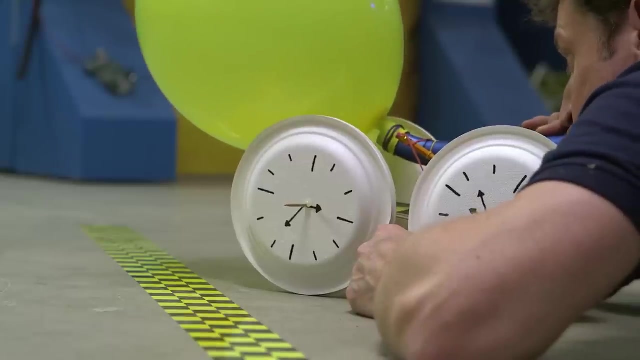 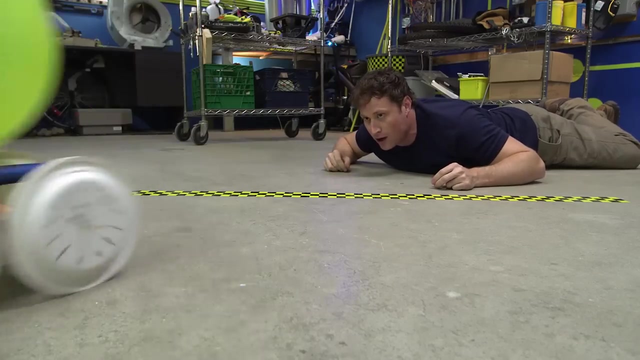 And the science max-a-drone. It's the balloon powered car winner. take all drag race off. awesome. First up the eliminator: Woohoo. Better late than never. it's the procrastinator Crushing the competition. it's the Terminator. 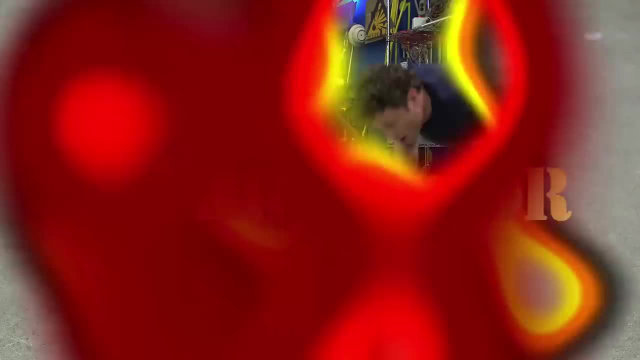 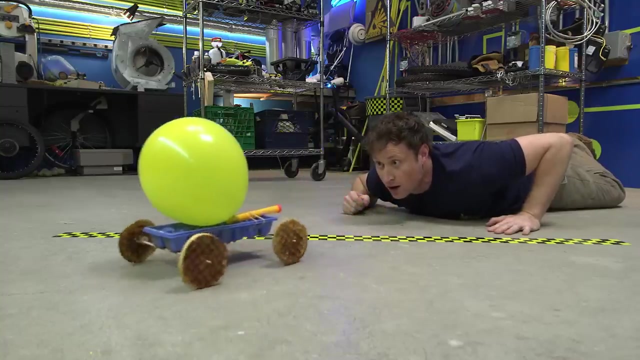 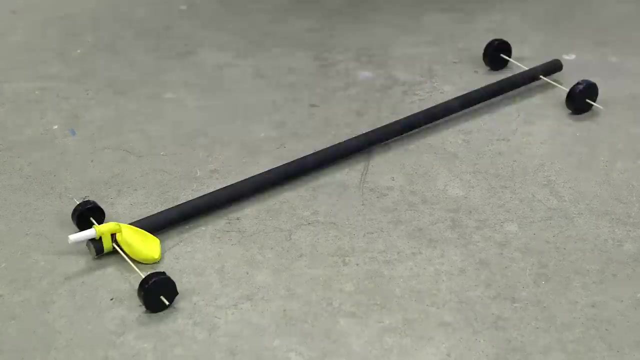 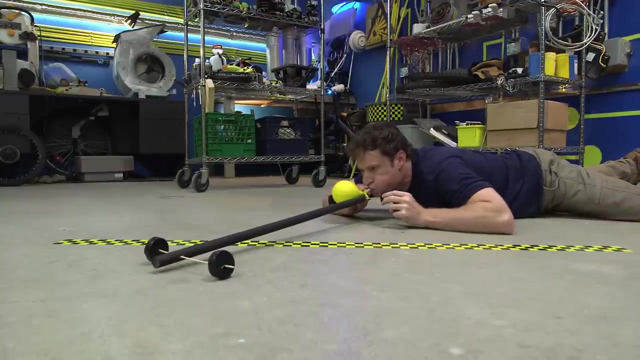 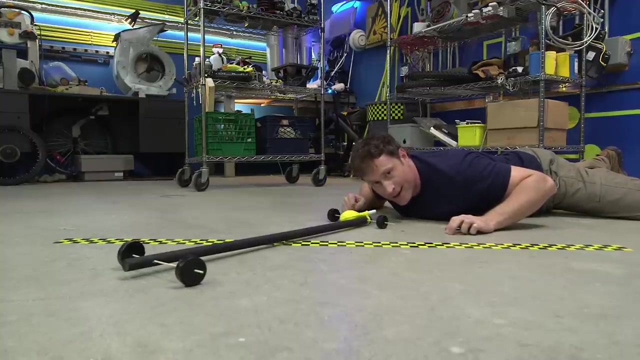 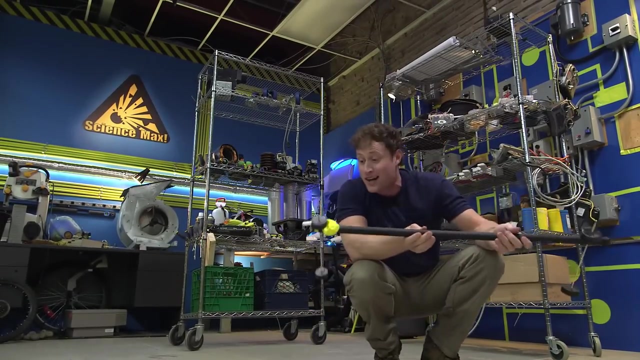 Feel the chill of the refrigerator And, last but not least, the um regurgitator. Ah well, when you build your balloon-powered cars, you can figure out what worked or what didn't work and try modifying your designs to make them work even better. 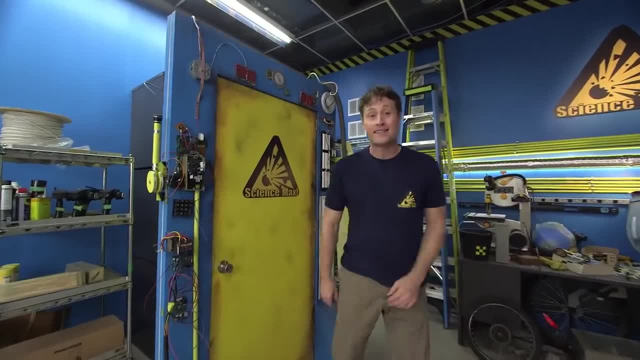 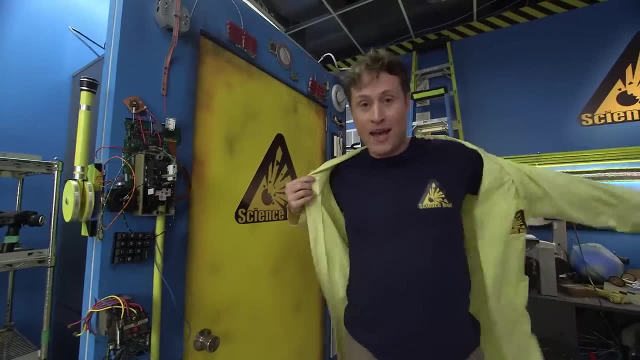 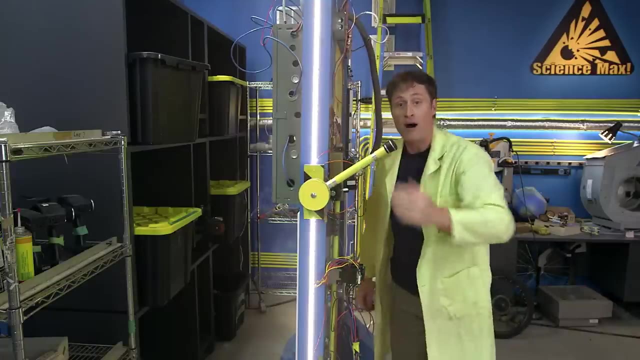 That is science, and now we're gonna max it out, because this is Science- Max Experiments at Large. So we're gonna take that small balloon-powered car that we just built and we're gonna make it much, much bigger. I'm gonna go to the Center for Skills Development and Training and we're gonna use the science. 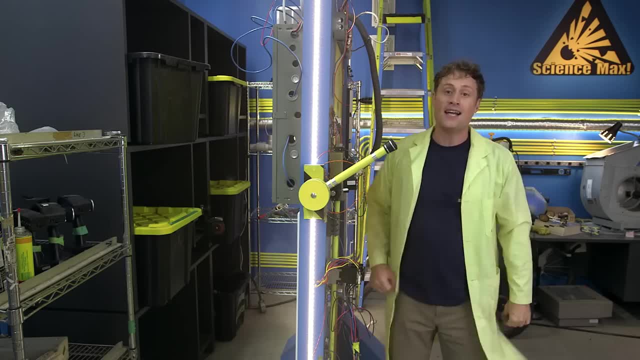 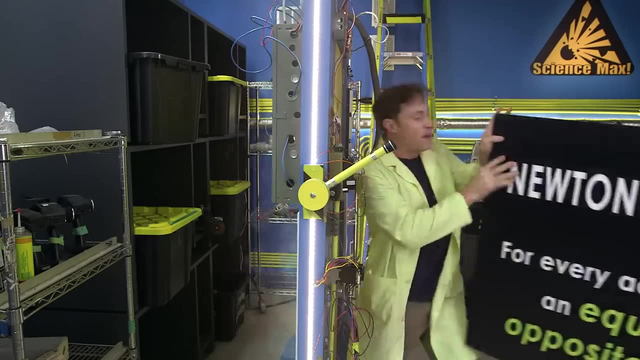 behind this small balloon-powered car and we're gonna make it big That science is Newton's Third Law. but there's plenty of time for this later. We're not doing. we're not doing this bit now, We're doing that bit. 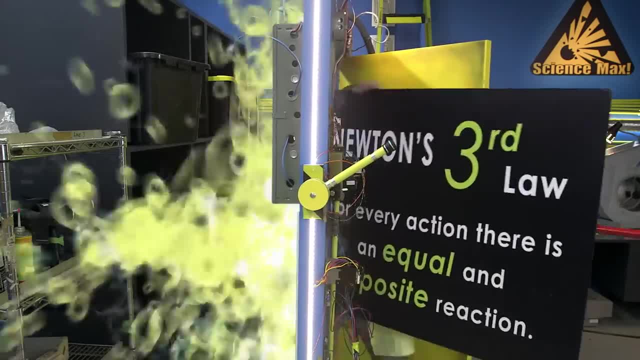 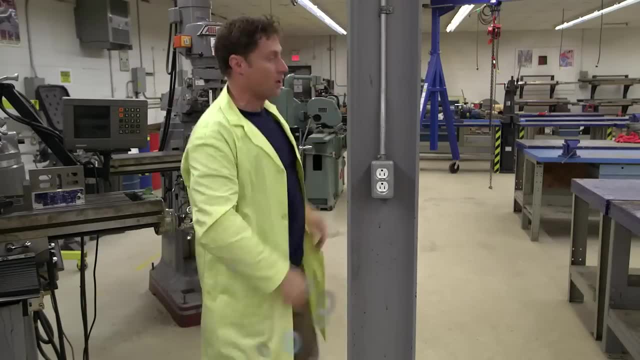 We're gonna do it in a minute, so we can. no, I, I said we're doing it later. We're doing it later Here, Whoa, Uh, hi Sarah, Hi Phil. This is Sarah and she's got a master's degree in physics from McMaster University. 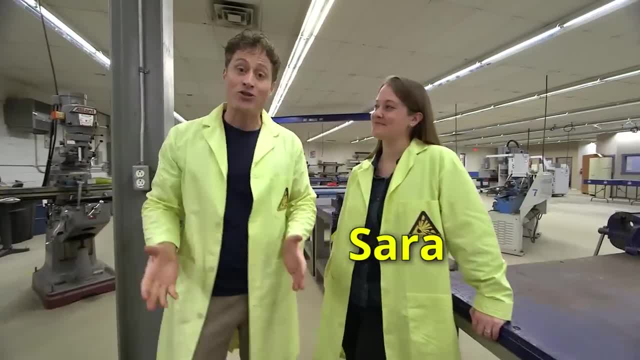 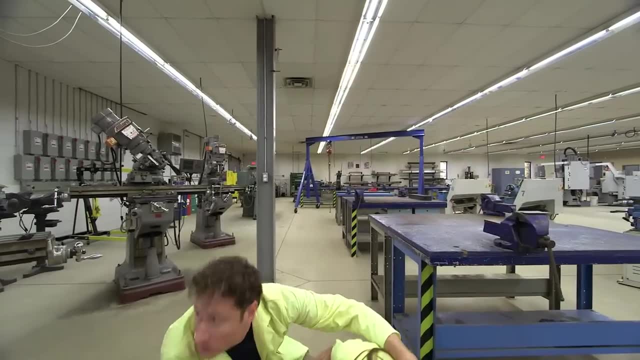 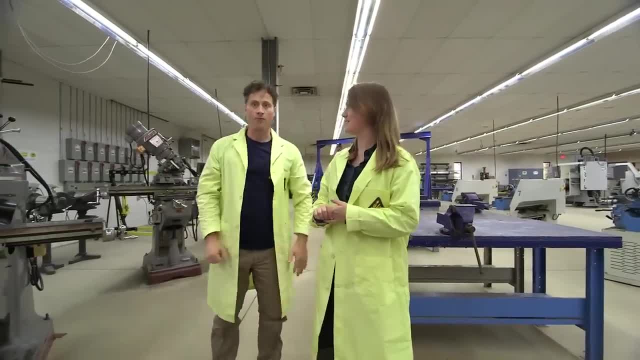 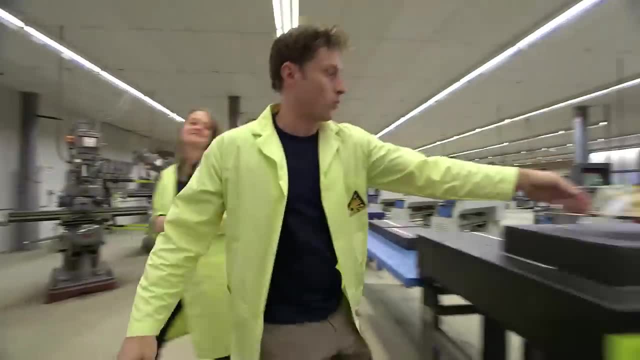 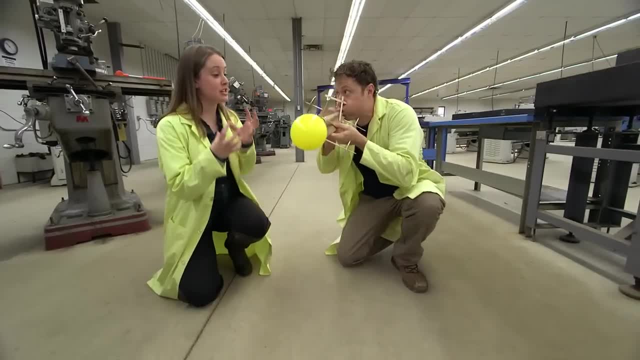 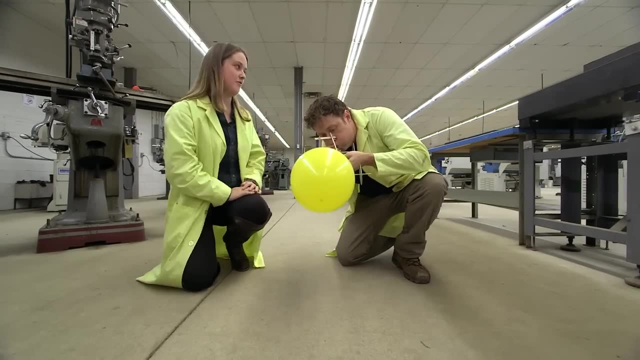 Okay. so if you blow up the balloon, what's gonna happen when you release it is the air's gonna push out with a certain force, which, in turn, is gonna cause the cart to move forward with the exact same force. Yeah, works great. 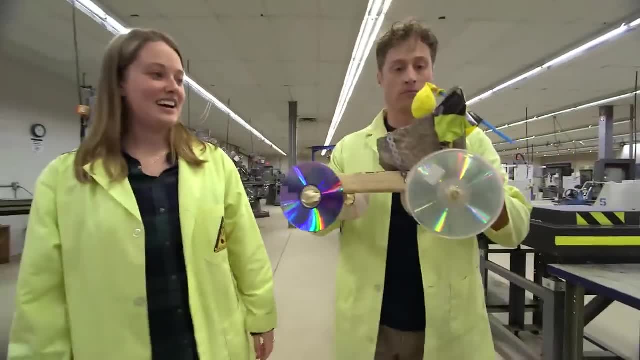 So how come it doesn't work with my rock cart? Ah, wow, Well, actually it did work. So the balloon still pulls out. So the balloon still pushes with the exact same force, which causes the cart to have. 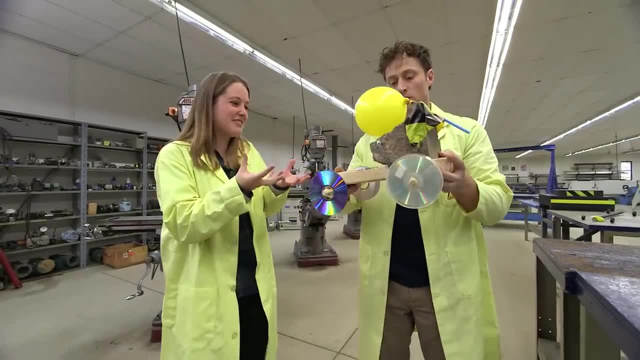 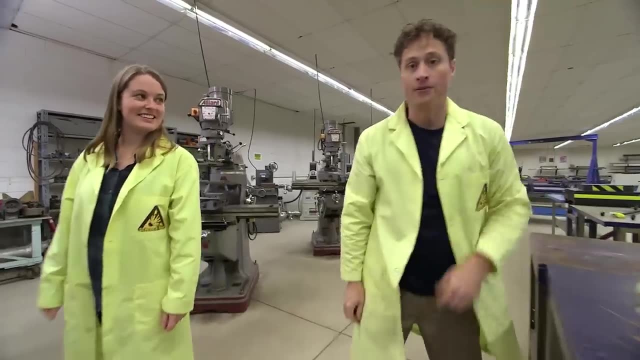 the exact same force, push forward, but your rock is really heavy, so you probably didn't see it move. Oh, so a lighter cart works better with the same amount of force. That's it. Well, there you go. Newton's Third Law. 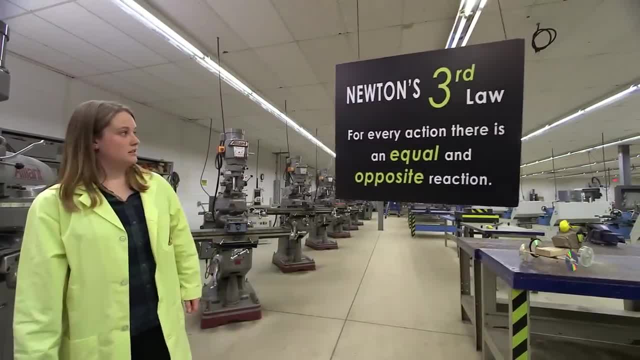 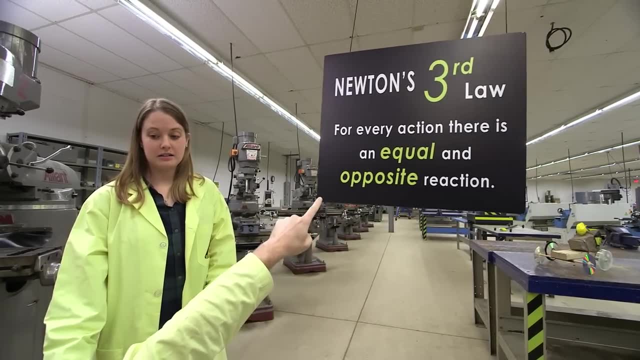 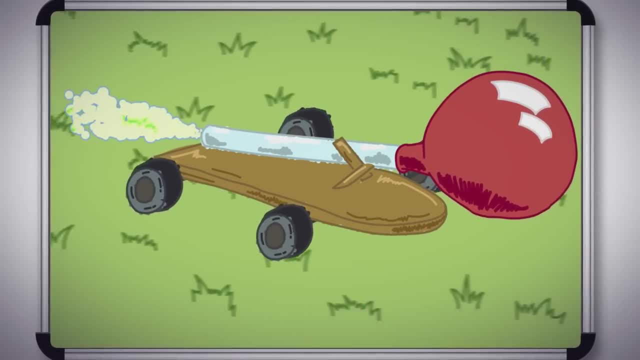 Our small balloon-powered car works because of Newton's Third Law: For every action there is an equal and opposite reaction. The air pushing out the balloon this way pushes the car with the same amount of force this way. So in order to max it out, the plan is just to get a bigger wheeled cart and a much bigger 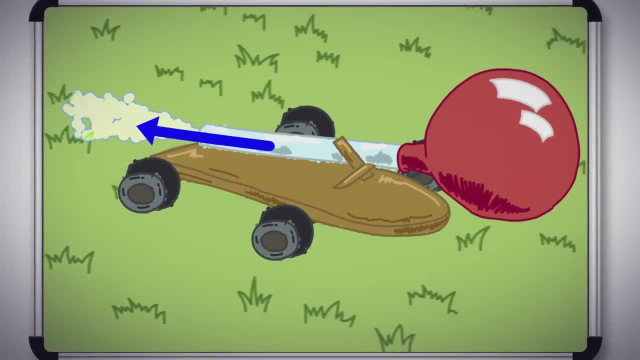 balloon, So everything should work out the same. Okay, So sorry. Whoa, Whoa, Whoa. I thought what we would do is I would, in order to get a bigger wheeled cart and a much bigger balloon, so everything should work out the same. 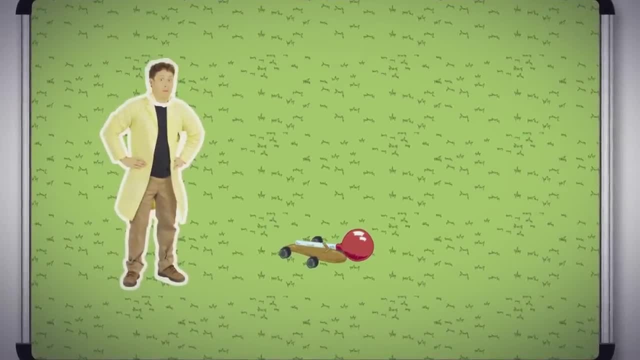 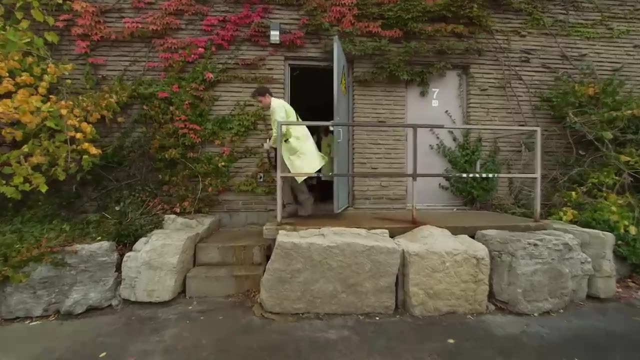 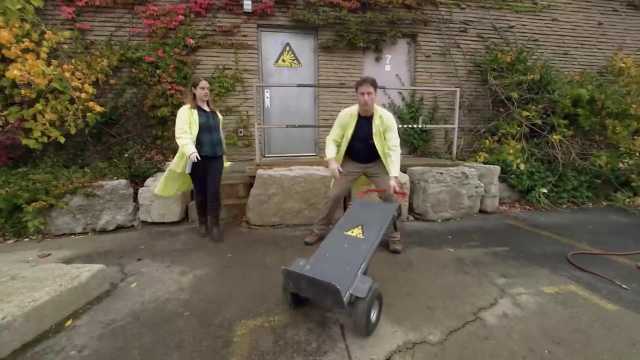 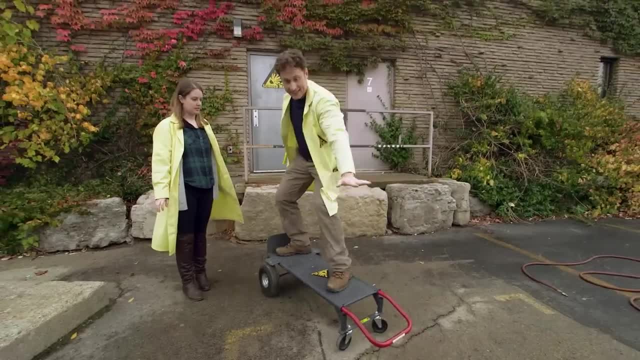 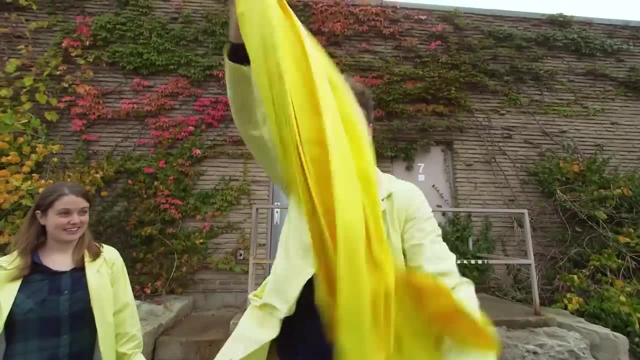 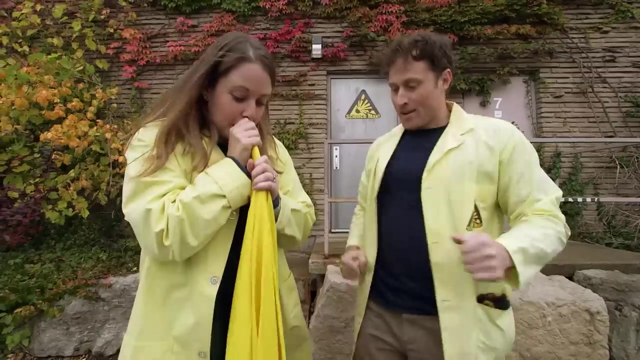 What we need is a cart to start with, and then I ride it And we have a giant balloon. and then I go: Do you have a giant balloon? Ha ha, ha, ha ha, Giant balloon. So, step one, Sarah blows up the balloon. 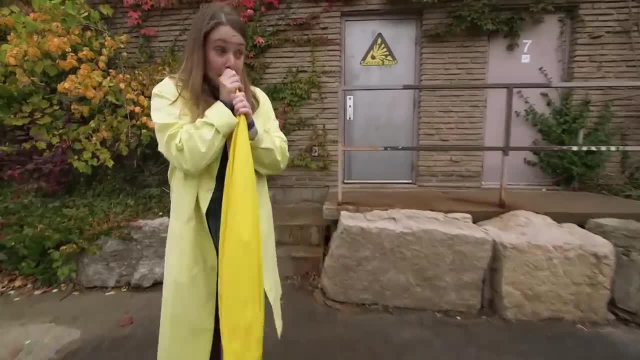 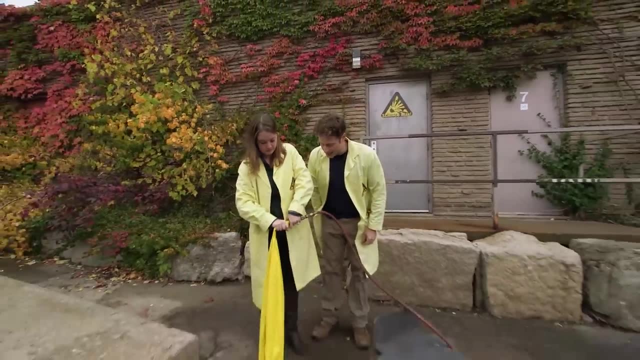 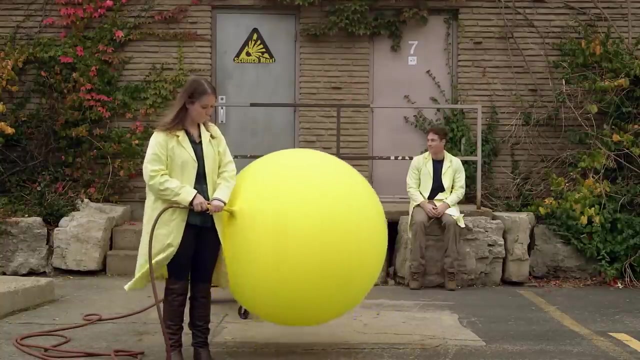 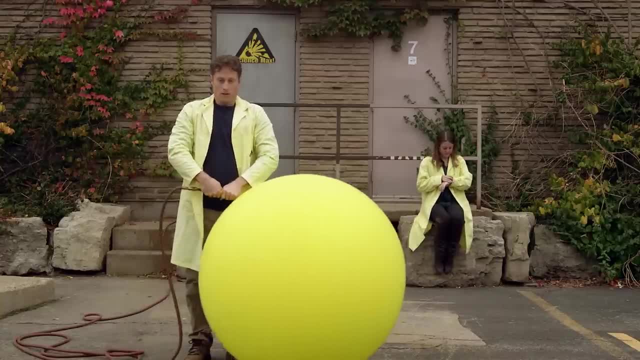 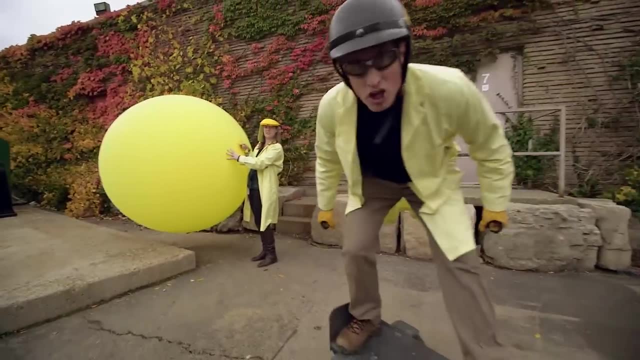 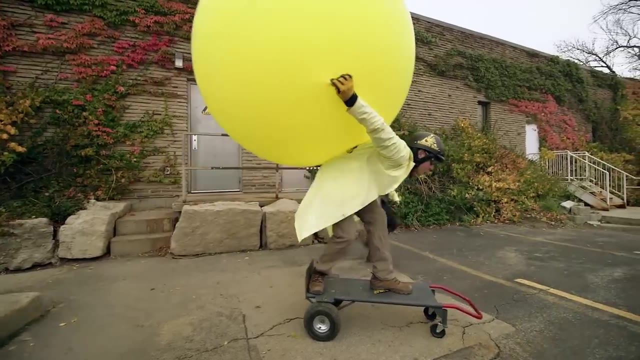 A very long time. Okay, human-sized balloon-powered car test, Take one. All right, Sarah, You got it. Yeah, Okay, let it go, Let it go go. Let it go. I did, You did, let it go. 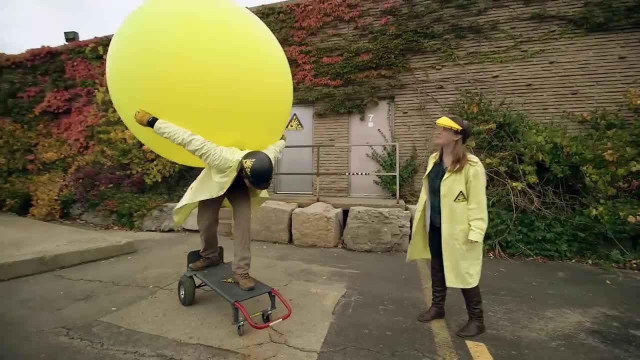 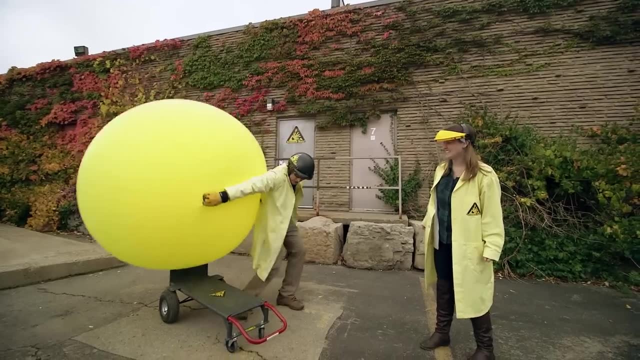 I let go. Nothing is happening. It's not coming out fast enough and you're a bit too massive. I don't think it's gonna work like this Really. Yeah, Okay, Balloon-powered car test two: No fill. 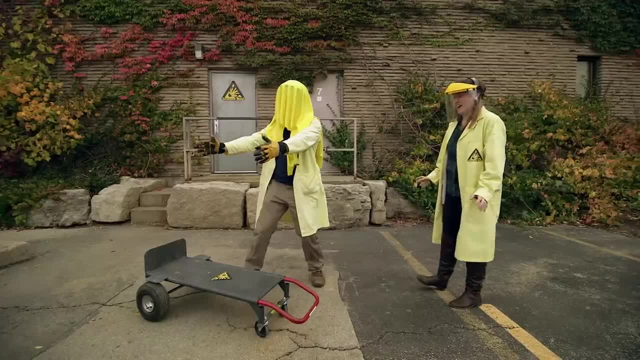 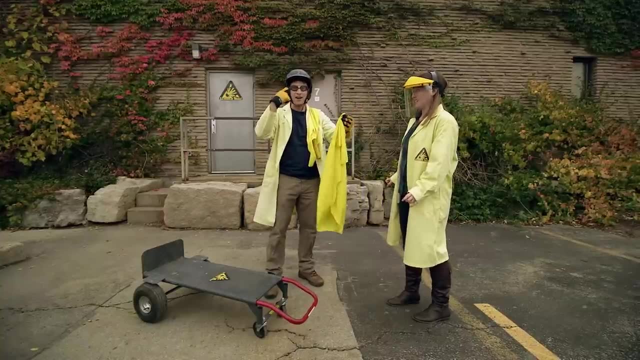 I'll just take it. What happened? I don't think it worked. The balloon popped, Phil you, okay. This is why you wear protective eyewear. Uh, yeah, So that didn't work. No, No, Should we get another balloon? 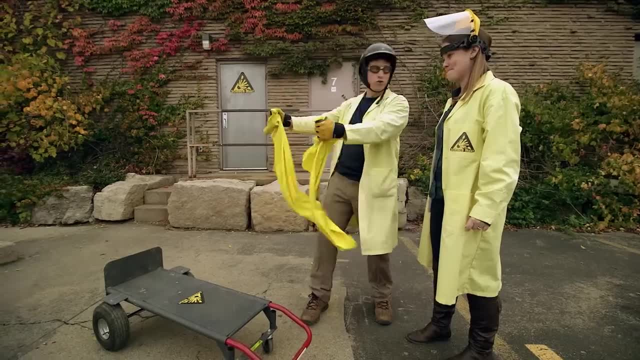 I think we need something else. Okay, well, the air coming out of the balloon just didn't have enough force, so We need the air to come out with more force. Yeah, Do we get? what a bigger balloon. I don't think that's gonna work. 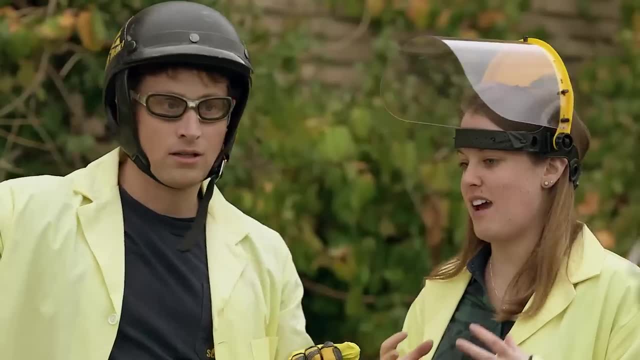 I don't think it's that. I think we need something with compressed air, Oh, like a scuba tank or a Fire extinguisher, something like that. Yeah, that's what we need. Okay, sure, Well, we can. 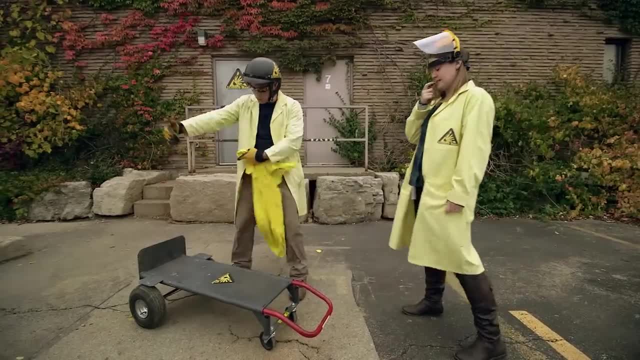 All right, so I don't know if that's safe to do that, so we'd have to build like a cage or something. Yeah, I don't know if it's gonna work on this. All right, well back. 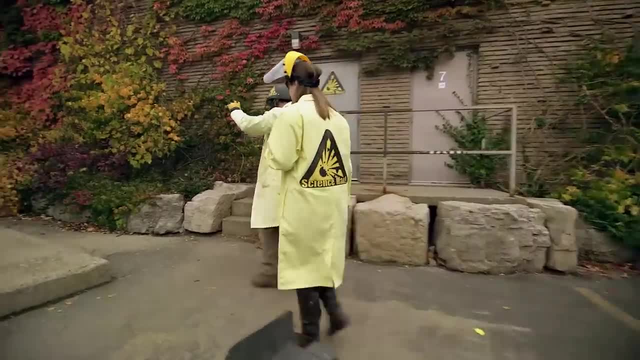 Back to the drawing board, Okay. So what we should do is we should get a. We need to find these tanks, Get the tanks and then we make like a frame out of aluminum or something. Okay, that could work. 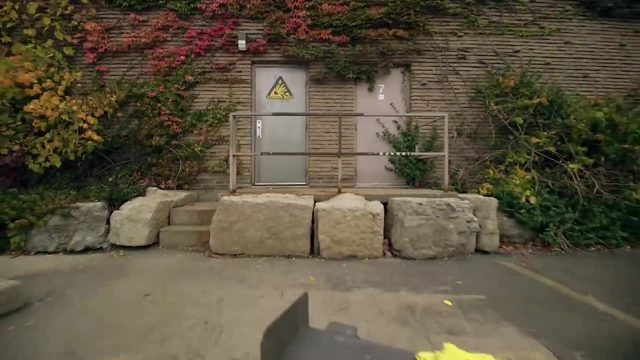 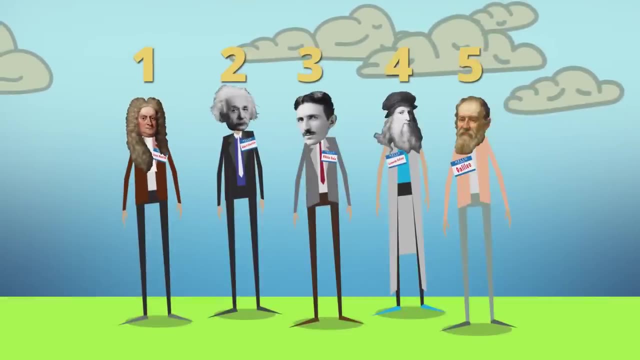 It's a good idea. Yeah, they can hold the tanks, so they're safe. And then what we should do is: Who was Isaac Newton? He was a mathematician and probably number one on the list of top scientists of all time. 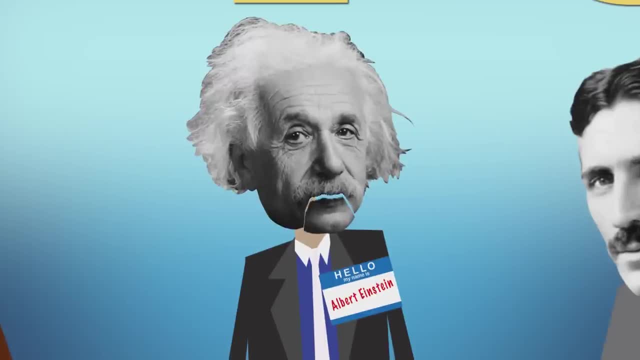 Albert Einstein said: "'Isaac Newton was the smartest person that ever lived. "'You've got to be special "'if I'm the smartest person in the world'". Einstein is calling you smart. Newton's three laws of motion was a huge idea. 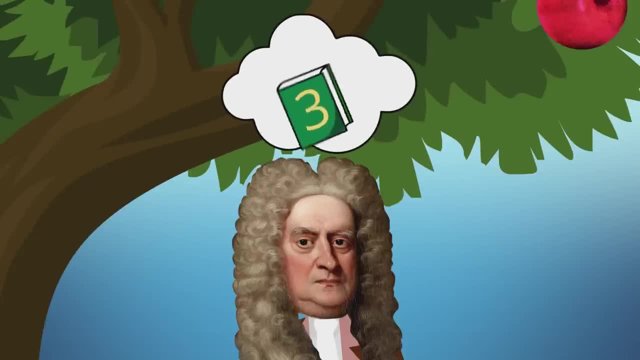 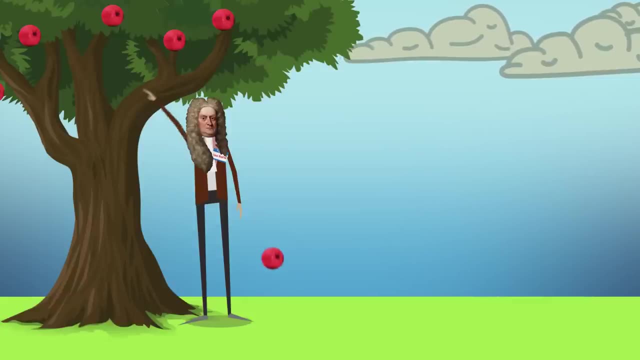 but did you know? Newton also came up with the idea of gravity. The famous story is that in 1666, Isaac Newton was sitting under an apple tree when he watched an apple fall and wondered why? Hey everyone, I just invented gravity. 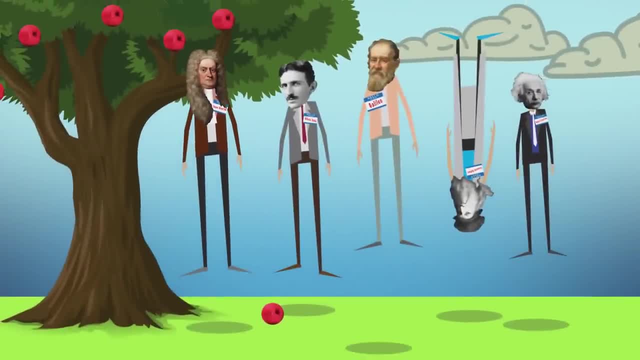 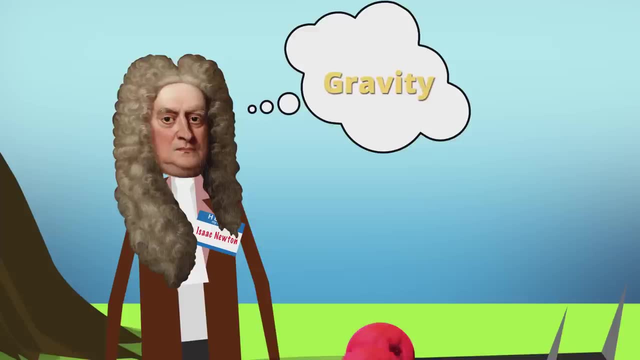 which was a big relief, because up until then, everyone was just floating around. Okay, so it didn't happen like that. He didn't invent gravity. He gave a name to this invisible force and then described how it works. Not only did it make things fall down, 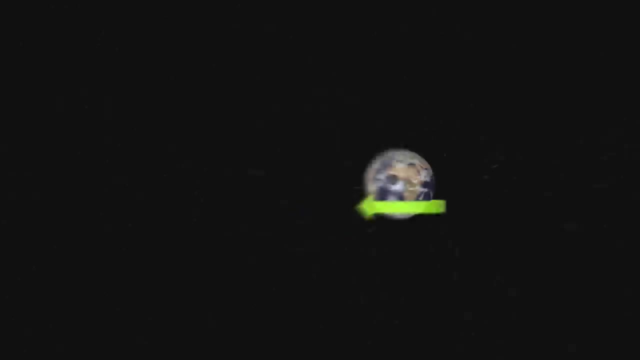 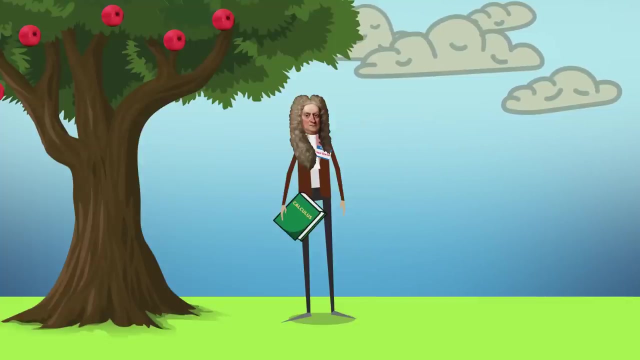 but it was the same force that kept the Moon circling the Earth and the Earth circling the Sun. And he invented a new kind of math to explain how We now call it calculus. See, I told you he was smart. He's very smart. 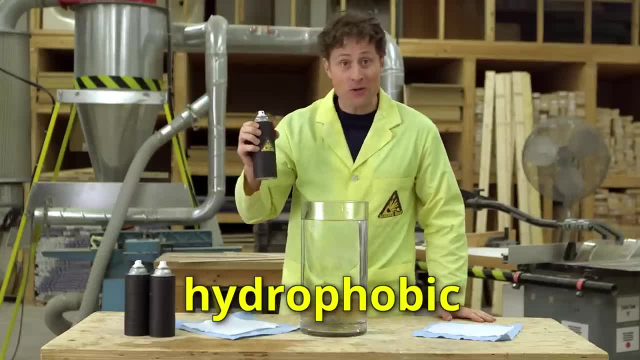 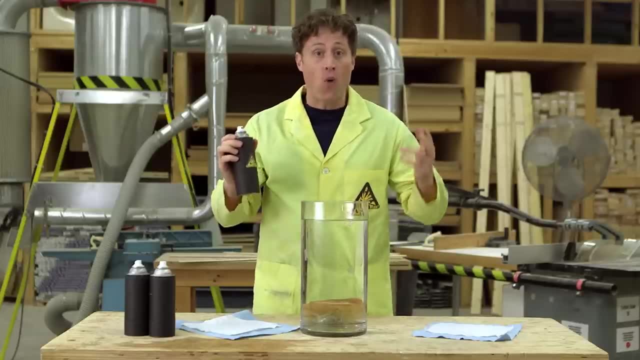 This is hydrophobic coding. Hydrophobic literally means afraid of water, But it's not actually afraid of water. The chemistry of a hydrophobic coding prevents water molecules from penetrating anything you spray it on. You can get this stuff at the hardware store. 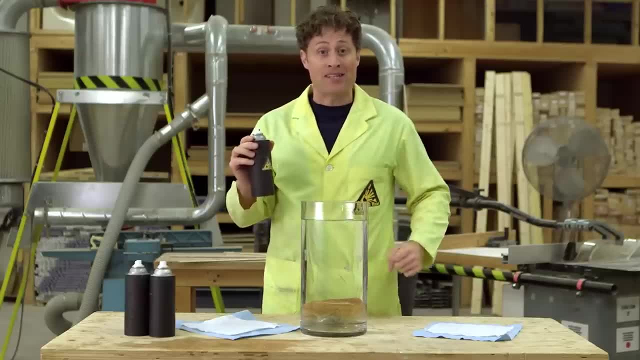 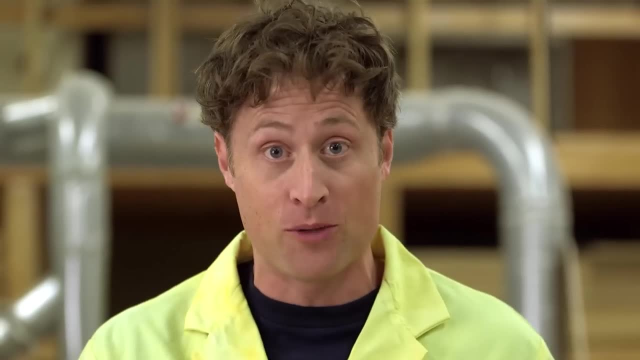 and, if you want, be science maximites and get an adult and think of the coolest thing you could spray with hydrophobic coding. I like to use things that do not go well when you put them in water, like uh tissue. 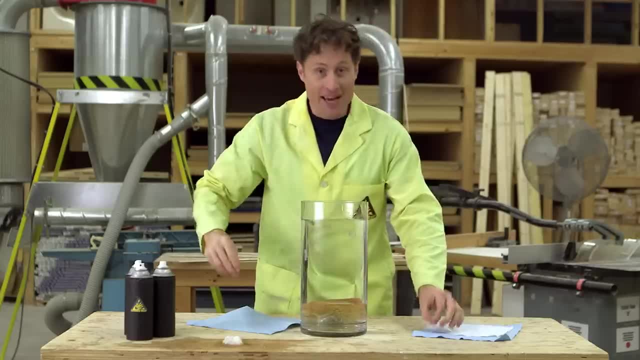 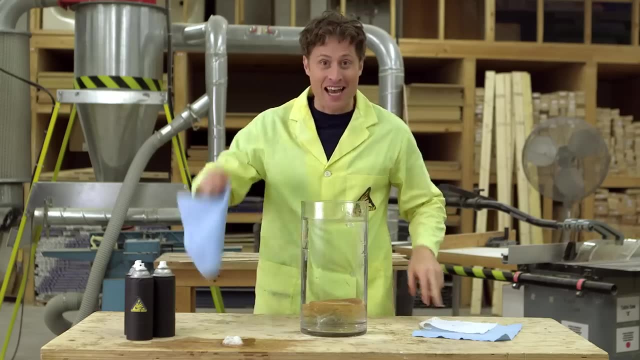 Yeah, doesn't look great when it gets wet. Here's a tissue coated in hydrophobic coding. Huh Weird. Or it works the same with a paper towel. Paper towel in water, Paper towel covered in hydrophobic coding. 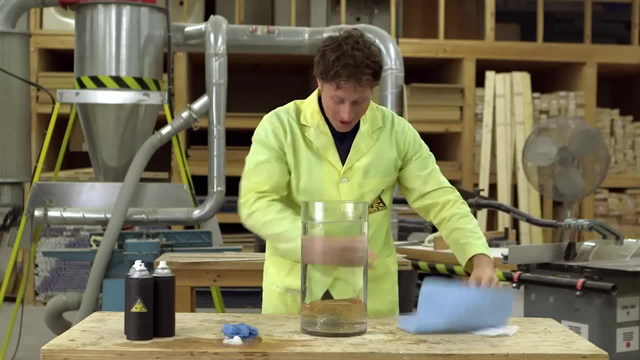 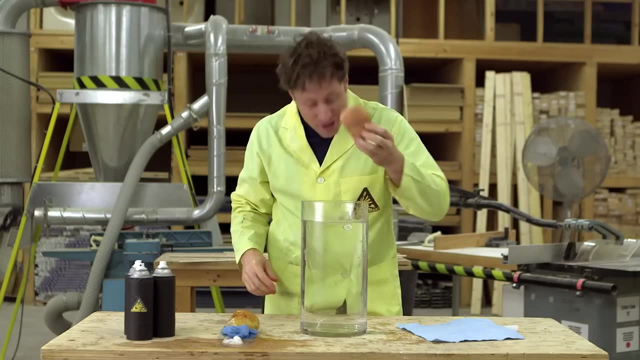 stays dry. Or how about a dinner roll? Dinner rolls really don't like water, See Gross, But a dinner roll coated in hydrophobic coding- Weird, Just don't eat it. Now it's time to max it out. 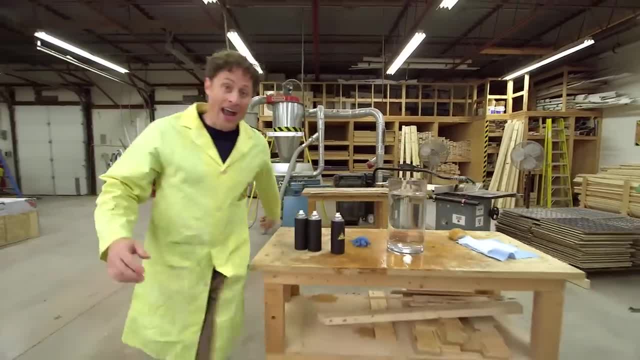 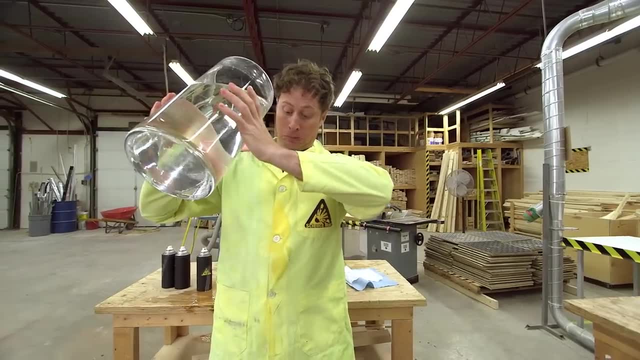 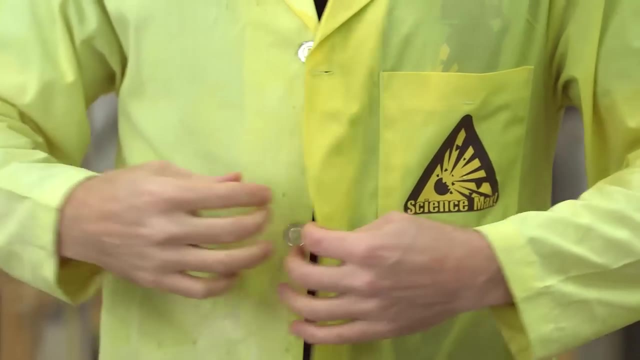 I have coated half of my lab coat in hydrophobic coding and the other half I have not Hydrophobic coding regular lab coat. Half of me is wet and half of me is dry. What's more, half of my outfit ended up being wet and half dry. 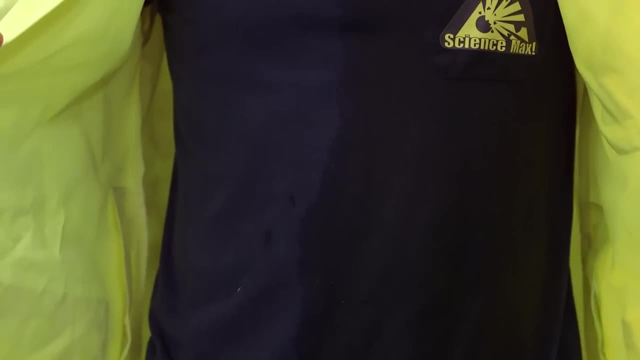 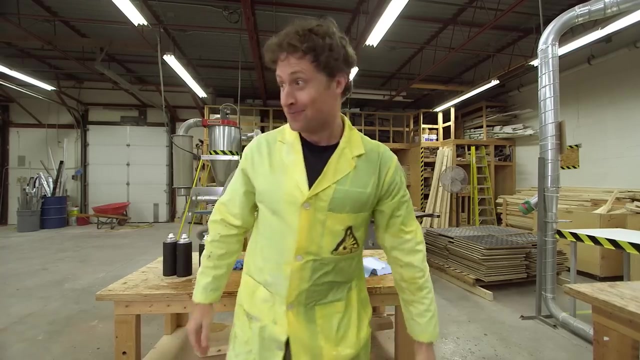 because the lab coat was protecting my outfit from getting wet. Now it's time to max it out even more. We have coated half of my lab coat in hydrophobic coding and more: We have coated my entire outfit in hydrophobic spray. 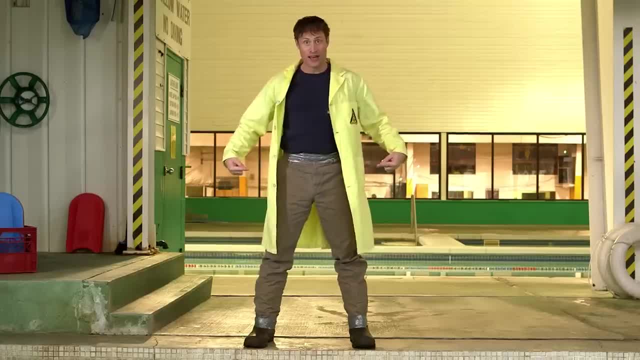 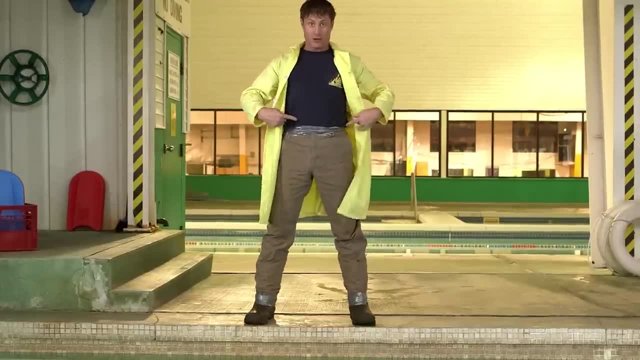 My shirt, my pants and my lab coat. The pants have been taped to rubber boots, so no water's getting in there, And my shirt has been taped to my pants, so no water's getting in there. So here's the question. 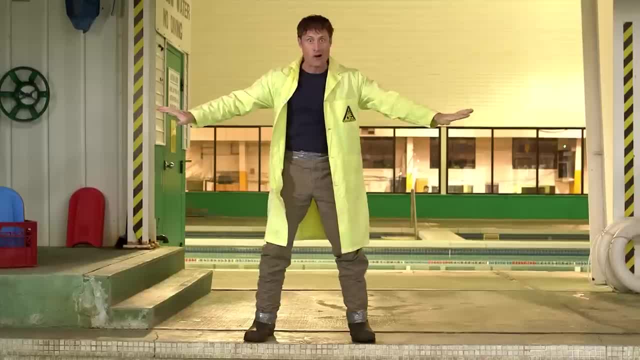 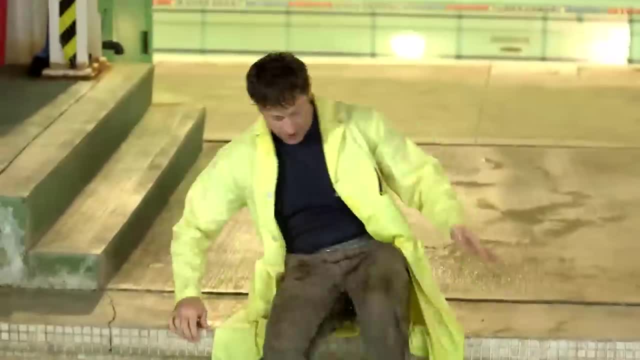 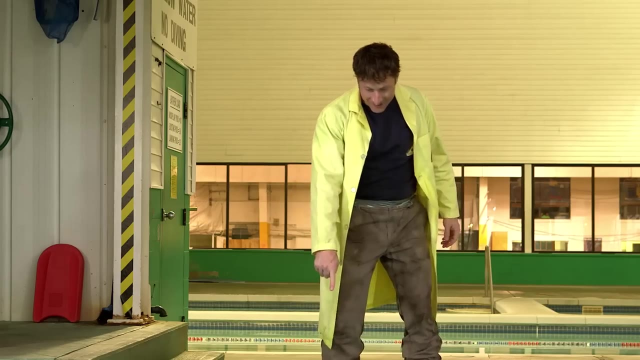 Can I get into the pool and out of the pool and stay dry? Let's find out. In the pool, Out of the pool- And I'm still mostly dry. Now here's what really happened. I got into the pool and I realized I should have duct taped the pocket. 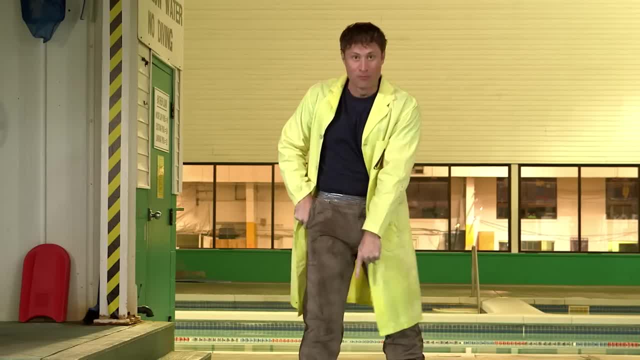 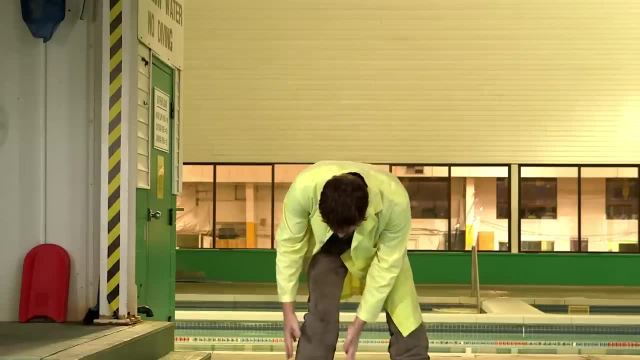 because all the water went in there down into the rubber boots, started filling up the rubber boots and now my entire leg is full of water because the hydrophobic coding isn't letting it come out. So the hydrophobic coding isn't keeping the water out. 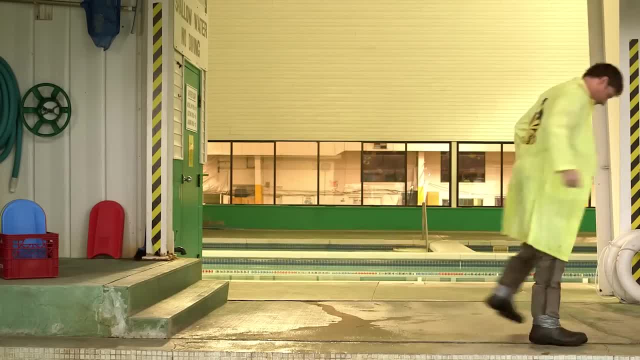 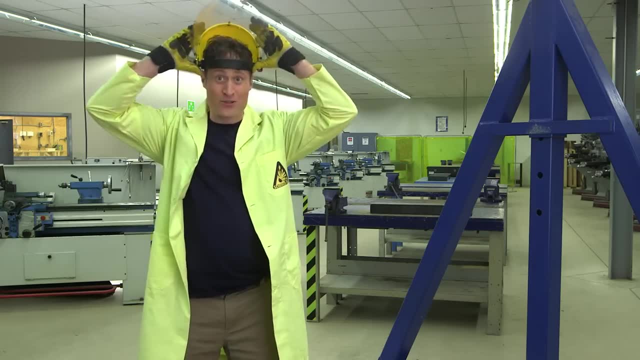 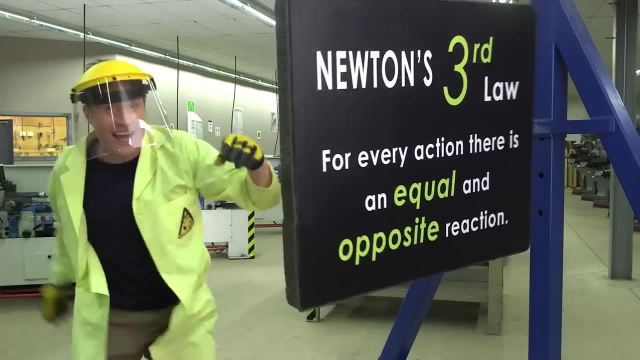 now it's keeping the water in. Let's take a closer look at Newton's Third Law. Newton's Third Law: For every action, there is an equal and opposite reaction. Okay, All right, let's watch it back When the sign hits me. 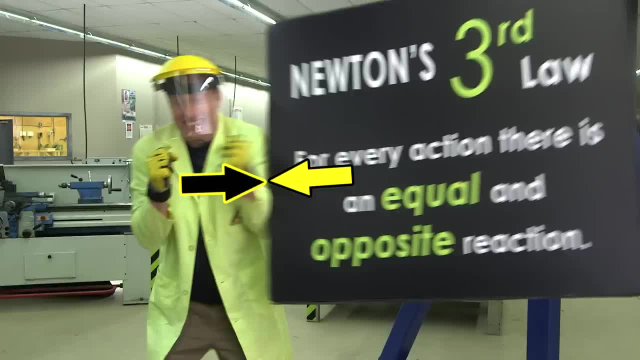 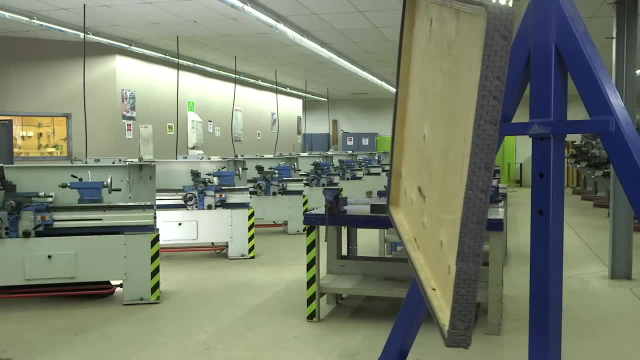 I exert a force on the sign in the opposite direction That makes the sign stop moving. It also exerts an equal force on me, causing me to fly off in this direction. Now, if I was to push this sign? I'm not only pushing the sign this way. 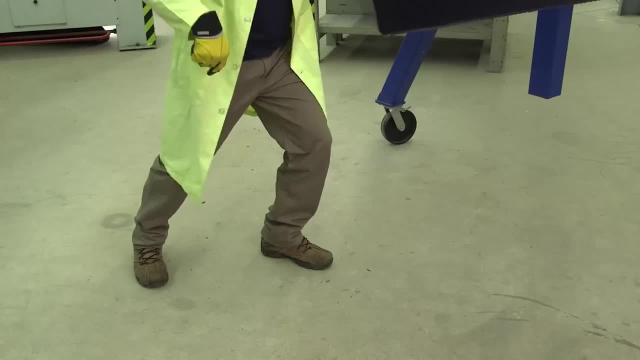 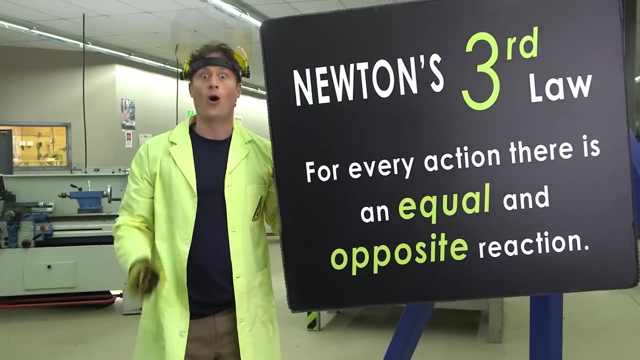 but my feet are pushing against the ground in the opposite direction. It's: um, Well, it's really easier to see if I'm not standing on the ground. Um, Oh, hold on, Okay, so Huh, Oh, okay. 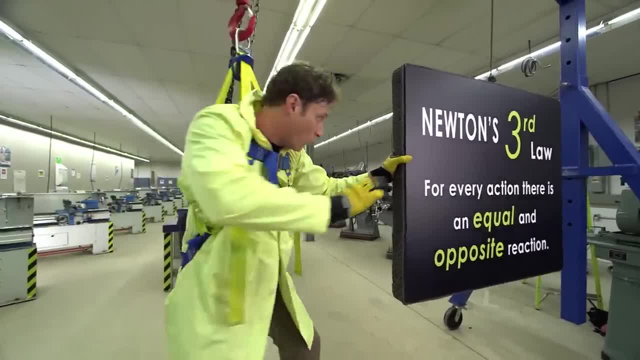 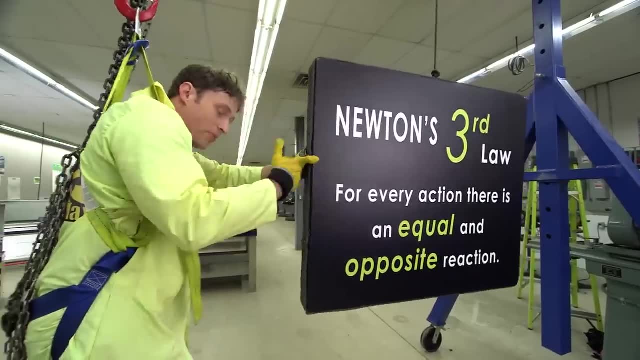 So now that I'm hanging watch, I push on the sign, but when I exert force on the sign to make it go this way, I go that way. Well, actually it doesn't work as well because the sign isn't as heavy as I am. 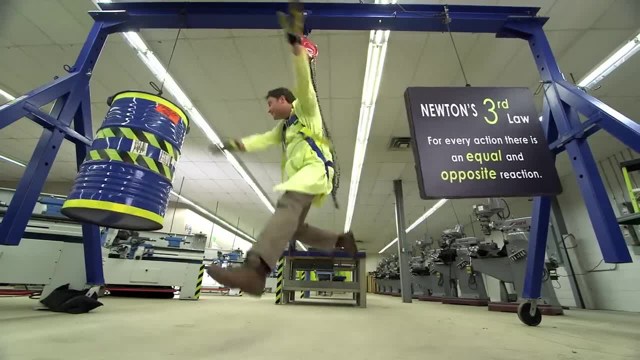 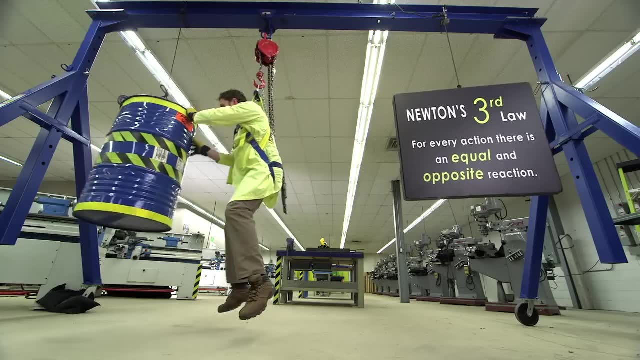 So wait, I have this over here. This is a barrel and it has stuff in it and it weighs as much as I do. Okay, so watch, If I push on the barrel like that, I go away from it as much as it goes away from me. 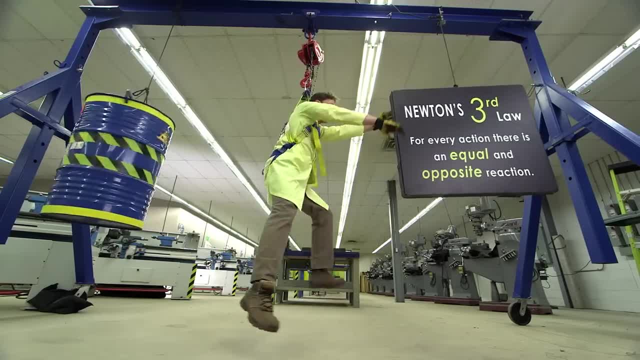 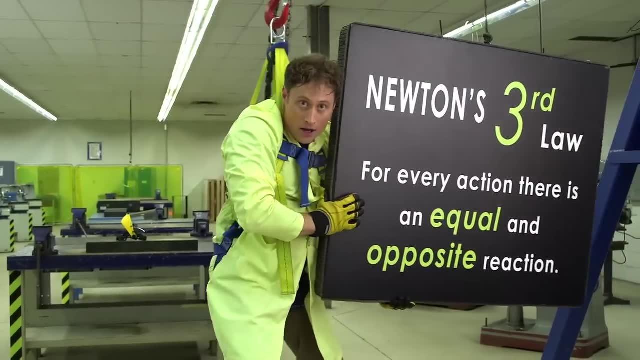 So there you have it: Newton's, Newton's Third. No, hold on. Newton's, Newton's Third Law. Newton's Third Law, Okay, go. Newton's Third Law. For every action there is an equal and opposite reaction. 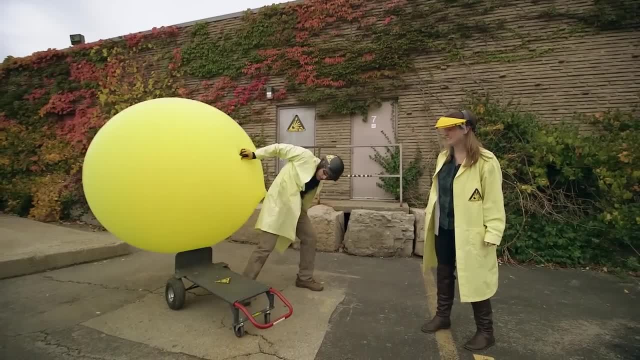 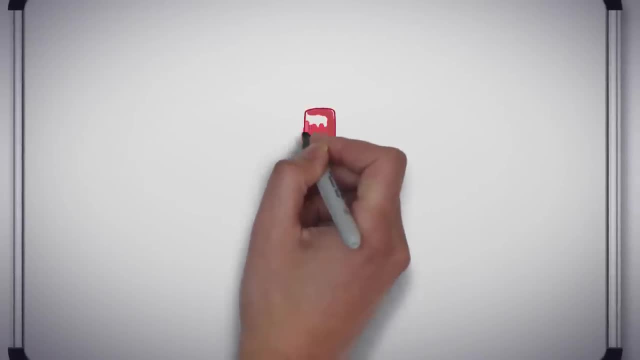 So using a giant balloon to push me on a cart, uh didn't work, And I What happened? The plan now is to use a compressed gas cylinder. Just like a balloon, these cylinders contain a lot of air. If we get a cart and put a gas cylinder in a cage, 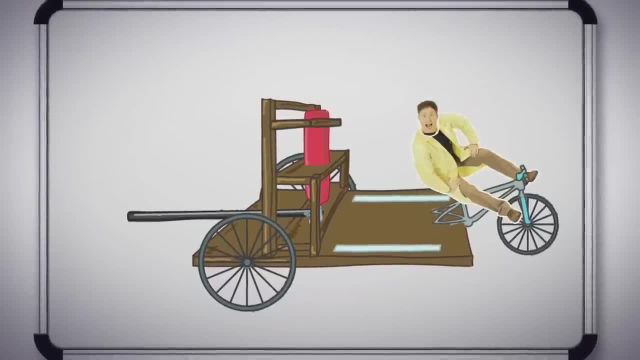 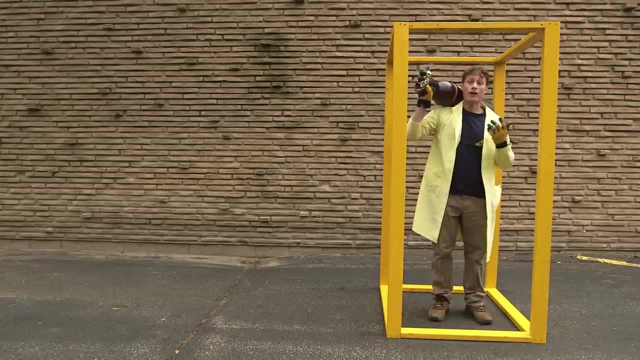 for safety on the back and open the valve, the escaping air might have enough force to push me. This is two cubic meters of air. If we were to put it in a balloon, the balloon would be this big. But if we compress the air, 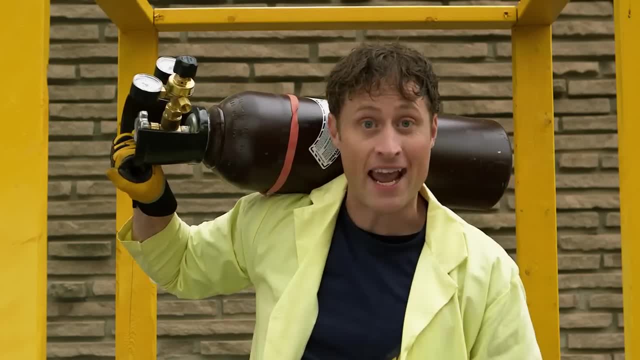 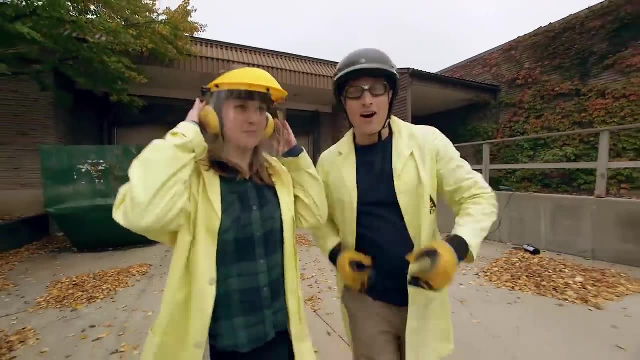 we can fit it all into one of these, A steel tank. This is what we're gonna be using next for our air-powered car. Got it? Yep, All right. So Sarah and I have been hard at work and we've built the air-powered cart. 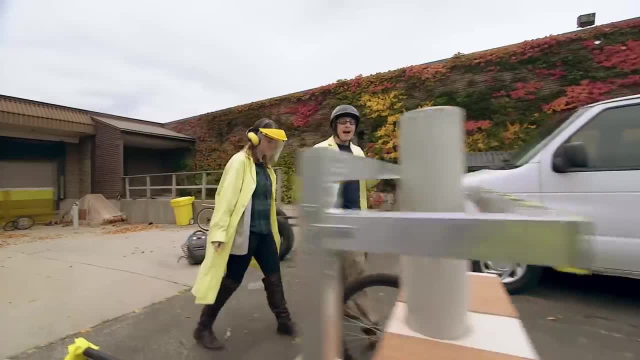 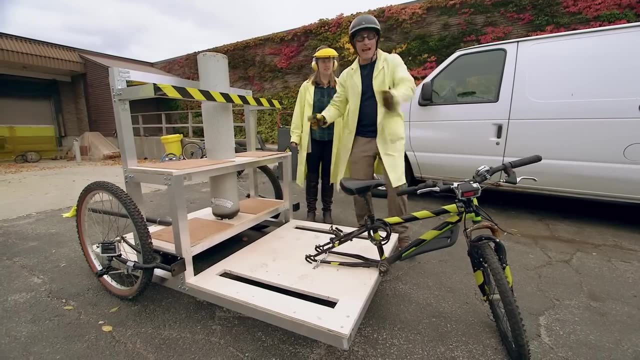 We can't call it a balloon-powered cart anymore, because now we've got a compressed air tank, so it's not a balloon that powers it, Exactly. Okay, so I'm gonna sit on here. Sarah's gonna turn on the tank. 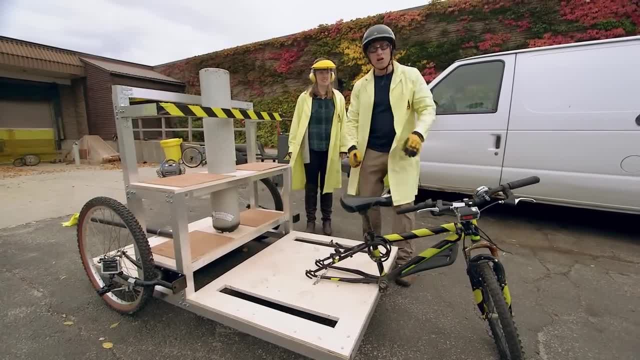 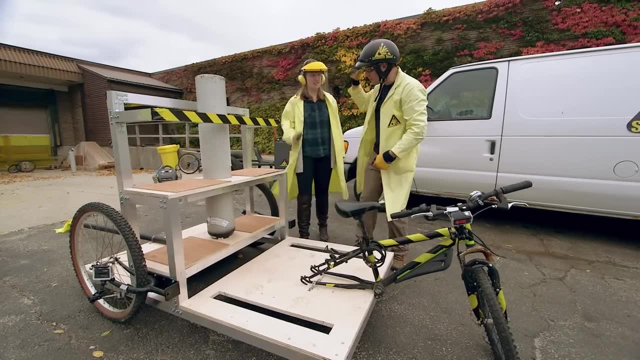 and I'm gonna go. And before we do this, we should say: do not, under any circumstances, try this at home. We are trained professionals. You ready, I'm ready? Okay, high five first. Okay, now we do it. 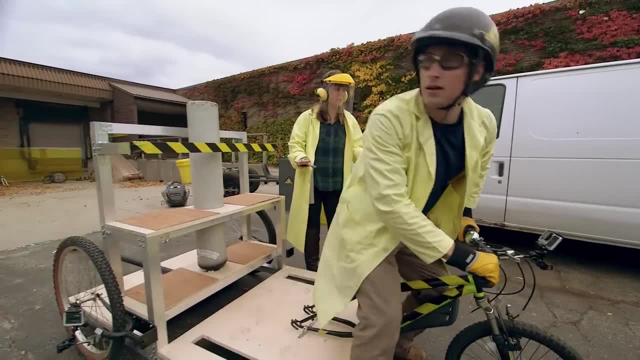 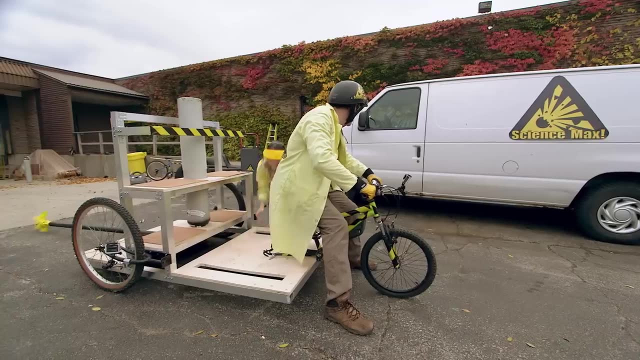 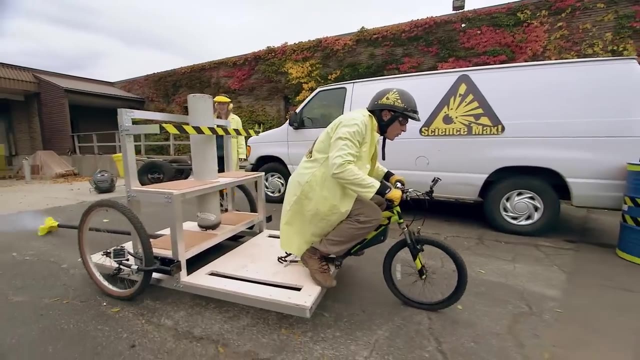 Okay. so before I turn the tank on, make sure your feet are down and the brakes are on. Gotcha, Don't take them off till I say go, You have got it All right Ready, Okay, Woo-hoo. 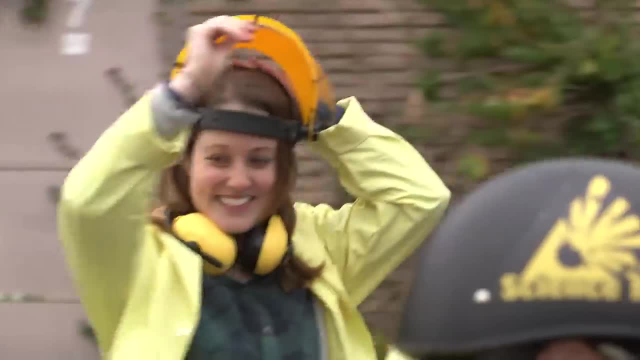 Yeah, It worked. Yeah, it did work, but I feel like it could work better. You wanna go faster? I do wanna go faster. This reminds me of the rock cart. Yeah, But we didn't have a big enough balloon. 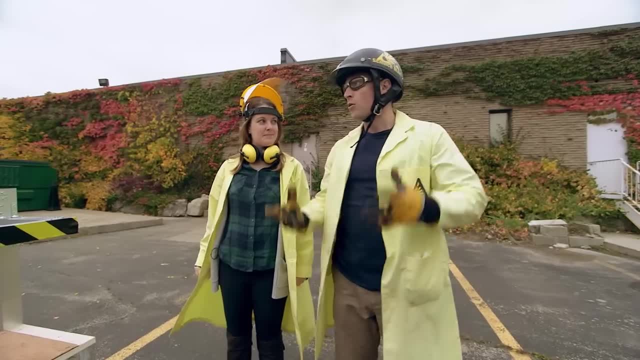 We need more force, We need more force. So should we get a bigger tank? Let's get more tanks, More, More tanks, more force. You're gonna go faster forward. Newton's Third Law. Newton's Third Law, High five. 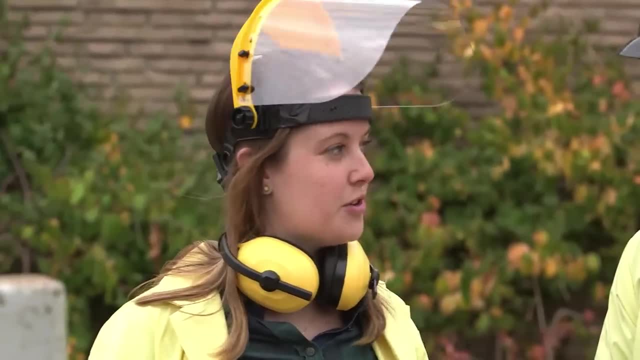 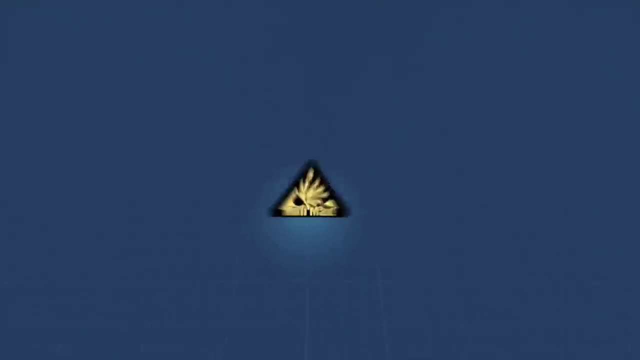 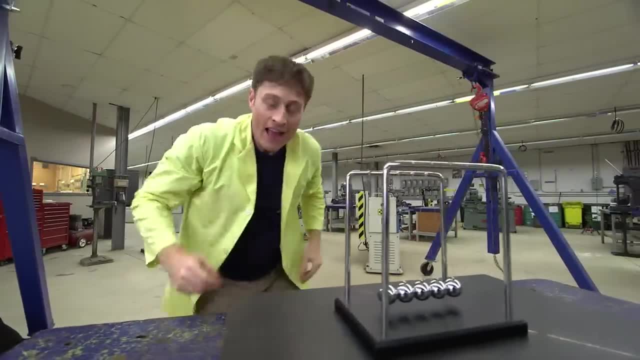 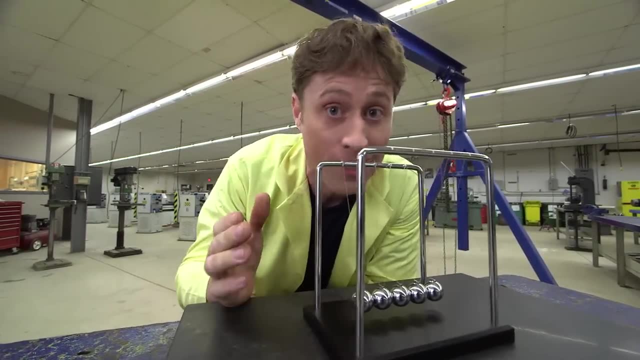 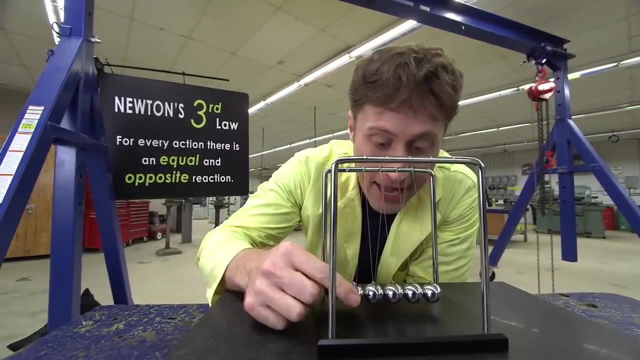 This is Newton's cradle And it's a really cool toy that demonstrates all kinds of laws of motion, including Newton's Third Law. What you do is you pull this one ball out and when it hits these balls, they exert force on that ball to make it stop moving, but it exerts force on these balls, which travels. 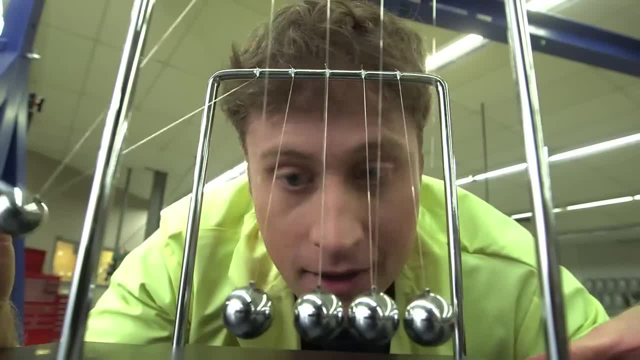 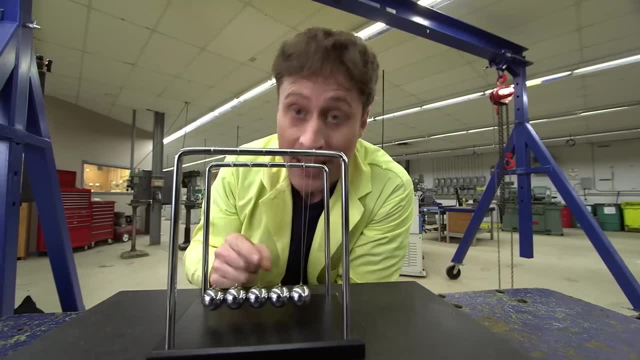 through the ball and makes this one amazing. In the end fly out like that. Now, there's a lot going on here, but you can really see how the force is equal that you put in and you get out if you use two balls. 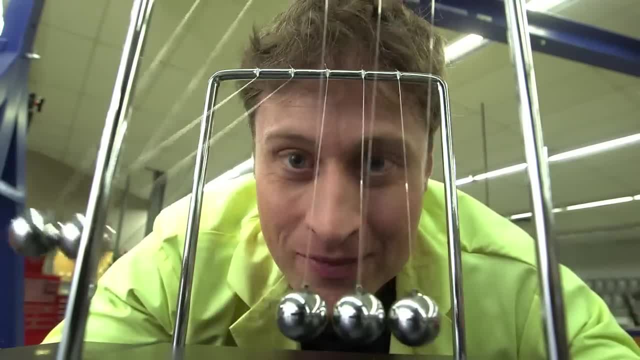 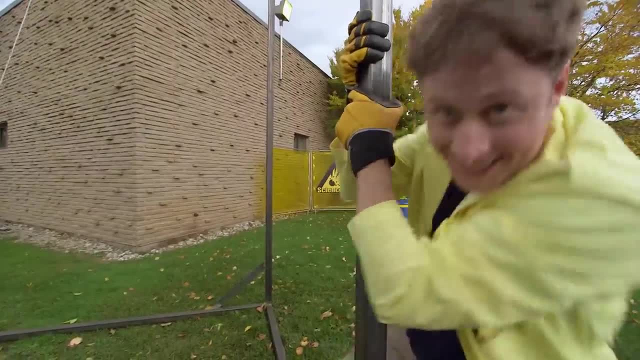 I swing two balls up and two balls go out. that side Isn't that cool. Now, it wouldn't be science max, unless we maxed it out. so come on, Whoa, okay, This is one we built out of bowling balls. 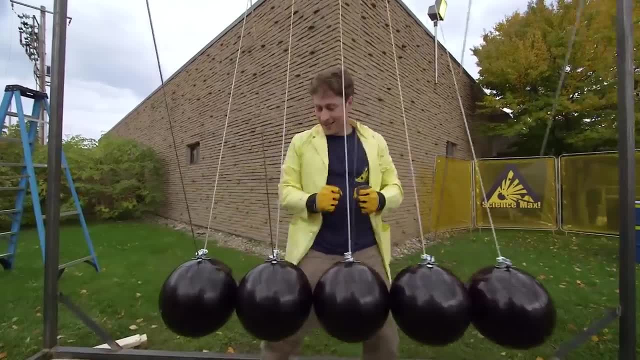 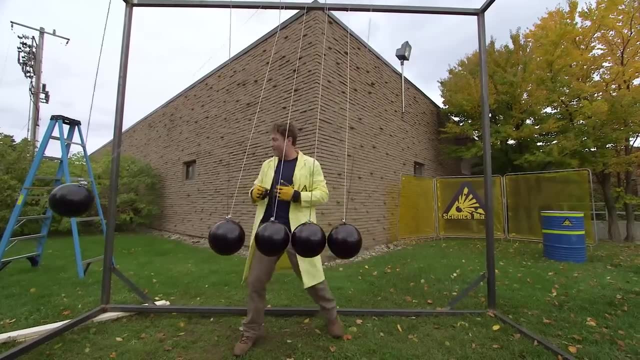 Bowling balls. bowling balls instead of smaller balls, And I think it's gonna work the same way. Let's find out. You throw one out and and ha ha, Yeah, it works the same. Okay, now let's try it with two balls. 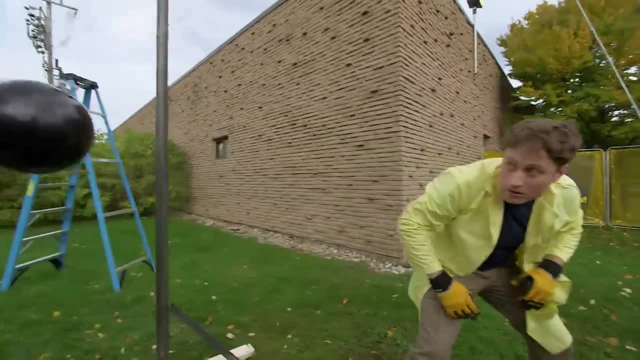 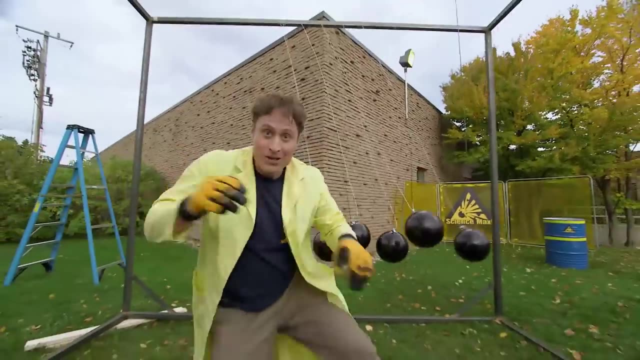 Okay, ready, Wait, wait, wait, wait. And two balls throw them out, And two balls on that side. All right, so there you have it. Whoa, Newton's Third Law. Oh, Ah, Newton's Third Law. 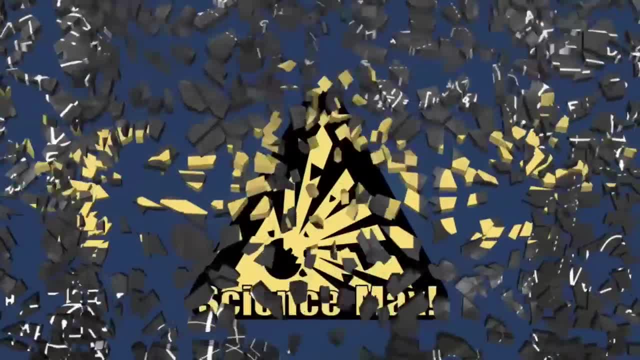 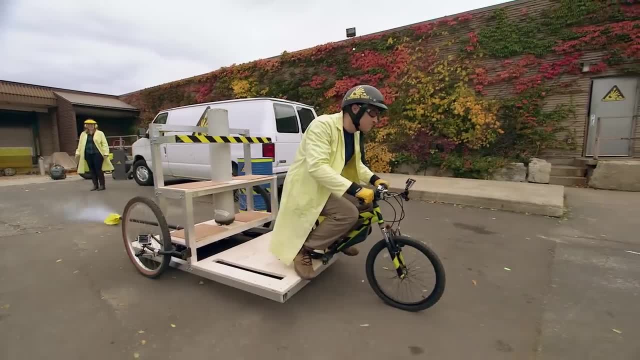 For every action there is an equal and opposite reaction. So our single pressurized tank created enough force to move me, but not very fast. The plan now is to do two things. First, we're going to triple the amount of thrust. 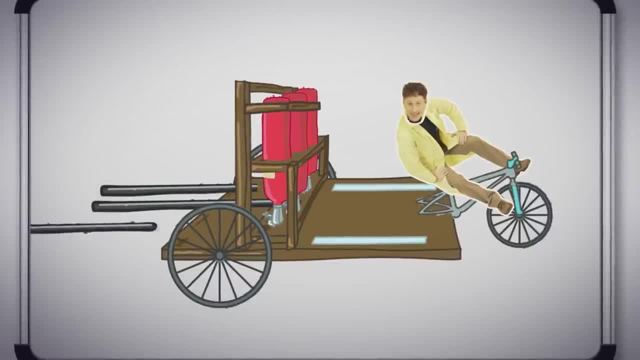 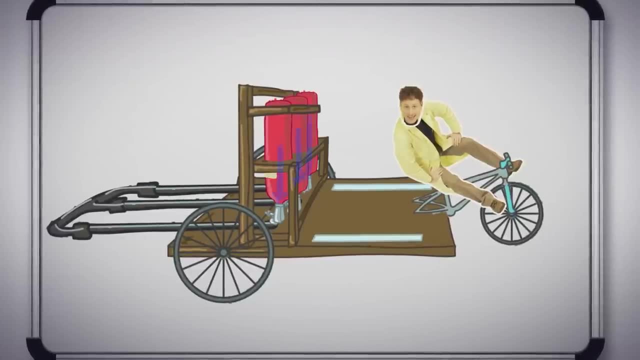 by using three tanks. We're also gonna use some pipes that lock into each other. to give me an initial push, These pipes slide together and when the air is turned on, the pressure in the pipes will cause them to slide apart, which will push me forward. 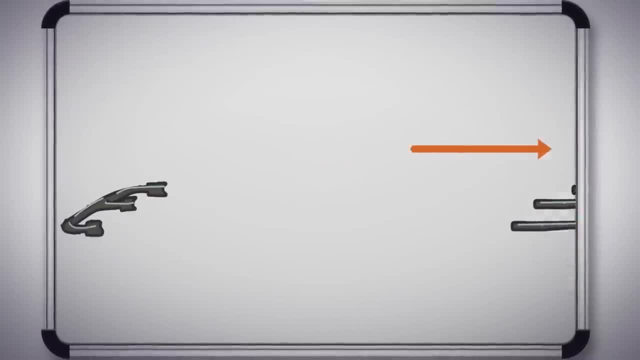 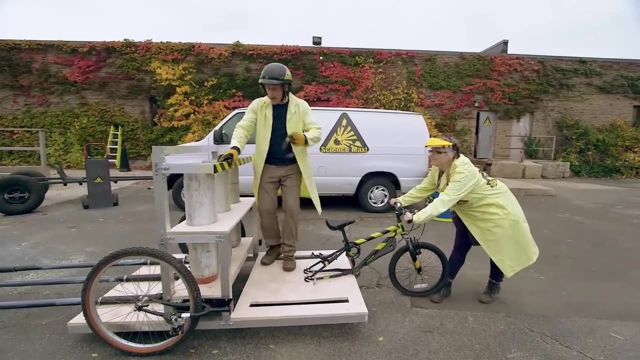 After that, I use what's left- left in the tanks to keep going. All right. now it's time to max it out. I've enlisted the help of a few more Science Max people. Thank you very much, Corey. You'll see. now we have three tanks of compressed gas. 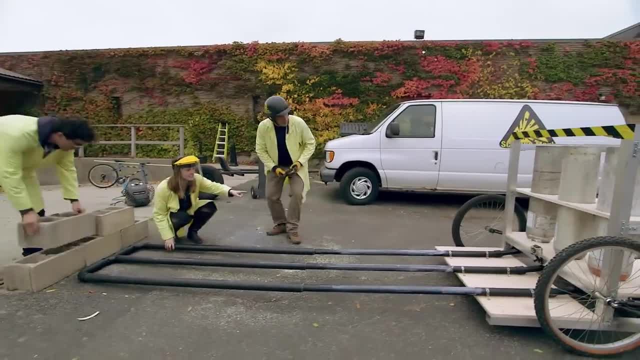 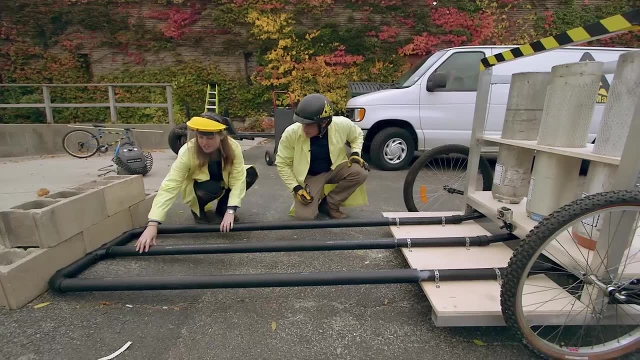 and we've also got this nifty little contraption. How does this work, Sarah? All right, so each tank is attached to a tube and you can see that each tube goes into this one main tube. so when we turn them on, pressure's gonna build up. 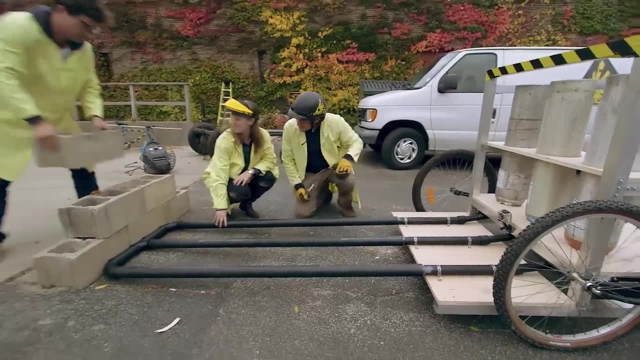 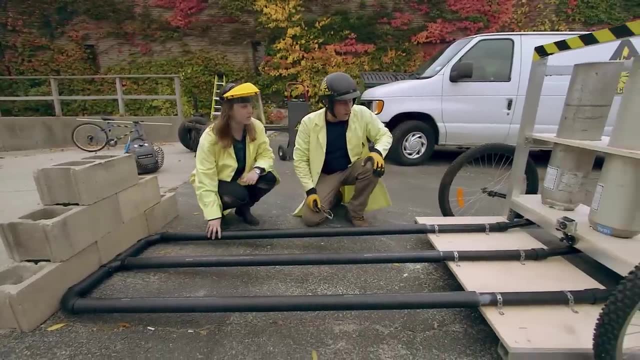 and we're gonna go forward with more force. Well, that's great. and Reid is stacking cinder blocks. Thanks, Reid Up. so that will push. the pipe will push against the cinder blocks, and then I'll go that way. 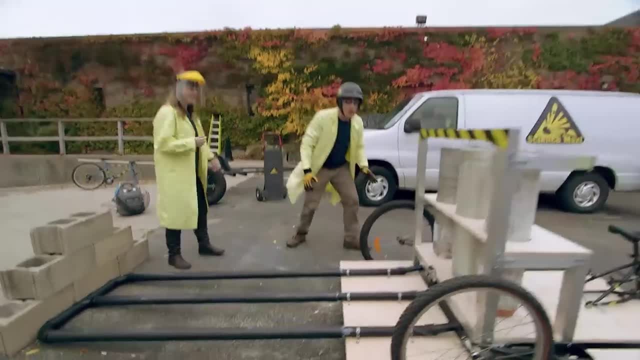 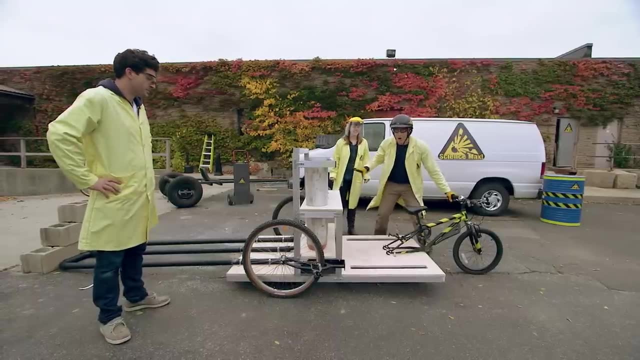 All right. well, are you guys ready? I'm ready. All right, let's do it. Now. again, I have to say thank you, Corey, I've got it. This is something you definitely don't wanna try at home. 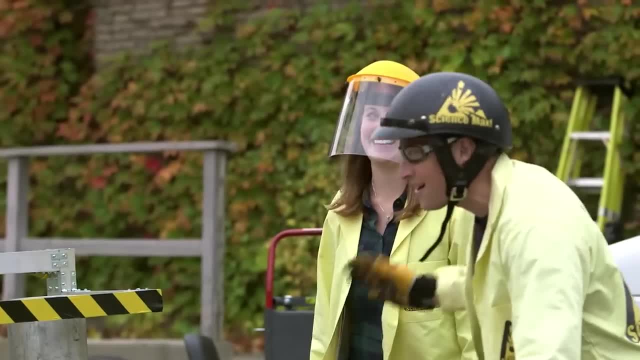 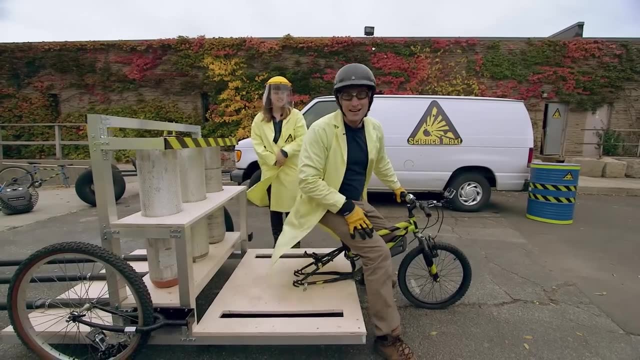 We are all trained professionals. We have a physics degree here. We've got TV people that make sure that this is safe, so watch it and enjoy, but please don't try any of this at home. Okay, I'm ready. Sarah, count me down. 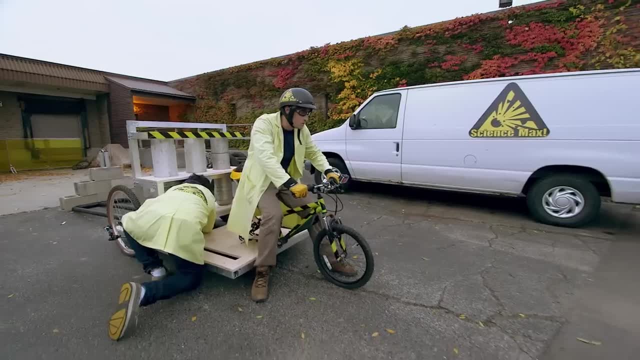 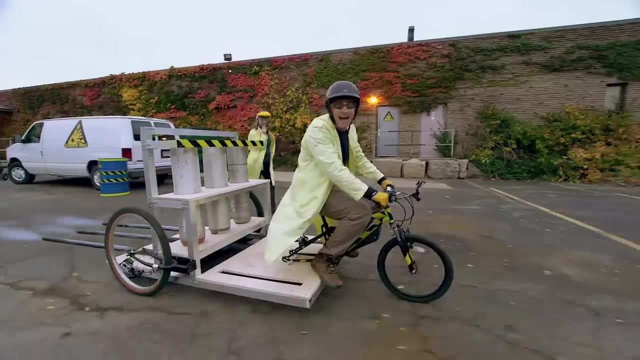 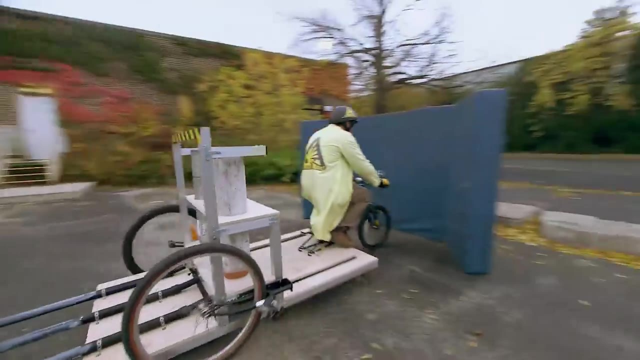 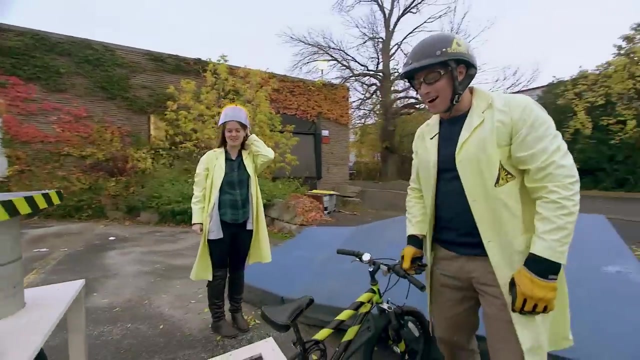 Three, two, one. Yeah, Whoo, Uh-oh, uh-oh, uh-oh, Uh-oh, Whoo-hoo-hoo-hoo. That was awesome. That was really awesome. All right, high-fives, high-fives. 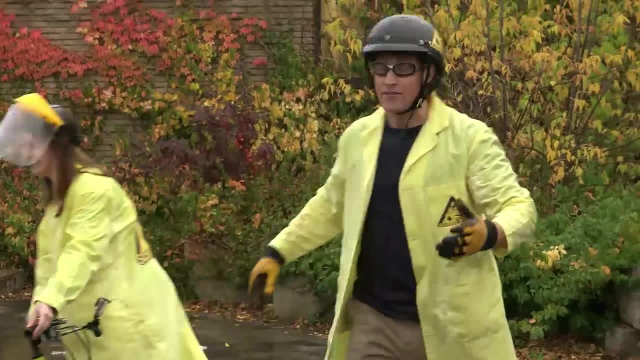 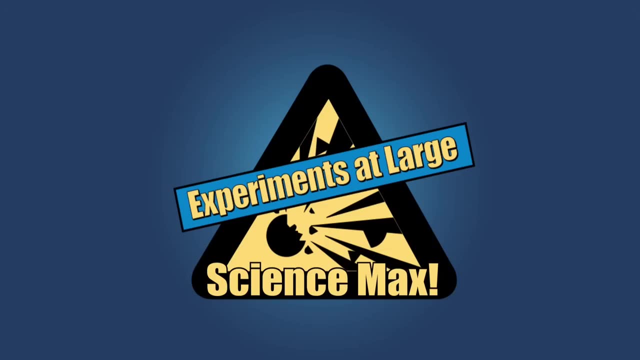 Yeah, yeah, And it's raining now, so it looks like we're gonna have to stop. so thank you very much for joining us on Science Max- Experiments At Large in our episode on Newton's Third Law. Science Max Three, two, one. 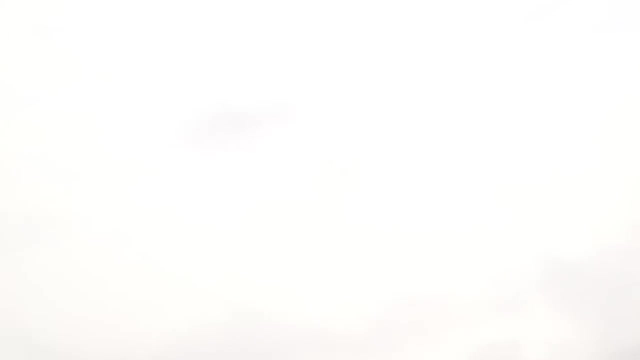 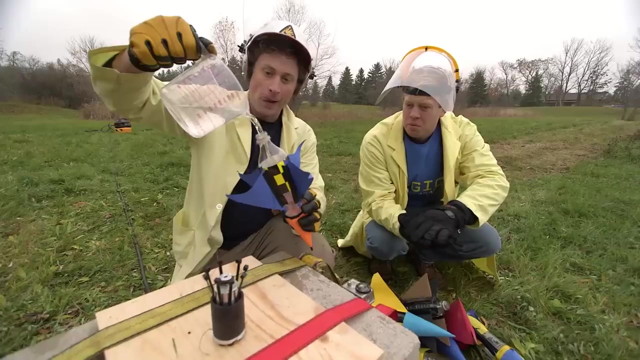 We're really under pressure during this episode of Science. Max, Compressing a gas till it's pressurized is how we can do this and this and, to a lesser degree, this Help. I'm being crushed by all this pressure. 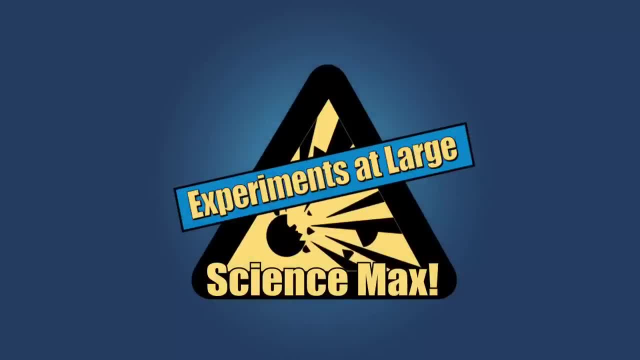 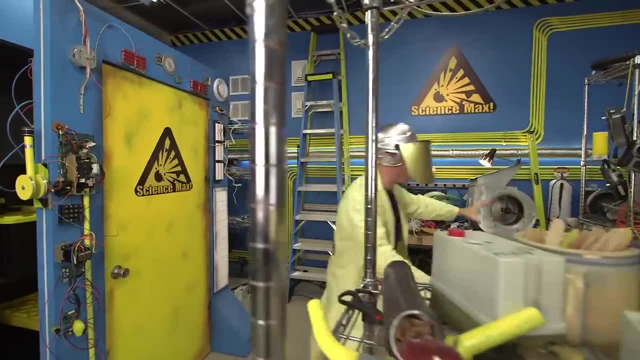 Pressure today on Science, Max, Science, Max, Experiments At Large. Phil to Mission Control. Come in. Mission Control. Psh. Uh, this is Mission Control Phil. Uh, we read you loud and clear: Psh. I would. 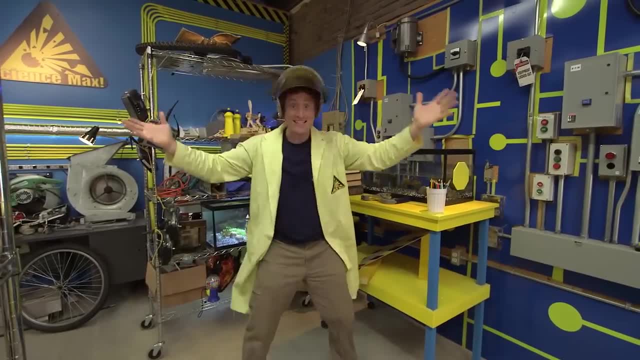 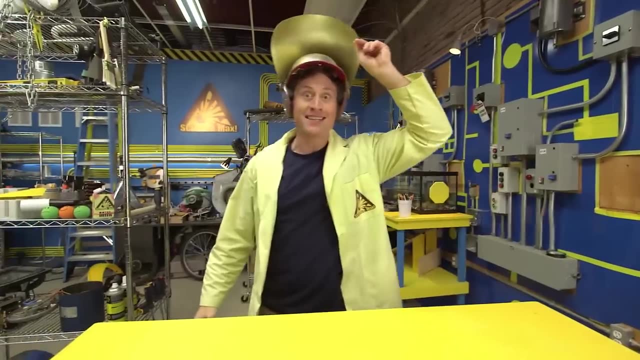 Oh, Greet, Greetings, Science, Greetings Sci. Greetings, Science Maximites. Welcome to Science. Max Experiments At Large. My name is Phil McCordick and today we're gonna be building an air-powered rocket. 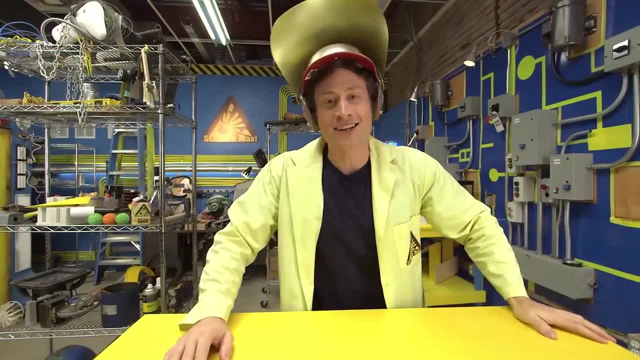 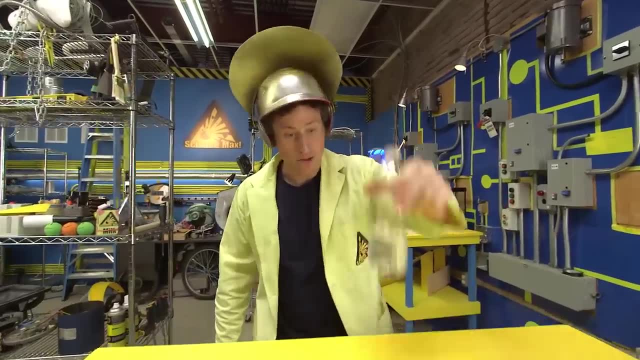 Too difficult. you say Nonsense. It's easy. It's not like it's rocket science. Hey, it is rocket science. Cool. Here's what you need. You need a bottle and a cork. Make sure that the cork fits nicely into the bottle. 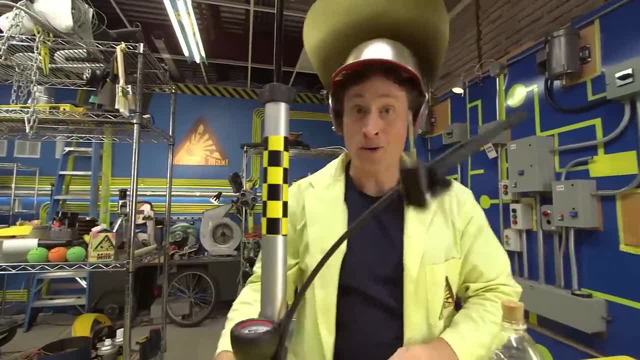 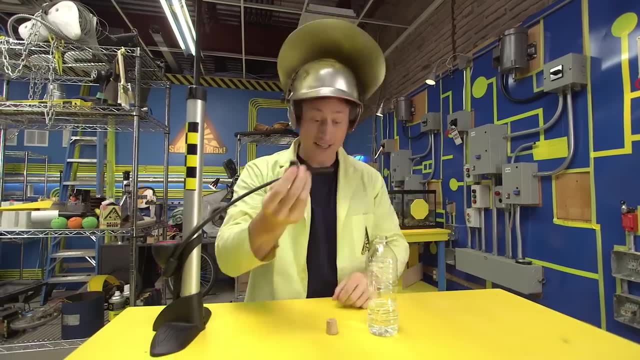 and then you need an air pump, because you can't have an air-powered rocket without air. And on this air pump you need a pin, the special kind that you use to inflate basketballs or volleyballs or stuff like that. Now, what you want to do is push the pin through the cork. 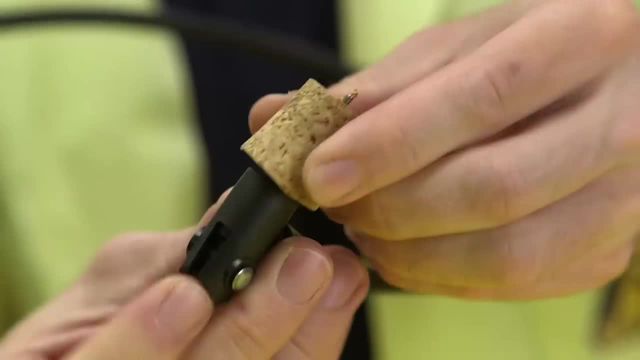 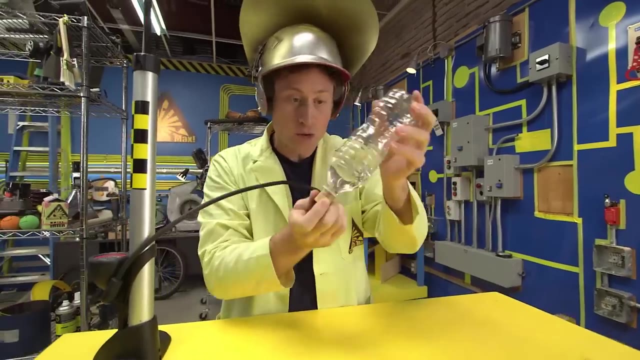 You might want an adult's help for this. Push it through until it goes through on the other side and then make sure you get a good seal with the bottle. Now you're ready to launch your rocket with air pressure, But first let's do a few other things. 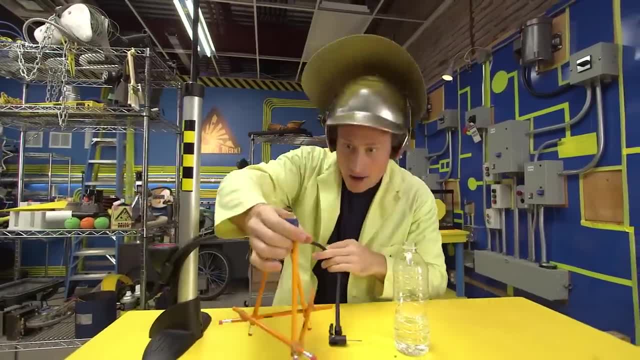 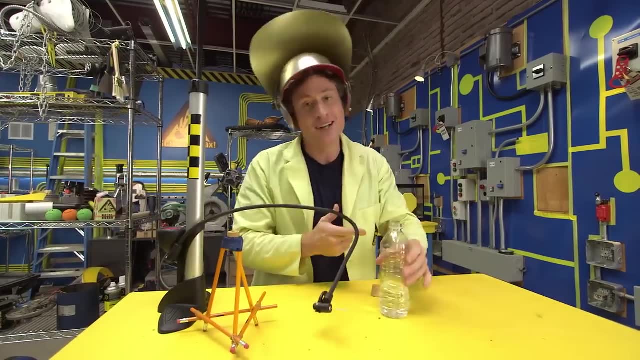 Take your cork and put it in a tripod launcher. You can make this out of pencils or anything you want, as long as it stands up nice and solidly. And then, of course, you want to decorate your bottle so it looks like a rocket. 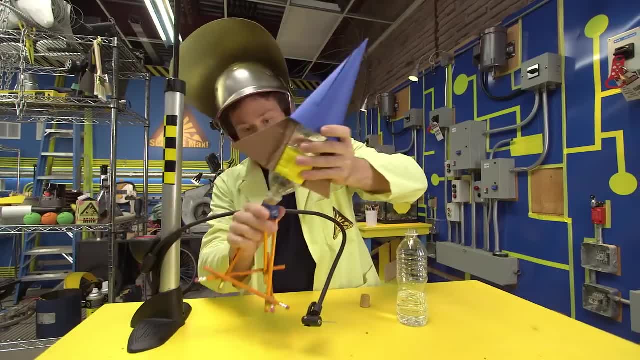 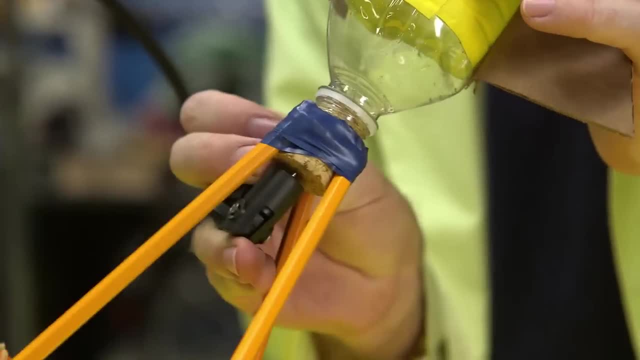 This is my rocket. Pretty good, right. So stick the bottle on the cork like before, like that, And then you stick the pin in the bottom, And what we're going to do is we're going to inflate the bottle with air pressure and then it's going to launch. 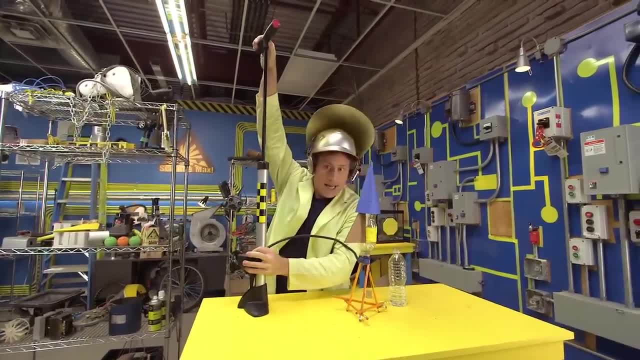 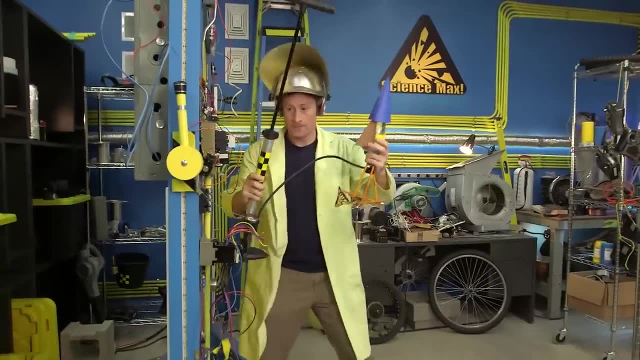 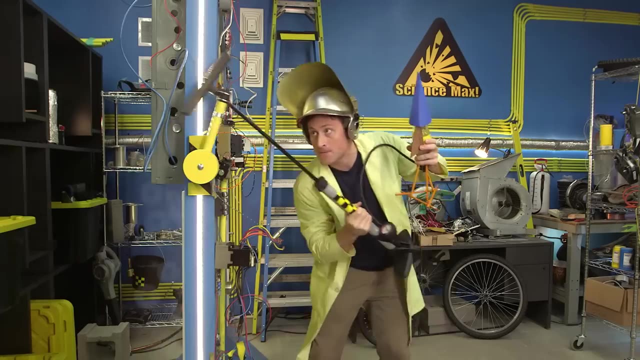 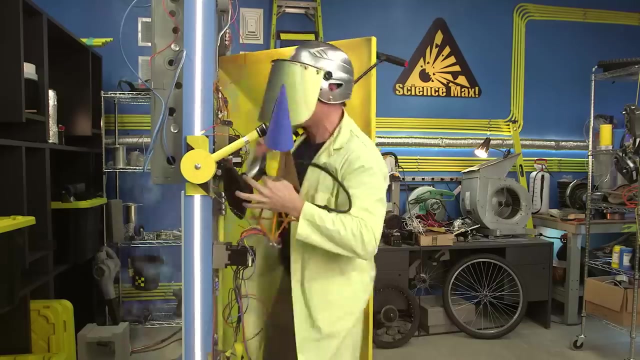 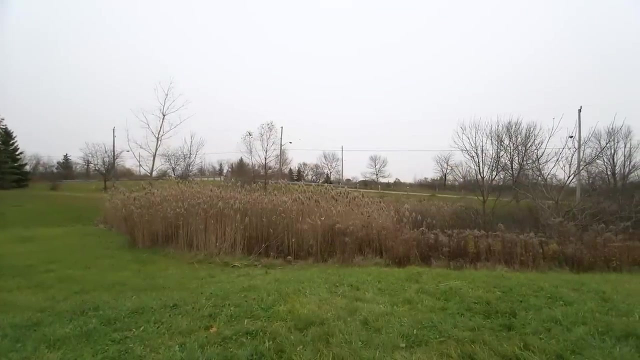 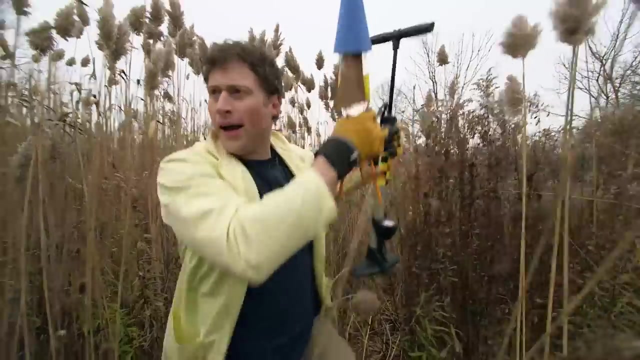 Okay, here we go. You know, rocketry really isn't something you should do indoors. Come on, Hey, this was supposed to be a field. What's going? Why are there? Oh, it's in my shoe, Huh. 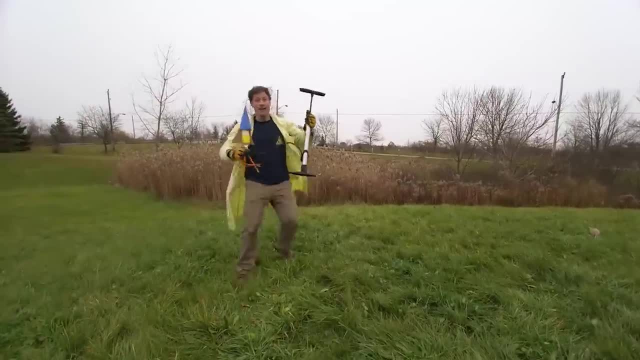 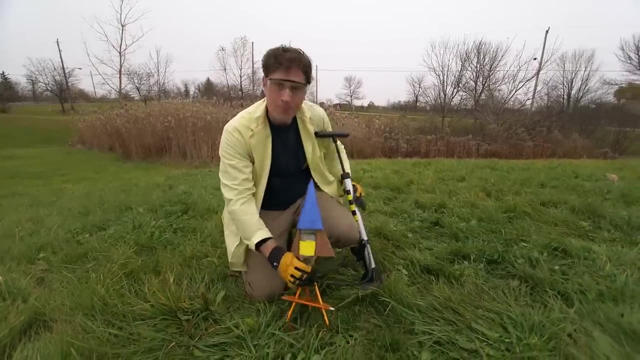 Oh, Oh, this will do nicely, Ha-ha. Don't forget to do this with an adult and don't forget your safety glasses. Now set up the rocket in a nice big open area and make sure it's pointed away from you. 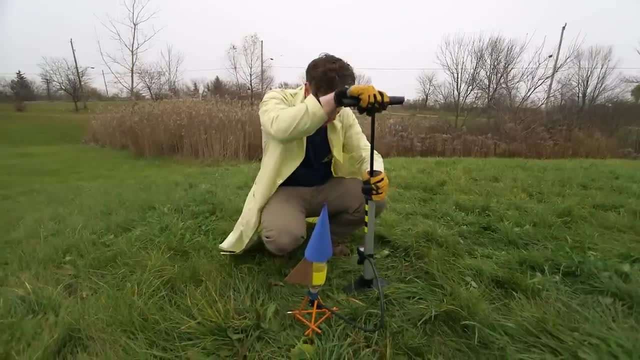 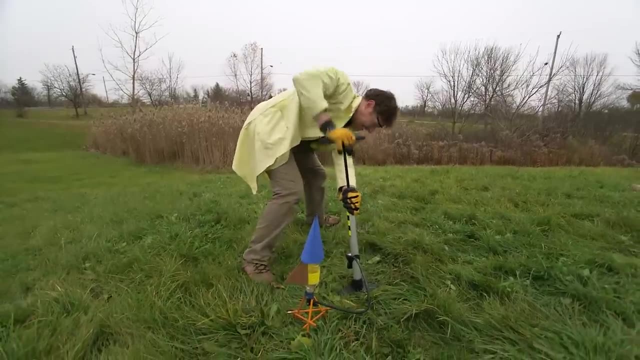 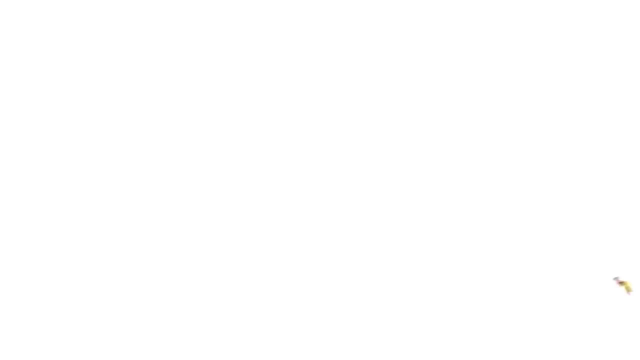 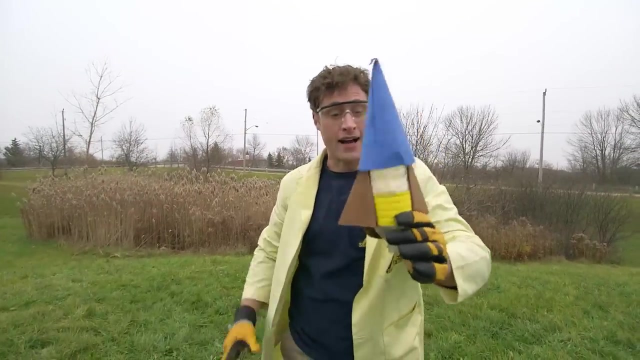 And then what you do is you pump the air pump And it puts air into the rocket, which pushes down on the water, which will push down on the cork until eventually. So be science maximites and come up with your own rocket design. 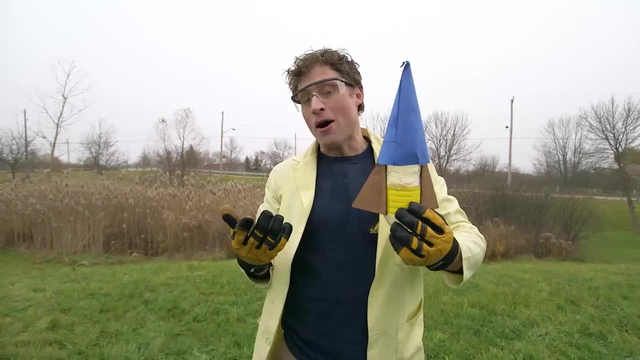 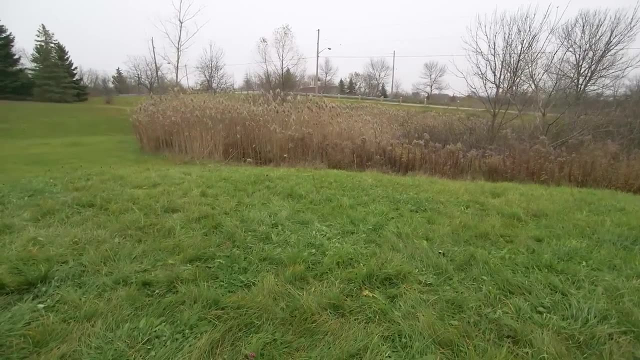 Try different amounts of water, different fins, even a different sized bottle. Try it for yourself and see if you can get one that goes higher than mine just did. How did I get in? I think it was this way. Do you want step-by-step directions? 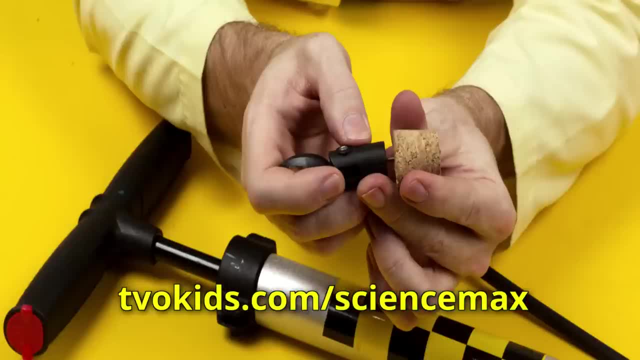 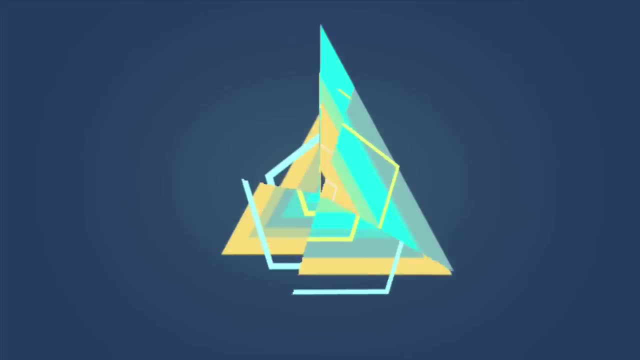 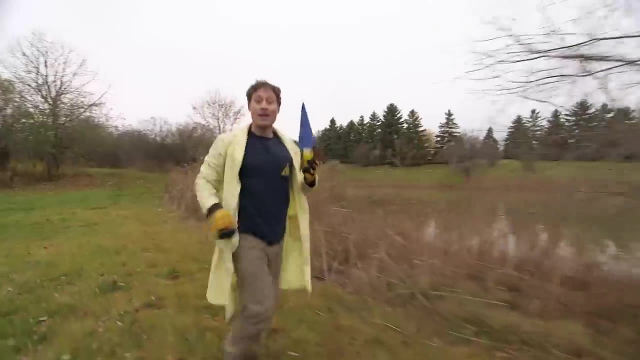 on how to build your own air-powered rocket. Well, don't worry, Everything you need is on our website All right. Now it is time to max out our air-powered rocket. I've got Adam here. Hey Adam, Hey Phil. 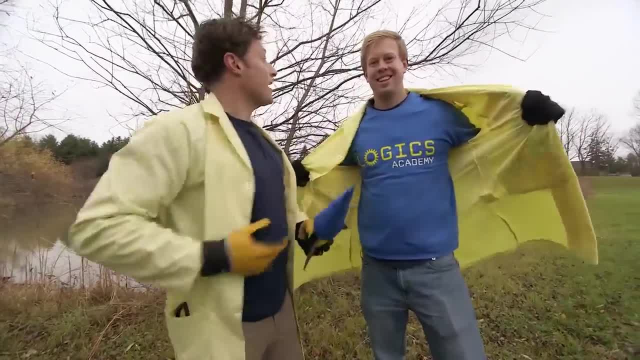 How you doing Good, how are you Good? Adam's from Logix Academy, Logix Academy And you guys go into schools and talk about science. We do Fantastic. Do you guys do an air-powered rocket? Yes, exactly. 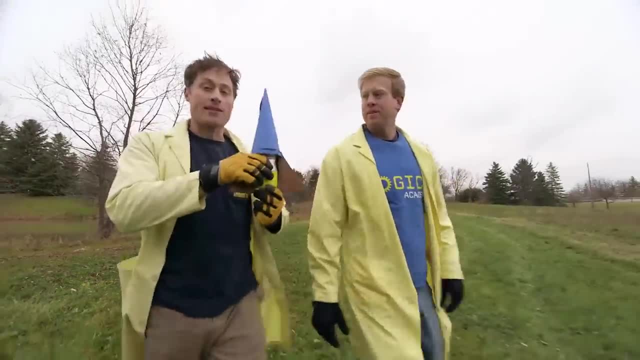 Does it look like this one? It looks exactly like that. Oh, that's great. So how do we max this out? So we want to add more pressure to this bottle and try to get it to launch a little bit higher. More air. 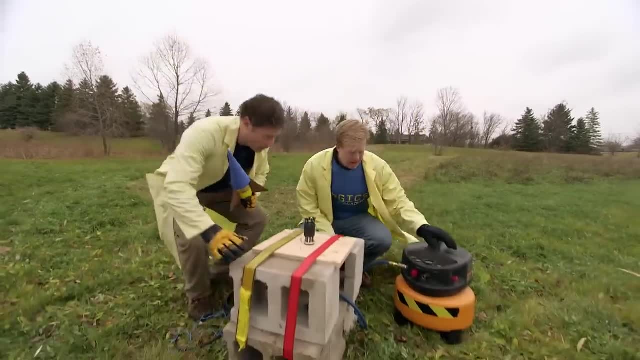 More air, Great. So what do we do? So we're going to use one of these- Ooh, It's an air compressor, Right, which works a lot like the bike pump, right? Yeah, exactly Cool. So we're going to have compressed air coming from here. 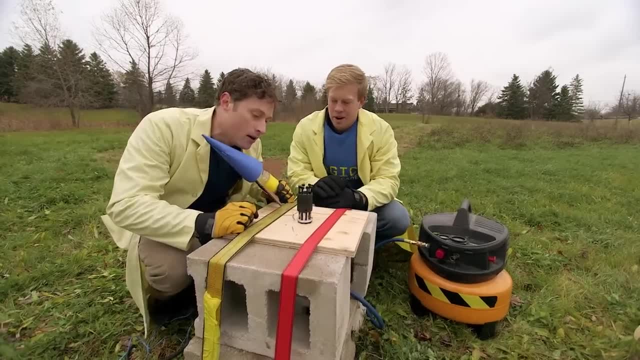 through this tube into underneath here, Yep, And out that nozzle there And you're going to put your bottle on top And out the nozzle into the bottle, like that, Yep. And now we want to be able to hold it in place. 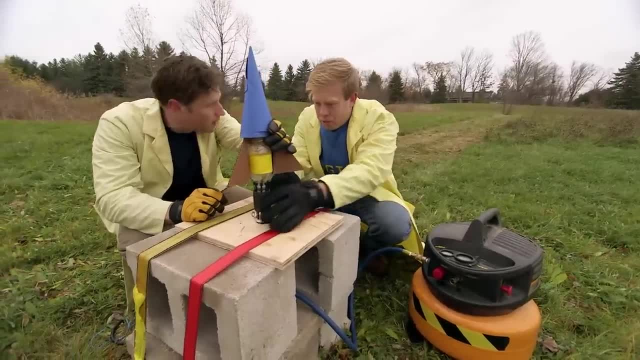 So we're going to have these little fingers here that are actually going to work to hold it until we want to let it go. So we're going to lock it in place. Oh yeah, Look at that. Totally locked, Exactly. And then what? 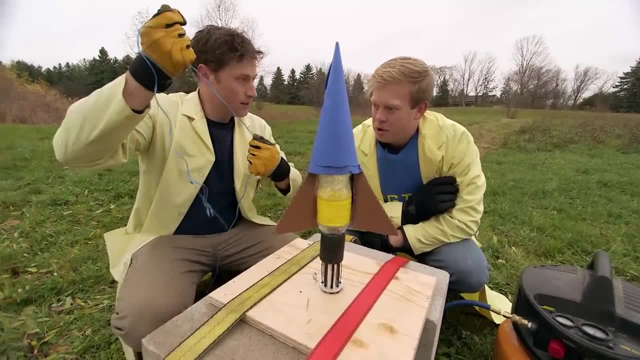 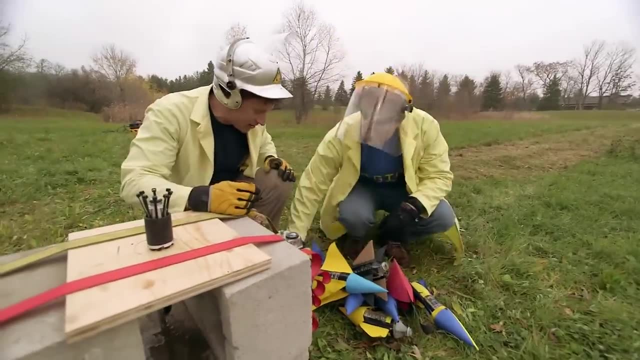 How do we launch it Now? you're going to take this cord and go a safe distance away and we are going to pull it, And then we would pull it. Which one do you want to start with? I think we should use this one here. 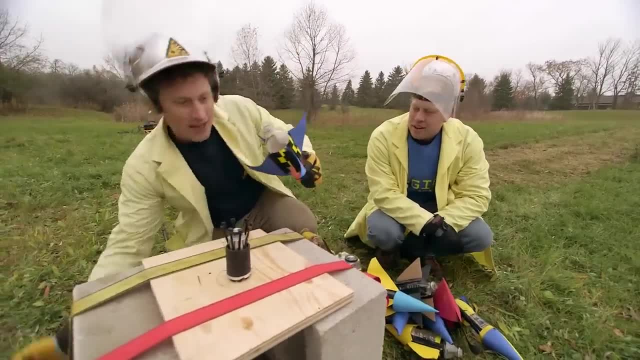 Okay, great, Now we put water in it, right? Yep, You're going to put water in there. Why do we use water? So the water is going to act to push the rocket up into the air. The air is going to. 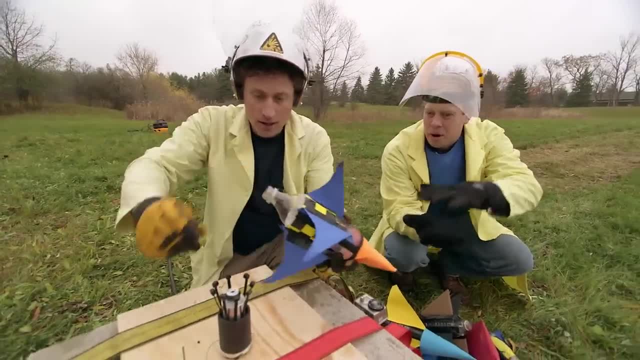 The compressed air in here is going to shoot the water out the back, Uh-huh, And the water is going to push on the rocket and make it launch. It's just to give it a push. Give it a little extra push. How do I get it on there? 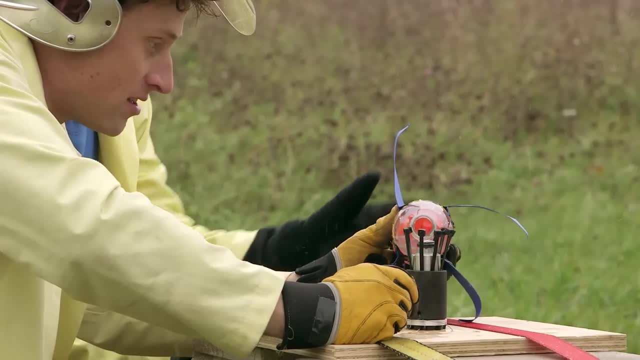 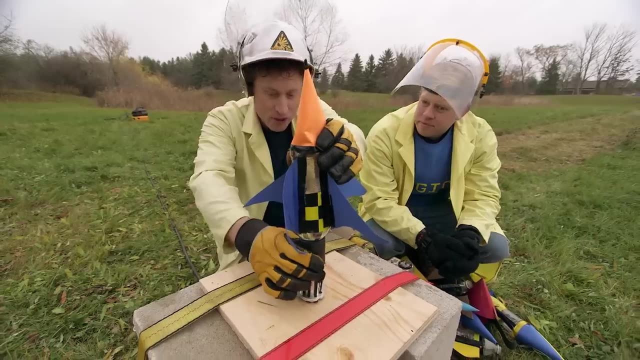 without spilling any water. So just rest it next to the launch there. Just go fast, Yeah, just go really fast. There you go, There we go Just a little bit And then Lock it in place. Locking it in place. 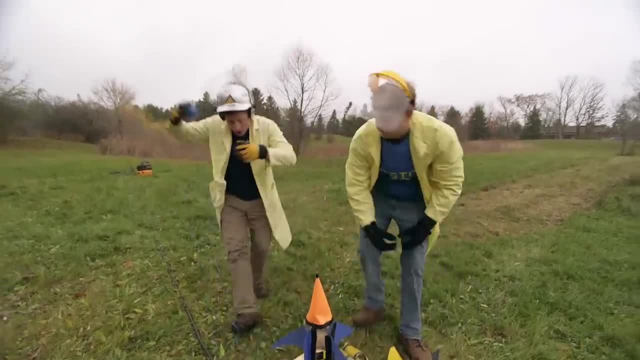 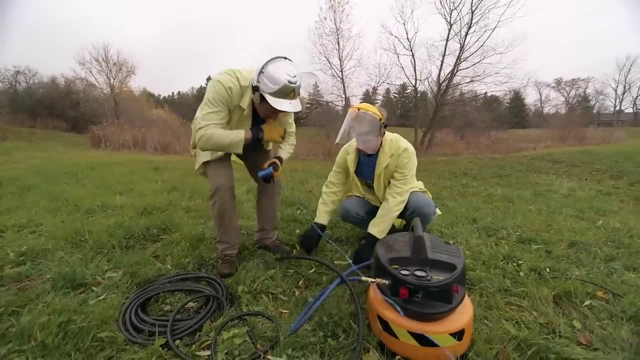 There's no air pressure in the hose yet, right? Not yet no. First we have to spool out the launch cord, So the air compressor has the compressed air in it. It's ready to go. Yep, It's all ready to go. 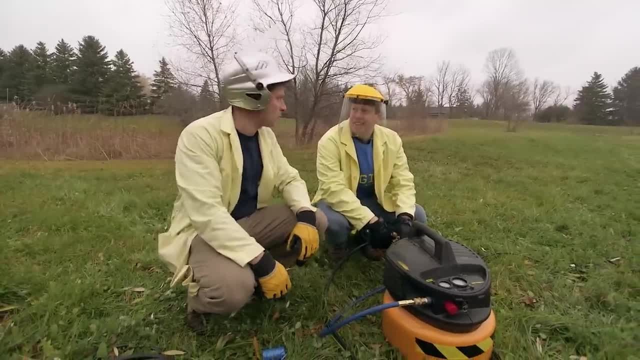 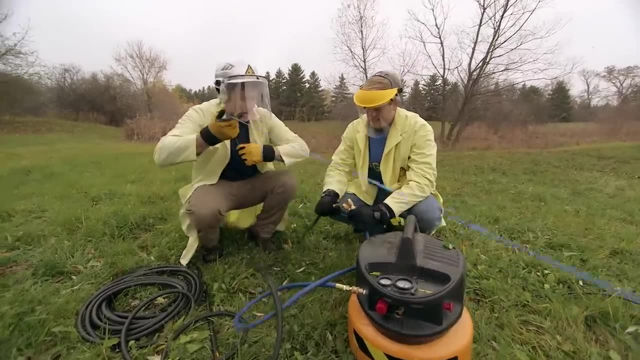 We just need to connect the hoses. Adam, I've noticed it's snowing a little bit. Do you think that's any reason why we should stop? I don't think so. Science must go on. Blast shields down, Connecting hoses. 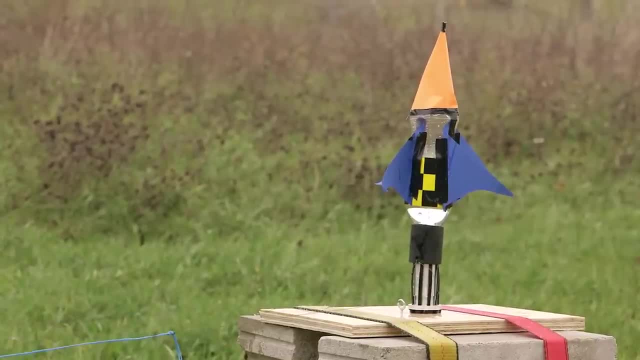 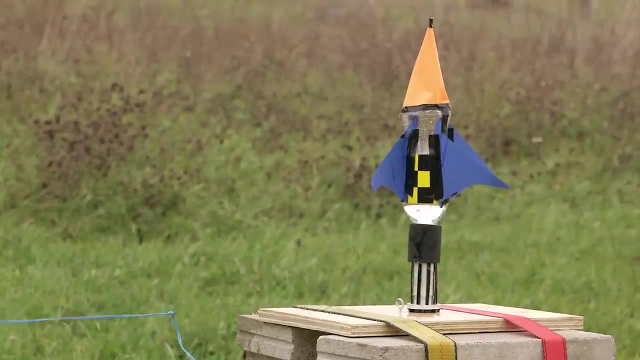 When we connect the air hose, the pressure from the compressor travels down the line and into the bottle. You can see the bubbles of air going in. Those bubbles are carrying more air into the bottle, giving it more pressure. Here we go: Three, two, one. 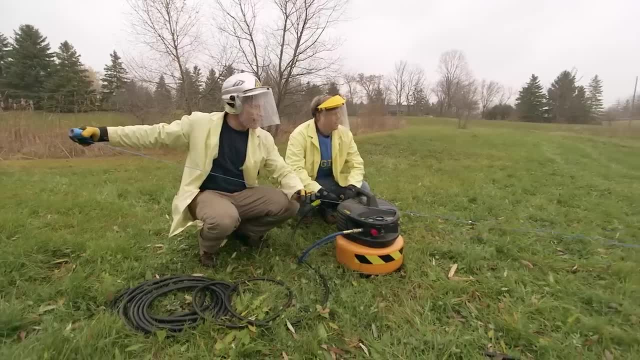 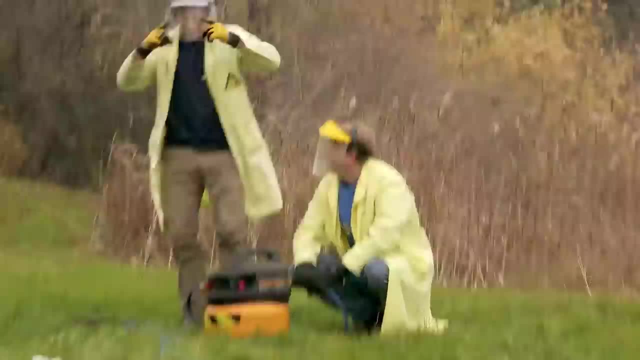 All right, And the rocket's going, Let's do it again. Launch it in three, two, one, Whoo Nice, Success, Success, Nice. So small bottle Worked really well. How do we make it bigger? 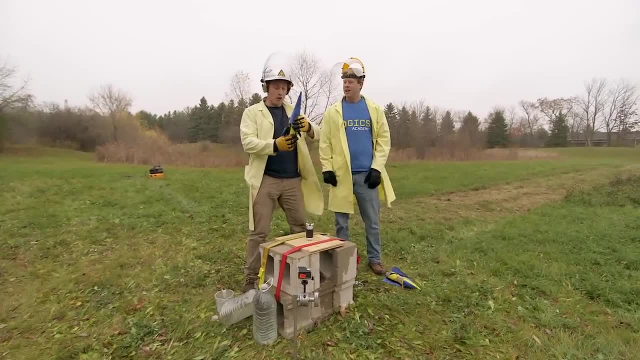 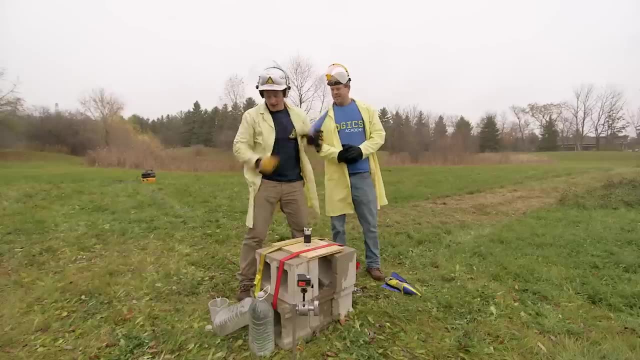 I know A bigger nose cone, I think a bigger bottle, Oh, a bigger bottle. Yeah, of course That's easy. How about this empty water bottle that we have now? That might work, except that the top here is too big. 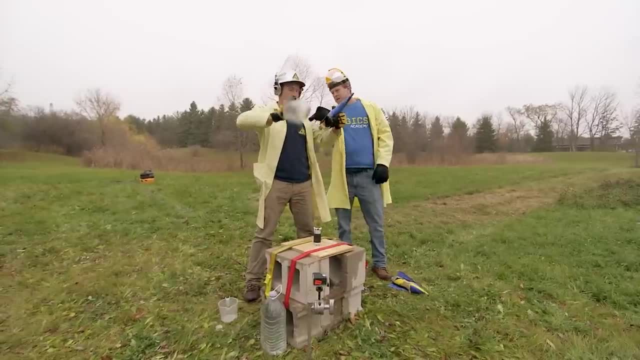 I don't think it'll fit on our launcher. Oh yeah, So what? should we use A two-litre pop bottle? Oh yeah, That's a good idea. Yeah, A two-litre pop bottle might work a bit better. 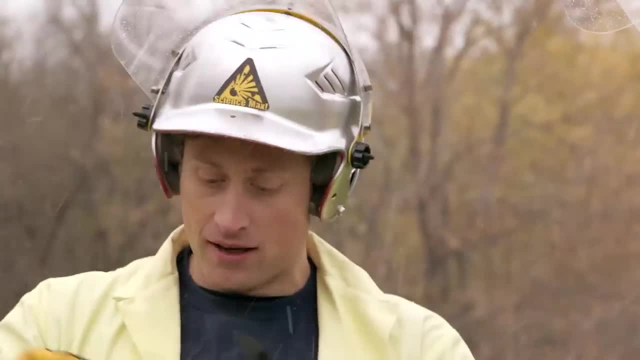 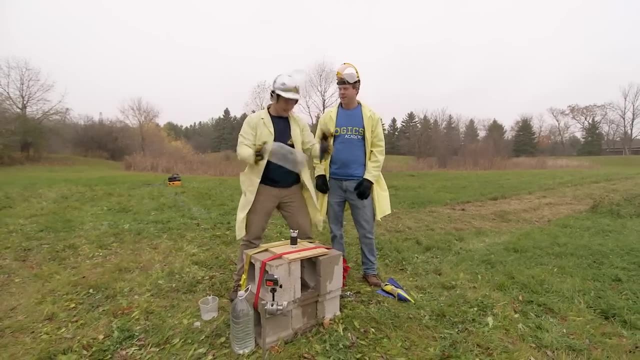 because it'll be about the same size. Oh, that's right. Two-litre pop bottles have the same opening as these small water bottles, Exactly, That's great. All right, Let's make a couple rockets out of two-litre pop bottles. 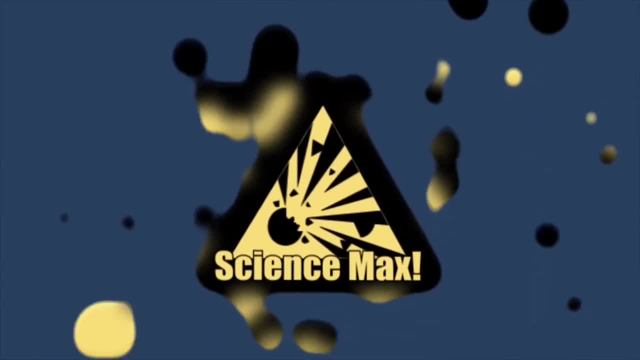 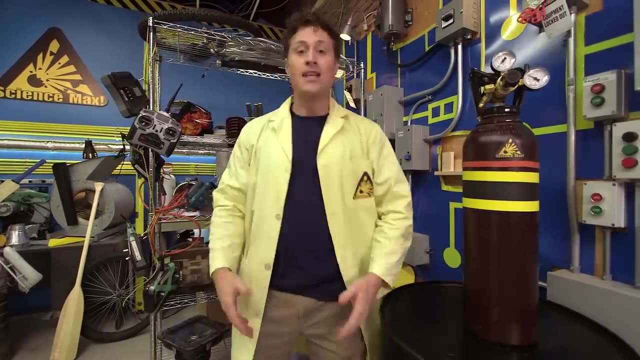 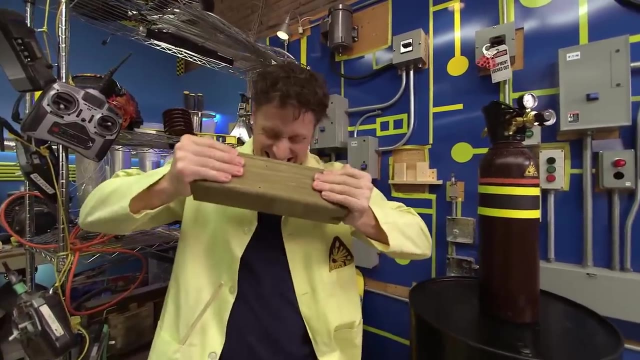 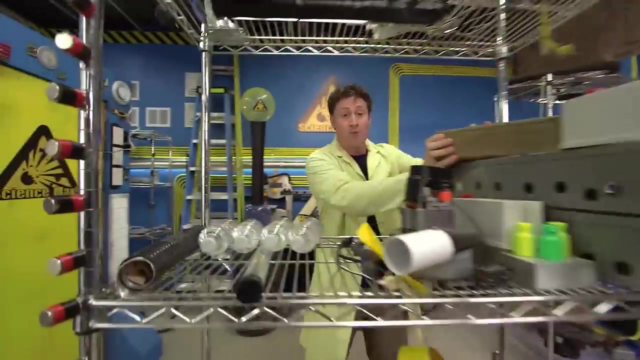 Awesome Pressure happens when you squeeze something or compress it. Solids do not compress very well. I will demonstrate. Solid, Is it compressing? No, Okay, Liquids don't compress very well either. You can demonstrate this for yourself by getting a plastic. 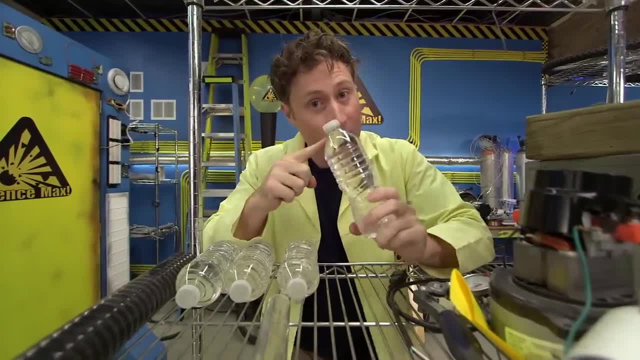 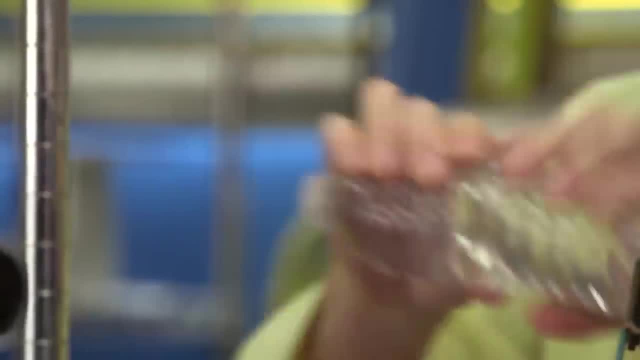 water bottle and filling it right to the very top with water and putting on the cap and squeezing, You'll find that you can't really squeeze the bottle very much. But if you empty out half of the water, No, Don't pour it on the floor. 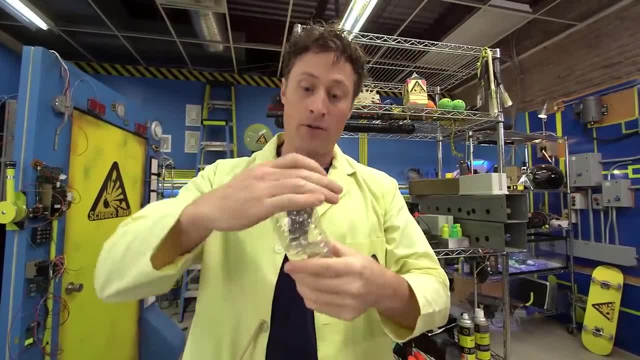 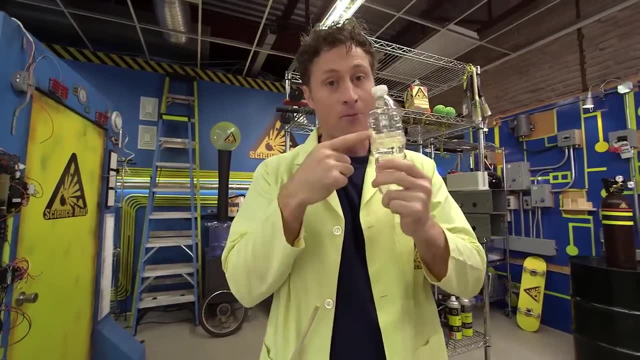 And then put the cap back on the bottle and try to squeeze it. you'll find that the water will come out. You'll find that you can squeeze it a lot more. That's because gases compress much easier than solids or liquids. Here's what's going on. 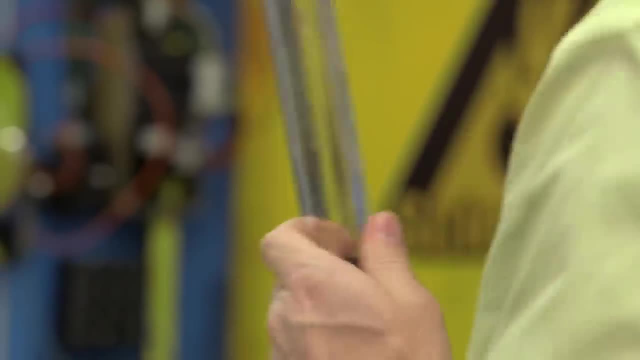 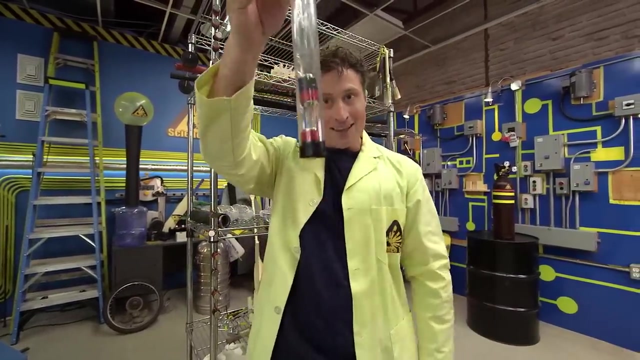 Say, this container is well, any container, And these magnets are air molecules. Now I'm going to put the magnets in pole to pole, so they repel each other and want to stay a certain distance apart, just like air molecules do. There we go. 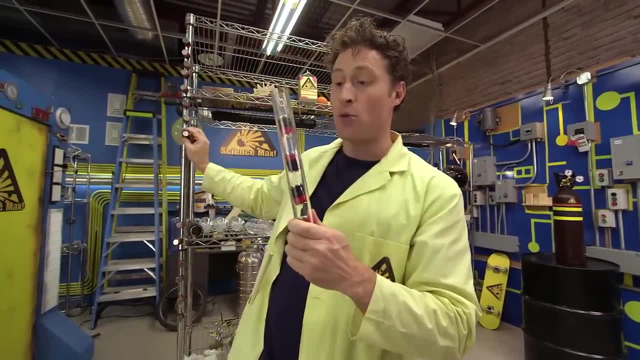 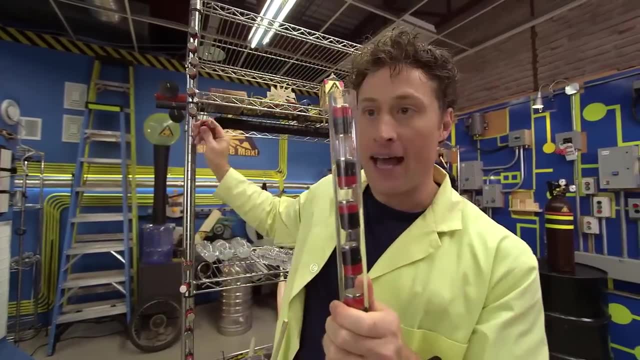 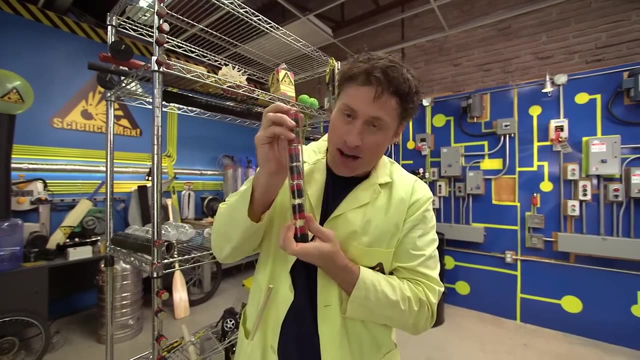 A container at normal gas pressure. Now watch what happens when I add more gas molecules. They start to get squeezed together, And if I add more, the amount of space that each one gets is less and less. Now this container is under a lot of pressure. 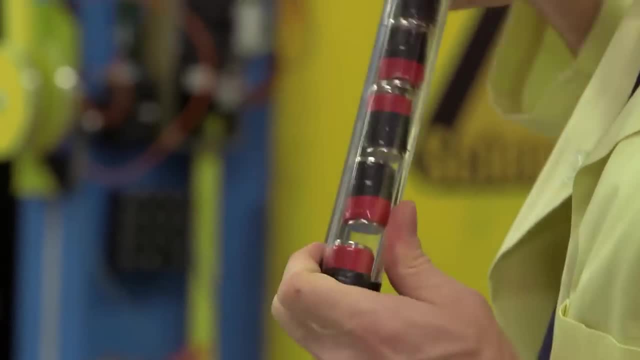 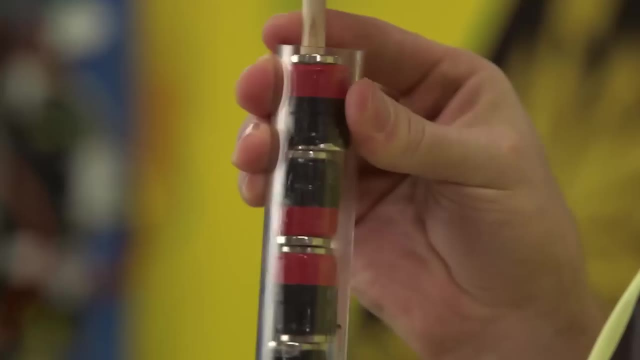 These molecules really want to escape through the top of the container but they can't because I'm holding them down. If I took something like this plunger and I pushed them down even more now they're really under pressure. They want to get out. 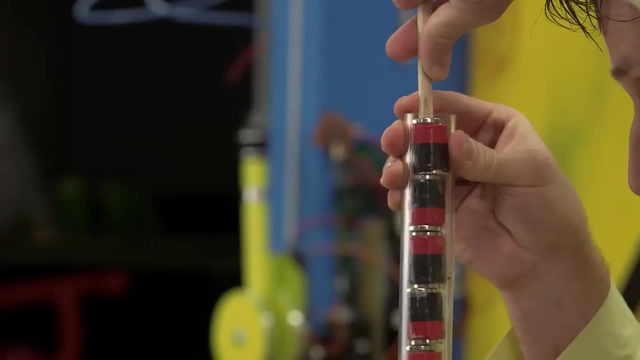 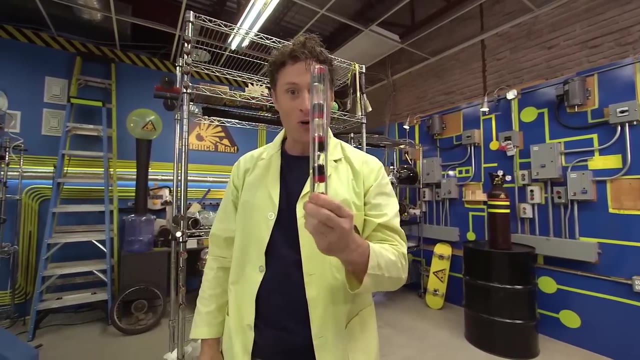 but they can't because I'm holding them in Now. watch what happens when I let them go. They all pop out the top and the container has returned to normal gas pressure. That's what happens when we put gas in a container like this one. 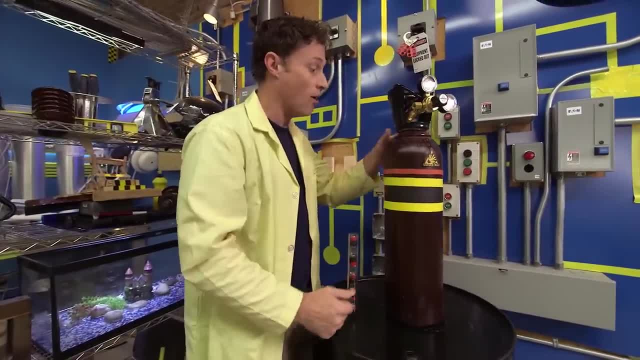 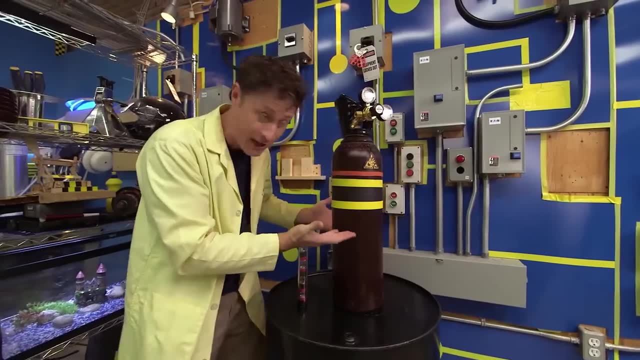 These containers that hold compressed gas are made out of solid steel because you need something really strong or it might explode if you put too much gas pressure in it. That's why these are only filled up by professionals who know exactly how much pressure it can take. 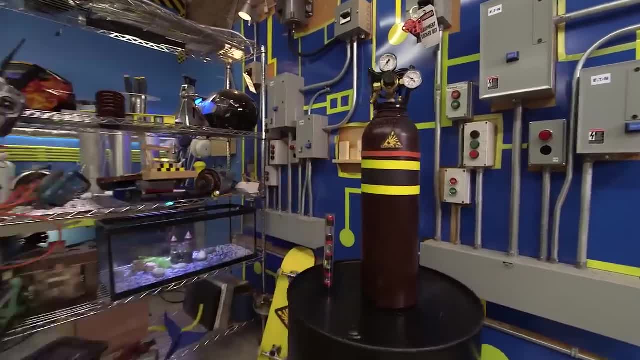 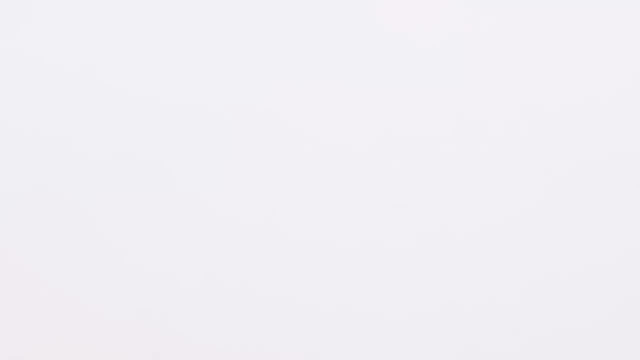 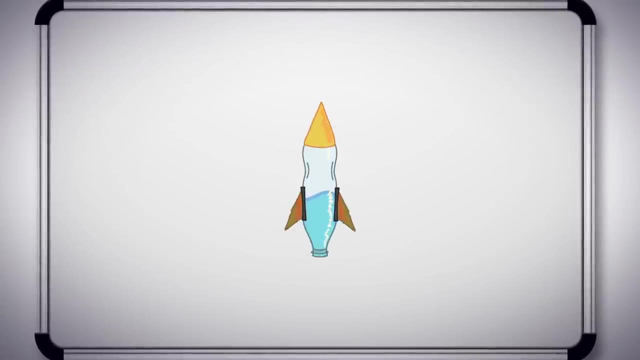 That is the power of pressure. Our air-powered rocket was working pretty well, but there's always room to max it out. In order to do that, we need to understand how it works. First, we fill the bottle almost halfway with water. 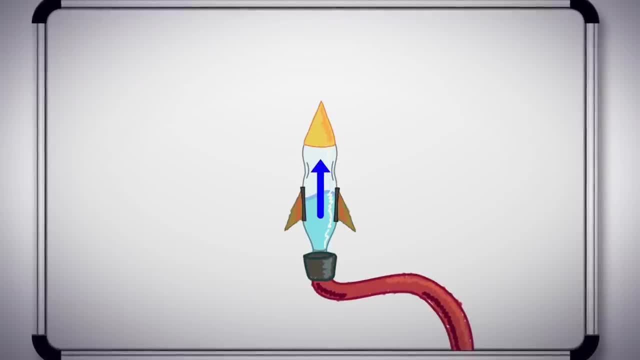 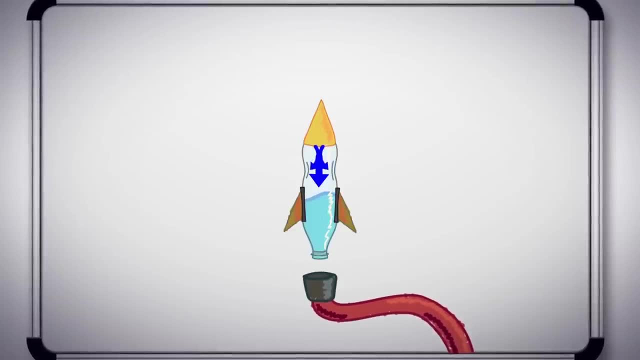 then we add air to the bottle, The air pressure builds up and the air presses down on the water. The rocket takes off when we pull on the release valve which was blocking the opening of the bottle. Once that happens, the air pushes out the water. 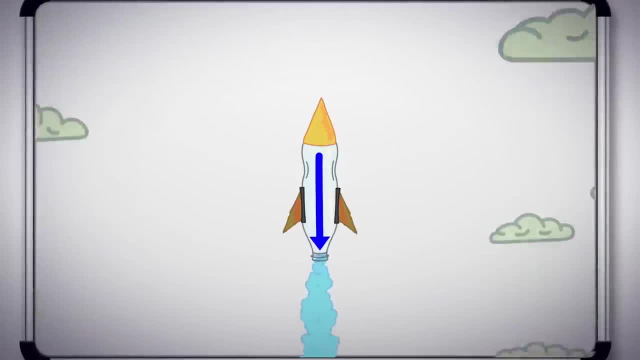 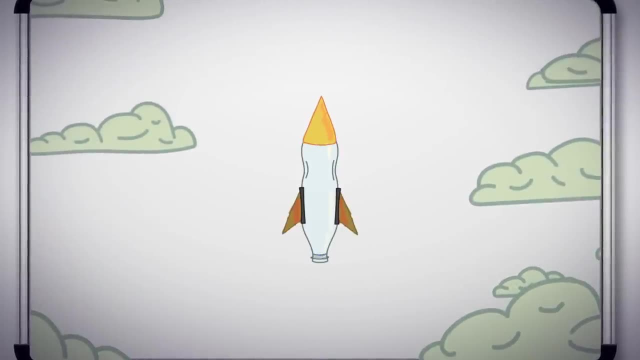 It's the water that gives us our thrust, so the water is very important. Once all the water is gone, the air escapes and the bottle returns to normal air pressure, But by that time it's high in the sky. Now the plan is: 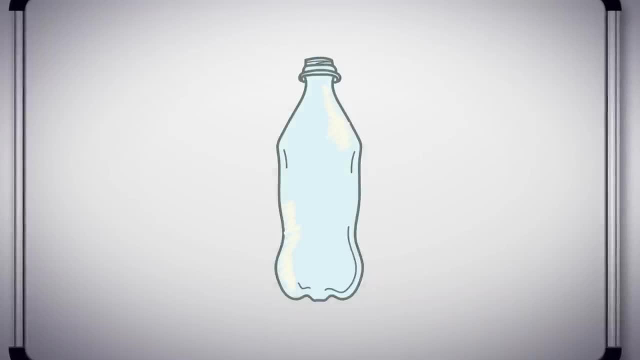 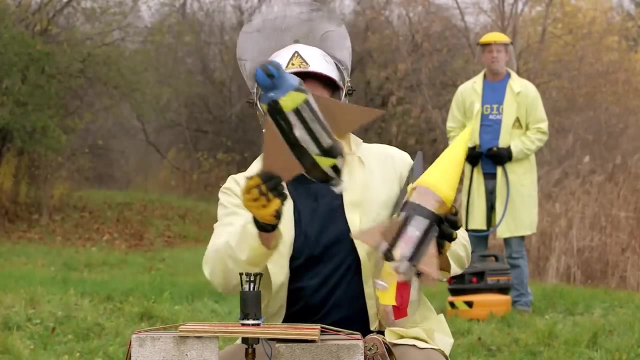 to use two liter bottles instead of regular water bottles to see if they work better. Now we've made a few more rockets out of two liter bottles and I'm going to fill this one up with water and we're going to fire it again. 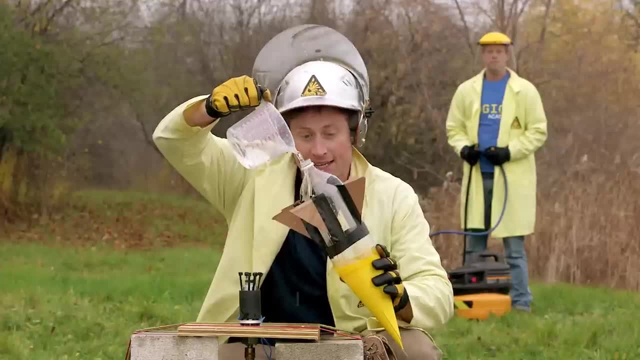 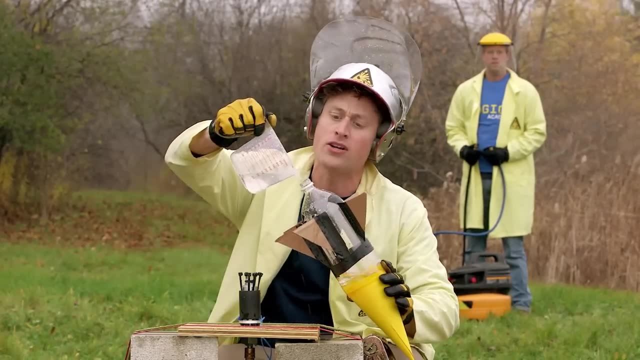 and see what happens Now. the idea is that these will work better because they have more volume, and more volume means we could possibly put more air pressure in. It's hard to know until you try it, of course, But the other reason why it might work better. 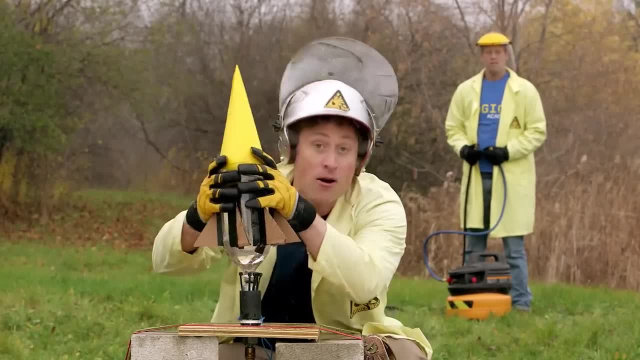 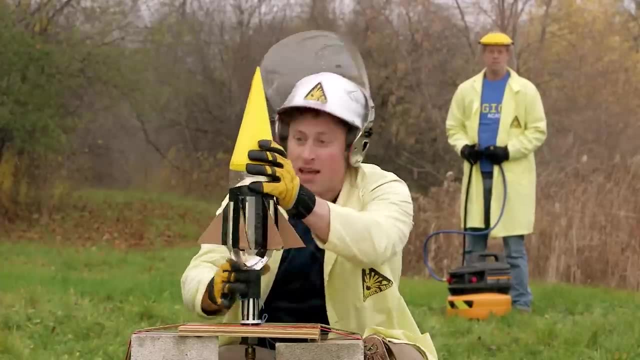 is two liter bottles generally hold carbonated beverages, which means that they already have to be made a little stronger than regular water bottles because they have to hold in the carbonation, which is just like air pressure. All right, Ready to go, Okay? 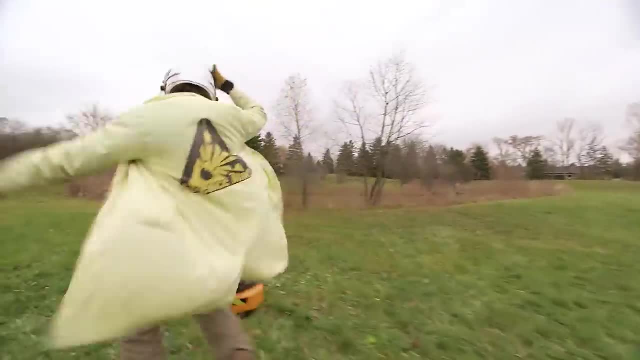 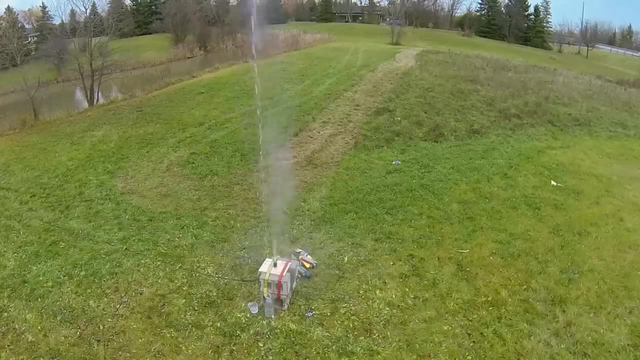 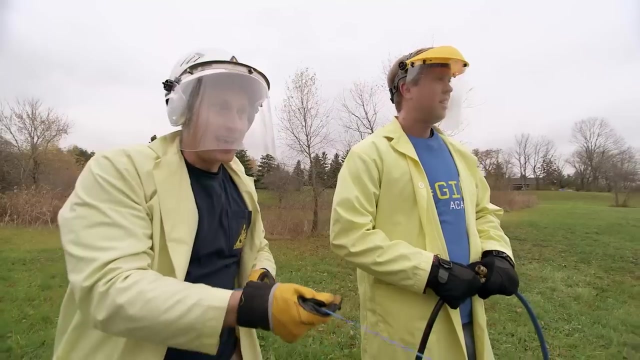 Here we go. You ready, Adam? Yep, Okay, Blast shield down, Pressurize. Three, two, one, Let's do another one. And three, two one, Three, two, one, Whoa Wow. 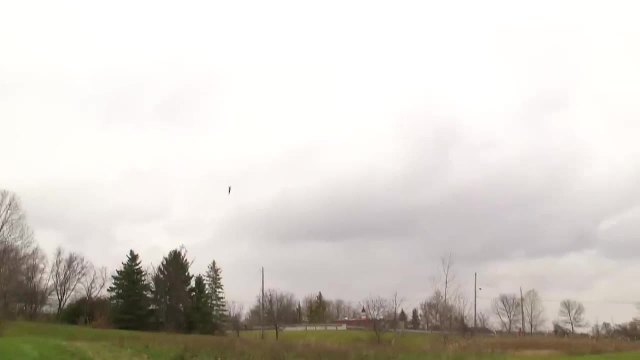 This is the superhero design rocket which I'm very excited about. All right Adam. It's going really well, But before we fire this next one, how can we make it bigger, better and more awesome? Getting more pressure, More pressure. 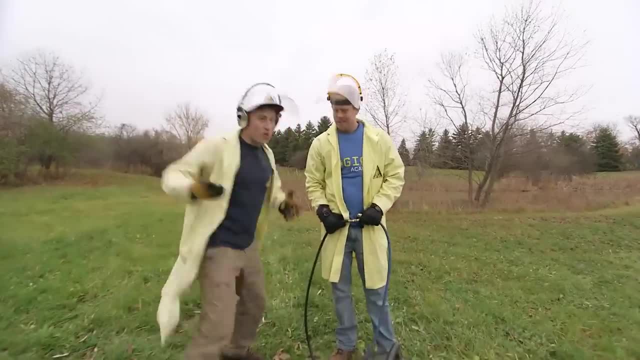 How do we do that? Well, we're firing at about 90 PSI right now. PSI pounds per square inch of pressure. right, Exactly, Yeah. So you know, you're going to have to get a little bit more pressure. 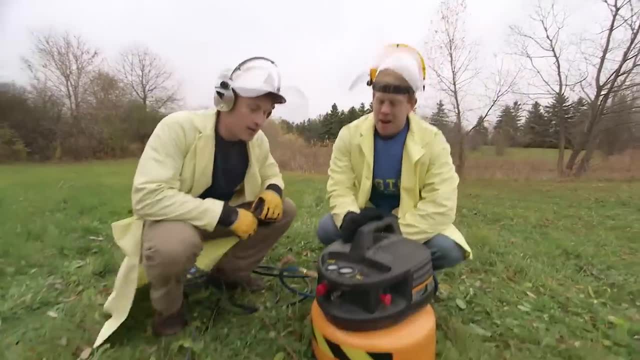 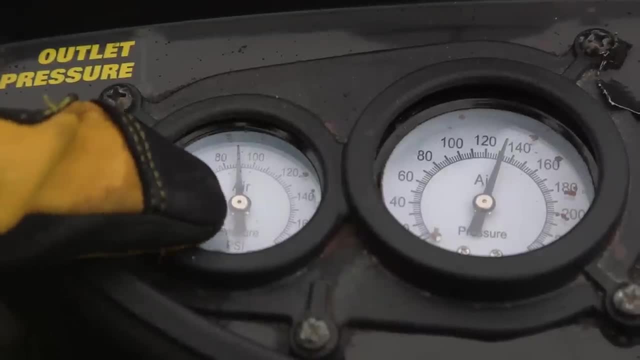 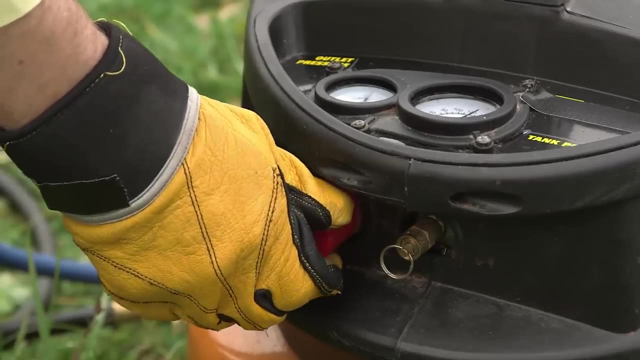 So how? We're at 90 now. How high does the tank go? Go to about 120.. 120 PSI, Let's see what happens. All right, Let's do it. Okay, Here we go: 90.. 110.. 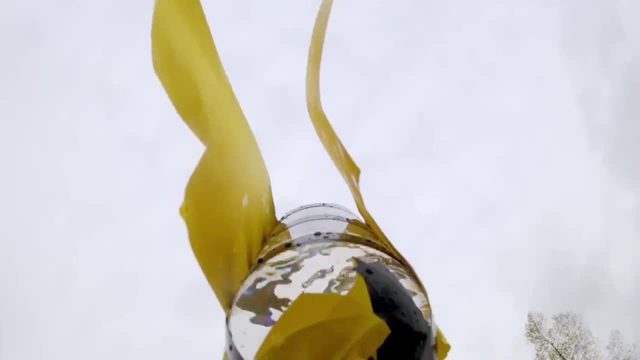 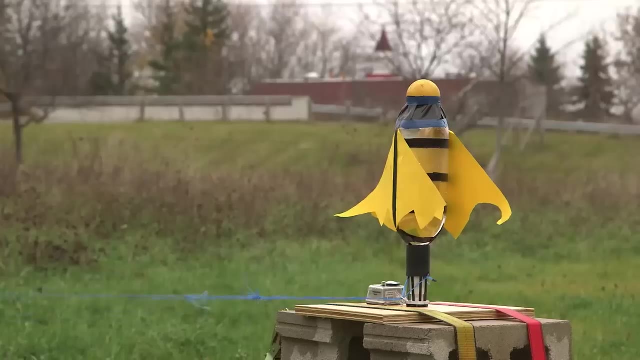 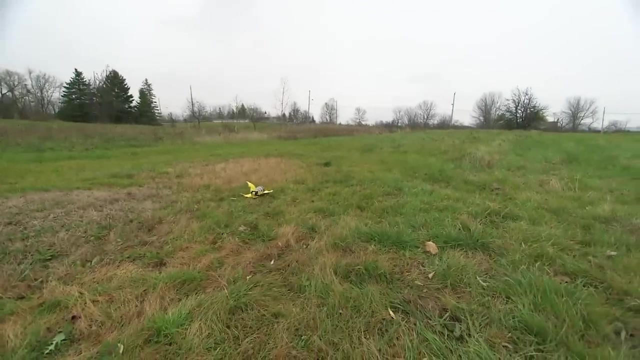 120.. Should we fire it? Let's fire it, Let's fire it. Here we go: Three, two, one. All right. Actually it worked okay. There's just a piece missing here. 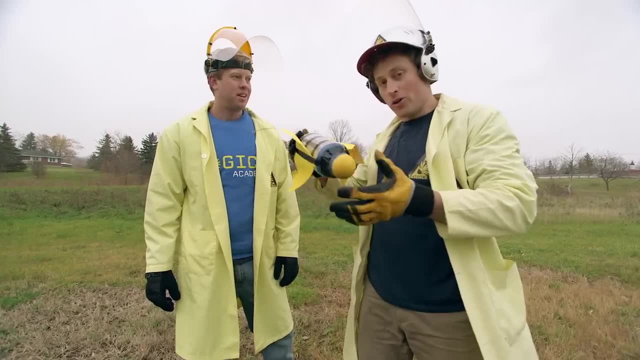 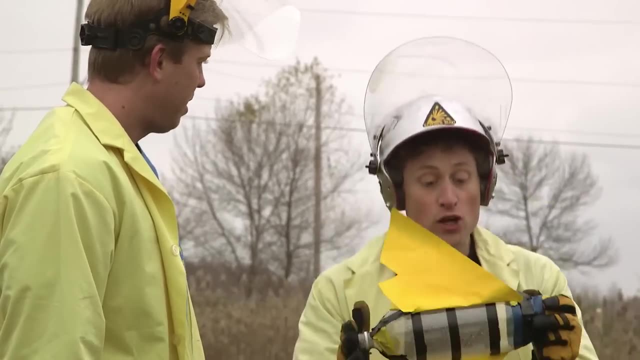 but I think the bottle is still okay. Yeah, So two-litre bottle, full pressure. I think we can still make something even better, even more maxed out. What if we used an even bigger bottle? You know, the five-litre ones that you see on water coolers. 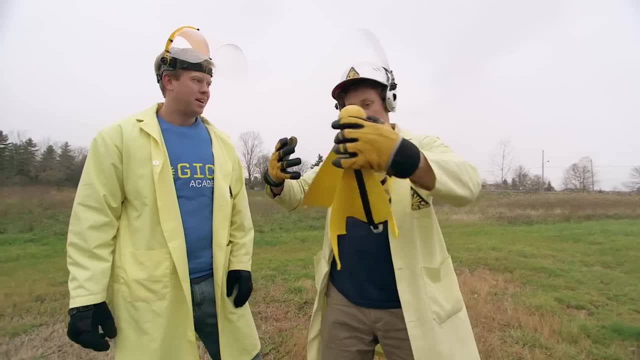 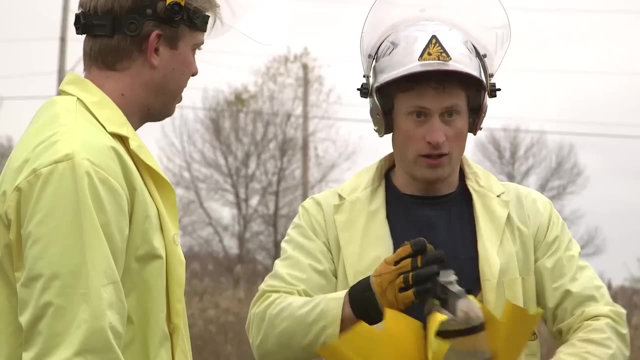 Yeah, You think we can use one of those. Definitely, I think we could use that. We need to change the mouthpiece size, Oh right, Yes, to fit our launchers. Well, let's do it, Let's do it. 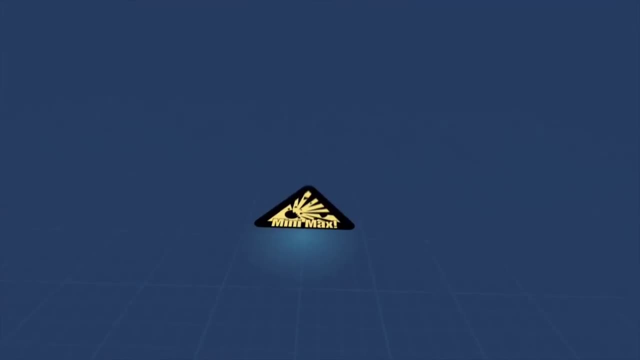 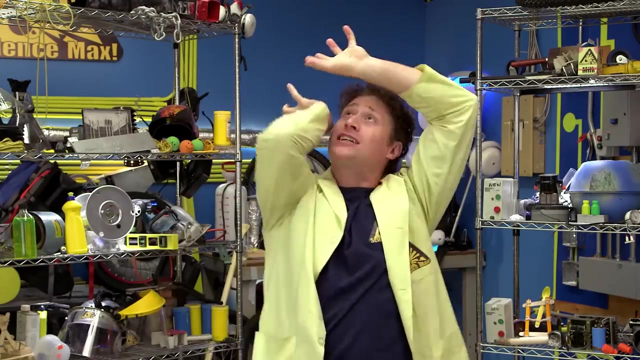 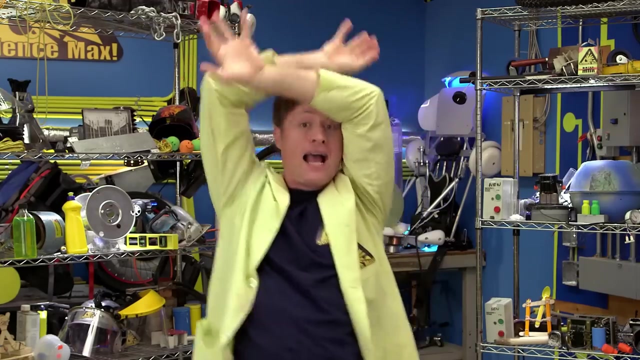 That's it. Mini Max, Help. I'm being crushed by all this pressure. A whole kilogram is being pushed down on every square centimeter of my body. 103 kilopascals, Ah, Actually, one kilogram for every square centimeter. 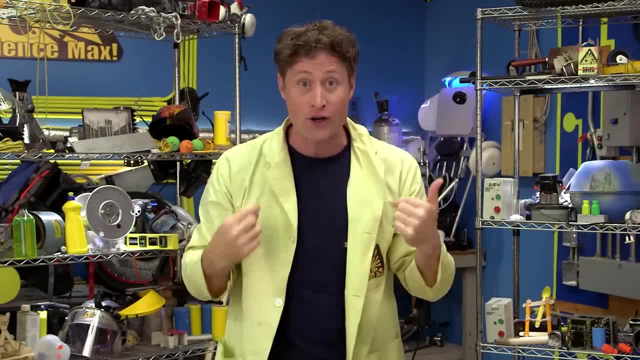 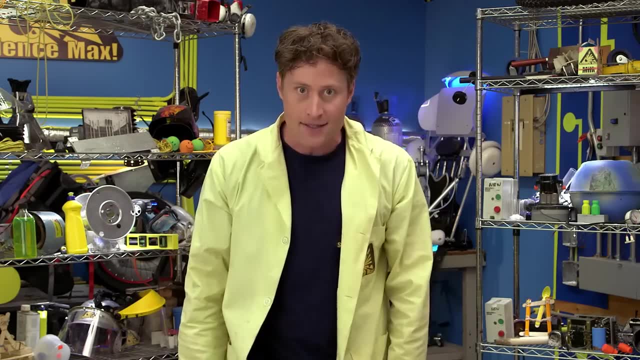 on your body is the exact kind of pressure that you and I are under at all times every day. We don't notice it because we're used to it, but it sounds like a lot, doesn't it? Well, it is. Here's an experiment you can do with a plastic bottle. 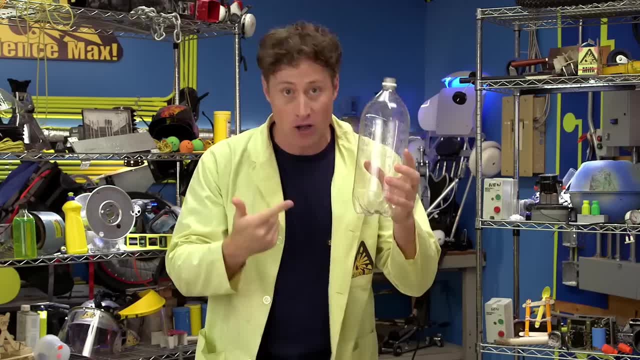 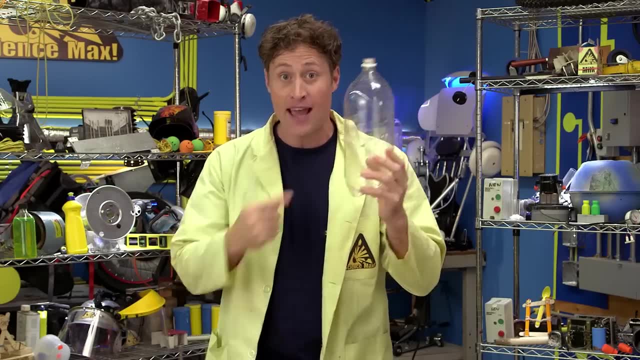 Say, at room temperature there are 10 million air molecules in here. Doesn't really matter how many, but we'll say there's 10 million at normal room temperature. What happens if I heat up the air inside this bottle? This is warm water. 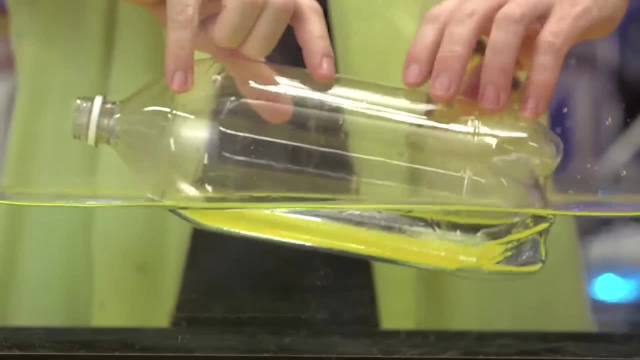 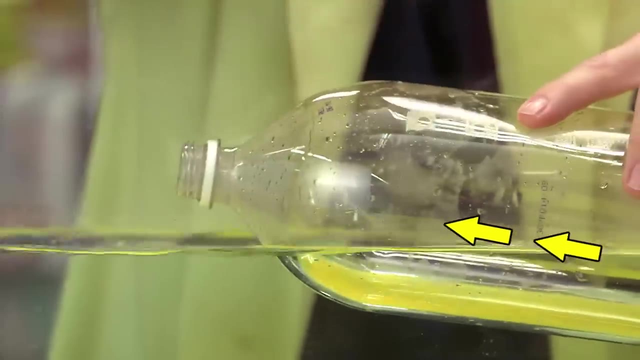 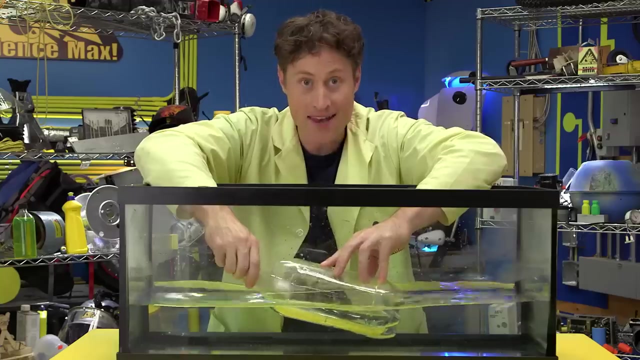 What I'm trying to do is heat up the air inside the bottle because the air molecules, when they get hotter, move faster and need more room. So the 10 million air molecules are starting to escape out the mouth of the bottle and reducing the number of air molecules inside. 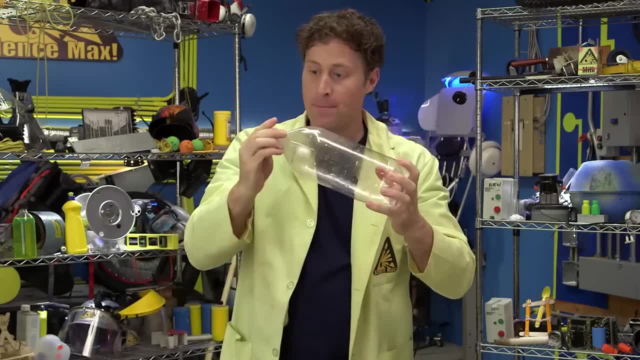 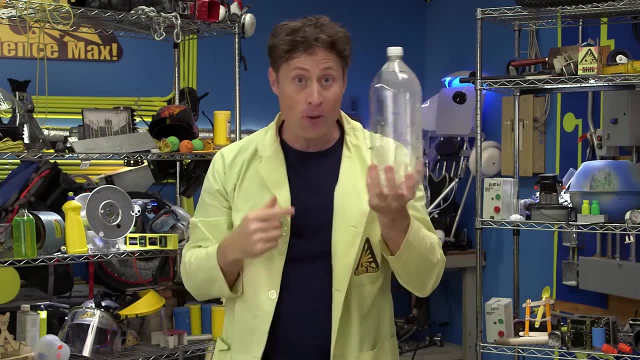 And now I take the bottle out and cap it Because the air molecules heated up and speeded up. they needed more room. Now there's less of them in the bottle. There's about 4 million air molecules inside this bottle, but they're all hot air molecules. 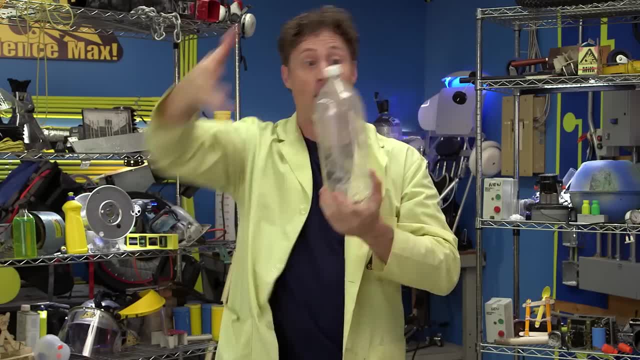 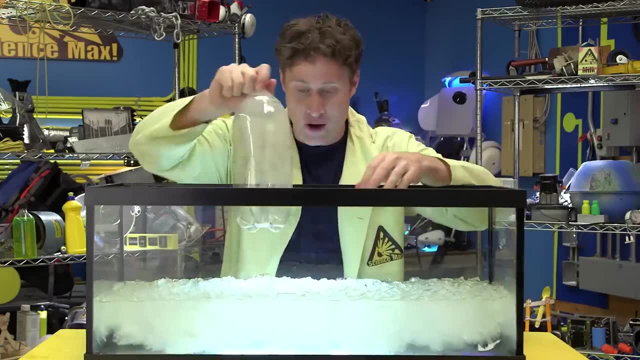 and they have a higher pressure and you don't notice it because the air out here isn't crushing the bottle. But watch what happens if I cool the air inside the bottle: This is ice water. So what's happening now is the molecules are slowing down. 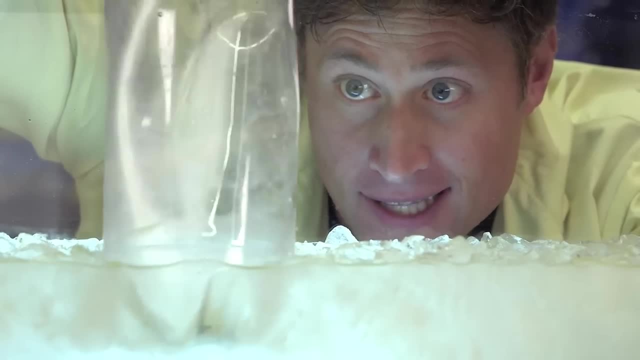 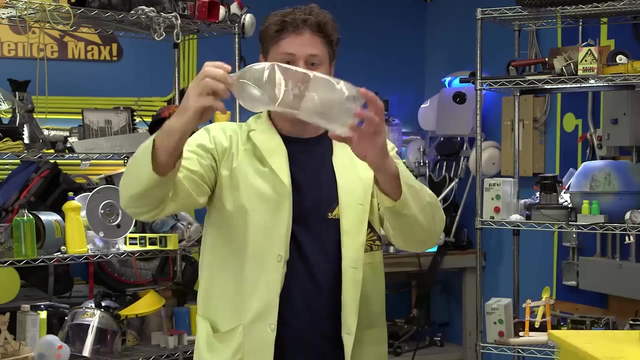 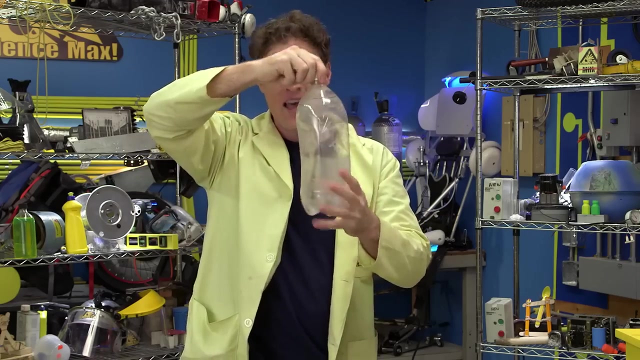 and they need less space. So they need less room and they're being crushed by the pressure on the outside of the bottle. It has been crushed because the colder air molecules don't need the same kind of room as the hot air molecules. The room temperature air has crushed the bottle. 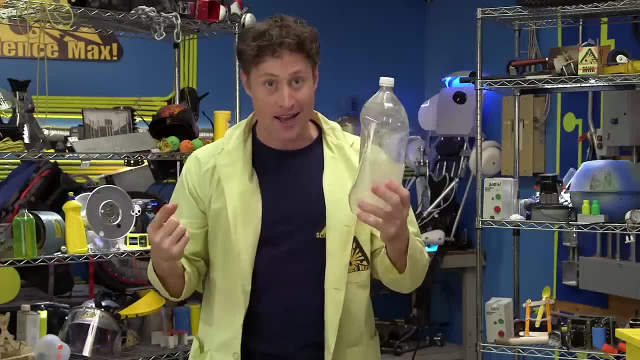 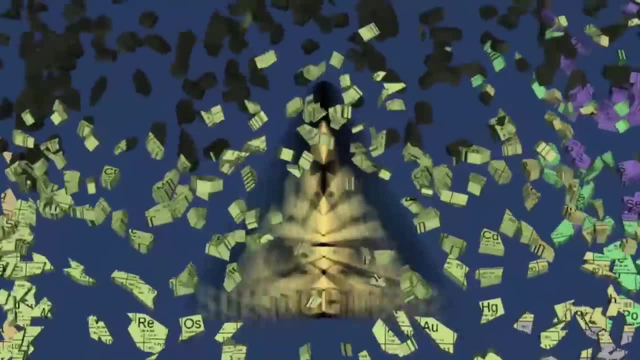 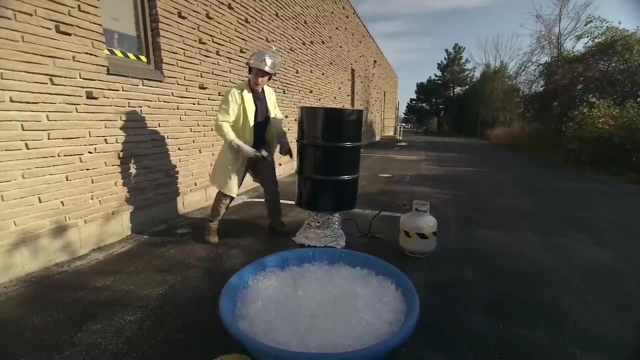 The air inside has a lower pressure than the air outside. Pretty amazing. Even more amazing when we max it out. This is a steel drum. What we've done is we've put some water in it and we're heating it up to boiling, so there's nothing but hot air inside the drum. 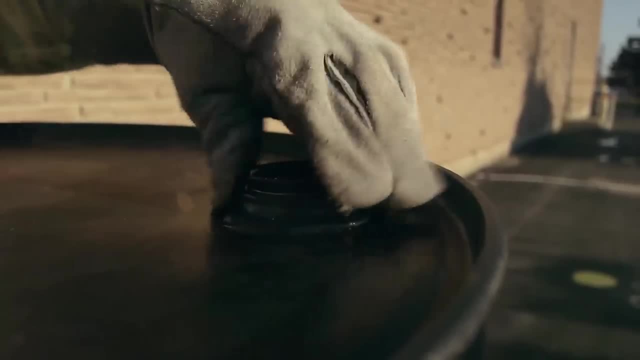 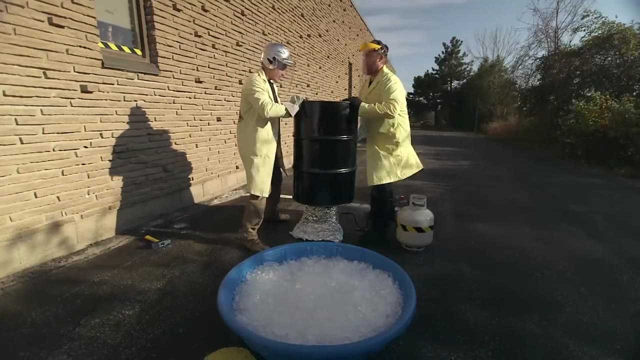 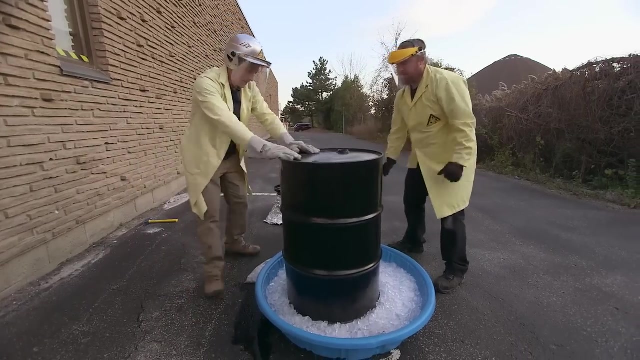 This is an airtight cap which we use to seal the drum And now we cool the drum off. Hey, Trevor, give me a hand Ready. One, two, three you lift. That's good, This pool is filled with ice. 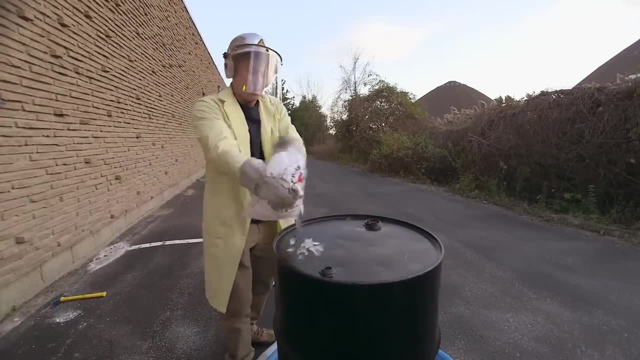 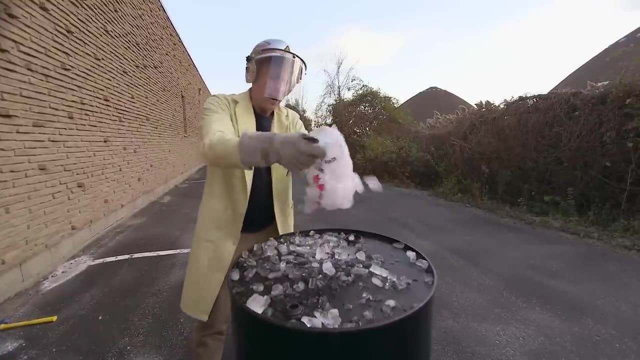 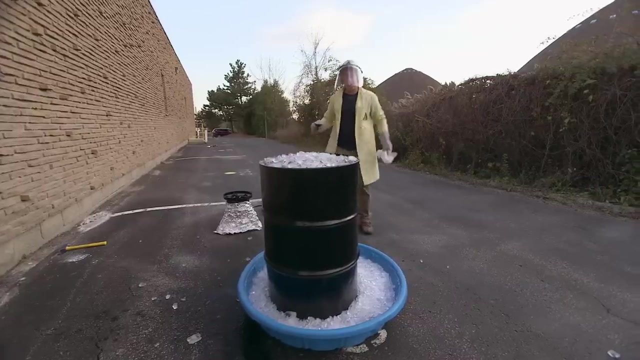 What we're doing now is cooling off the steel drum, which will cool off the air inside it, Which means eventually, the air inside the steel drum will be a much lower pressure than the air outside the steel drum, Because this steel drum has a lot more volume. 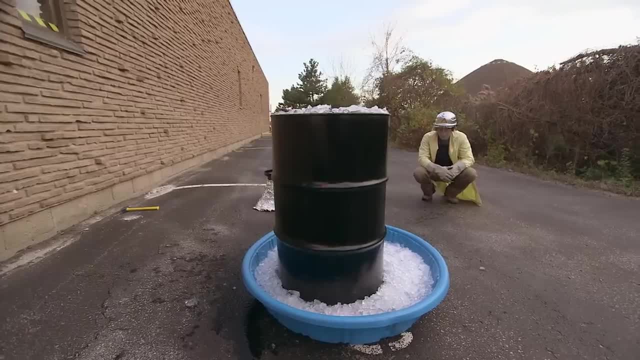 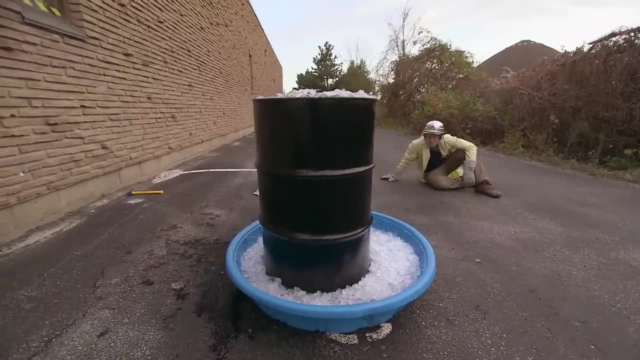 than a two litre pop bottle. it takes a lot longer for the air to cool down. The other thing to think about is that it's a steel drum. I could stand on it and it wouldn't even dent, but sure enough, after a few minutes. Whoa, Check it out. The barrel has totally crushed. The low pressure air inside the barrel wasn't enough to withstand the force. The low pressure air inside the barrel wasn't enough to withstand the force. The low pressure air inside the barrel wasn't enough to withstand the force. 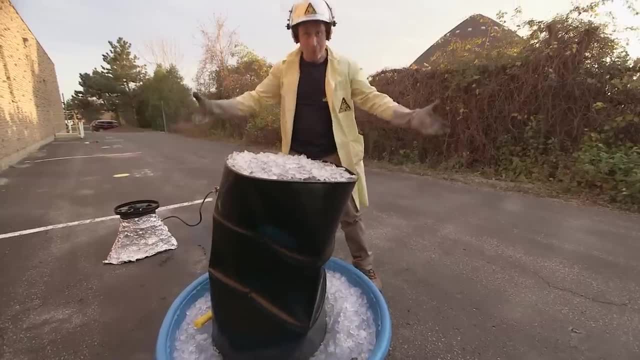 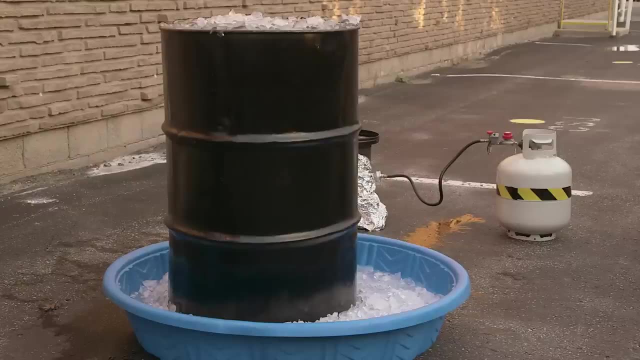 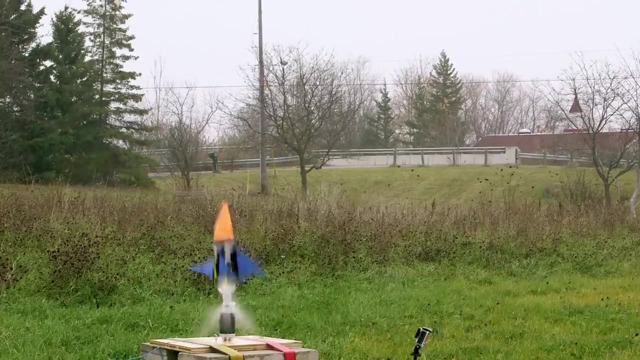 wasn't enough to withstand the force of the regular air pressure that you and I walk through every day. The air pressure all around us is enough to crush a steel drum. How cool is that? Our air-powered rockets have been working really well, but we still want to go further. 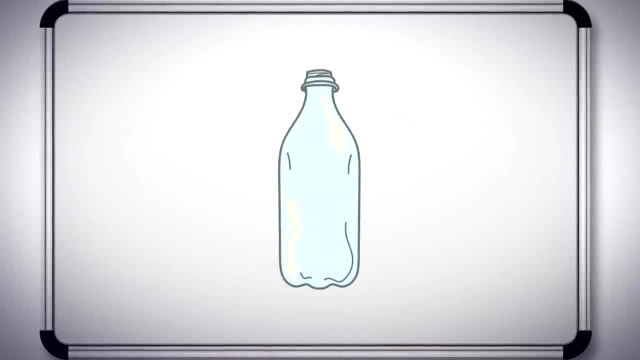 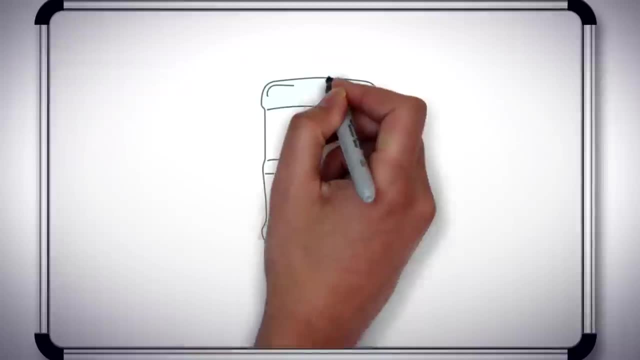 Since the two-liter bottle worked better than the water bottle, we think increasing the size again might make it more awesome. So now the plan is to switch our two-liter bottle with a 20-liter water cooler jug and make a rocket out of that. 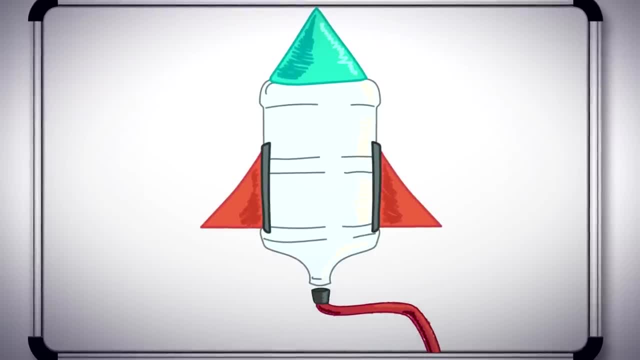 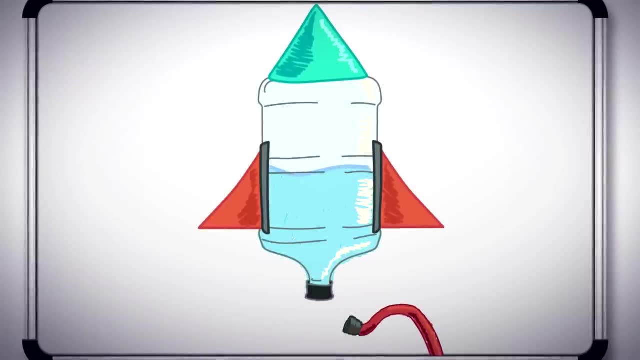 Because the launcher nozzle, which holds the bottle in place till we're ready to launch it, isn't going to fit the opening of this bigger jug, we've decided to use the cap that came with the jug. If we screw the cap on, it'll work sort of like the cork. 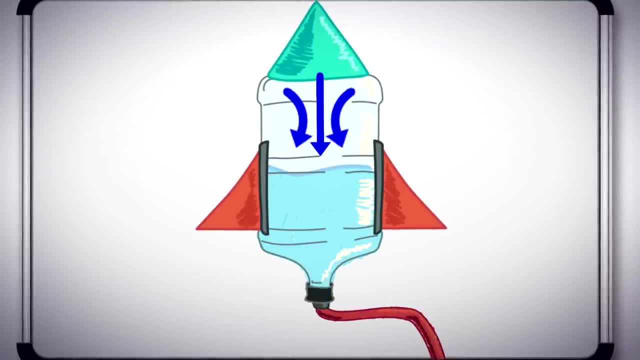 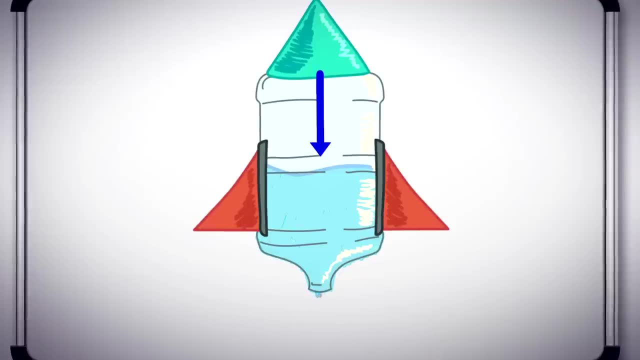 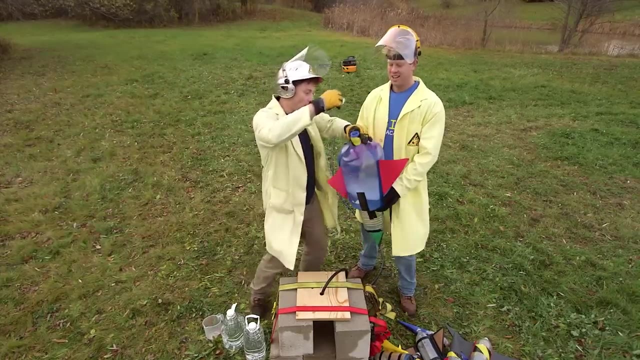 The air pressure will press down on the water and keep pushing against the cap until the cap has a catastrophic failure, which is a very cool way of saying that eventually the cap will break and the bottle will shoot into the sky. 20-liter water cooler jug filled with some water. 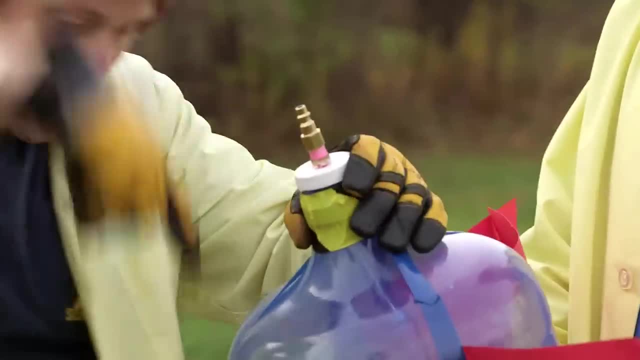 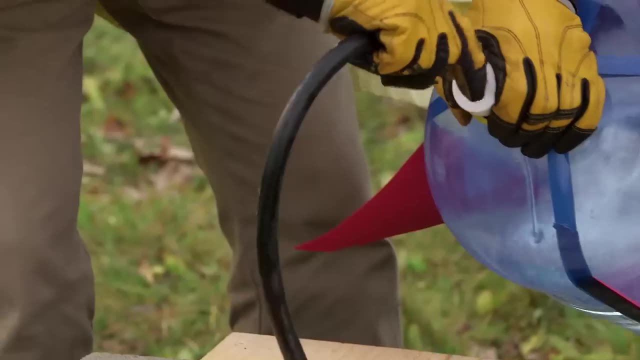 This is the cap that'll work sort of like the cork: We put the air pressure in there, the cap can't take it anymore, pops off and the thing flies. hopefully Let's find out. Okay, that looks good There. 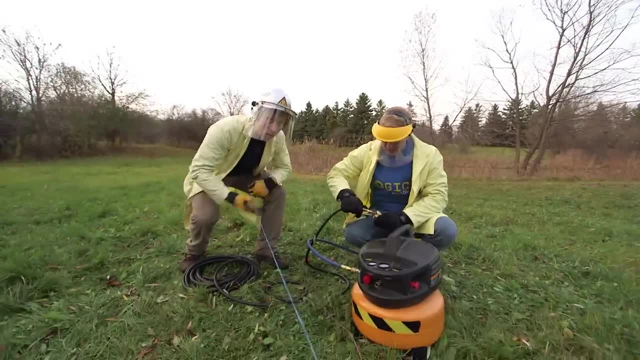 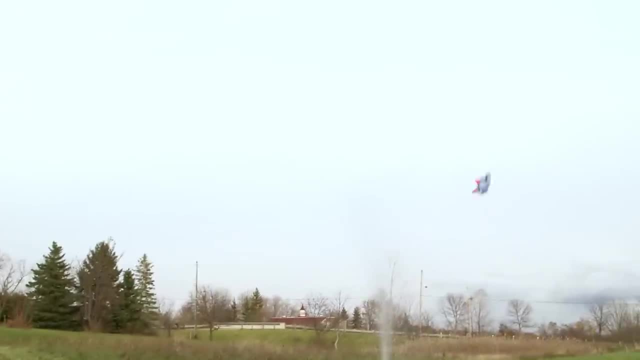 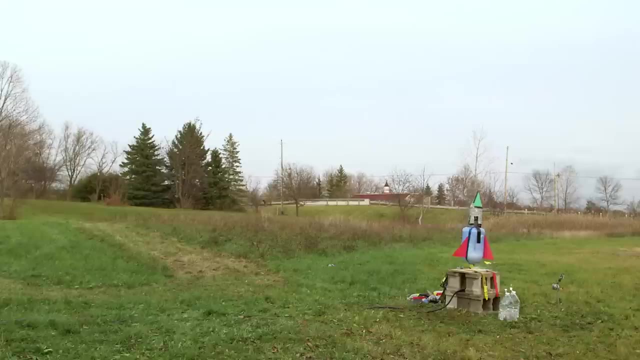 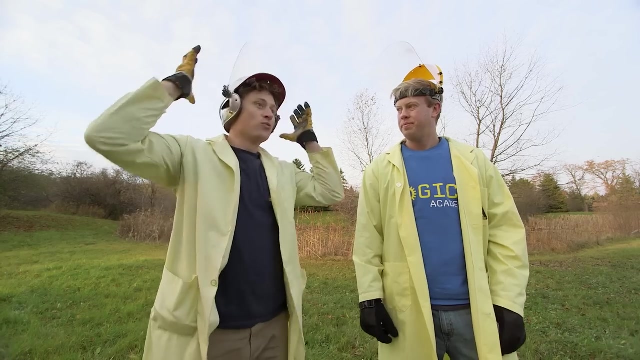 Let's do this. Go for pressure. Uh-oh, Uh-oh, Whoa Hilarious. That worked pretty well. It sort of does that. I wonder if it's aerodynamic? No, No, So how do we? 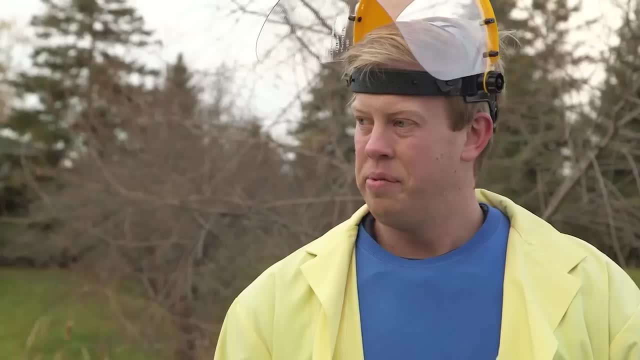 What else can we do to make it even more maxed out? I think we can use the 2-liter bottles. They work really well. The 2-liter bottles are the best right, I think so. So what do we do? 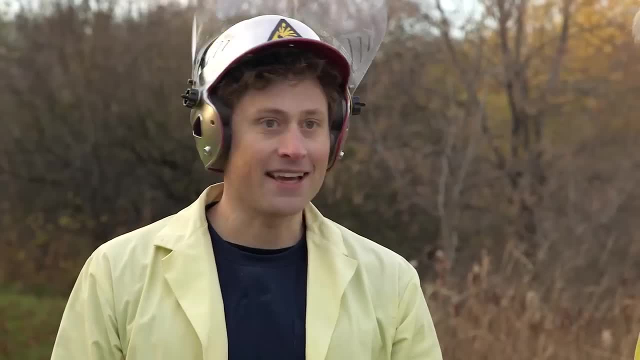 We can probably stack them. We stack them on top, Top each other. Yeah, That'd work, I like that. So we'd put a whole bunch of them together. Yeah, Tell you what I'll do you one better. 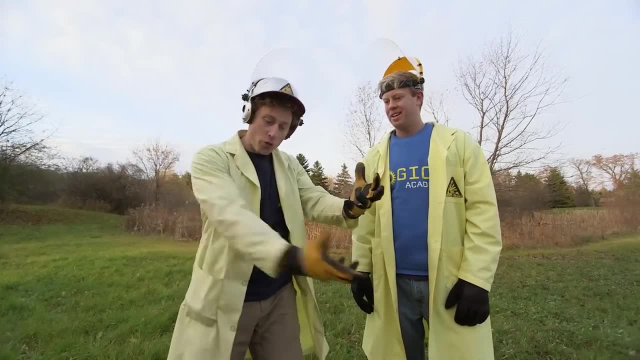 Why don't we use three stacks? Awesome, We'll use three stacks, three launchers, three times the thrust, and we'll make a giant rocket out of a 2-liter bottle. Yeah, great idea, High fives, Here we go. 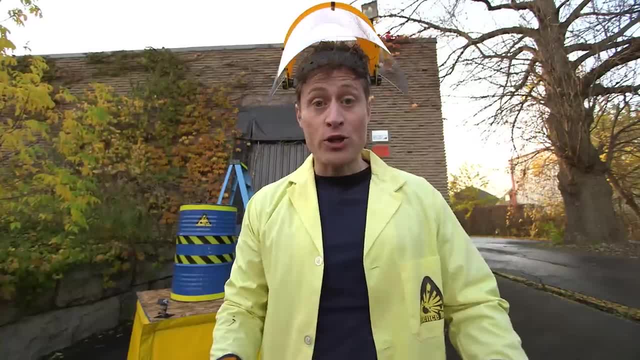 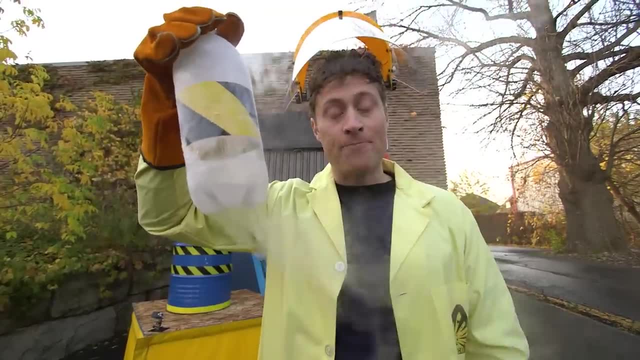 Gas molecules get further apart when you warm them up and closer together when you cool them down. So what happens if you keep cooling them down? Well, they turn into this. This is liquid nitrogen. Nitrogen makes up 78% of the air we breathe. 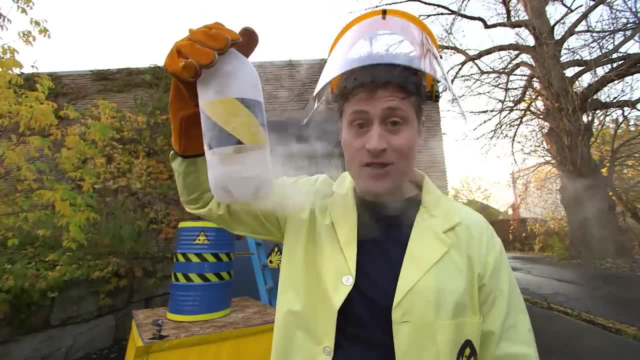 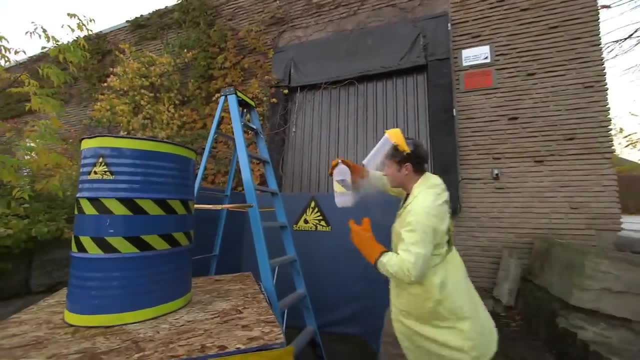 but when you cool it down to minus 196 degrees Celsius, it turns into a liquid. It's boiling right now because at room temperature, nitrogen wants to be a gas. So the liquid nitrogen is turning into gaseous nitrogen and all of the extra molecules are escaping. 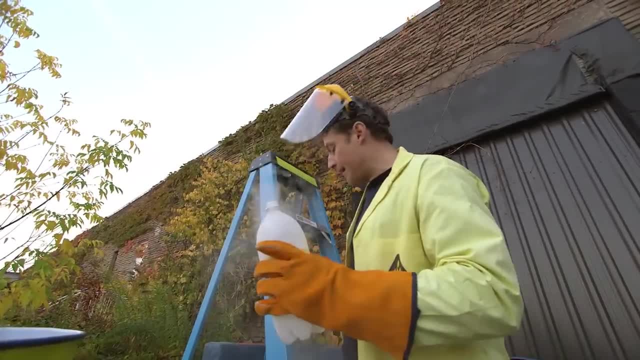 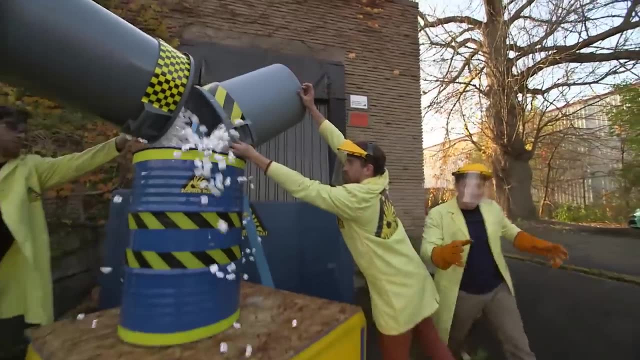 through the top of the bottle. So what happens if I put a cap on the bottle Right now? the liquid nitrogen is turning back into a gas. but what happens if I put a cap on the bottle? But because there's a cap on the bottle, the gas has nowhere to go, So the pressure is just going to keep building and building until the plastic bottle can't contain it anymore. and, And, And, And. It pops like a balloon. Science, Science, Science, Science. 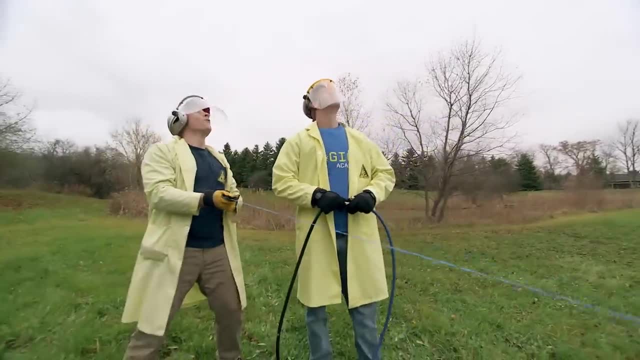 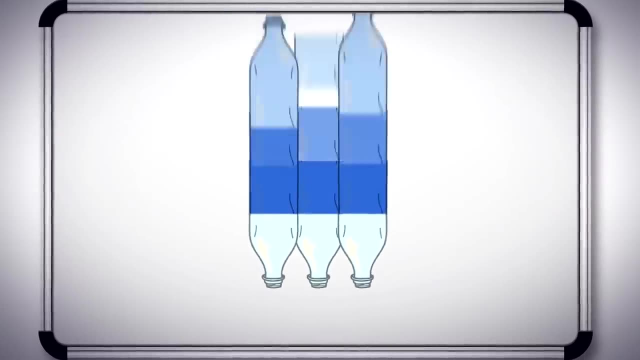 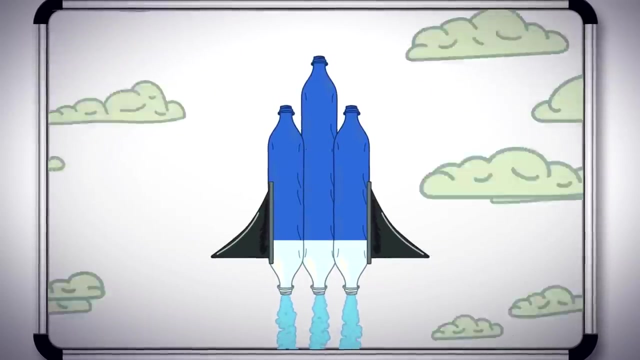 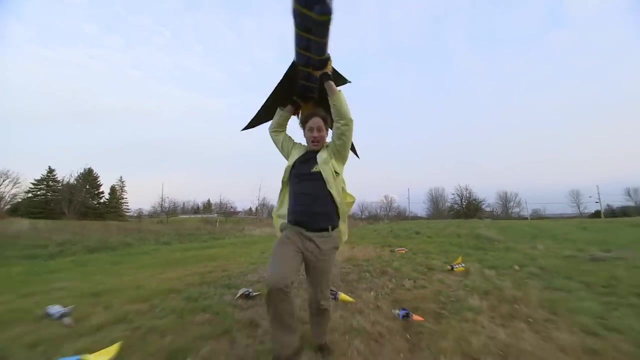 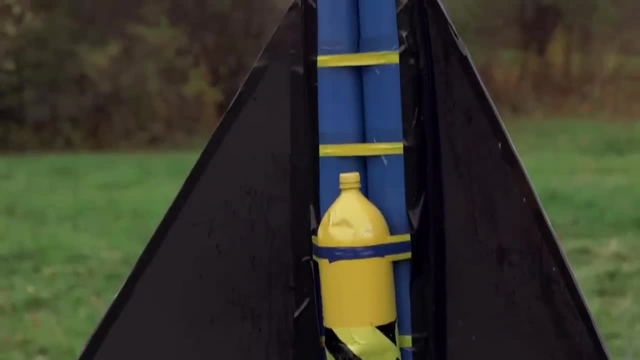 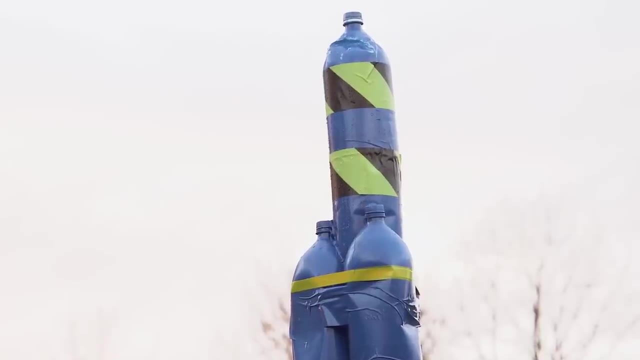 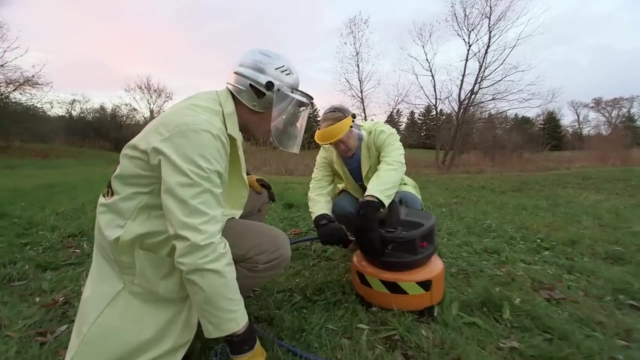 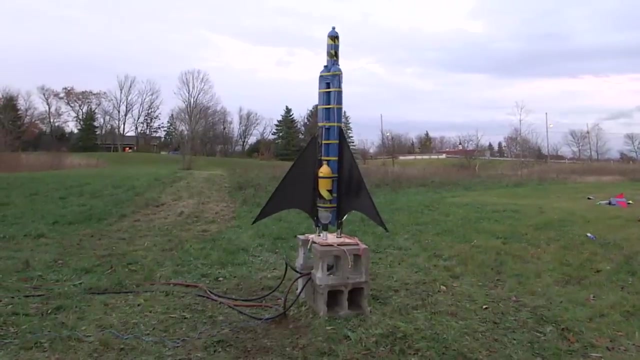 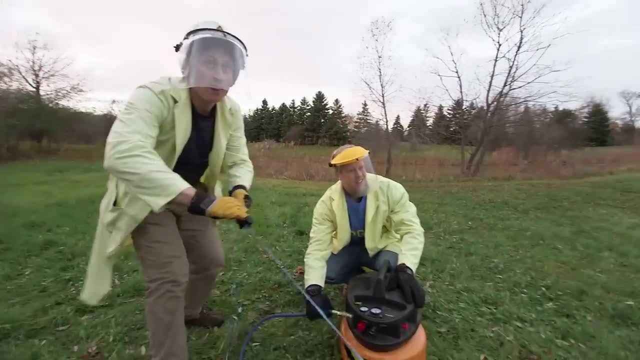 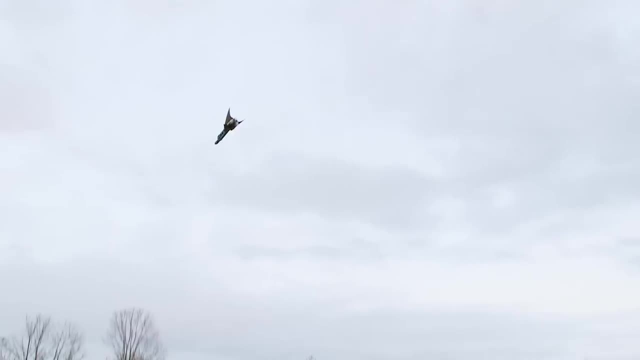 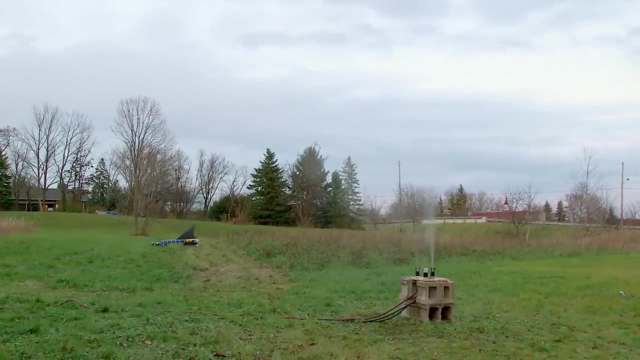 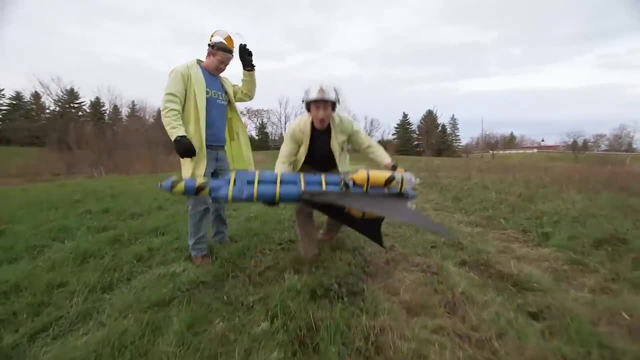 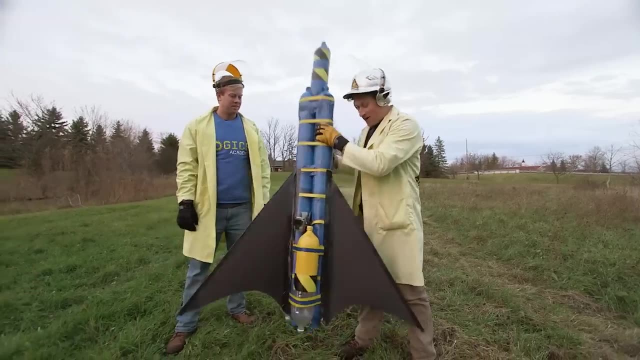 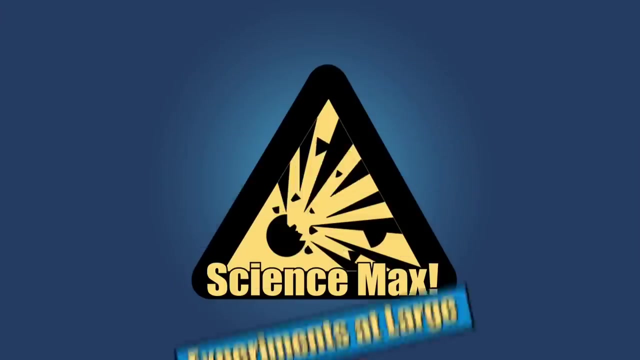 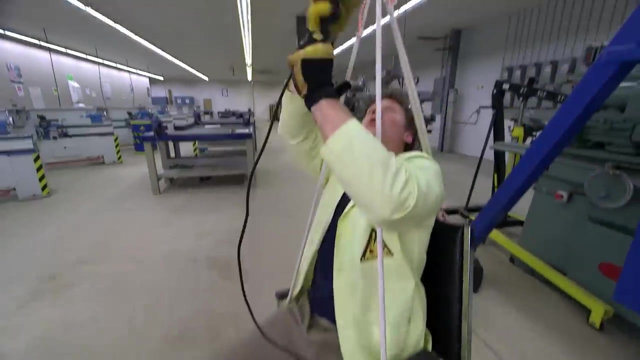 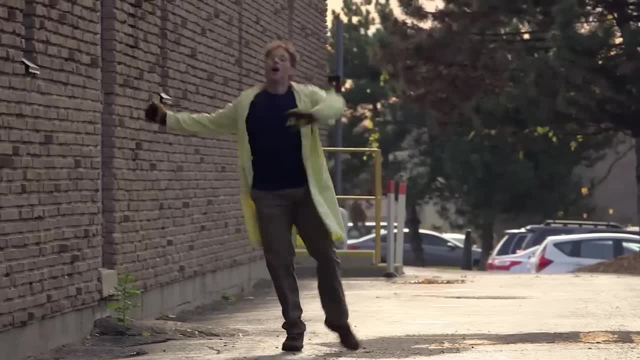 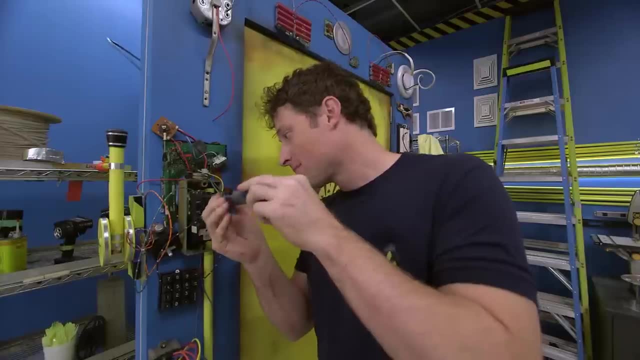 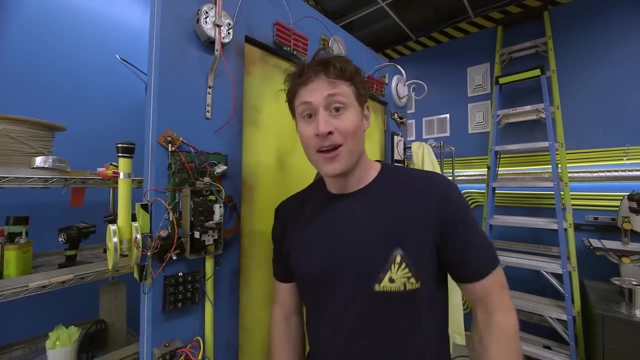 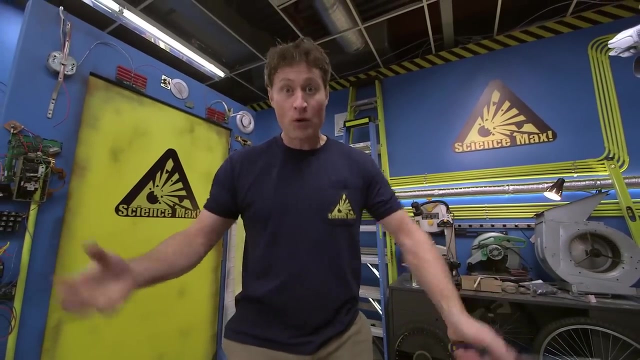 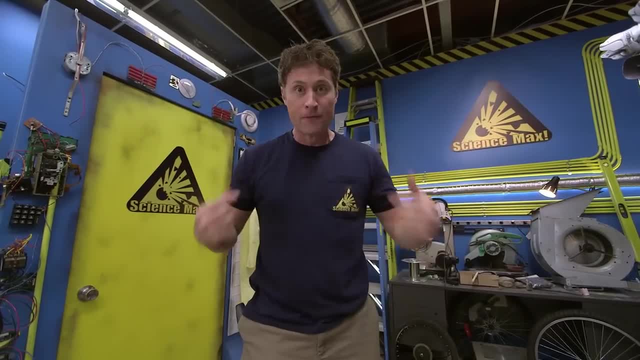 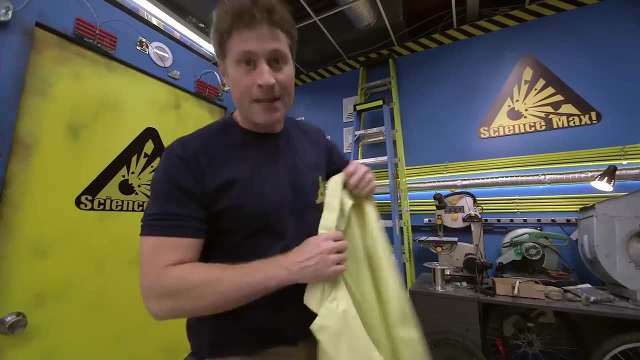 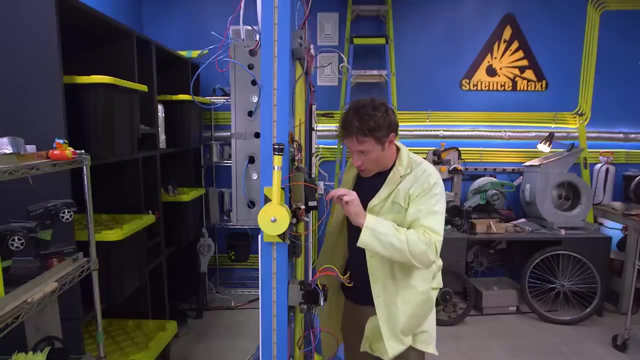 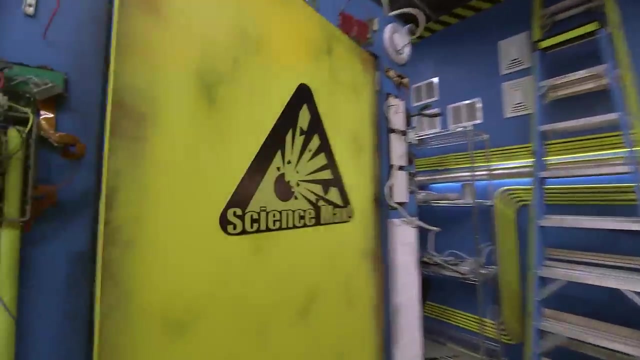 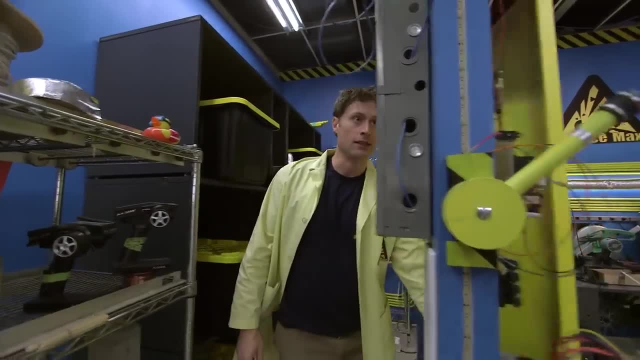 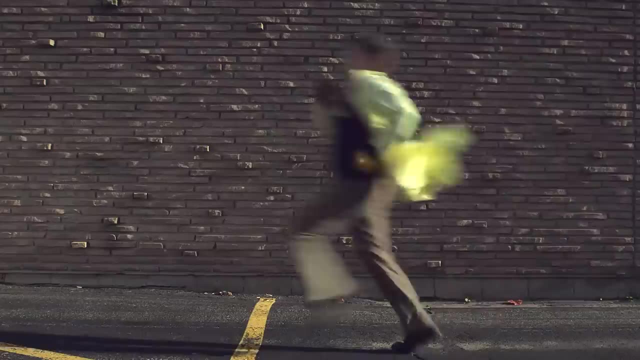 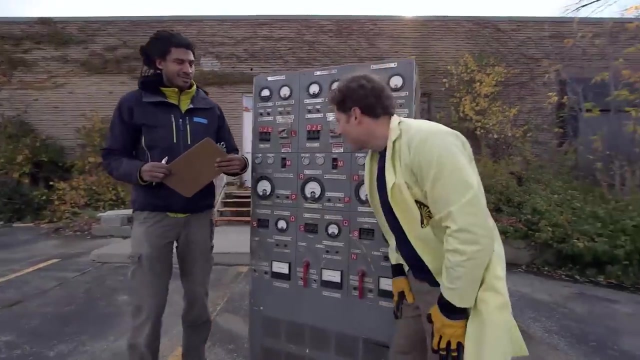 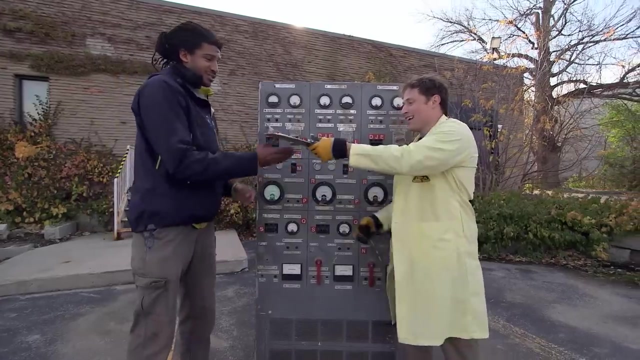 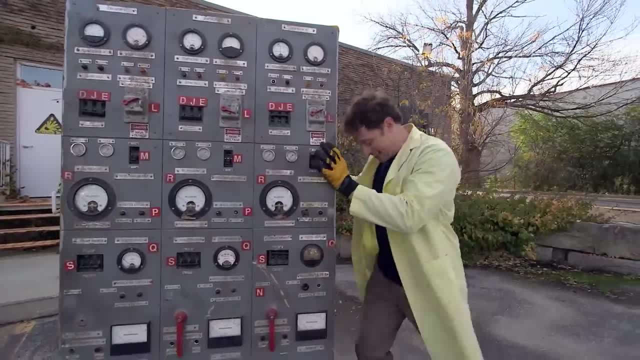 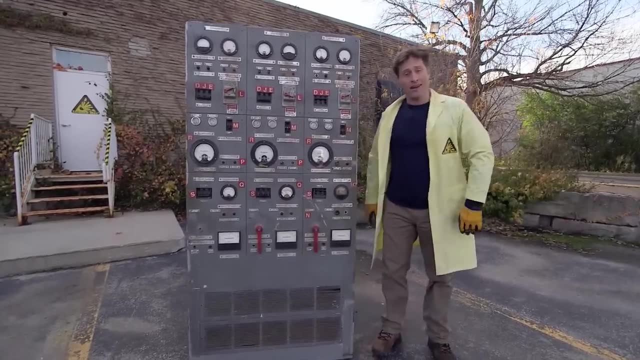 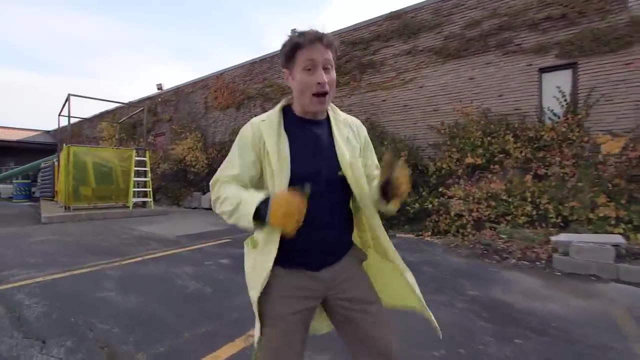 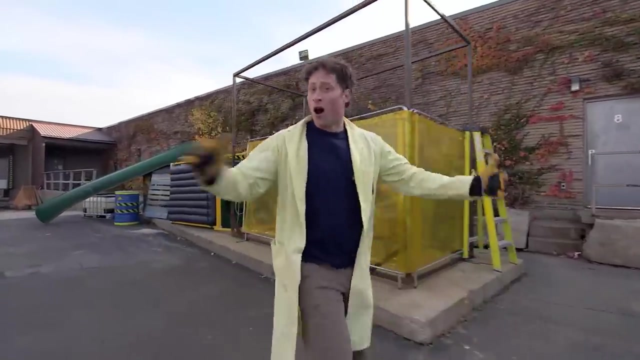 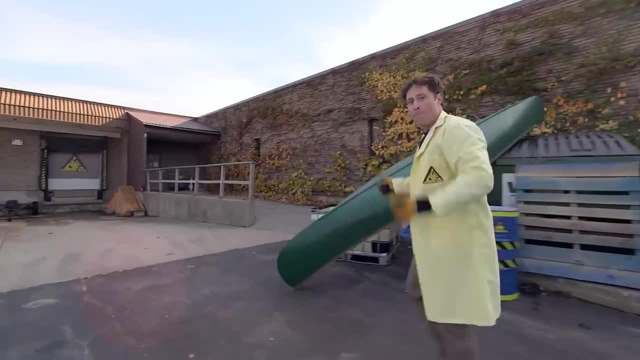 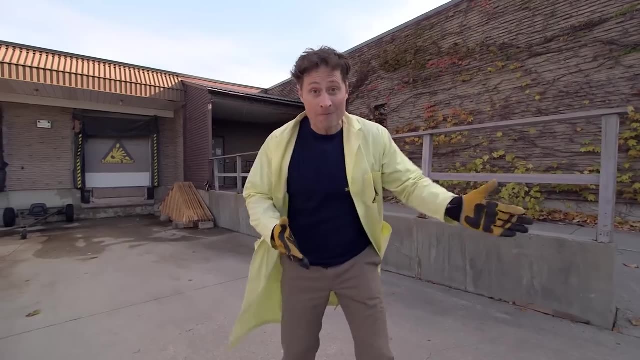 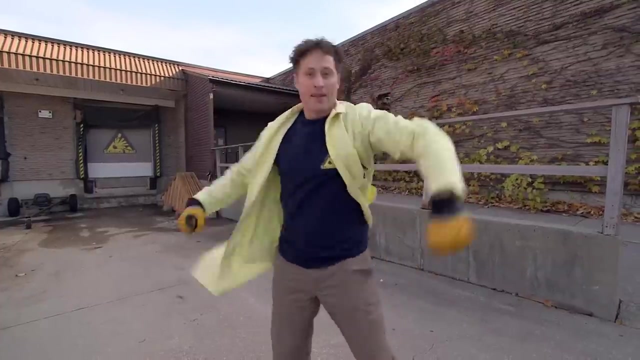 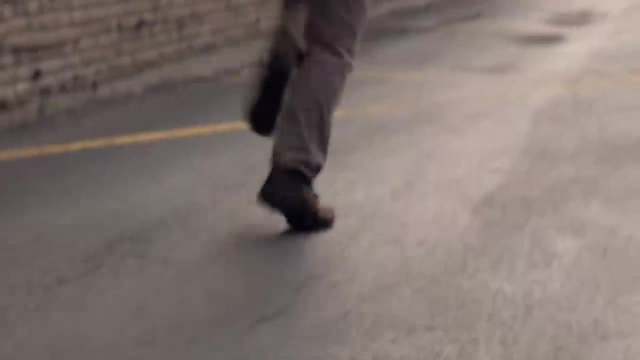 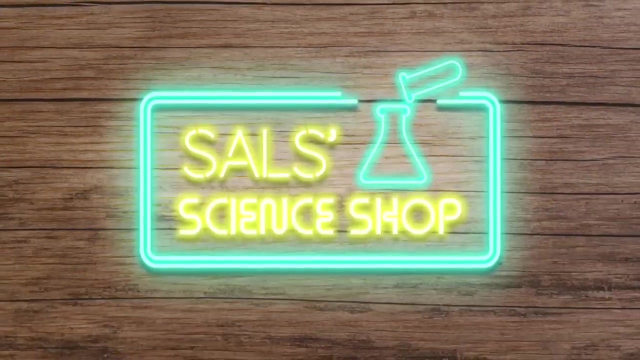 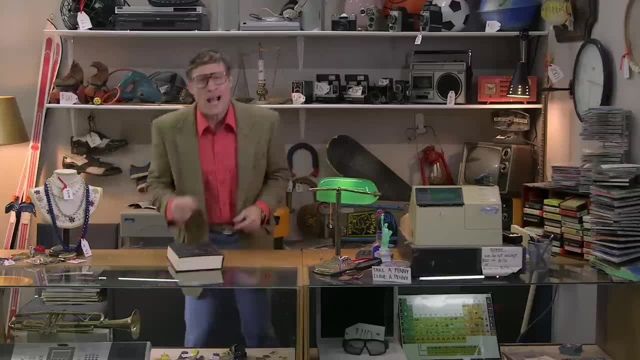 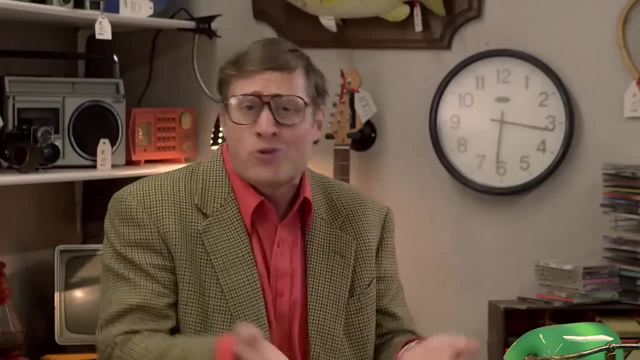 Oh, hey, how you doing. Let me guess You got some work to do and you need it done easy, right? I mean, look at this book. I mean you could pick it up, but what are you going to be some sort of book-picker-upper person now? 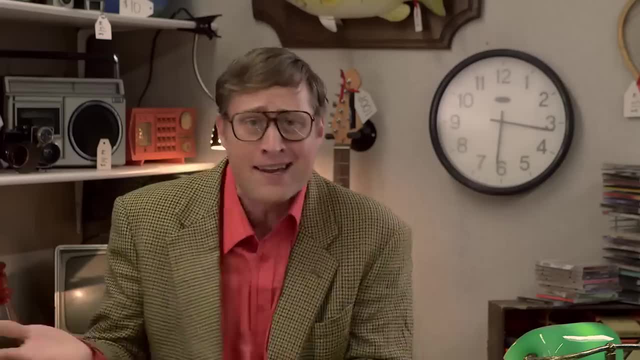 Is that all you're going to do? Is that going to be your life just picking up books left, right and center? No, you're smarter than that. You know what you need A lever like this. Now, I know what you're thinking. 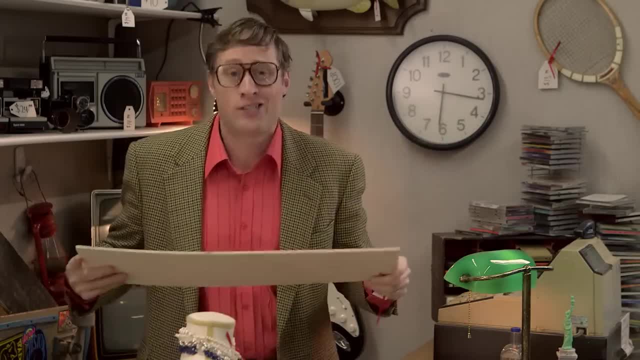 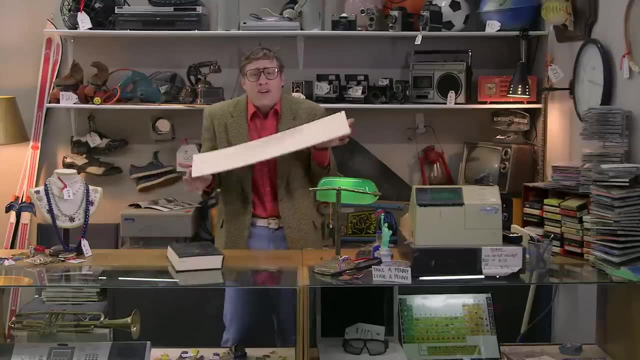 I know you're thinking: hey, this is just a plank. You're right, That's because you're smart. A plank can be a lever. All you need is two sides and a place for it to pivot- A fulcrum. 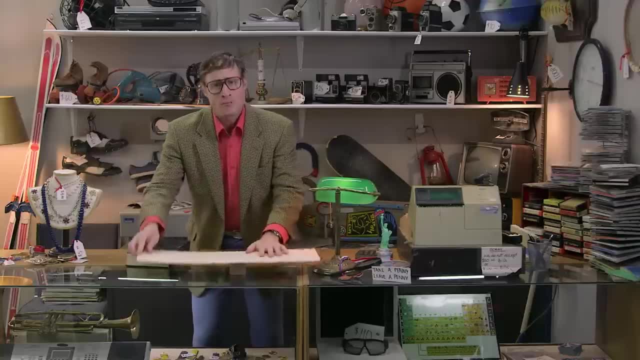 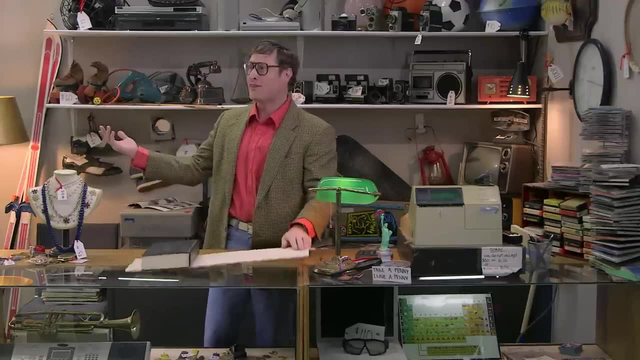 It can be anything. Look at this Bam. Now it's pivoting. I put the book on this side and then I push down on that side. I'm doing work easy. Hey, look at me doing this work over here. 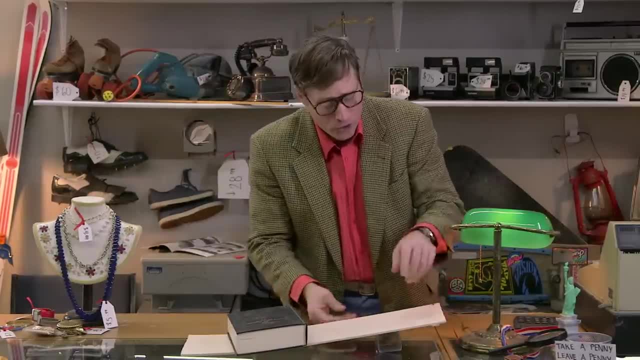 If I want to do more work, I could move this book over here. I could move this book over here. I could move the fulcrum a little bit further over. Now I do lots of work, but I lift the book a lot further. 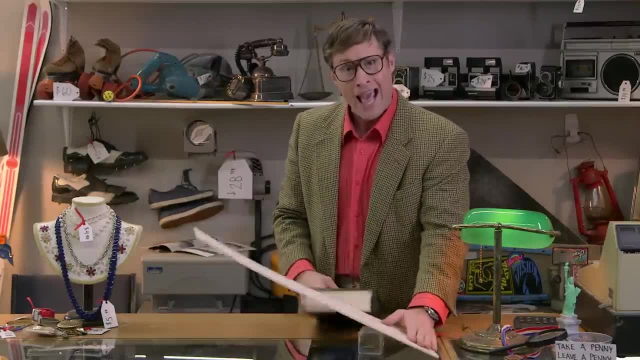 Look at that: Whoa, What, Whoa, Yeah, Huh. What do you say? What do you say? Huh, Huh. You don't like this lever, Don't worry, Hold on, I got another one for you here. 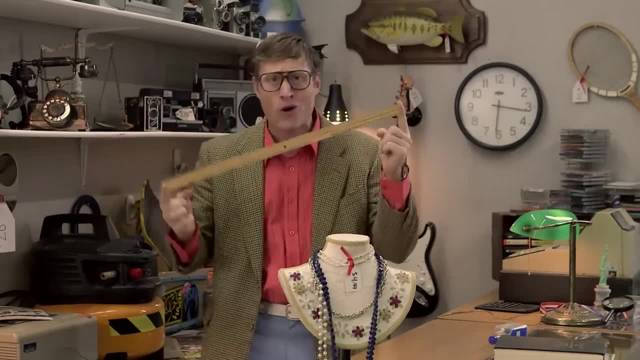 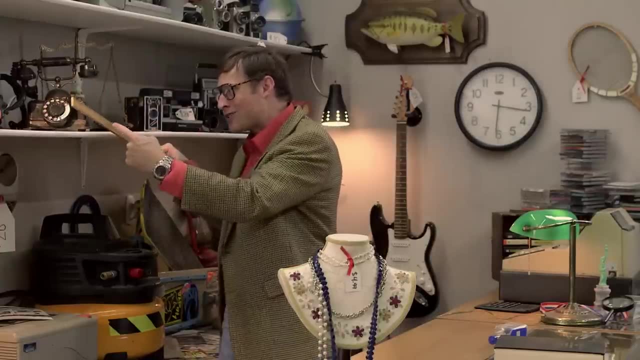 Hey, take this stick. All you need is two ends and a place for it to pivot like this Bam. Now it's a lever. This side goes down, That side goes up, Down, Up. It's a lever, It's a lever. 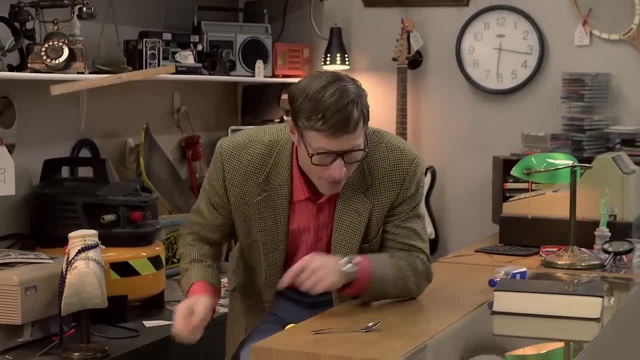 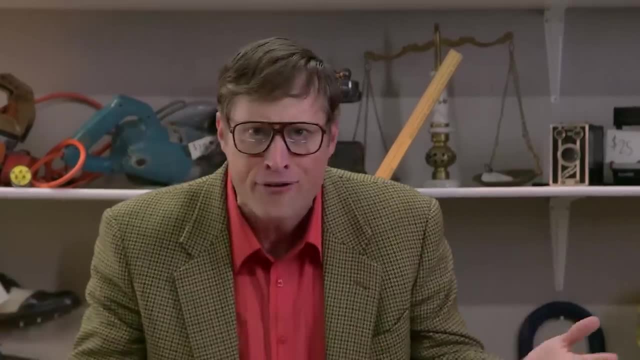 You want to make a catapult, Use a spoon. The place where the spoon pivots is the fulcrum, And now it's a lever. It's a lever, It's a lever. Look at this lamp. Now it's a lever. 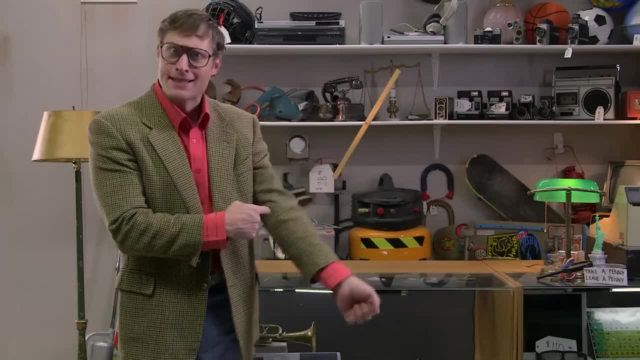 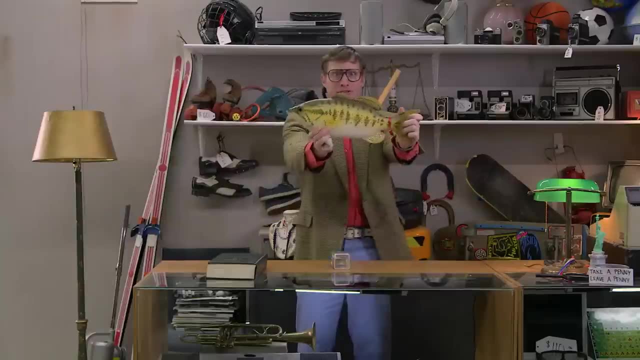 Scissors. two levers. Your forearm it's a lever. Two ends and the fulcrum where it pivots. Yeah, the fulcrum can be at one end. Crazy, This fish. you guessed it. Now it's a lever. 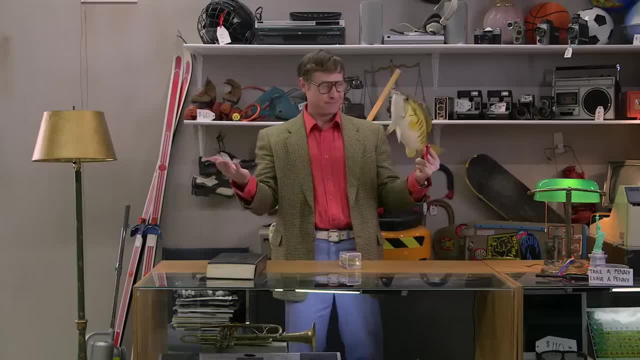 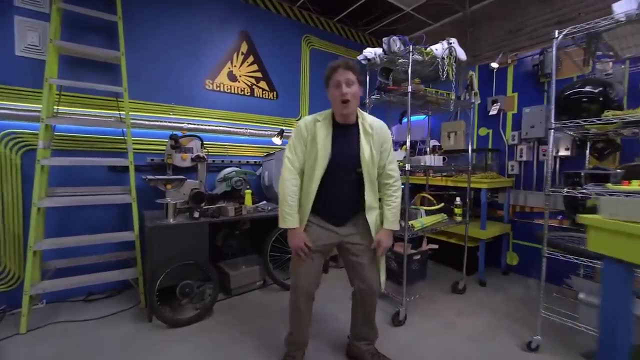 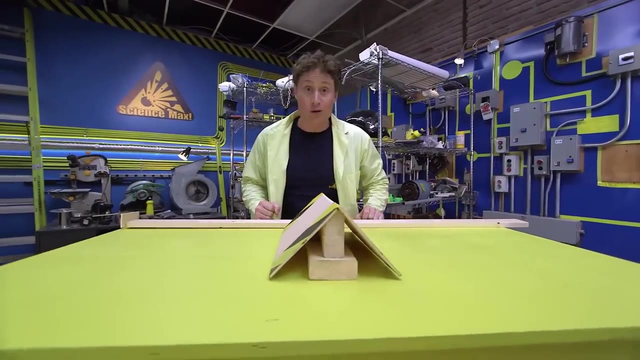 It's a lever. It's a lever. And now you know your levers. Okay, Where were we? Oh yeah, levers. So you can use levers to become much stronger or at least lift something you couldn't normally lift. 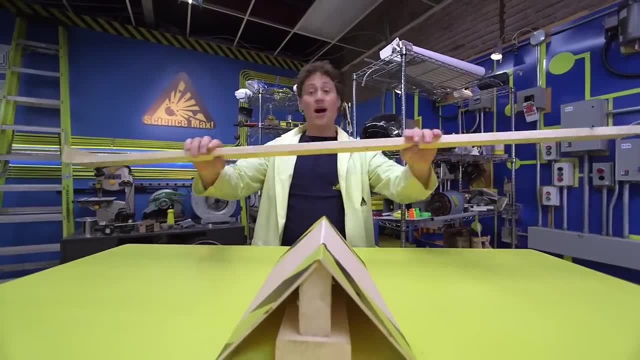 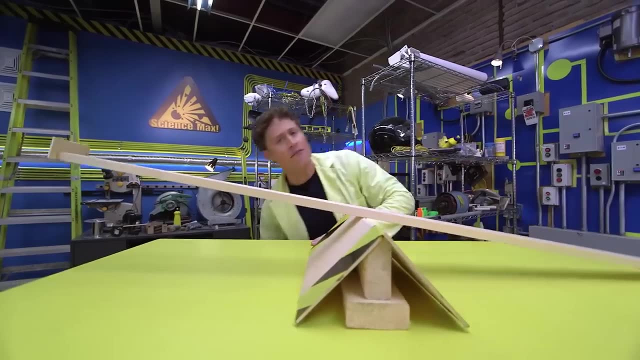 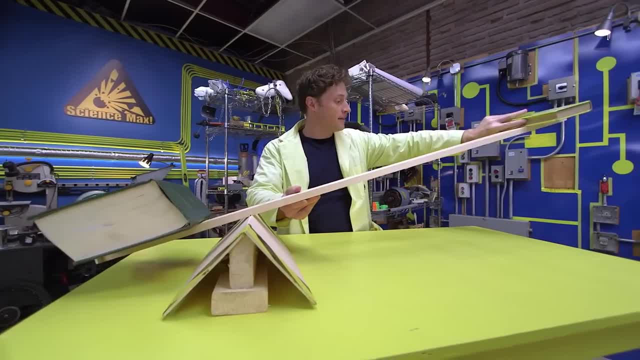 the other book. But watch what happens when I move the fulcrum. But watch what happens when I move the fulcrum. But watch what happens when I move the fulcrum. Mm-hmm, mm-hmm. move the fulcrum, Mm-hmm, mm-hmm. move the fulcrum. Mm-hmm, mm-hmm, Huh, Mm-hmm, mm-hmm, Huh, Mm-hmm, mm-hmm, Huh. It's like magic, but it's not magic. Huh, It's like magic, but it's not magic. Huh, It's like magic, but it's not magic. It's science. It's like magic, but it's not magic, It's science. It's like magic, but it's not magic, It's science. Whoa. 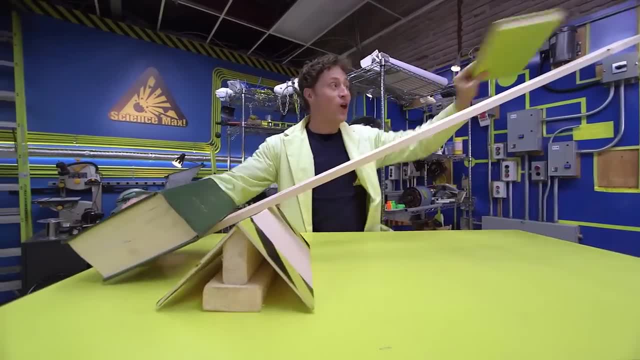 It's science, Whoa, It's science, Whoa. It's because the small weight is Whoa. It's because the small weight is Whoa, It's because the small weight is moving a long distance, and the It's because the small weight is moving a long distance and the It's because the small weight is moving a long distance and the heavyweight is moving a short. moving a long distance and the heavyweight is moving a short. moving a long distance and the heavyweight is moving a short distance. heavyweight is moving a short distance. 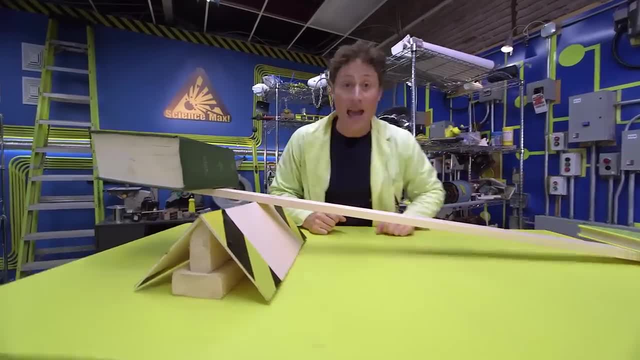 heavyweight is moving a short distance: Small weight- long distance distance. Small weight- long distance distance. Small weight- long distance. Heavyweight short distance. Small weight- long distance. Heavyweight short distance. Small weight long distance, Heavyweight- short distance. So everything balances out. 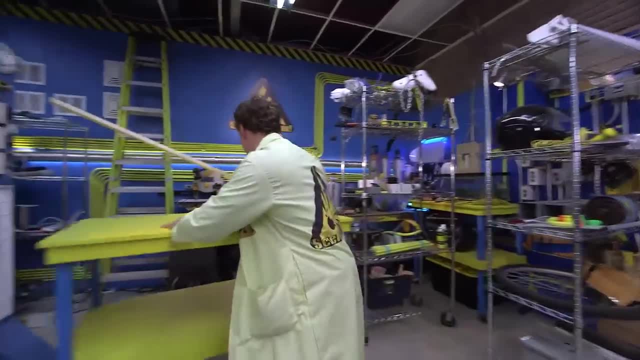 Heavyweight short distance, So everything balances out. Heavyweight short distance, So everything balances out, But here's where it gets interesting. Heavyweight short distance, So everything balances out, But here's where it gets interesting. 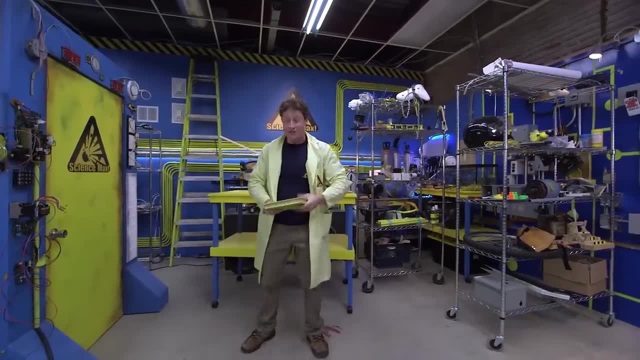 So everything balances out. But here's where it gets interesting. So everything balances out, But here's where it gets interesting. The longer your lever, But here's where it gets interesting. The longer your lever, But here's where it gets interesting. The longer your lever, the more weight you can lift. 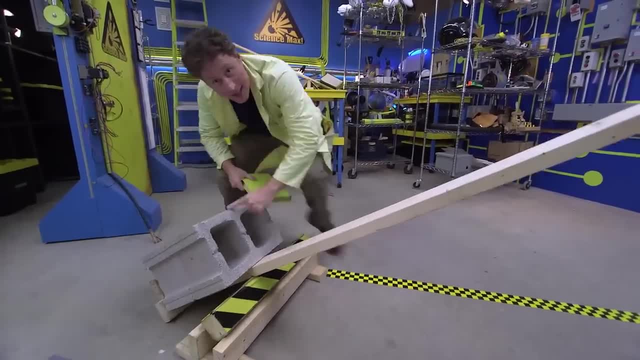 The longer your lever, the more weight you can lift. The longer your lever, the more weight you can lift. These are two heavy cinder blocks. the more weight you can lift- These are two heavy cinder blocks- the more weight you can lift. These are two heavy cinder blocks. There's the fulcrum and here is 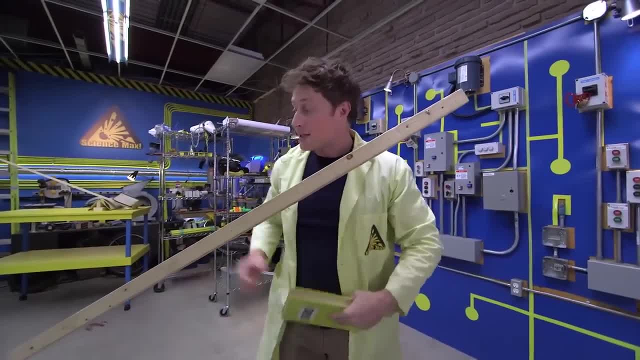 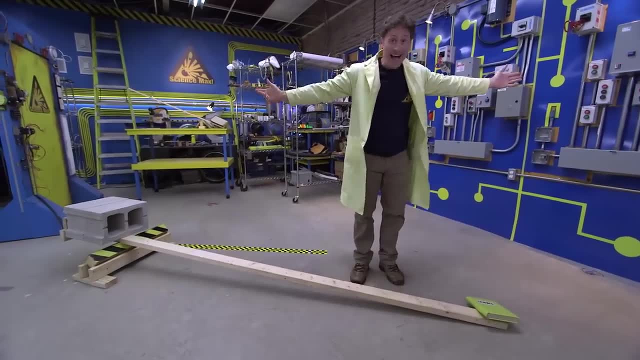 These are two heavy cinder blocks. There's the fulcrum and here is a very long lever with which I am going to lift those cinder blocks with this book. And there you have it Levers. Now back to the Particle Impulse Controller. 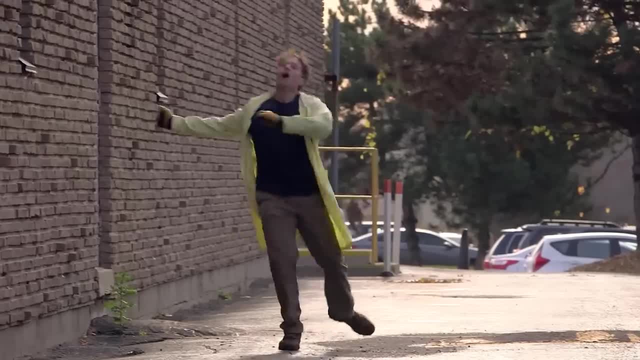 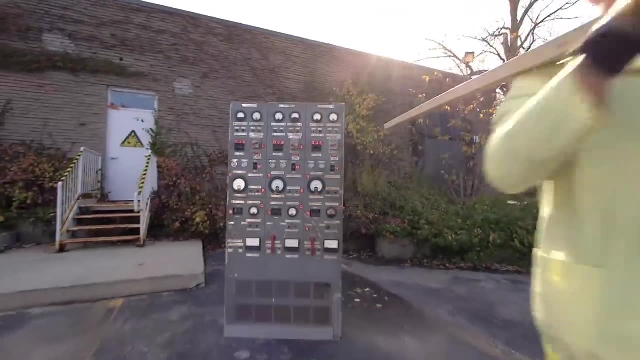 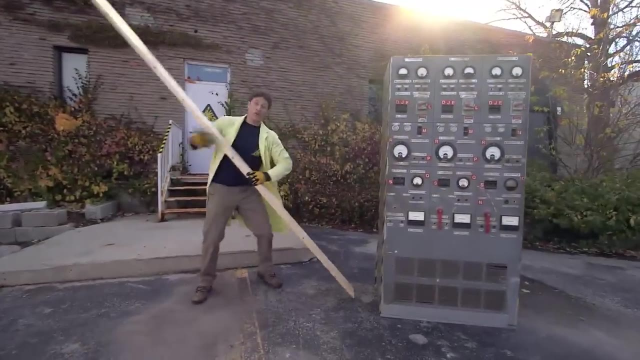 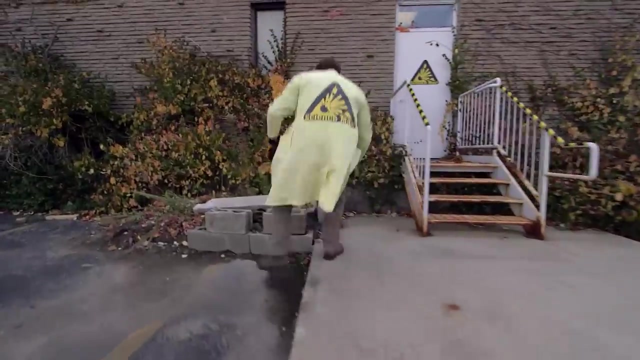 Oh right, Ah, lever, Here we go. I got my giant lever. The bigger the lever is, the easier it is to do the work. I need a fulcrum. Oh, Just about anything will do for a fulcrum, And put that there. 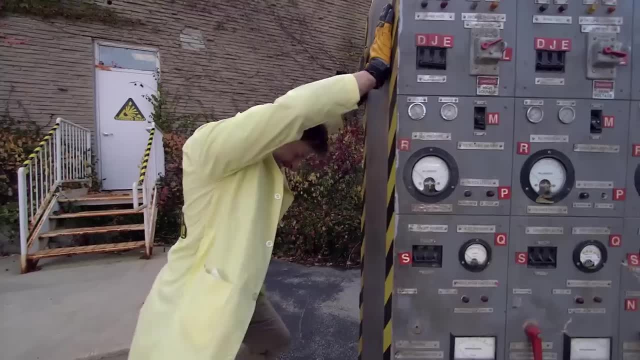 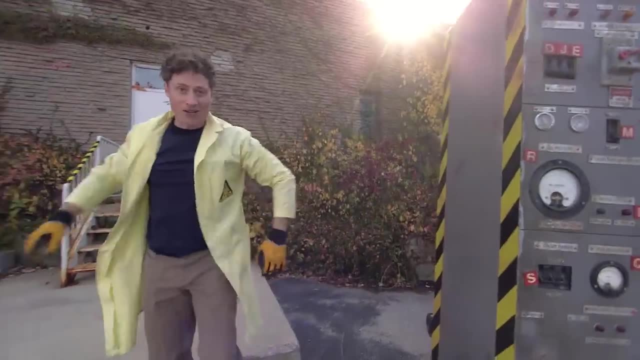 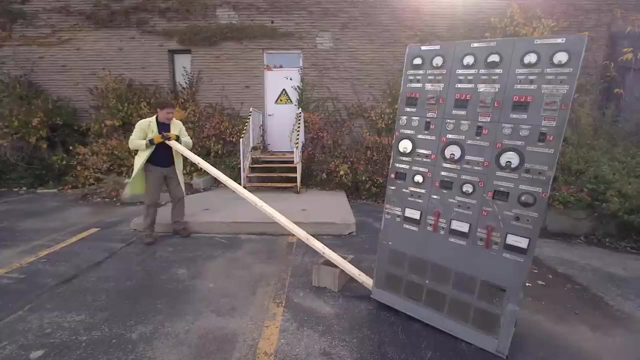 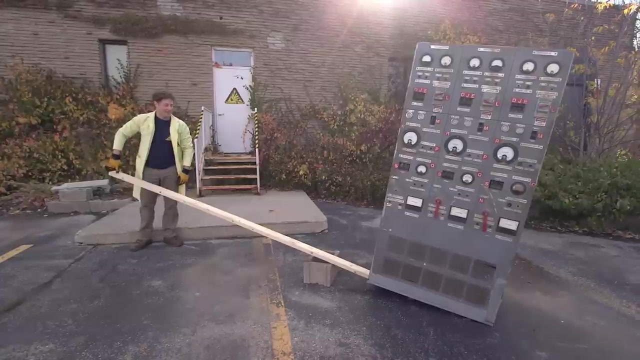 Now the hardest part is getting it on the lever. Alright, hardest part is over. Get the lever up on the fulcrum And Look at this. No problem, One finger lifting. It suddenly became very easy for me to move this. 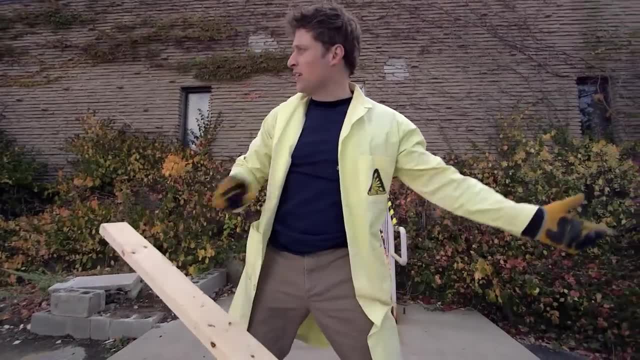 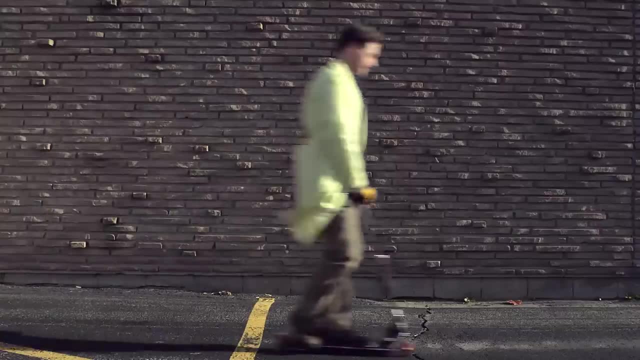 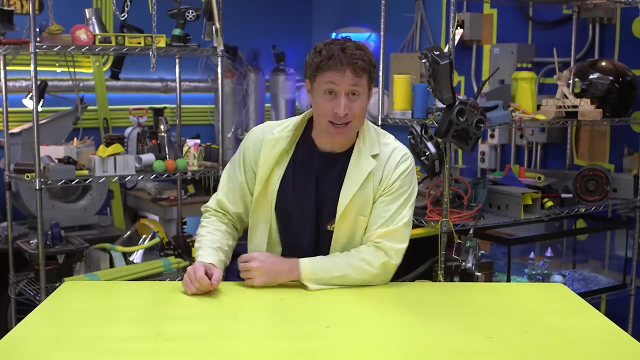 I guess I need to do more than just lift it, though huh, Because I have to move it all the way. Oh, Rollers, Come on back to the lab. Okay, Rollers, Rollers are like wheels, except they're not attached to anything. 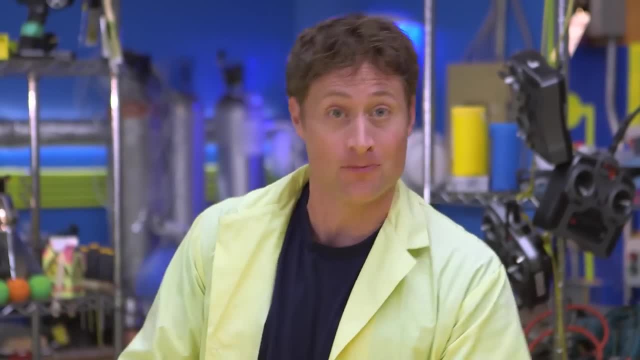 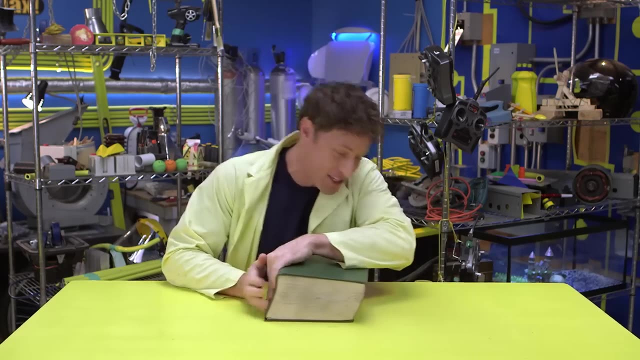 In ancient times they used to move giant, heavy blocks of stone using rollers. We can demonstrate using a book. Now get a book, put it on a table and try to move it across the table. You'll see that it's very difficult. 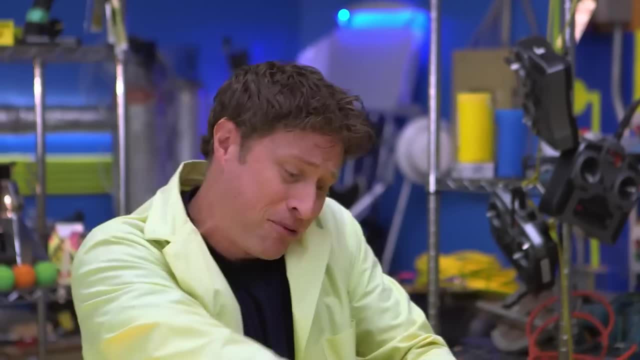 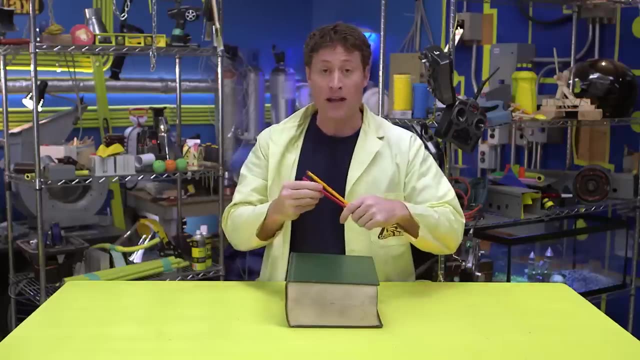 I can't move this book across the table. I can't. Okay, it's not really that hard, But still it takes effort. But if we get some rollers, I like to use pencil crayons and not pencils, And here's why Take a closer look. 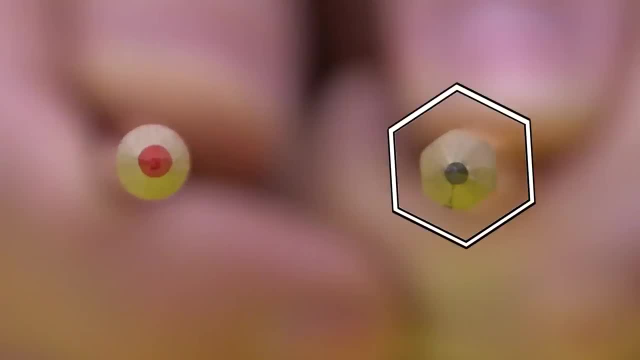 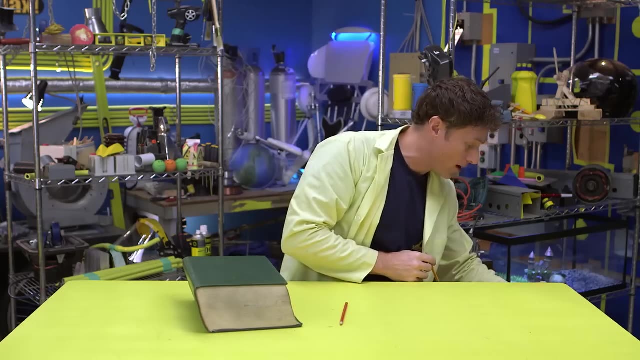 You see, pencils aren't round, They're hexagonal, They have six sides, Whereas pencil crayons are round, And, of course, if you want something to roll, you want something round. So get a bunch of pencil crayons and put them on the table. 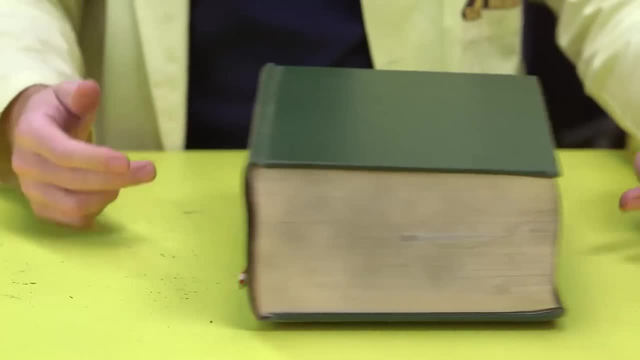 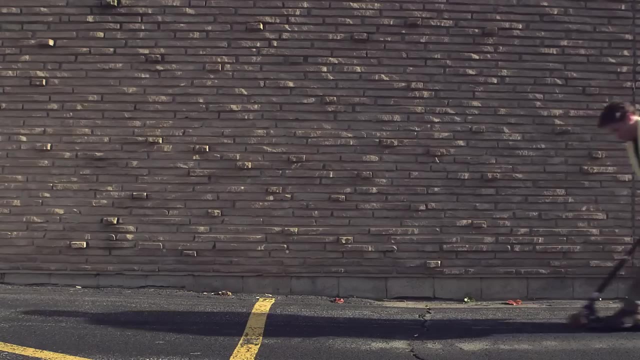 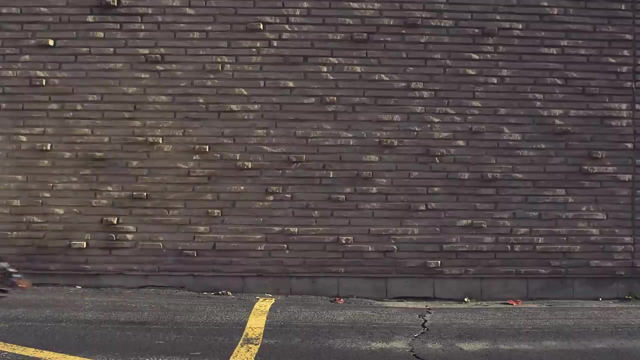 And put the book on the pencil crayons And you'll see that suddenly moving it is a lot easier. All right, That's rollers Back, I go. Now it's time for Science. So Simple A Caveman Could Do It. 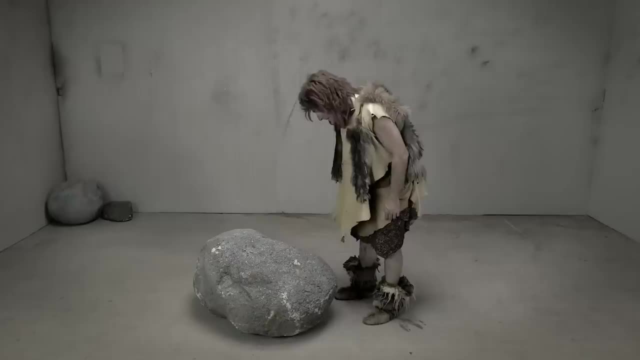 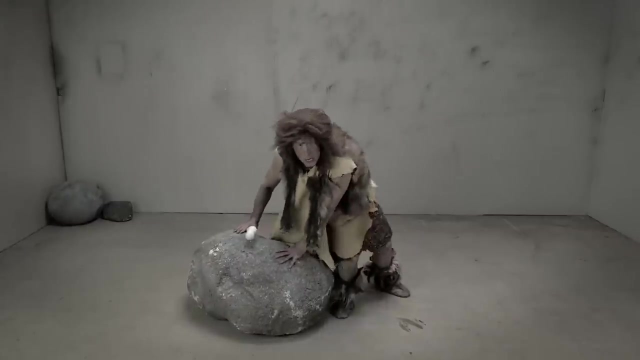 This is a caveman, This is a rock. It is a well-known scientific fact that if this caveman were to try to move that rock, he would not know how to do it easily. Poor caveman. But in ancient times people learned how to move heavy rocks using ropes. 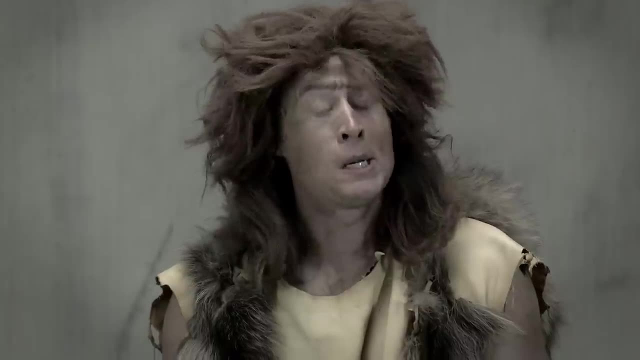 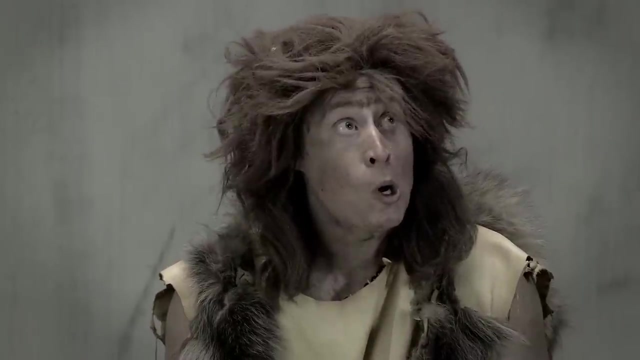 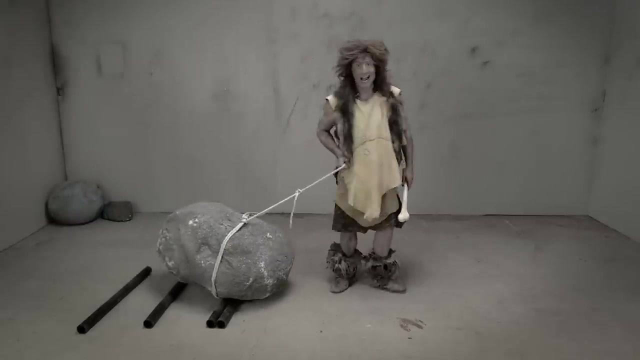 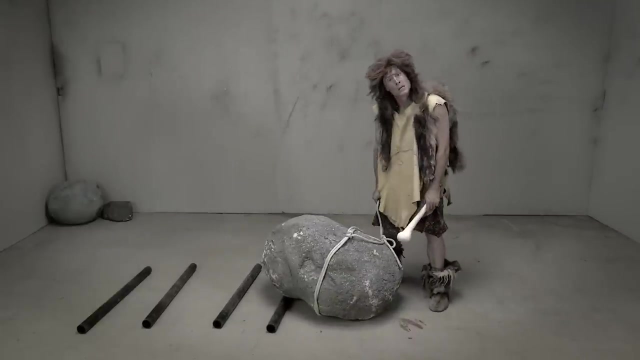 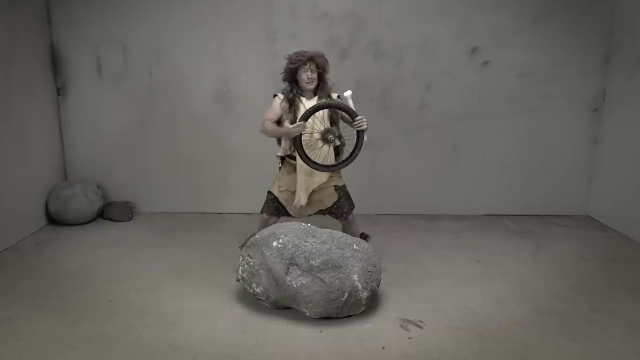 and rollers, Rollers- Yes, Rollers, Rollers, Rollers- Close enough. Rollers make it much easier to move a heavy object, But they aren't perfect, So the wheel was invented. The wheel is a simple machine and one of mankind's greatest inventions. 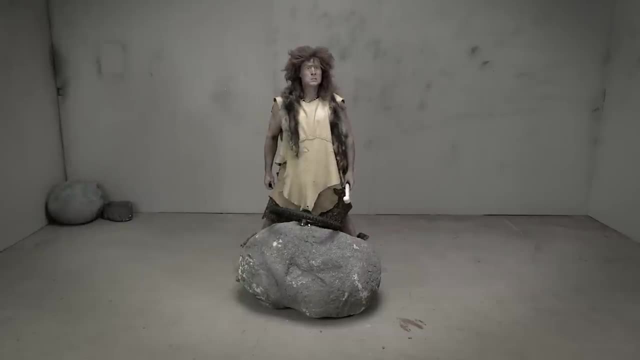 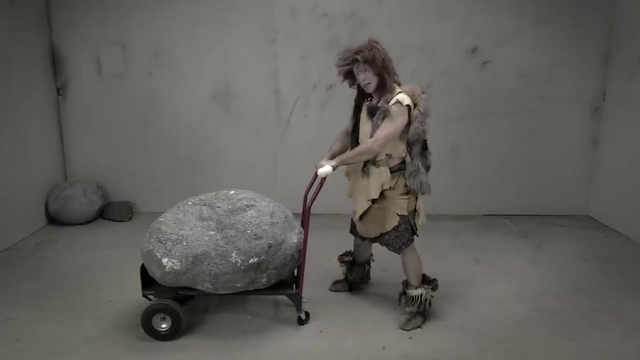 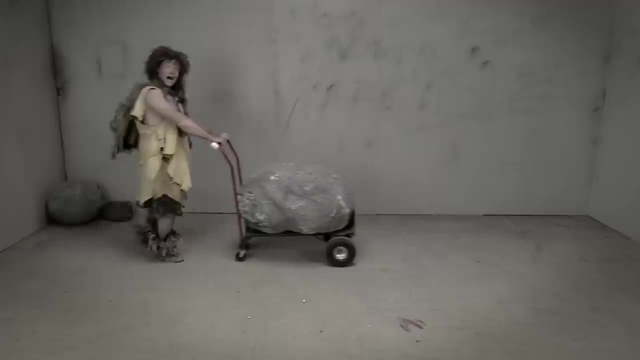 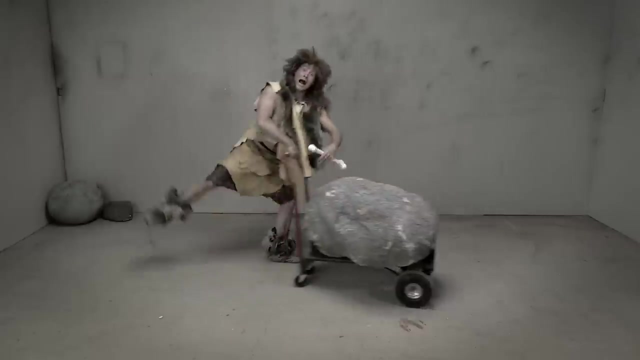 But no, that's not how it works. Wheels go on axles which go under a platform. Now you have something to place that heavy rock on to move it around. But all these great inventions came after the time of the caveman. 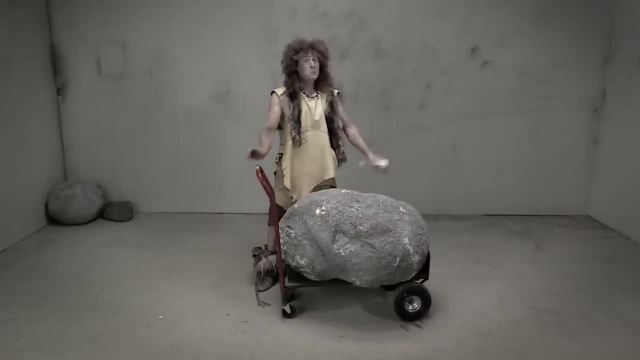 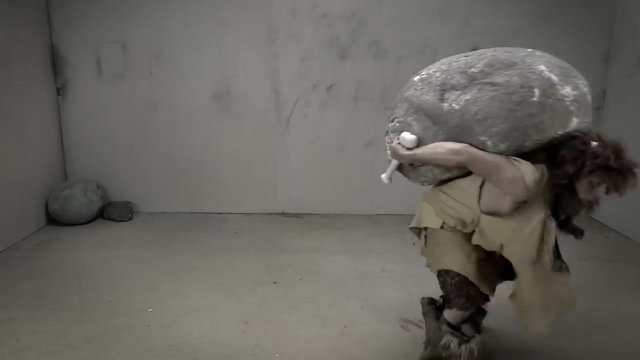 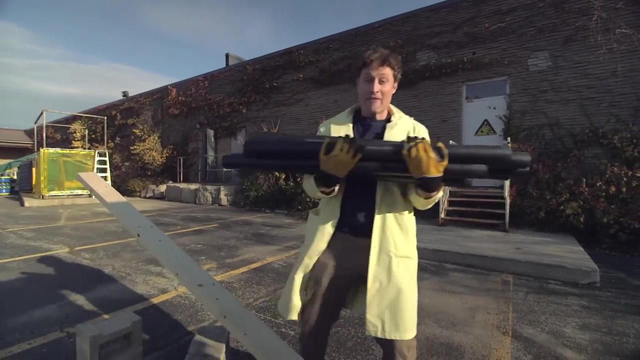 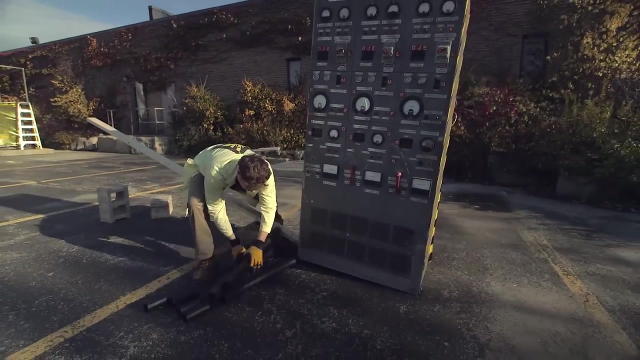 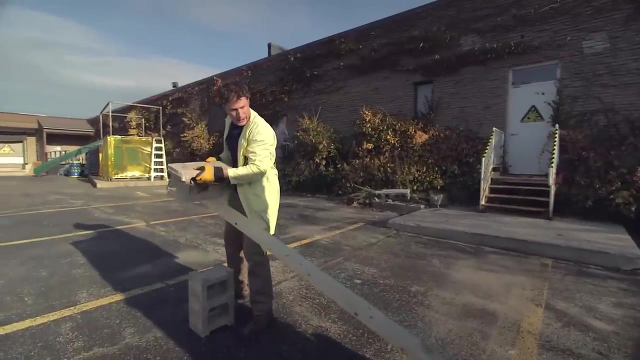 Caveman had to do everything the hard way. Join us next time for more science. Okay, I've got rollers. They're just plastic pipes, but they'll work perfectly. I put them here And now to lift up the machine- Perfect. 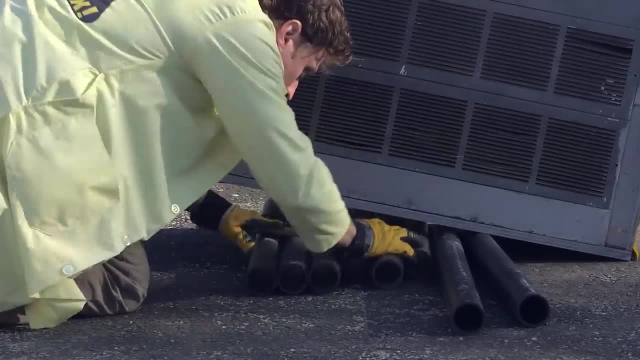 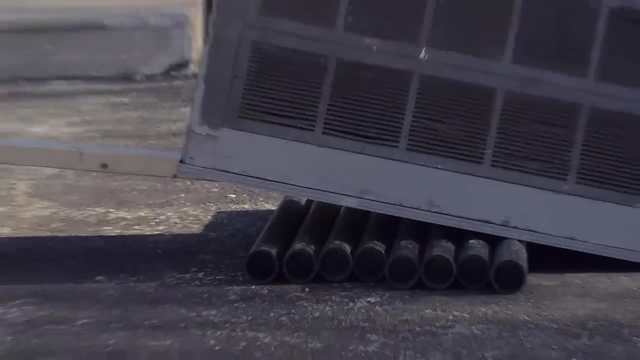 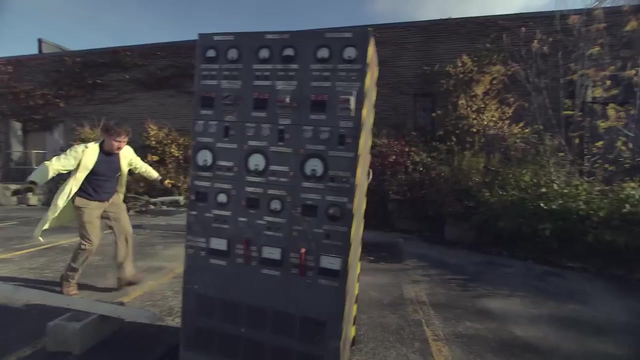 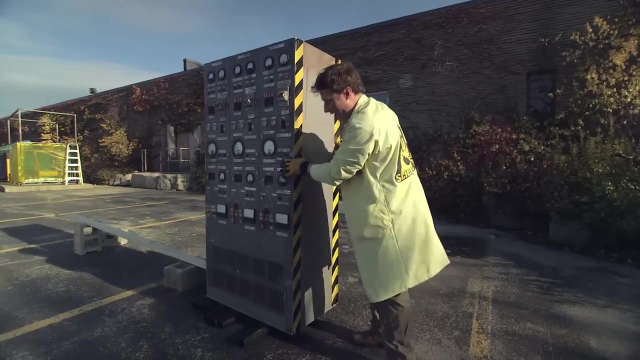 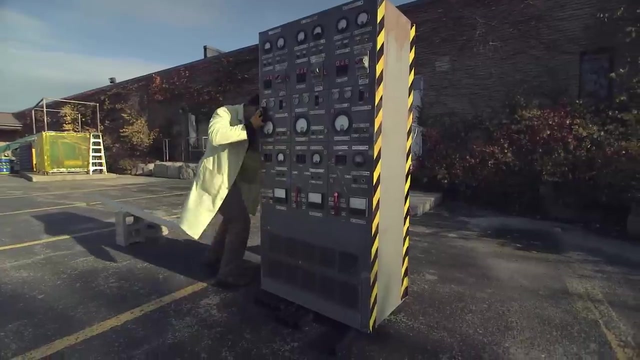 And so the rollers go underneath like that. And then Whoa, Whoa, Careful, Uh-huh, Look at that, No problem. Wait, I've got to get rid of this. Get it Moving Now. the trick with rollers is you have to keep taking them out of the back and putting. 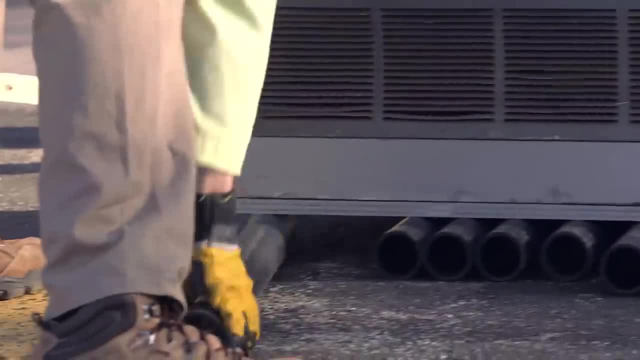 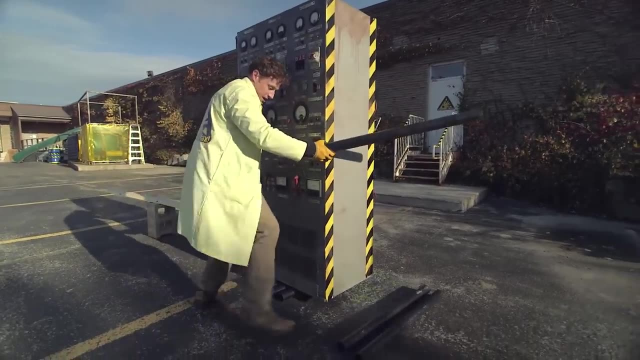 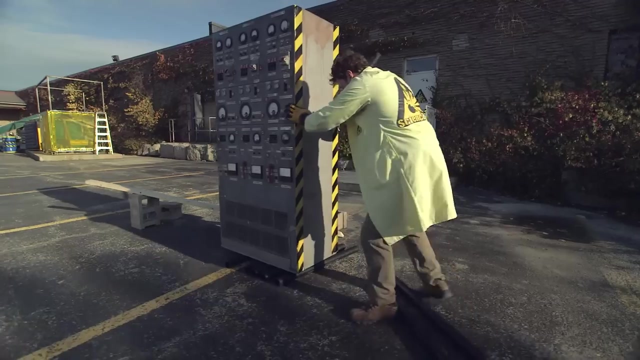 them in the middle. But Whoa, Whoa, Whoa, It's Stop, Rollers, Stop, Oh no, Oh no, Okay, Okay, Whoa, Rollers, Easy, There we go, Okay. 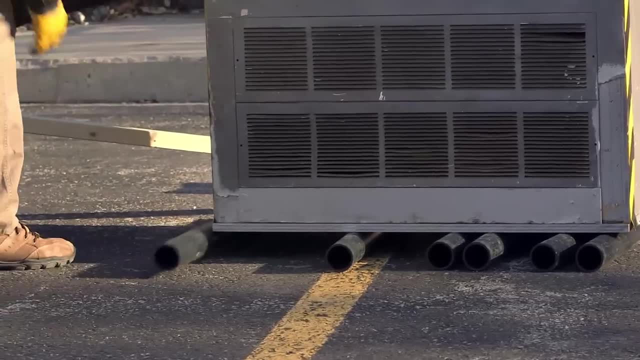 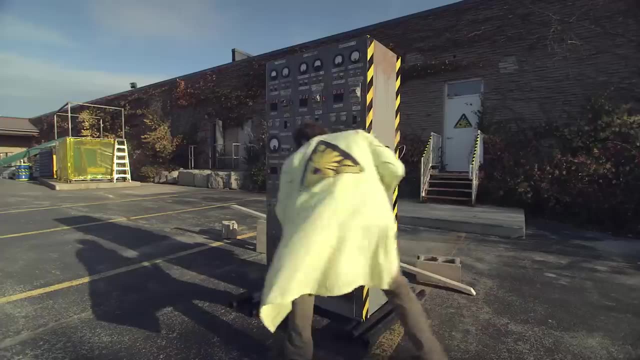 In the front, Roll it forward. Now I know what you're thinking. You're thinking this seems like a lot of work, And it's true: It's a lot of work. Moving the rollers back and forth and back and forth does take some time. 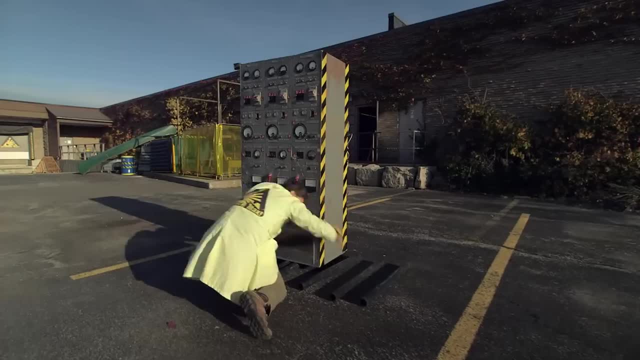 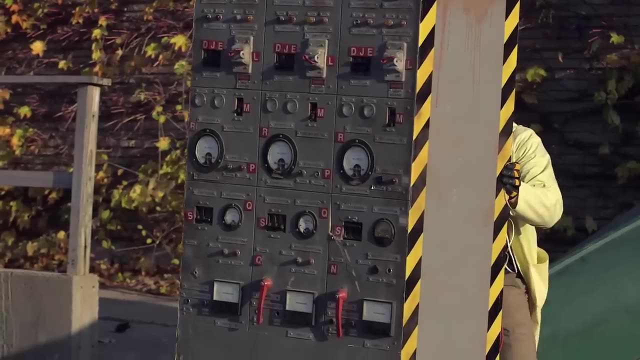 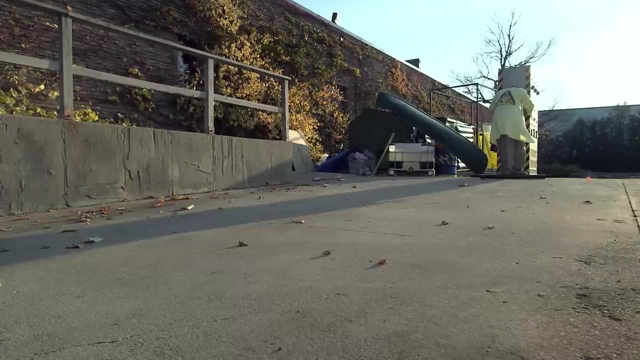 But did you know? this was how the pyramids were built. It's true, Giant stone blocks were moved on rollers, just like I'm doing here, And, as you can see, what worked for the ancient Egyptians works for me too, Uh-oh. 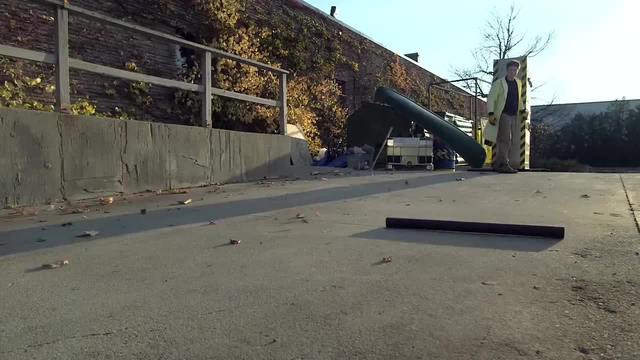 Yeah, There is a hill here. If I go down the hill it's gonna start rolling faster than I can do the rollers. I'm gonna need some help. Oh, I know, Pulleys, pulleys, pulleys. Okay. 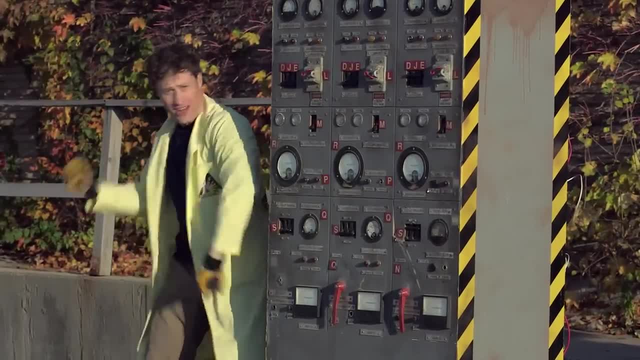 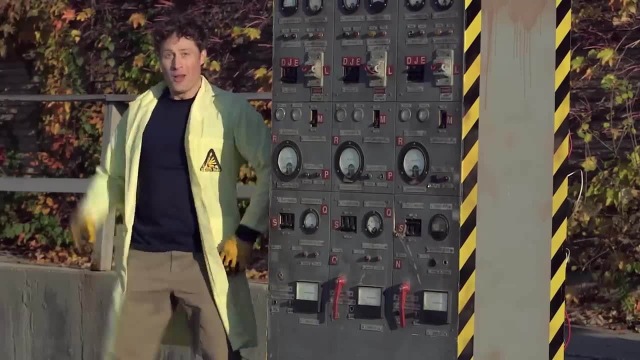 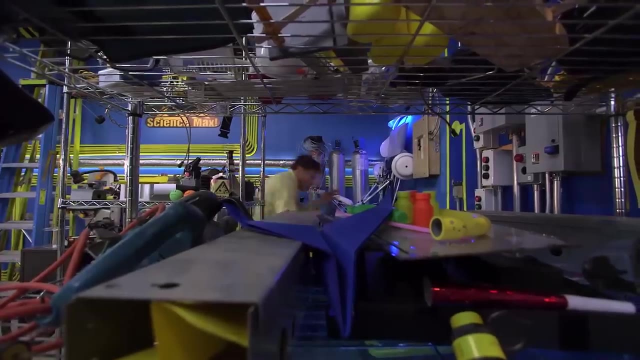 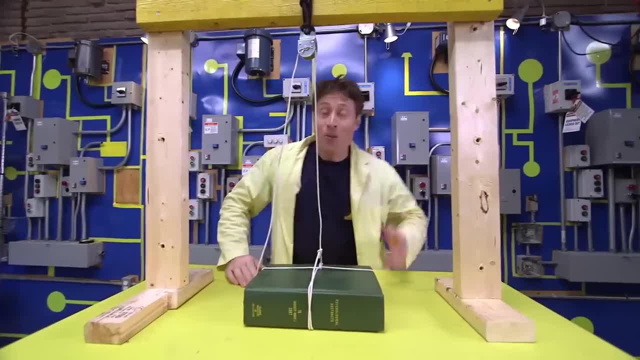 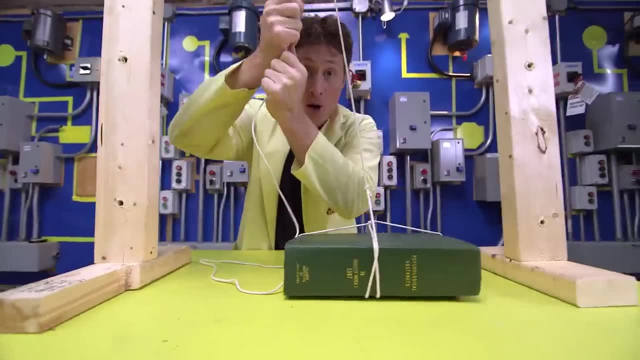 Pulleys, Pulleys, Pulleys, Pulleys are a great way to change the direction of force. I've got a rope going through this pulley and down to a book, So when I pull the rope down, the book goes up. 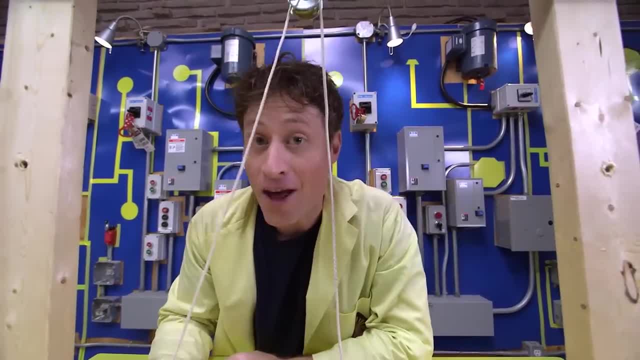 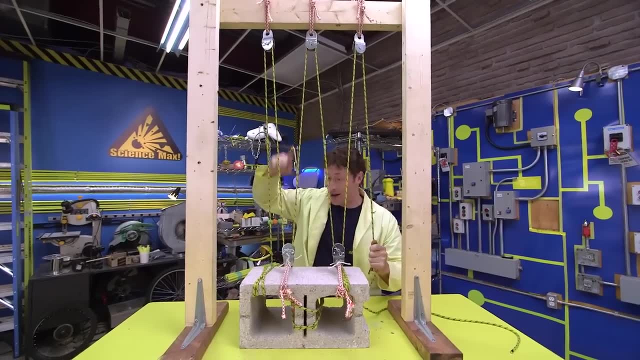 Changing the direction of force can be very helpful, but pulleys can be helpful in another way. Pulleys can let you lift something that you couldn't normally lift. Now the rope goes up and down, and up and down, and up and down, and the force I need to lift 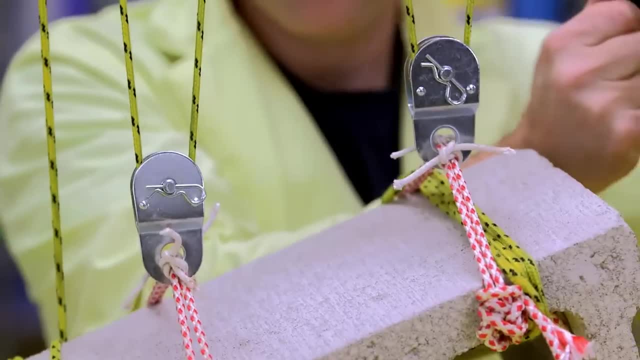 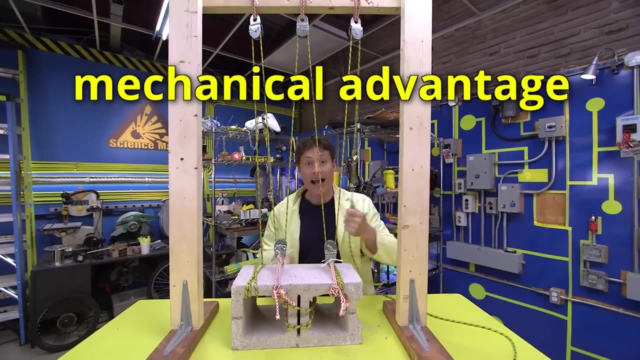 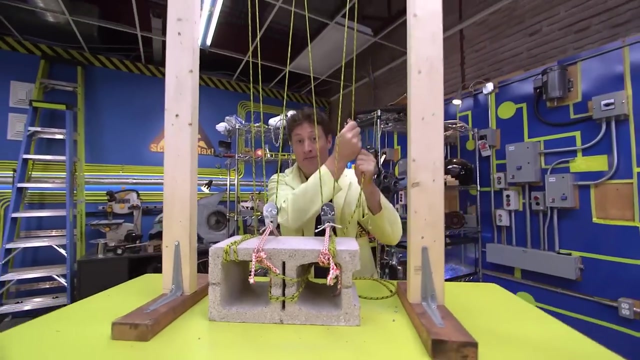 this cinder block is a lot less than if I was just lifting it by myself. I've got to pull a lot more rope. That's called mechanical advantage: spreading out the force over a longer pull so you can lift a larger weight. If you use more pulleys, it reduces the amount of force. 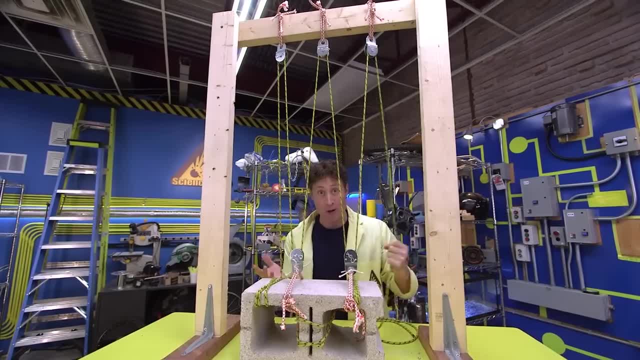 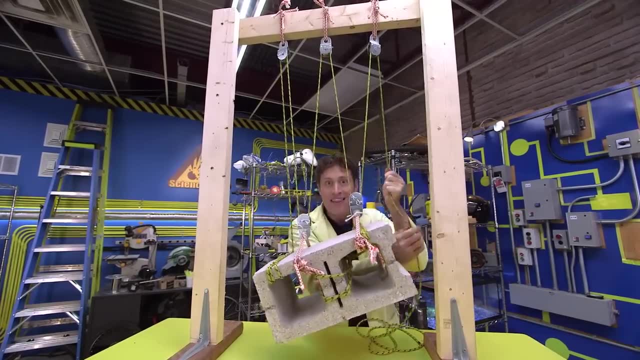 One pulley, same amount, Two pulleys half the force, Three pulleys, one third. So I've got five pulleys here, which means I only need one fifth the force to lift this cinder block. So there you go, pulleys. 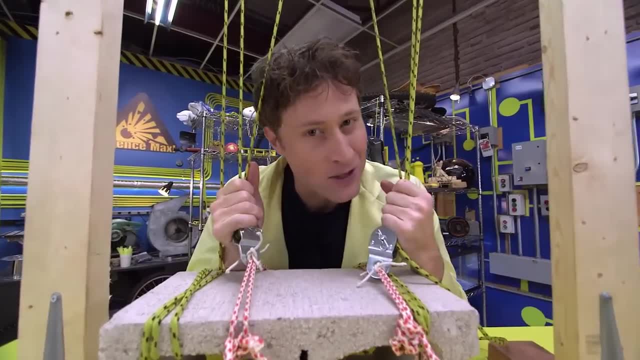 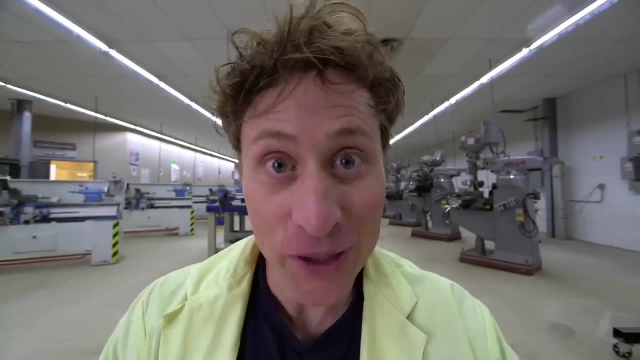 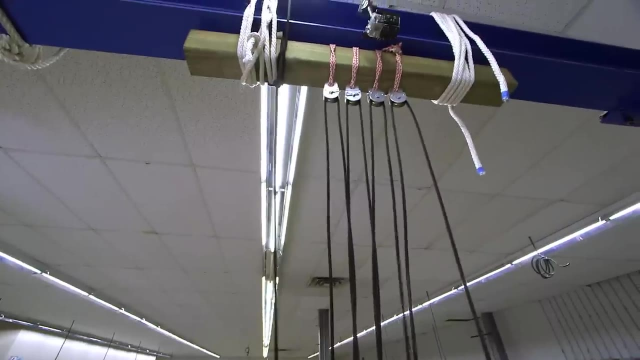 Now back to the Wait a minute, Wait a minute. This calls for a mini-max. So how much weight can you lift with pulleys? Well, as much as you want, really. I have four pulleys on the bottom and four pulleys at the top. 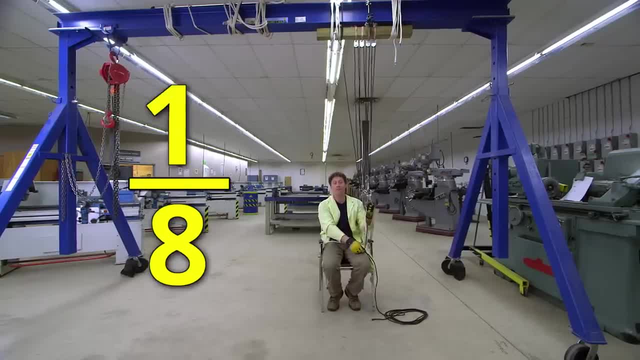 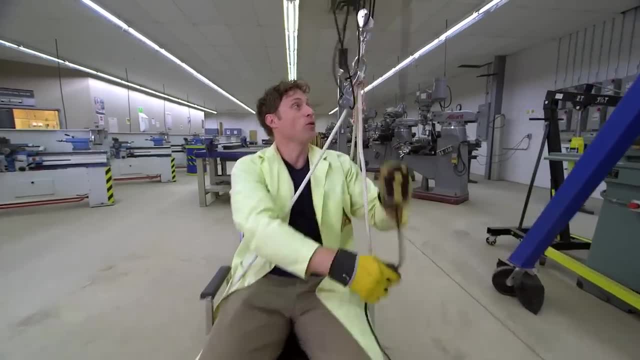 That means with eight pulleys I only have to lift one eighth of my weight plus the weight of the chair I'm sitting in. And if I keep pulling, you will see that the chair I'm sitting in is roped Is roped to the pulleys. 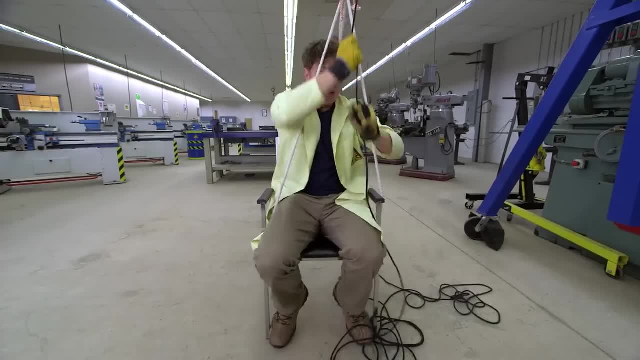 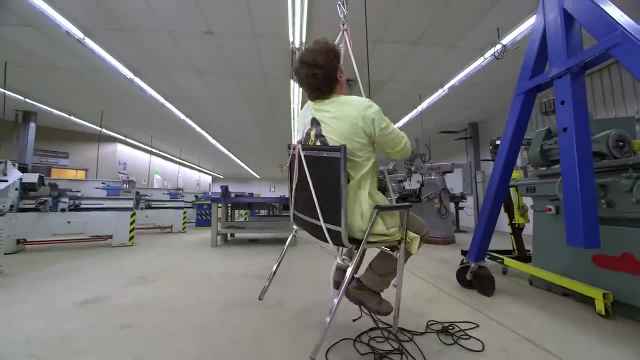 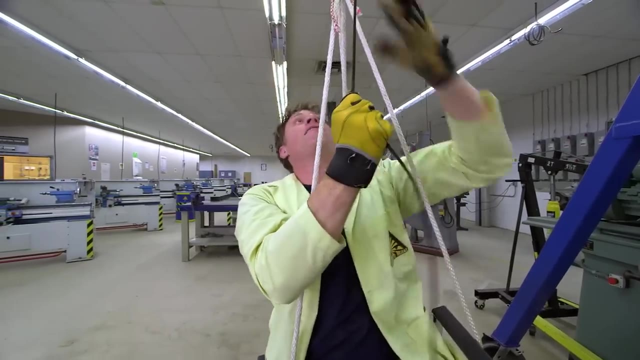 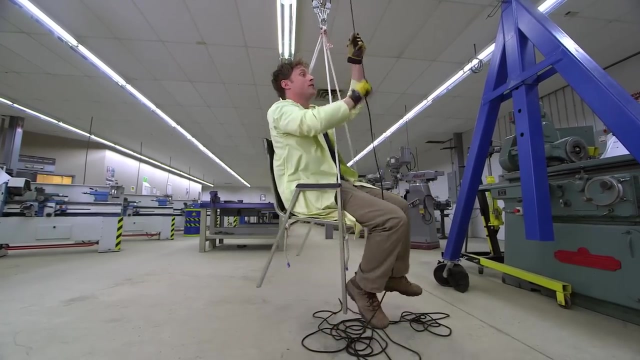 So now we see if I can pull myself up with nothing but pulleys. Look at that. I'm totally lifting myself into the air with the power of pulleys, And I don't need to use two hands. In fact, I only need to use one finger to hold myself up. 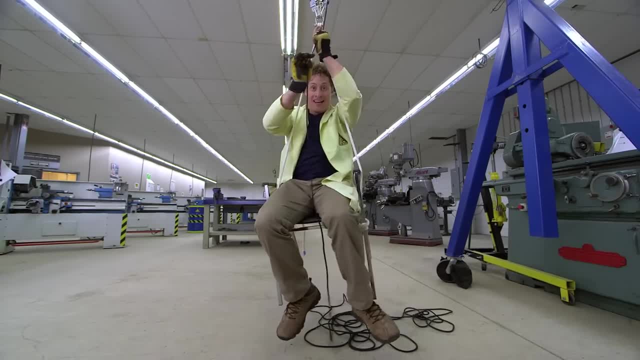 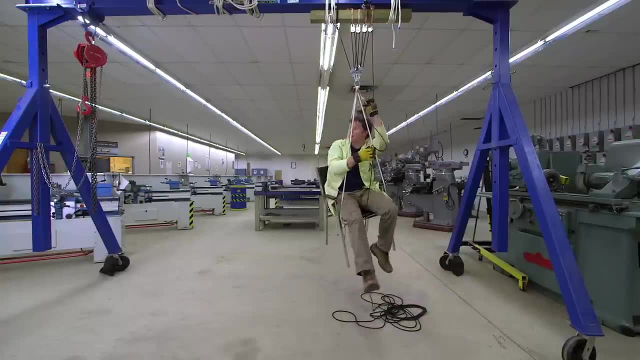 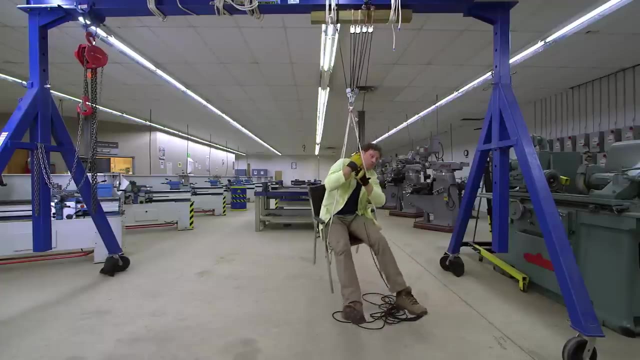 And my thumb, obviously, to hold the rope. That is the power of pulleys. I can almost make myself fly. Well, almost Now back to the particle impulse controller, Letting myself down. Whoa, Whoa, whoa, whoa. 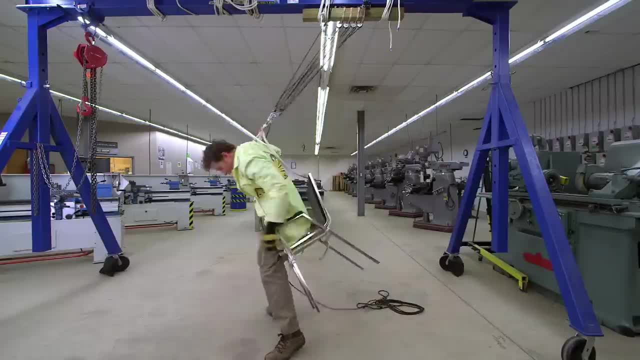 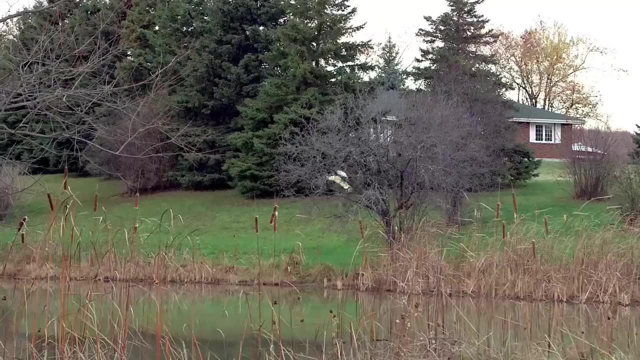 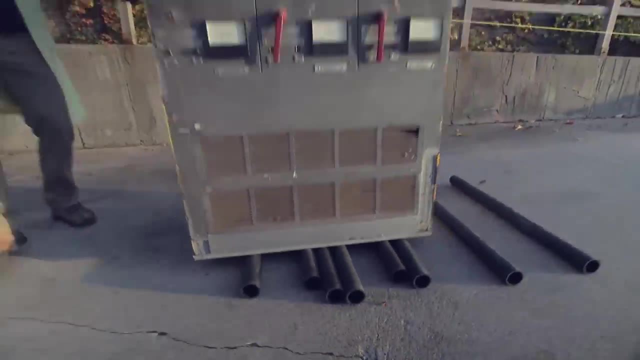 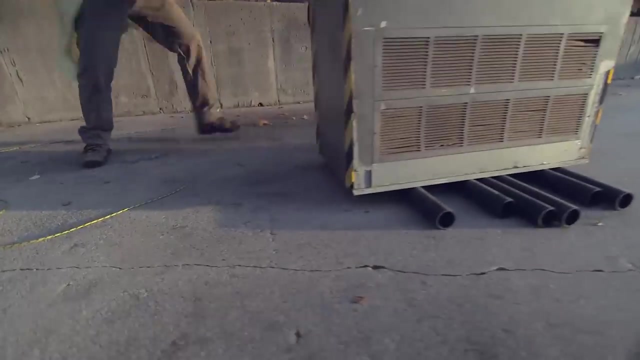 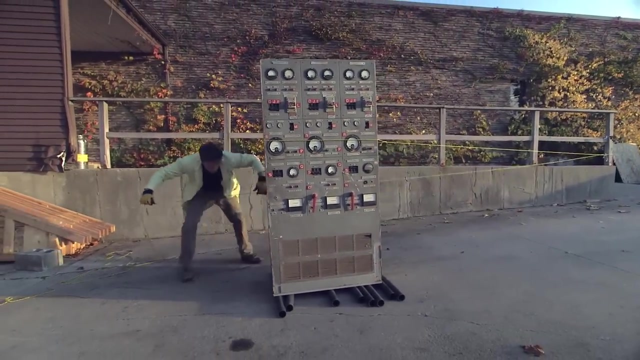 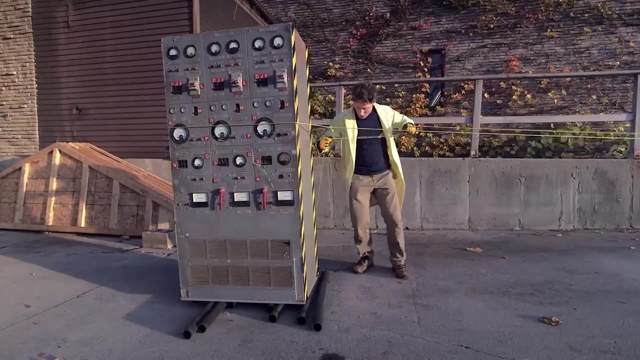 Ah, Particle impulse controller. Let's go, Wait, Okay. All right, I've been able to use this pulley to lower it down the hill at the speed of light, All right. All right, At the speed I want to go. 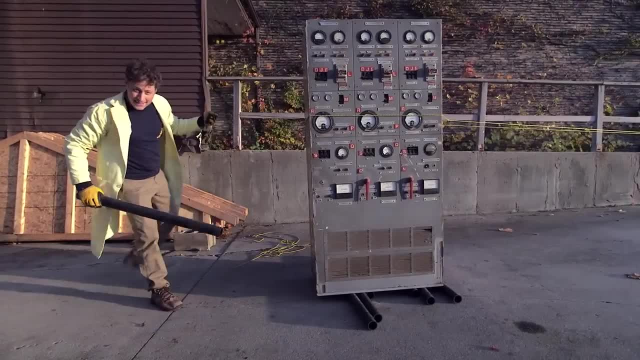 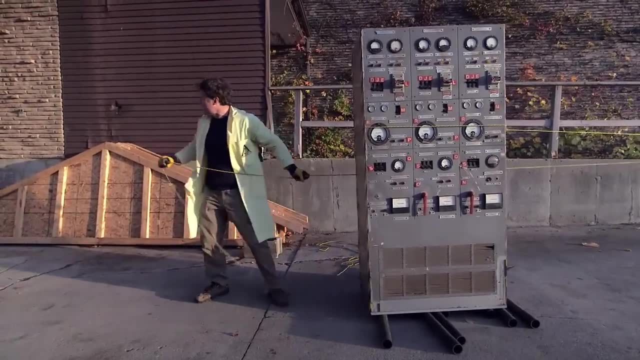 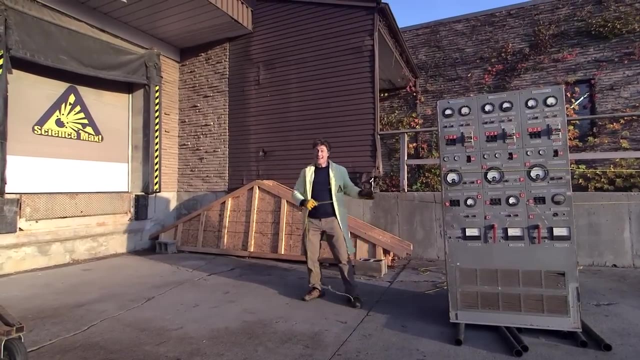 Interestingly, I'm using the pulley, not to make it lighter, but to just change the direction of force, And I managed to get it right here at the bottom. Now I've got to get it up onto the loading dock, So I think this is where I need a ramp. 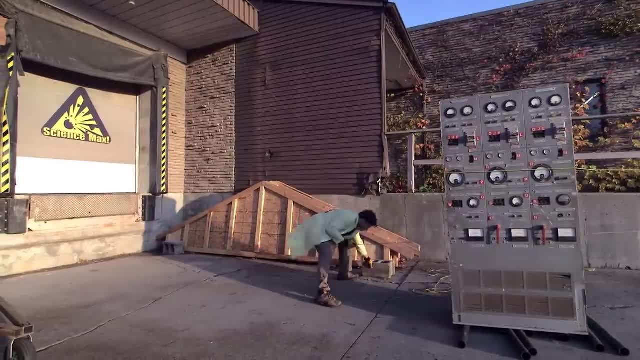 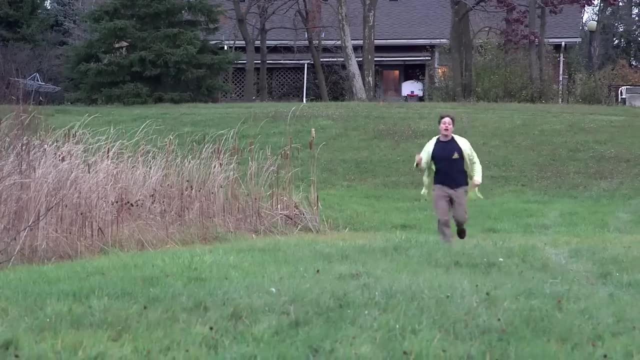 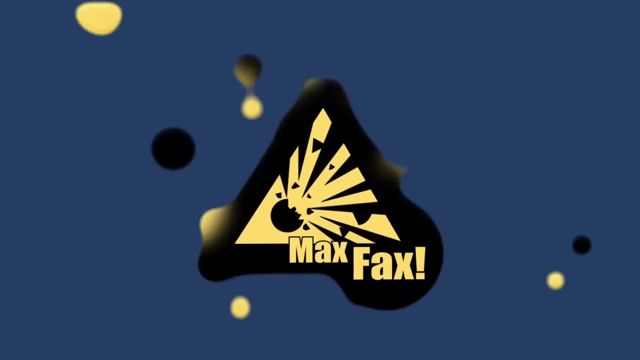 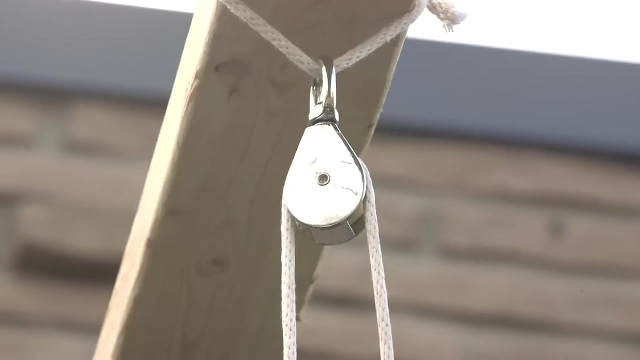 Whoa, Whoa, Oh Yeah, I'm going to try it. Oh No, Here is something mind bending you can do with pulleys. These buckets are attached to the table through a pulley. There's nothing holding this table up, except for the weight of the buckets pushing down. 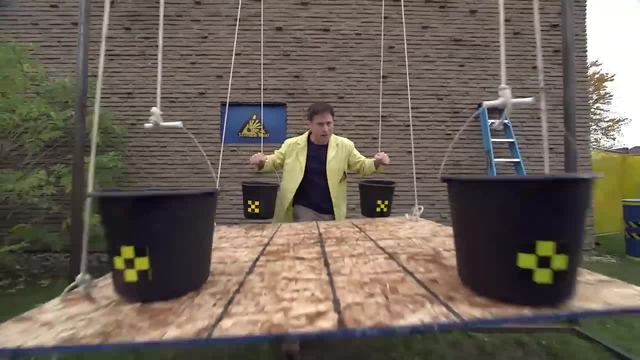 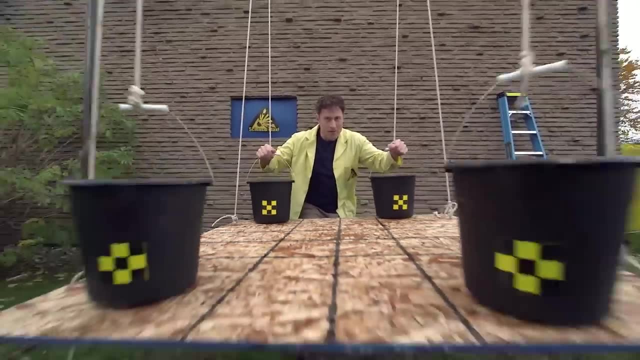 on the table. So if I took the buckets off the table, the weight of the buckets pulls the table, the weight of the buckets pulls the table up, But because the buckets are on the table, everything is in balance. Mind-bending right. 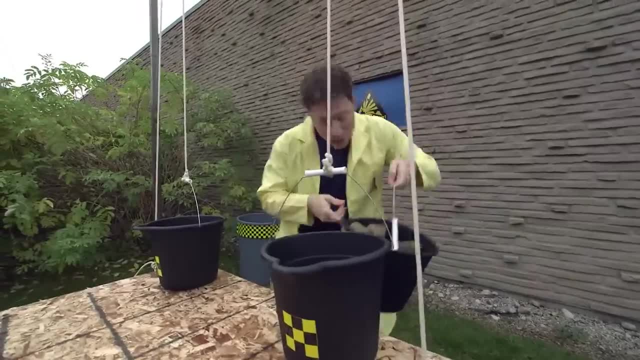 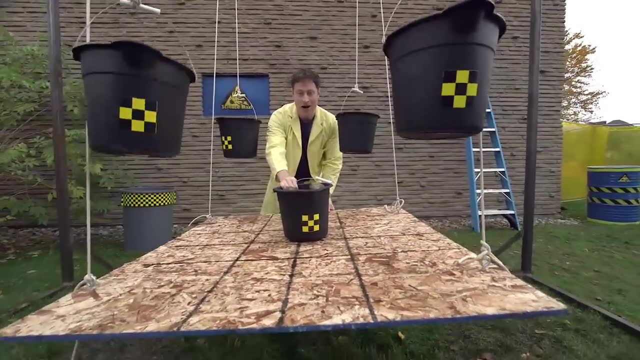 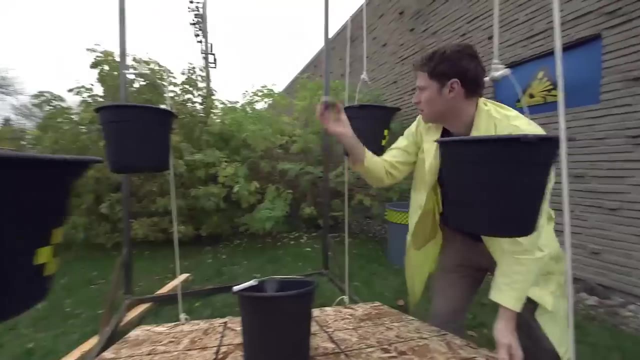 Okay, wait, it gets better. If I took a weight and I put it on the table, the weight of the buckets isn't enough to keep the table up, So I have to add more weight to the buckets, so the buckets pull the table up. 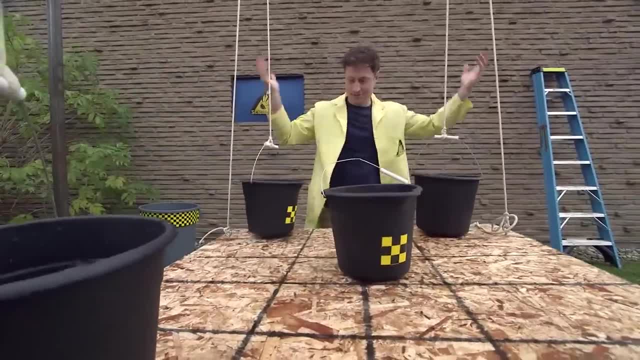 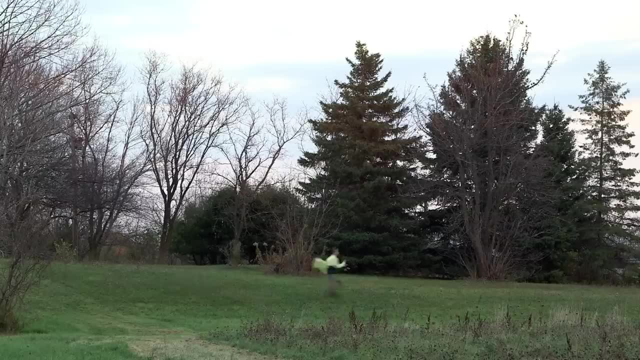 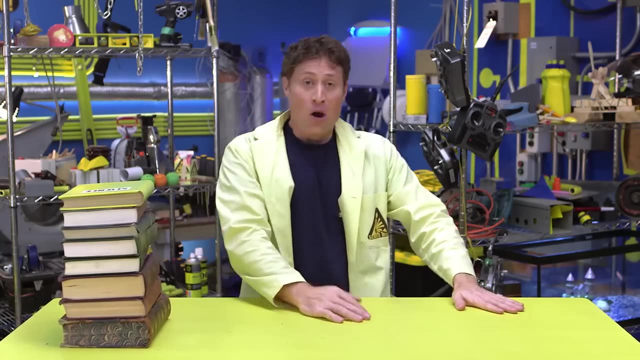 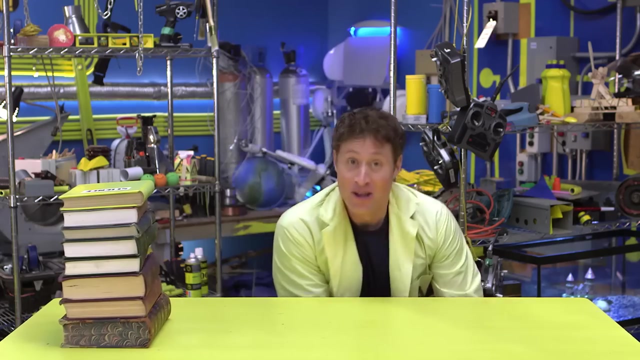 Whoa, And there you have it. It's weird, it's mind-bending, it's science, Okay, okay, Ramps. Ramps are a great way to move something up. I will demonstrate using- you guessed it- a book. 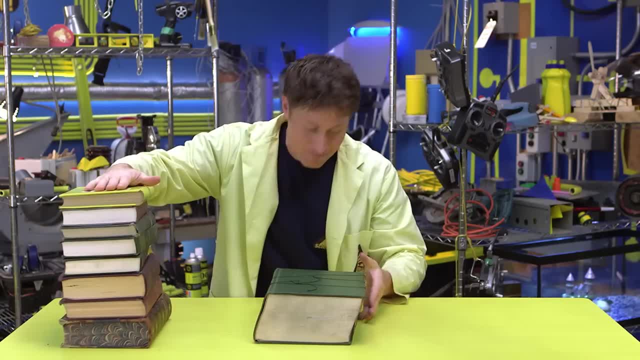 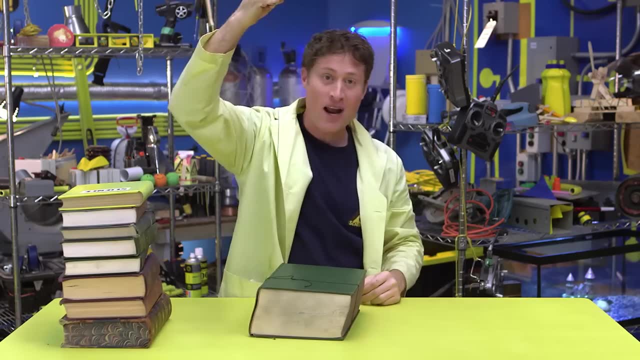 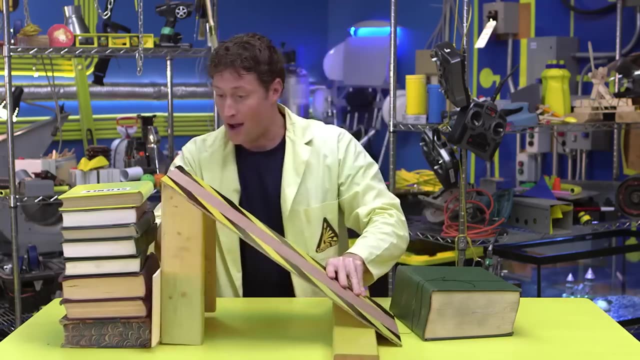 Let's say I wanted to move this heavy book on top of this stack of books using just this little string. Watch what happens: The string breaks. But if I built a ramp to get the book on top of this stack and I use the same kind of string, 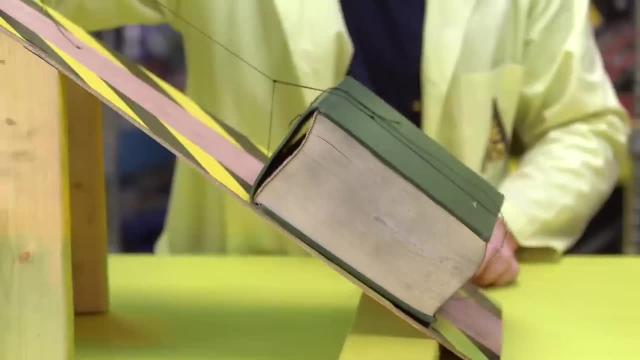 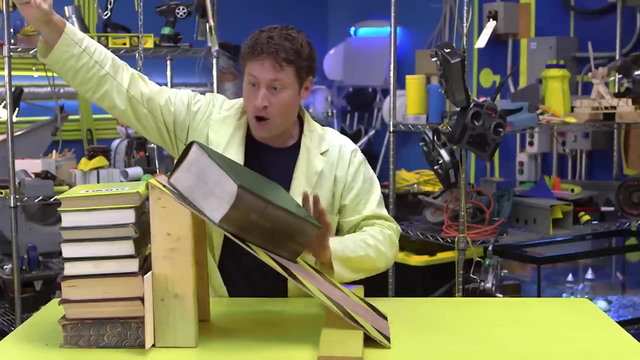 watch what happens this time. Whoa, You see, the ramp distributes the force, so you use less force. so you use less force, so you use less force to pull the book over the same amount of distance and I can get it up to the top of the stack of books. 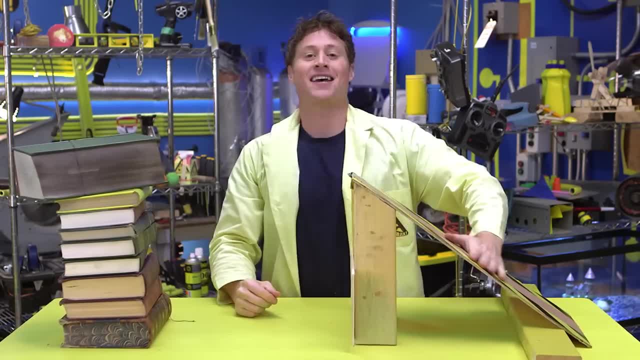 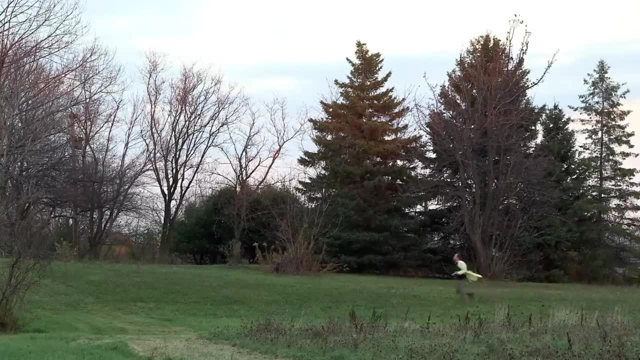 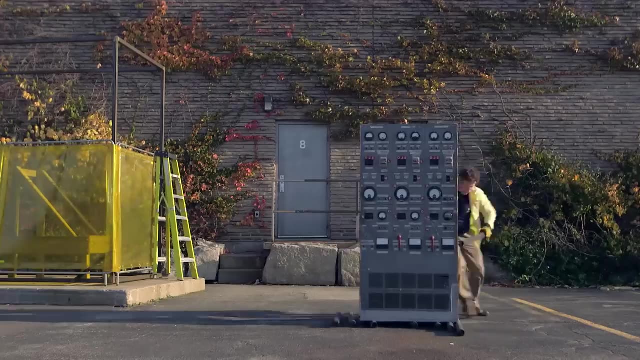 and the string doesn't break. So ramps, Let's put them into action. Whoo, My simple machines have worked great. I've managed to get the particle impulse controller all the way to the loading dock. But now it's time for the hardest job. 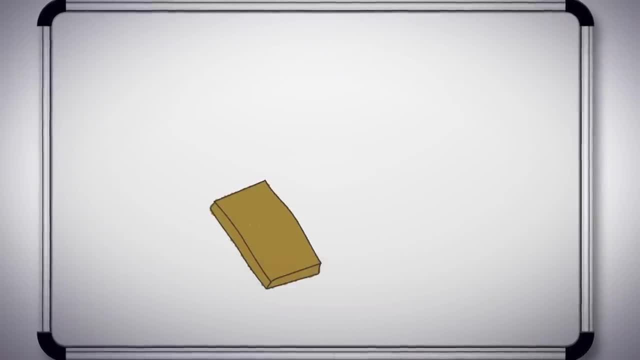 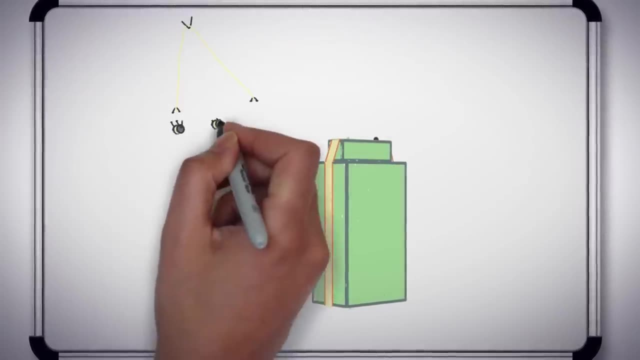 What I need to do is build a ramp that goes from the ground up to the loading dock. Then I need to pull the heavy impulse controller up the ramp. The best way to do that is to use a system of pulleys. I have three pulleys on one end. 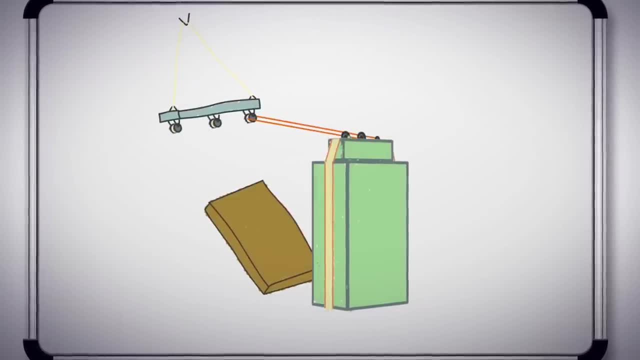 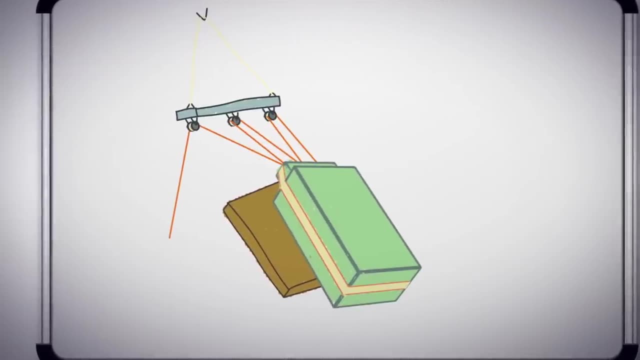 and two pulleys on the controller. Because I have five pulleys working together, I'll only have to lift one fifth of the weight. The plan is to get it tipped over onto the ramp, then use rollers to help it roll up as I pull on the rope. 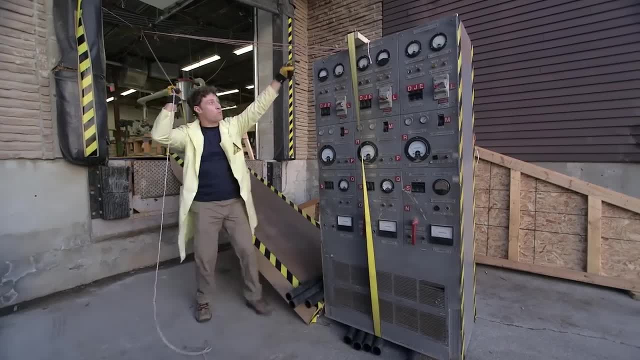 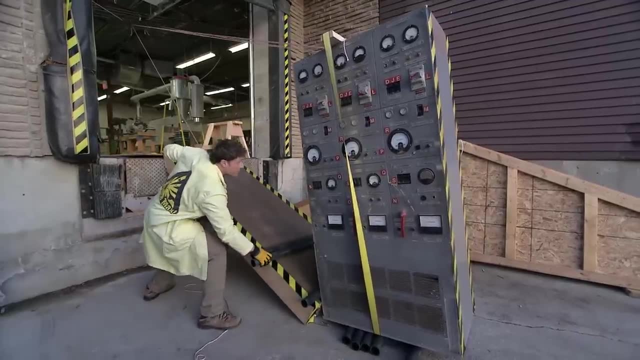 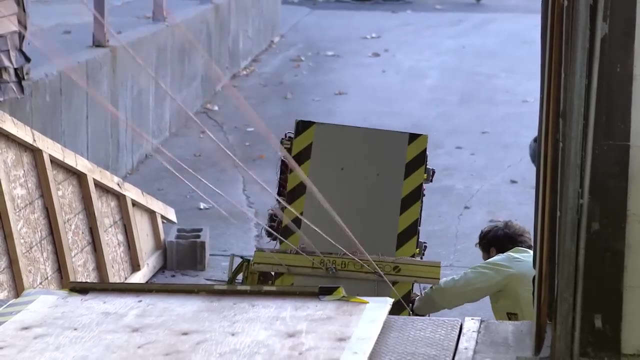 There's three pulleys on that piece of wood over there And I got two pulleys on this piece of wood here And now, if I pull and I carefully put the rollers underneath. Careful, Careful, Perfect, OK. 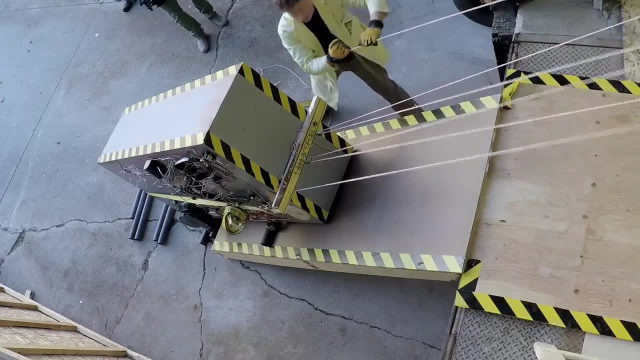 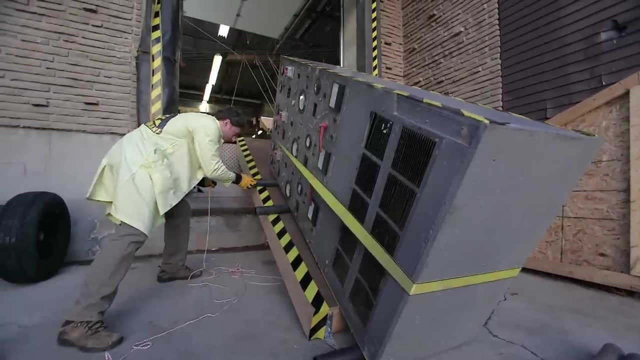 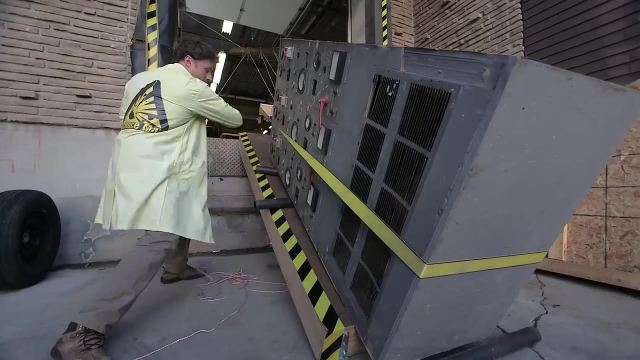 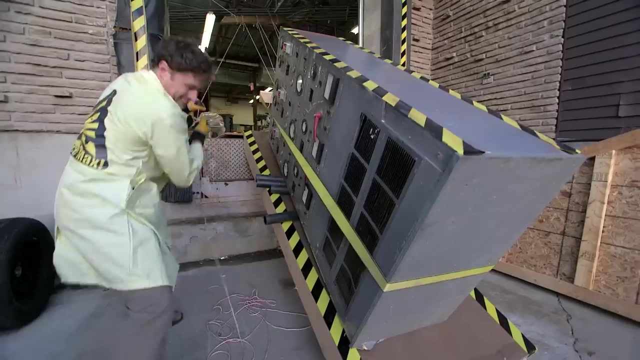 Now it's on the rollers And now I can pull it up the ramp. Now I got to carefully. OK, Put new rollers underneath as I go, Pull it up the ramp Roller. I know what you're thinking. It still seems pretty difficult. 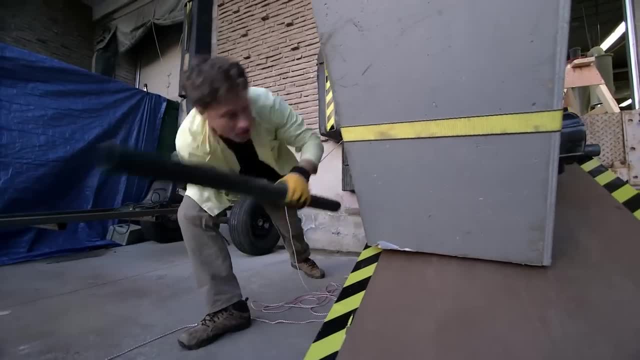 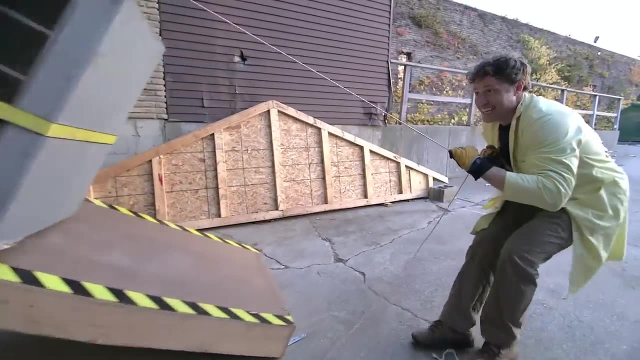 If only the simple machines could give me longer arms. Well, they can't do that, But what they can do is give me the strength to do this heavy job with no one else around but me. Hopefully that won't be a problem. 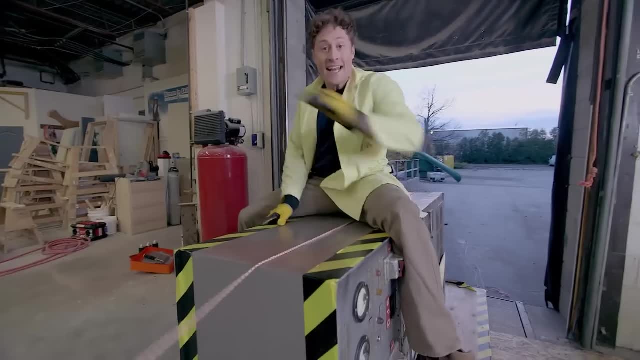 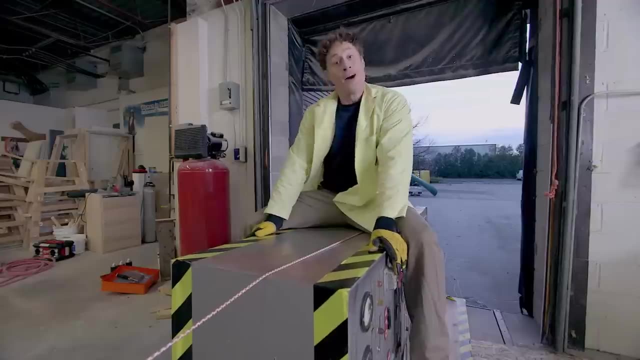 There we go. I did it All the way across the parking lot and up onto the loading dock with the help of levers, rollers, ramps and pulleys. The hard part's done. Now I just have to get it into the lab. 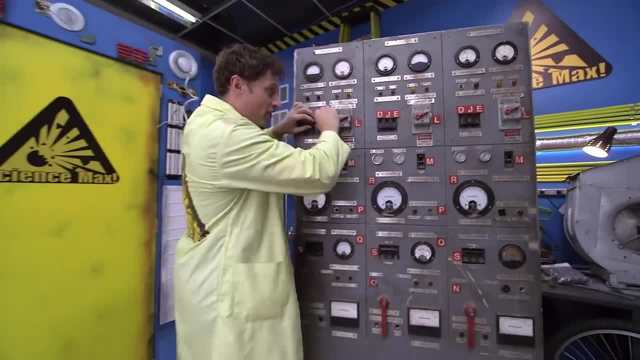 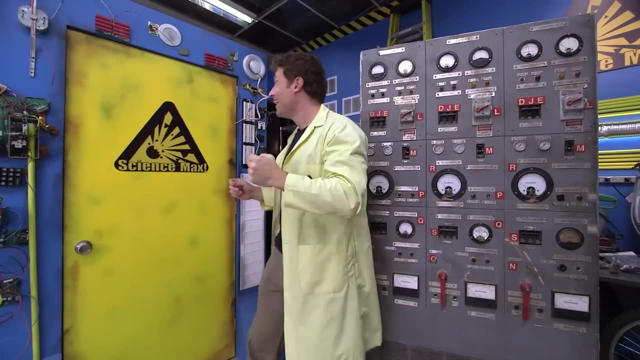 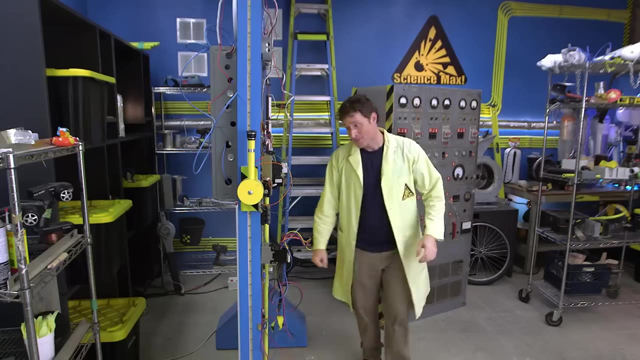 All right, All right, Let's see if all that effort was worth it. I think it's working Well. there you go. Thanks very much for joining me on Science Max Experiments At Large. I think I'm going to go home because it's been a long day.